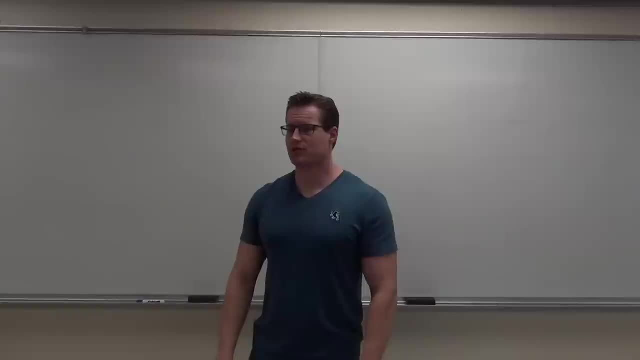 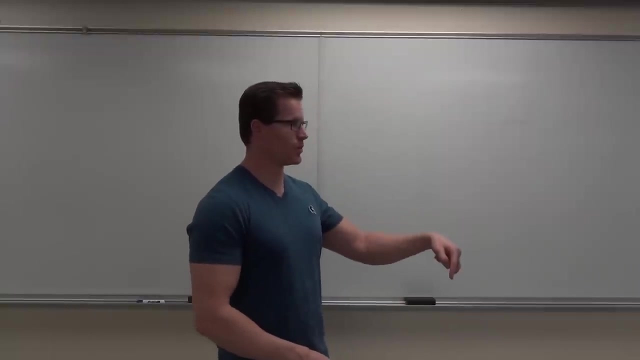 what if it's not just sine to the fourth power of x? What if it's sine to the fourth power of x times cosine to the fourth power of x, or something weird like that? Well, we're going to talk about that exact example and I don't know if we're going to get there today. 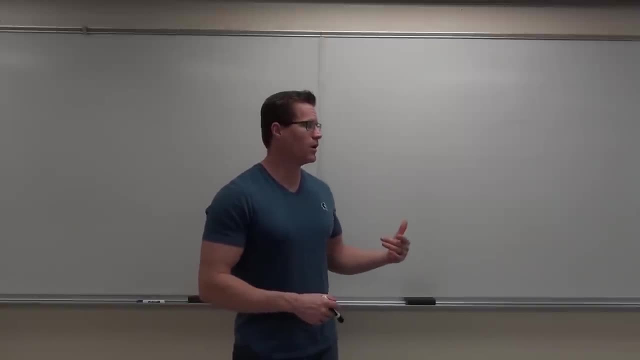 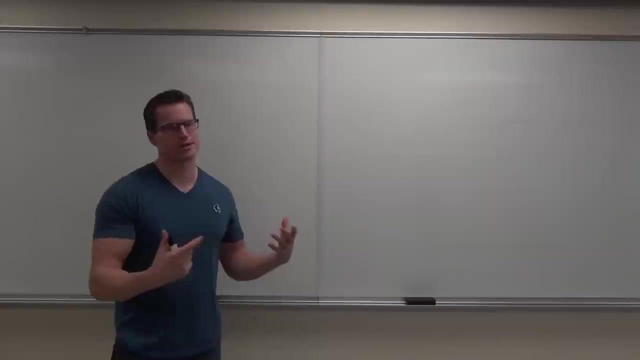 but we're going to talk about it eventually, probably next time, probably tomorrow when we get back at it. We're going to see what happens in these cases when we have trigonometric functions being multiplied certain powers inside of our integrals. It's going to get. 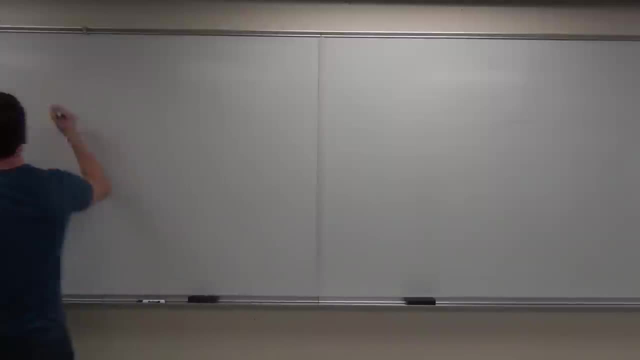 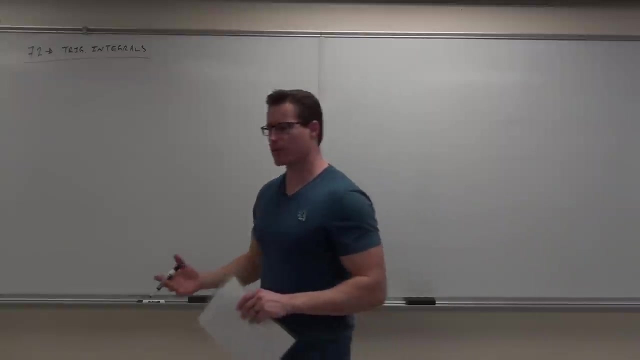 kind of fun. It's going to get a little weird, It's going to get crazy, but we're going to have a good time with it. 7.2, we're going to talk about trig integrals. You know, the one we're going to start off with first is a very common one. We're going to start 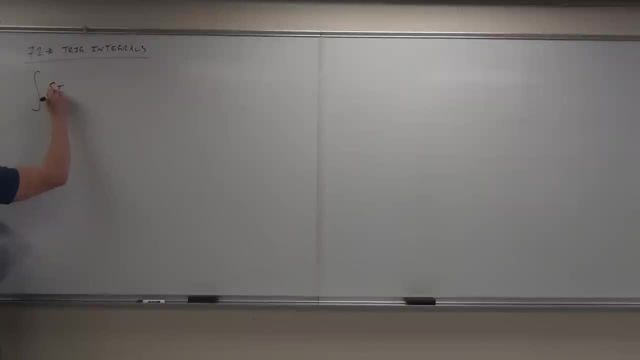 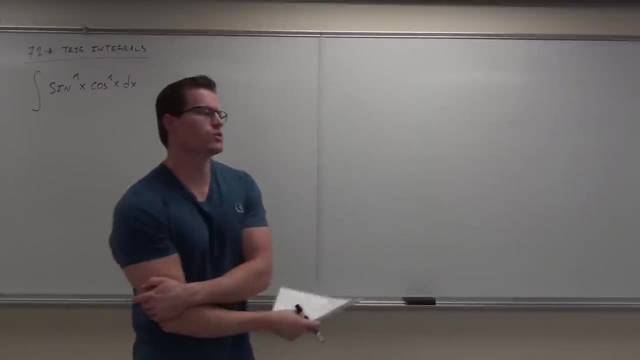 talking about what happens in your integrals when you have sine to a certain power and cosine to a certain power being multiplied together. So sine and cosine don't necessarily have to have the same power They could. but I want you to consider the two cases that we're going to talk. 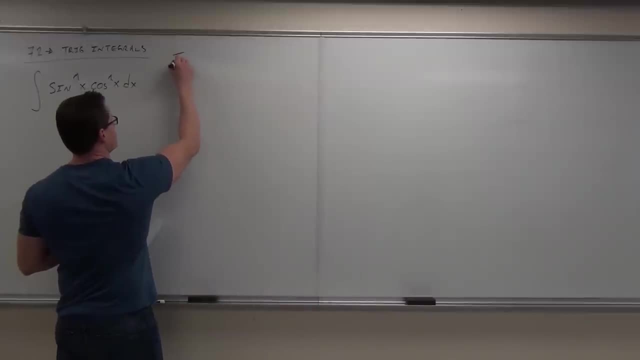 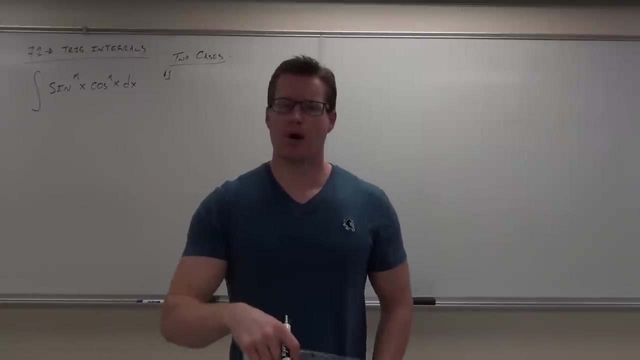 we have. okay. so here's two cases, case number one. case number one is the case where we have an odd power on at least one of these functions. so either M is odd or n is odd, or both are odd, you guys yet I know it sounds silly, but you know. 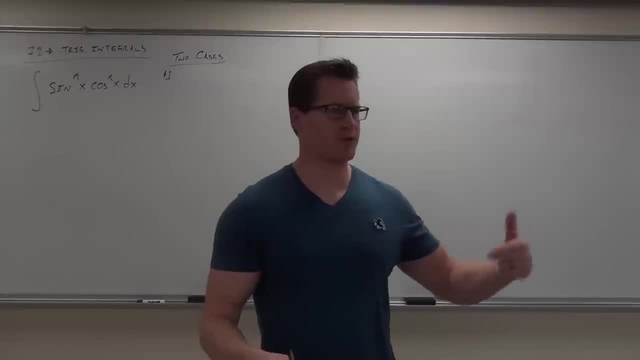 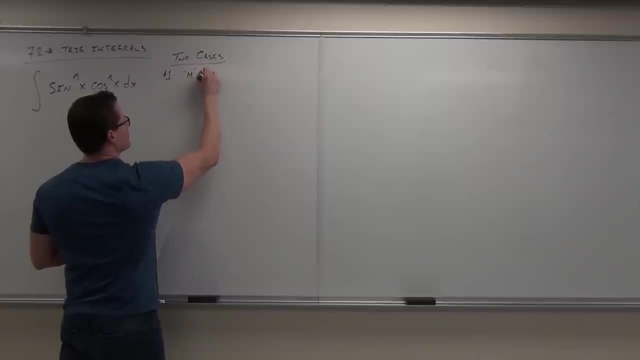 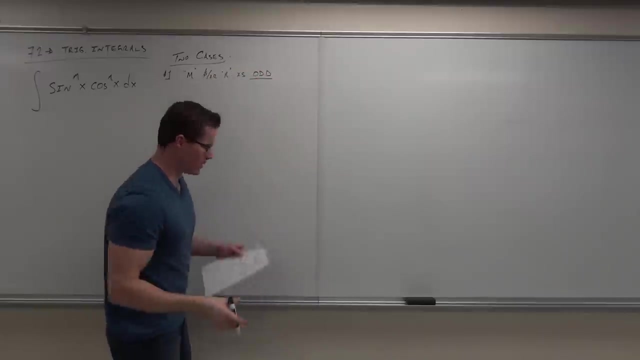 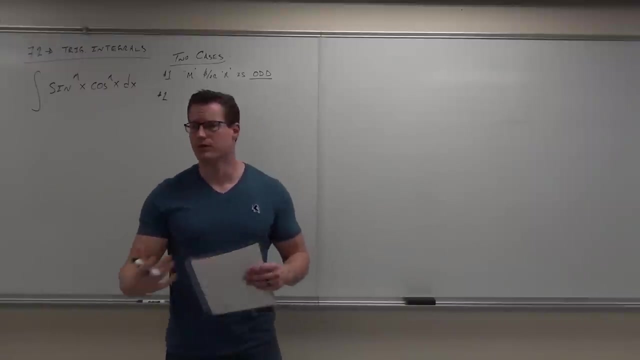 what odd means? yes, odd is like one, three, five, seven, nine. those those powers. so case number one is where M and or n is odd. so they get both the odd. what's the only other case? they're both even. yeah, see, if one of them is odd, naturally the 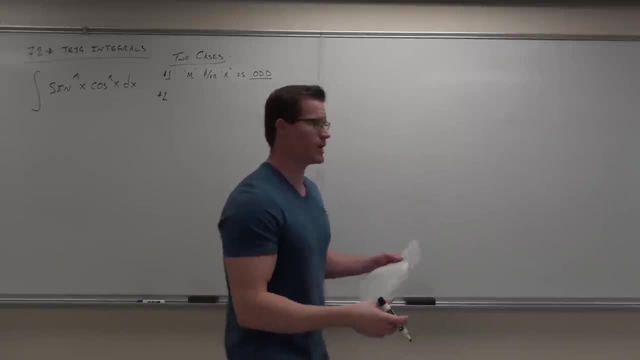 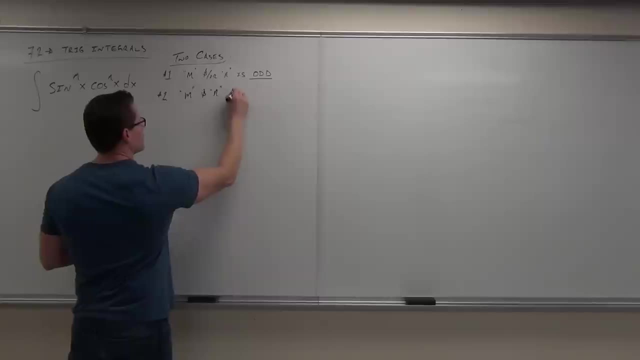 other one's gonna be even. hello, if they're both odd, none of them are gonna be even. but if none of them are odd, they're both even. so M and n are even. of course, I'm not gonna leave you hanging, we're gonna talk about both. 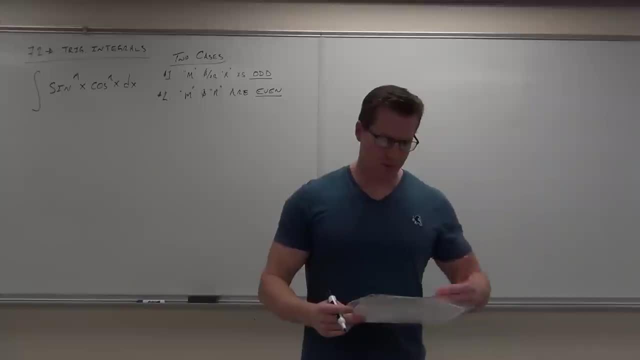 cases here, what I'm gonna do for you. I'm gonna give you the the case by case, to tell you exactly what to do first, and then we're gonna follow those cases with a series of examples. that's not okay with you. so let's talk about case one. 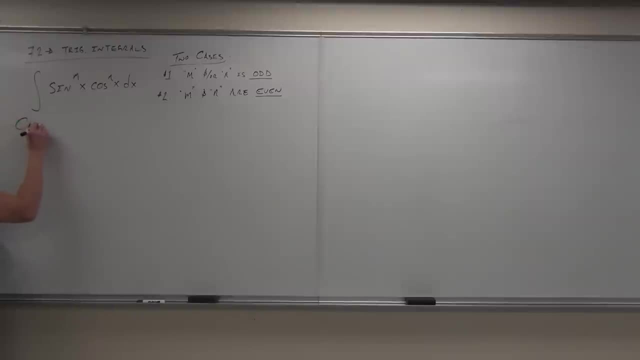 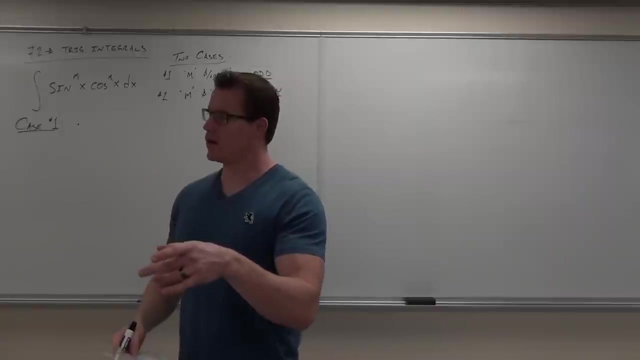 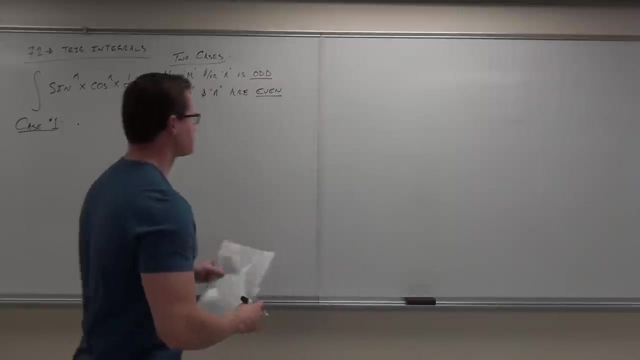 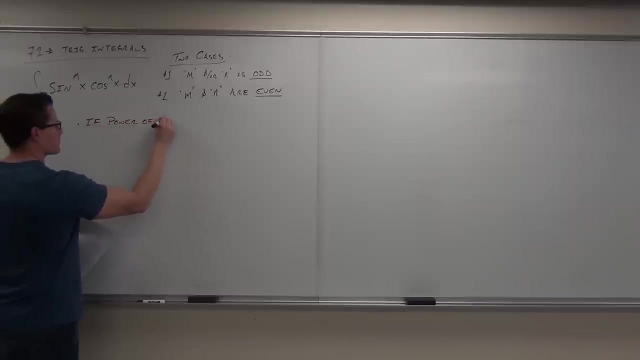 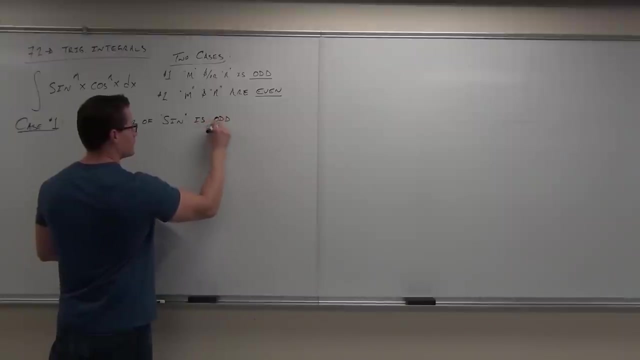 first, case, number one, let's suppose. so case number one: either M is odd or n is odd. so either sine has an odd power or cosine has an odd power, or they both have an odd power. if sine has an odd power, you. if power of sine is odd, what we're gonna do? we're gonna strip off one of the 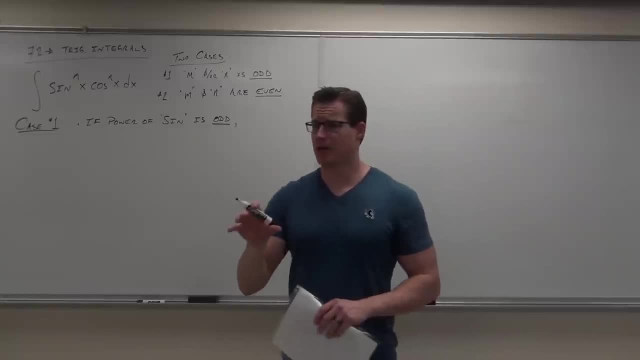 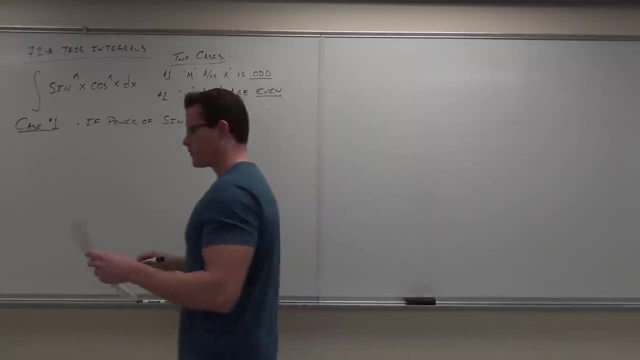 signs, so that what that means is like if it's sine to the third power of X, we'd strip off one. we'd have sine squared times sine. does that make sense? we're gonna strip off one power, so we're gonna keep one factor of sine you. 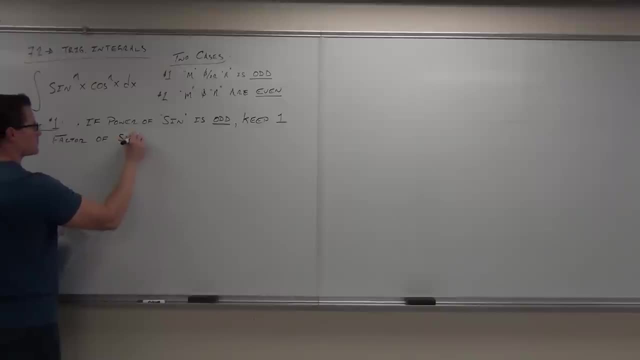 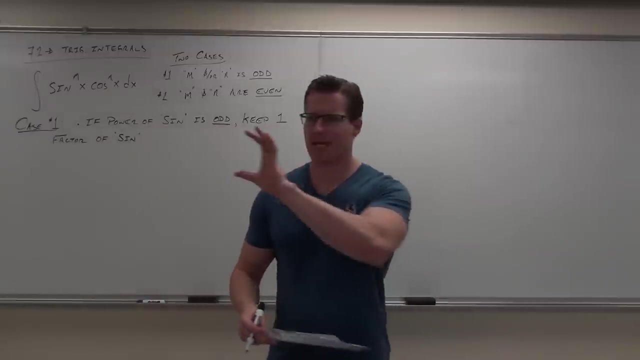 omit that, because sine is not always an equal power, because sine is an equal power, you know. so that's why we have three-dimensional functions where it depois either these six, there's all four points, they're all equal, so they're all 지를als. so what we can do, if there's anything, we've drawn a square between: 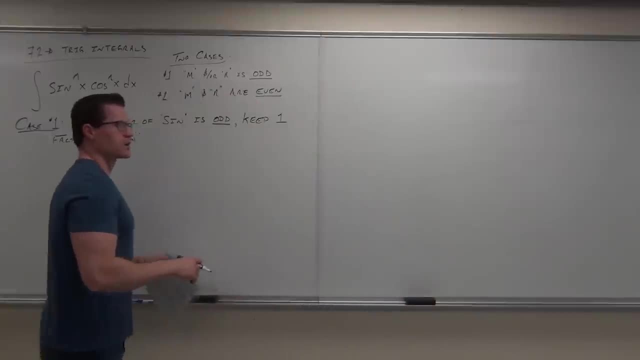 them. we can is use sine there, these two things more. atah, if we're done, even ones. you see, if we have an odd power of sine and we take one sine away, we strip off that factor. the net odd power now becomes an even power, doesn't it, if it? 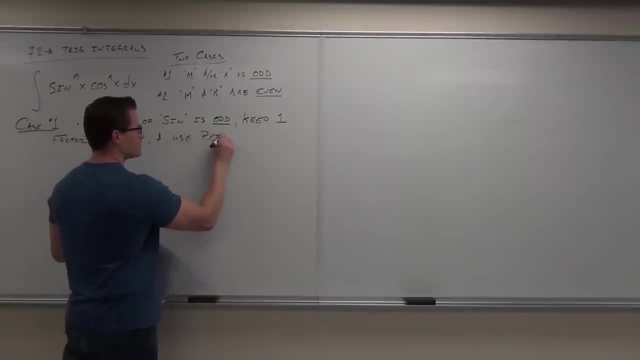 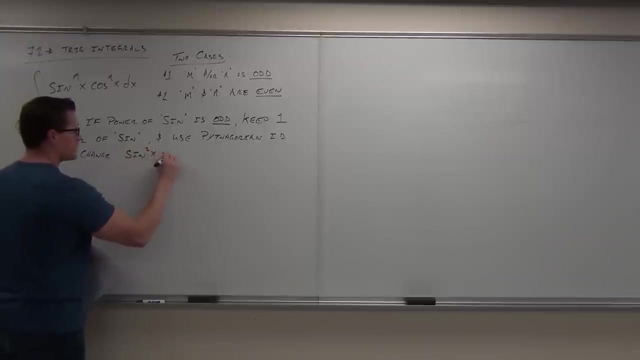 becomes an even power. we can do a couple things with it. we can not, I'm sorry, not a couple once you one thing with it. so we're gonna do so. keep one factor sine and you. So this is a Pythagorean identity. to change sine squared x into one minus cosine squared x. 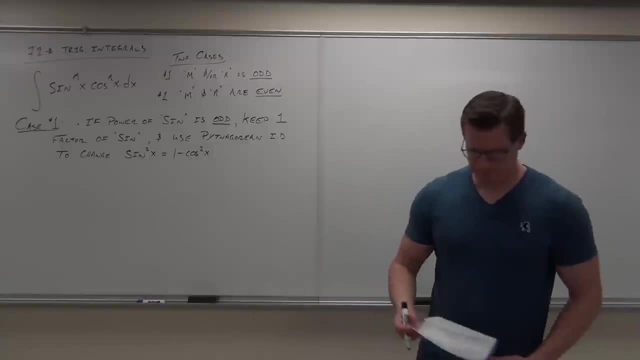 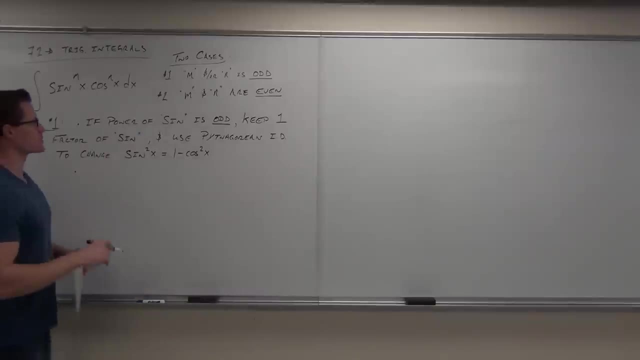 You'll see why this happens, why this works, in just a minute, while we're doing it. Okay, so if the power of sine is odd, no problem. Strip off one factor of sine, keep it. Use Pythagorean identity to change your even. 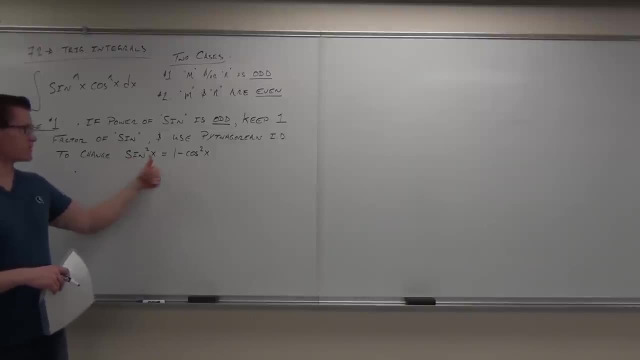 the rest of the, even into this, using Pythagorean identity. If it's sine to the fourth, well, hopefully you can do something different with this. If not, you'd still do it. You'd have sine squared, squared and you'd still use this. 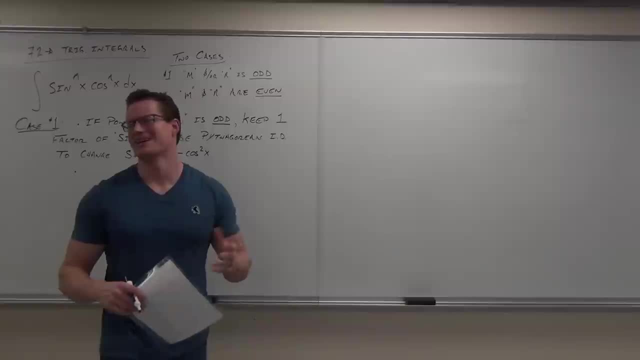 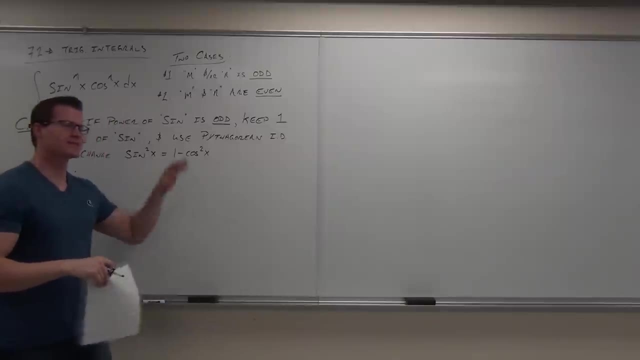 Then you'd distribute. That would be a very long, tedious problem, which we're definitely gonna get to. yay, If it's the power of cosine, that's odd. you do the same exact thing only with cosine. Does that make sense? 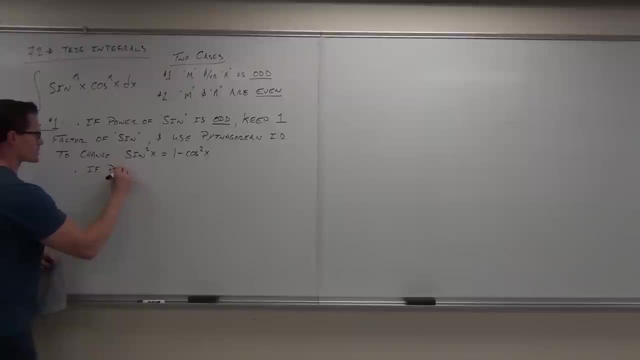 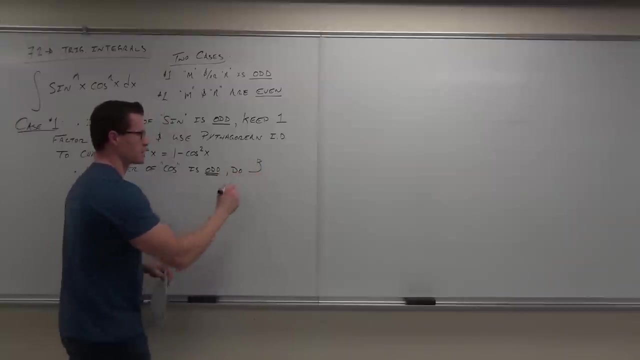 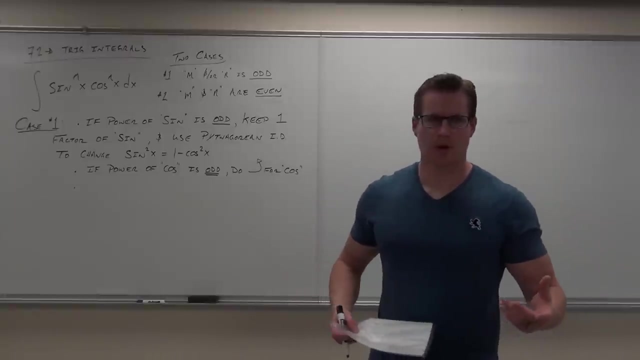 So if power of cosine is odd, do this, basically this for cosine. Now, what if they're both odd? What would you do if they're both odd? I don't know. Well, use the one that benefits you the most. 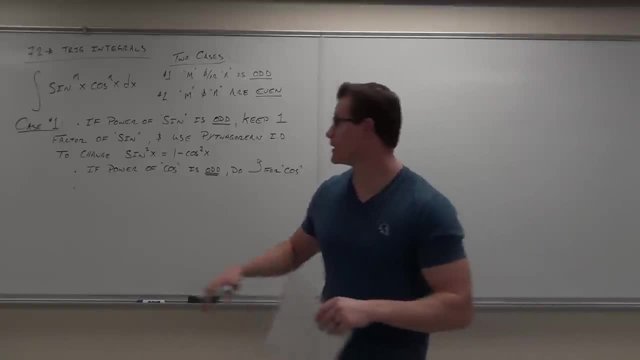 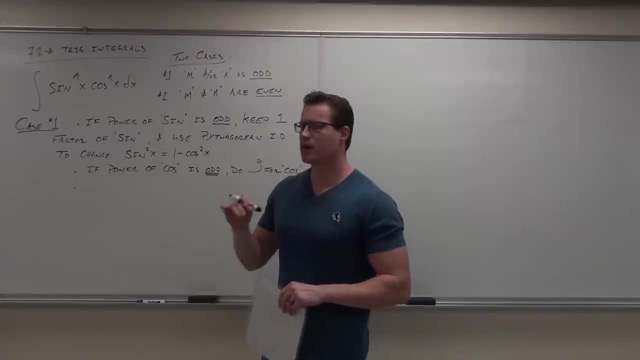 For instance, pick the smallest power, Pick the one that gives you, hopefully, a sine squared or a cosine squared by itself. Does that make sense to you? So we use the- I'd say the smaller power, or use the power that's gonna give you something squared. 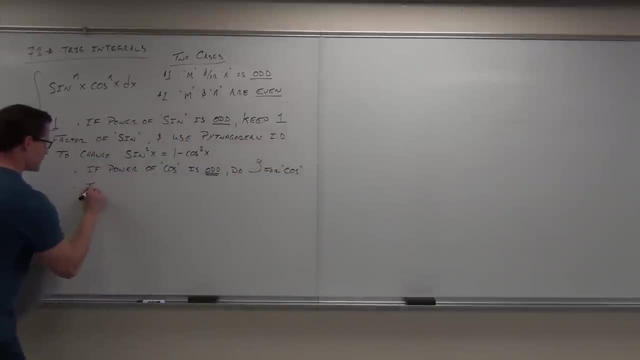 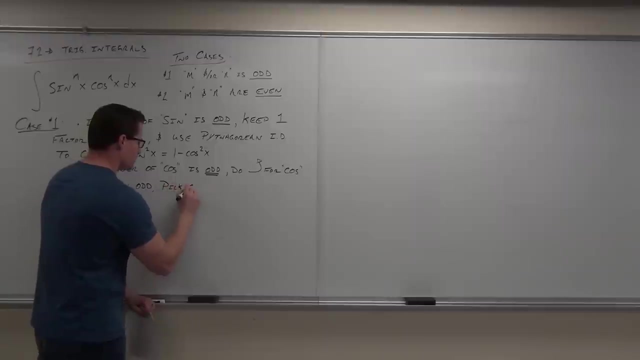 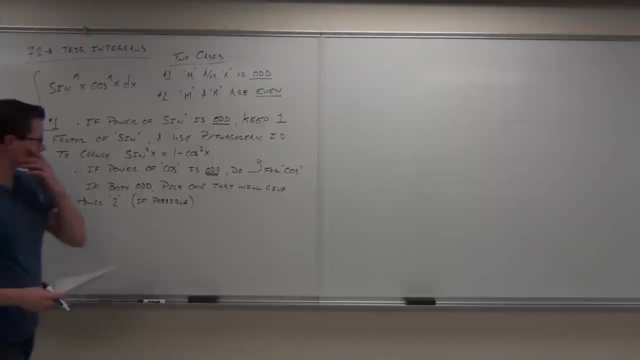 Okie dokie. So if both odd, pick the one that will give you a power of two, if you can, If possible. Okay, are you guys all okay with case one? Probably not, actually, because we haven't even done an example. 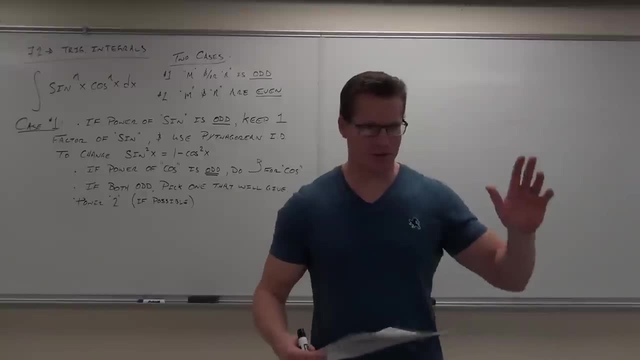 You don't even know what I'm talking about right now, except that we're gonna be stripping off a sine or a cosine. You'll see it in a minute. Let's talk about case two first, before we get to an example. Definitely wanna do at least two of these things. 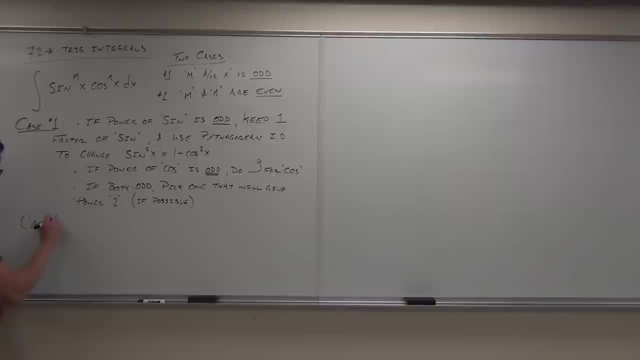 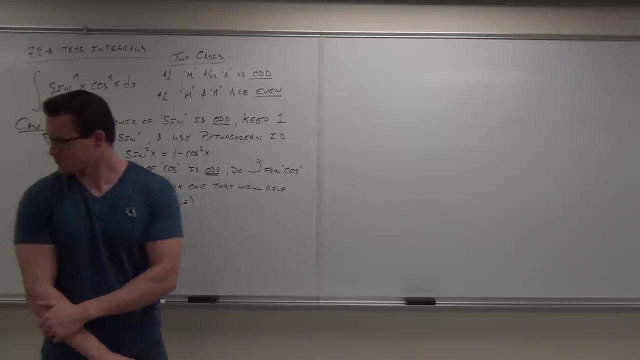 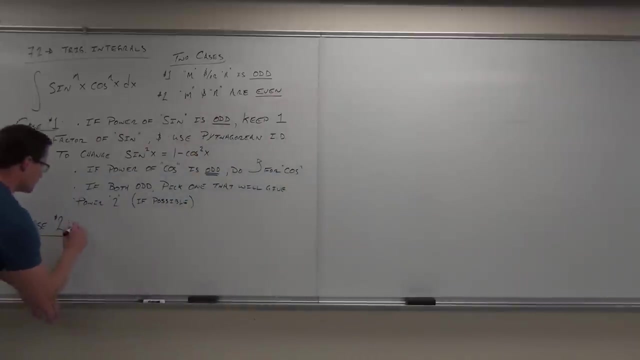 before we're done today. So case number two. For case number two, Let's say that both the powers of sine and cosine are. even If both powers are even so, cosine squared and sine squared, you've got both of them. 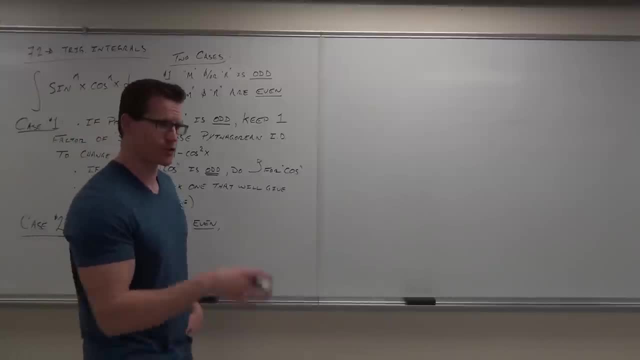 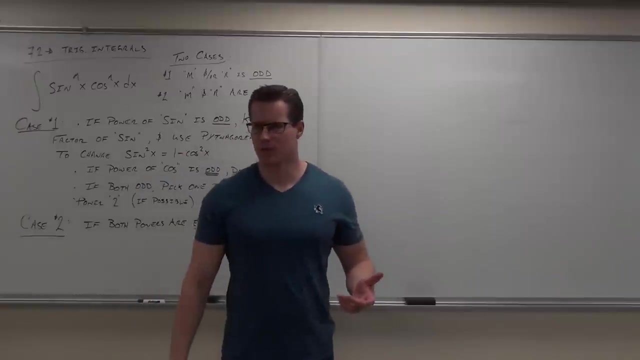 What we're gonna do is we're gonna use our half-angle formulas and you're hopefully gonna see why in just a minute. Use half angle formulas, Do you? does anybody have to remember the half angle formulas? Do you remember what they are? 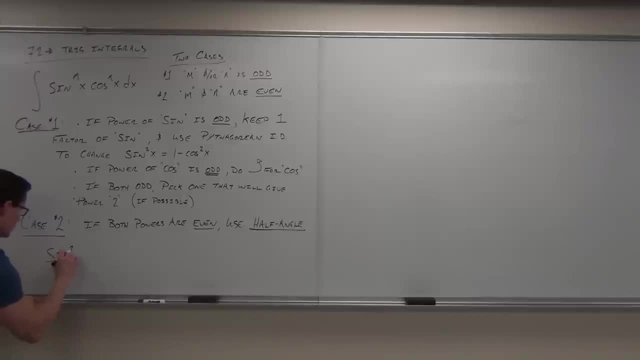 Some of you might. They're actually really, really, really similar. For sine, we'd have a one half. For cosine, we'd have a one half. For sine, we've got a one. For cosine, we've got a one. 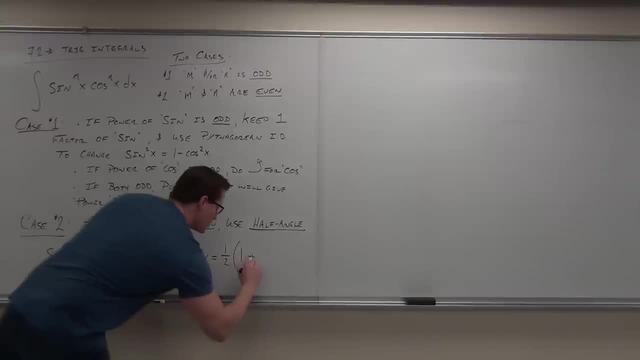 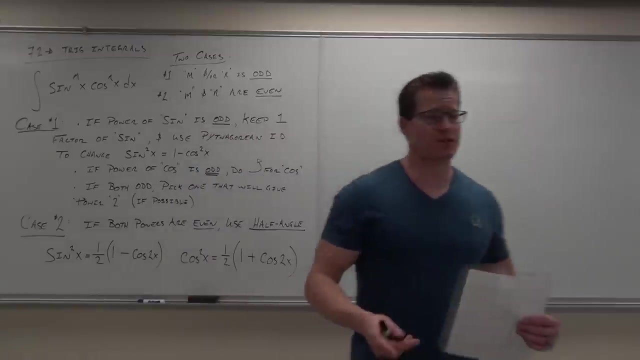 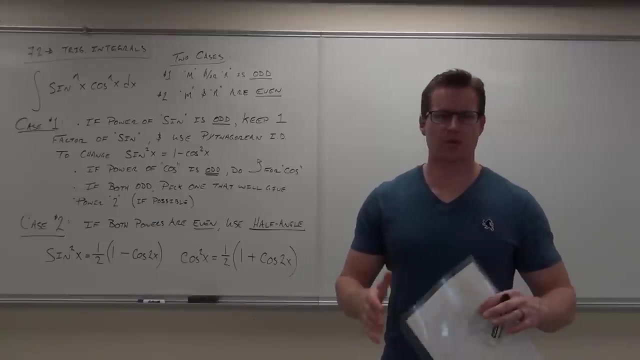 For sine we have a minus. For cosine, we have a plus, But for either of them we have a cosine 2x. Now I'm wondering if you see why this helps us Change it. Chain rule works for derivatives. 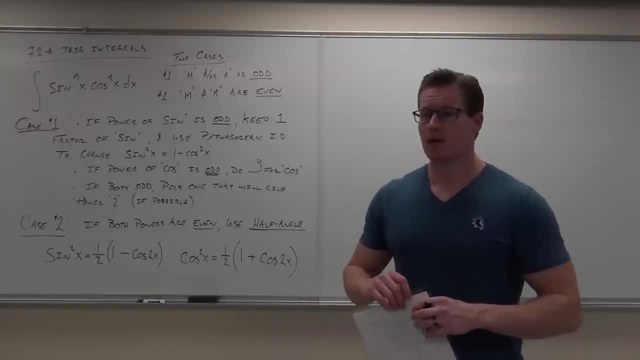 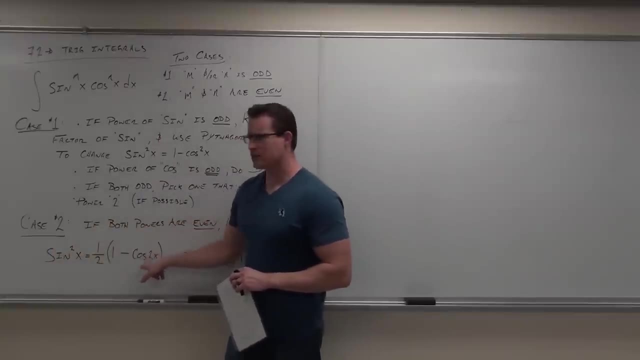 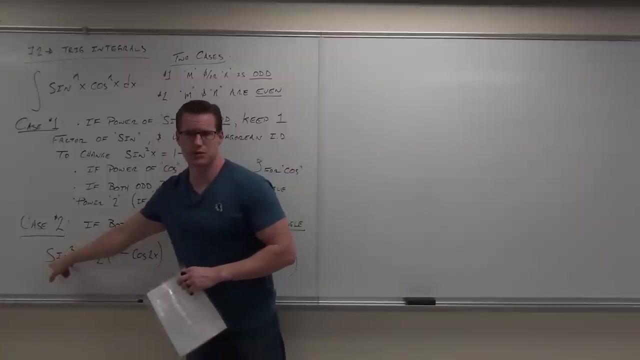 What are we doing? Substitution, Aha. So can you do this derivative by itself? No, But if you change it can you distribute that Easily. Can you do this? integral, Yeah, Integral here, Not so much, unless you want to do the reduction formula. 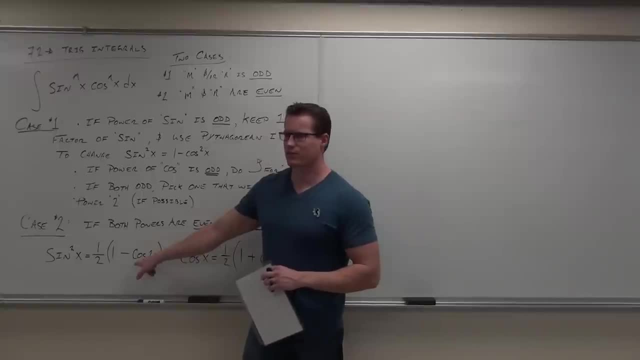 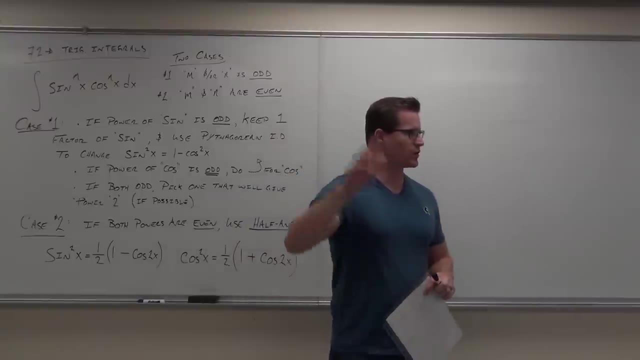 You can do that. I suppose Integral here Piece of cake. Very easy, because that's just a simple little substitution. You'd probably do it in your head and then you're done with that. So can't you be okay with that one? 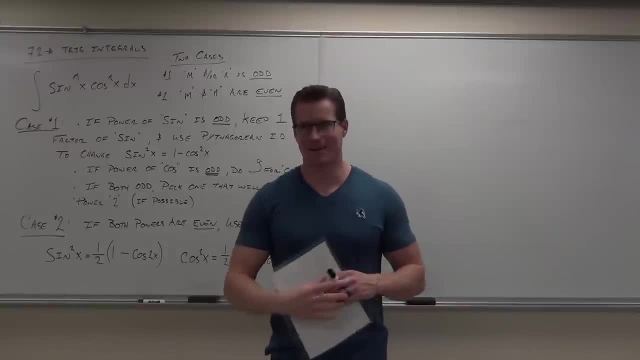 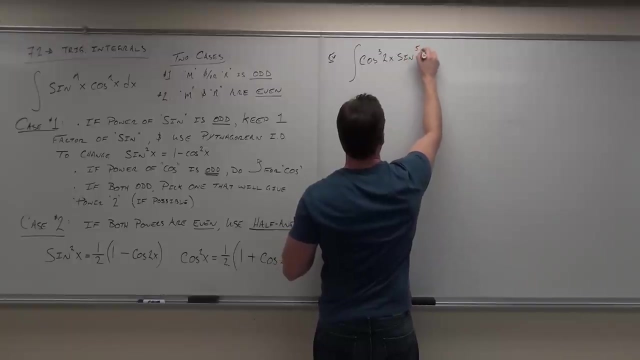 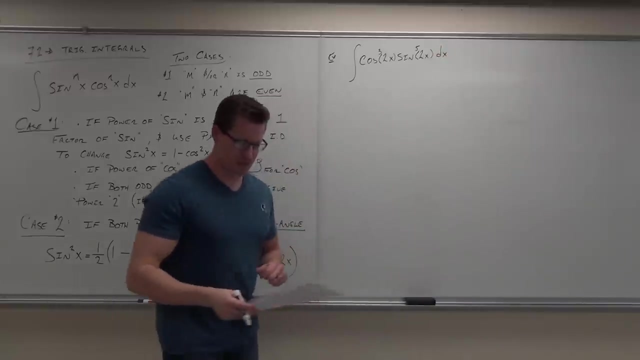 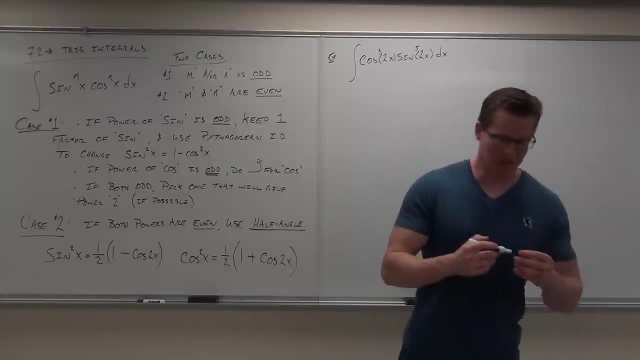 Good. Would you like to see a couple examples? Let's bring it on right. So, So, let's consider that. Okay, Let's go through the whole process. okay, First things first. Does that fit in our integration table? 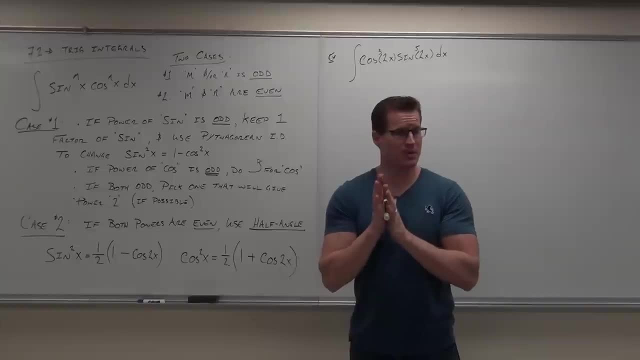 No, Will you do a substitution? Maybe, I don't know. yet We don't know What this is designed to do. is make your integral possible, okay, So we're going to manipulate this thing until it's possible. So notice, we're not doing hardly any calculus at all right now. 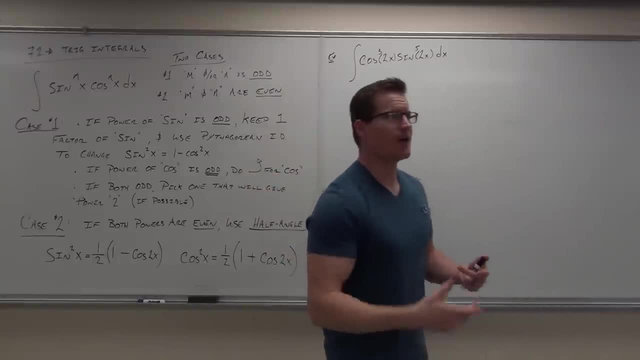 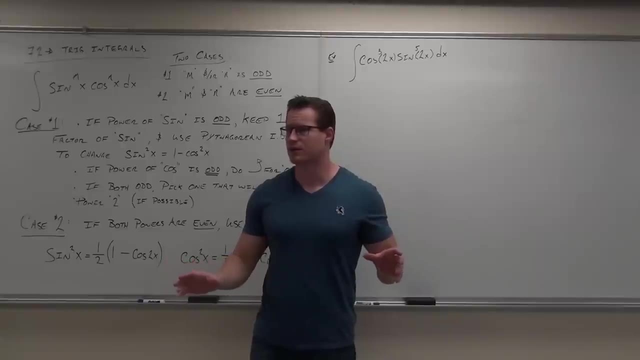 All we're doing is using some identities, breaking this stuff up and then trying, hopefully, to use a substitution. So let's see, Is it definitely gonna be integration by parts all the time? No, not necessarily. So check it. 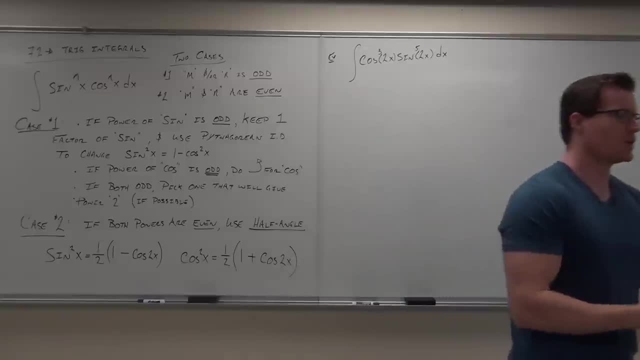 What do we have here? Do we have a case one or a case two? Case one: Okay, we have some odd powers. If you have an odd power, you're in case one, no matter what. okay, So case one. In this case. they're actually both odd. 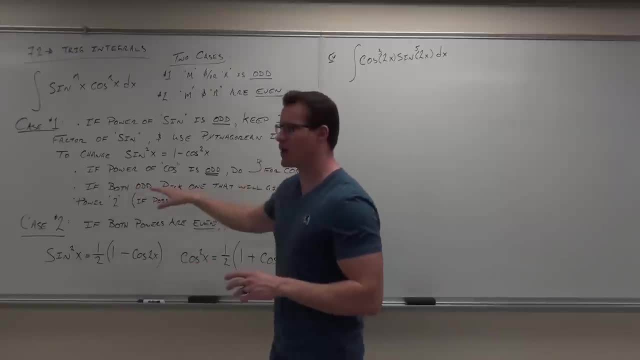 So what we're gonna do is we're gonna look down here. If both are odd, pick one that will give a power of two. So what I like to think of it, pick the smaller one. That's gonna be a little easier to deal with. 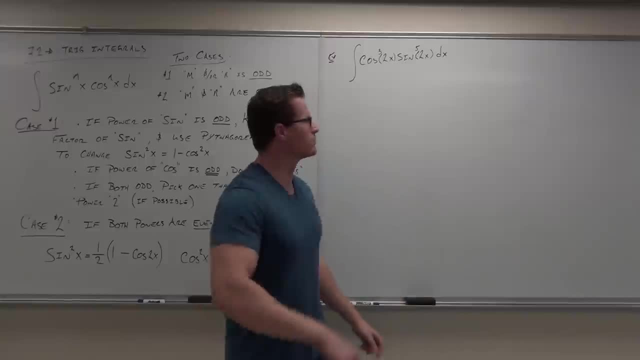 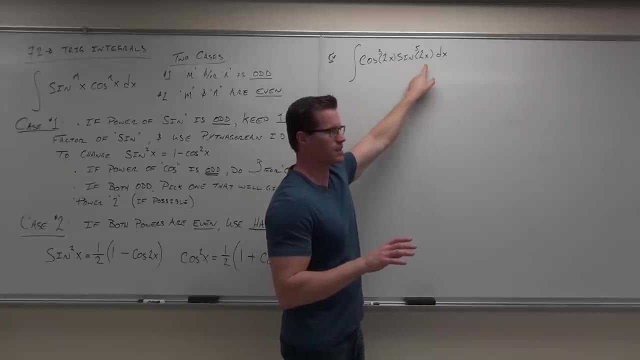 because you can substitute out with the other one. So okay, we got cosine to the third, We got sine to the fifth. Fortunately for us, they have the same argument. If they didn't, it'd be crazy. all right, 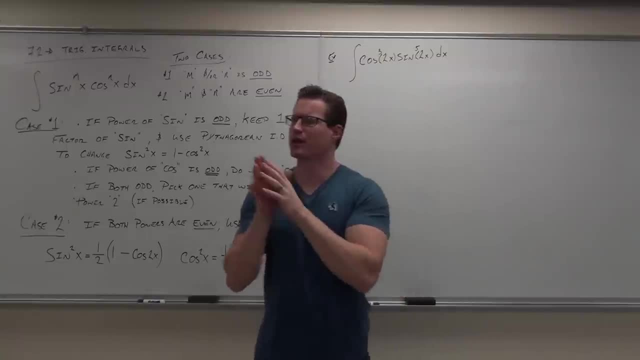 So we're gonna leave it the way it is. We're gonna look up at our powers. What one would be our appropriate- I almost said stripper, our appropriate stripper here? The stripper-offer. which one do we wanna strip off The sine or the cosine? 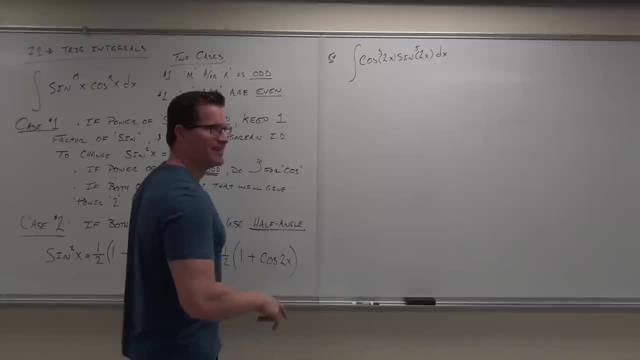 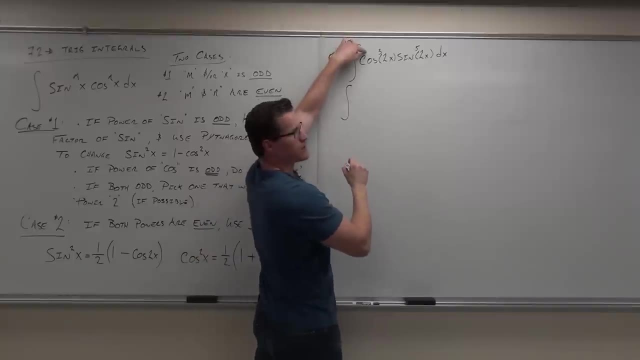 Cosine, Cosine. I'm not gonna edit that, by the way. That's funny. So, So, cosine to the third power. No, no, no, What I'm gonna make this? I'm gonna make this cosine to the second power of two x. 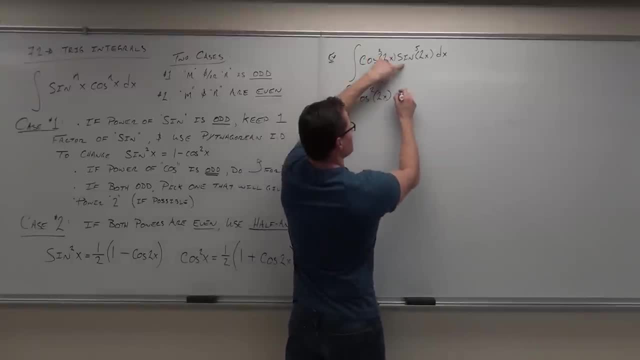 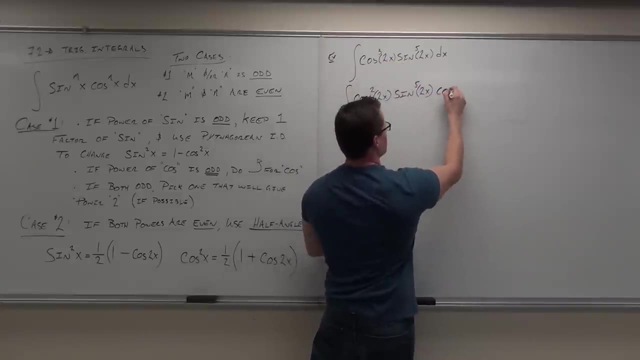 What's the way I do this? So hopefully this will make sense to you. I'm gonna write the sine to the fifth power. We're gonna leave that there. I'm gonna put the extra cosine that I stripped off over here. Don't lose track that this is actually cosine of two x. 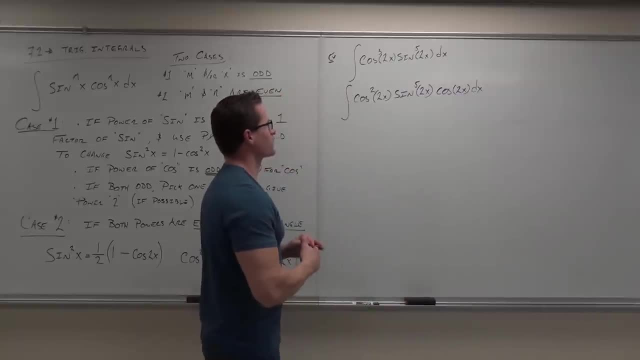 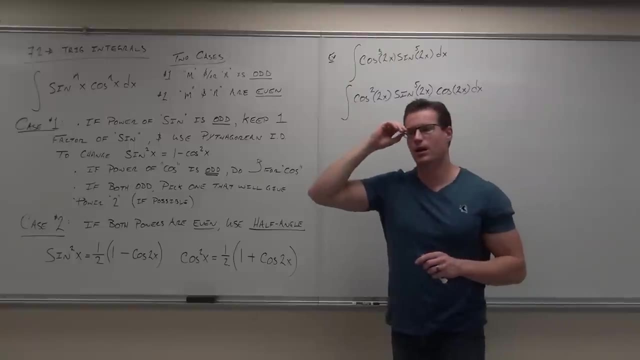 Don't lose the argument. Okay, it is two x there. Okay, I wanna see if you guys understand that this is exactly the same as this. These two things are the same Show of hands. if you're okay with that, Good deal. 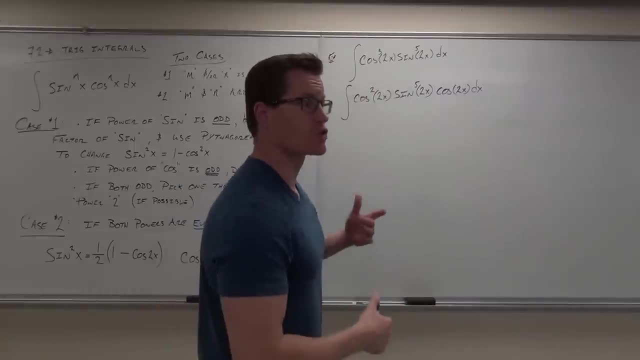 Now, why did we do it? Well, check it out. Now that we have a cosine squared in there, we change it from an odd to an even Cosine squared. we have an identity for that. So, instead of cosine squared, we go no, no, no. 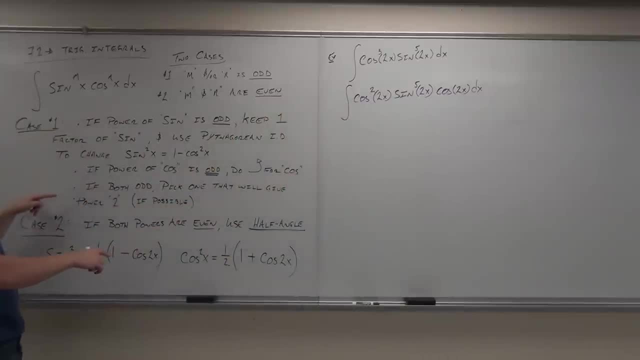 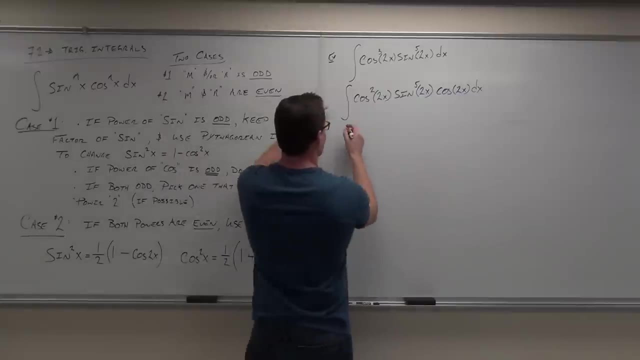 Well, cosine squared, it says: for odd powers, try to use the Pythagorean identity. Okay, well, that's this. or the reverse. Cosine squared equals one minus sine squared. So cosine squared of two x no, this is one minus sine. 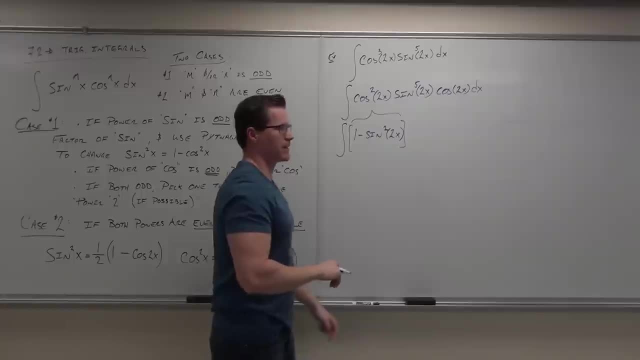 This part is this part. Pythagorean identity says so. Don't forget about the two x. I can't stress enough how important that is. Some of you people who don't do well in the chain rule, you need to do well here with substitutions. 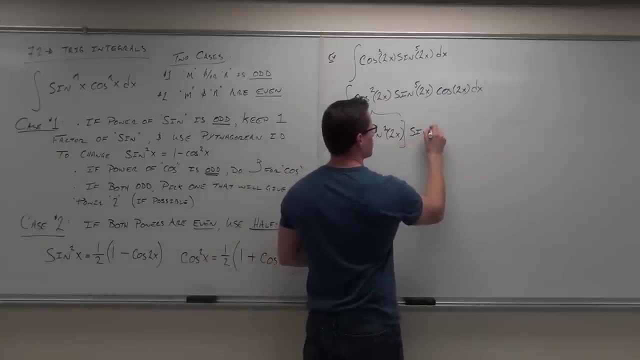 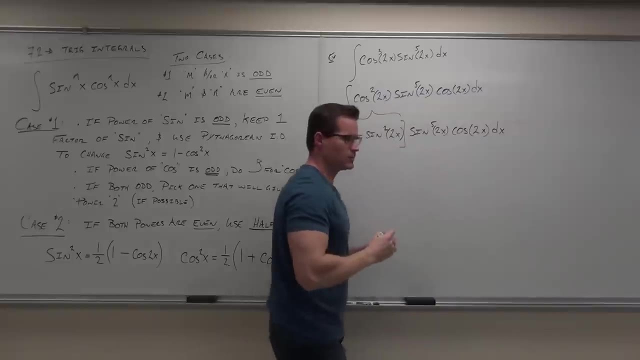 You need to keep an eye on it. After that, we have sine to the fifth power of two x. We've got cosine of two x dx. Okay, I wanna make sure you're still okay with that. Are you all right with it? 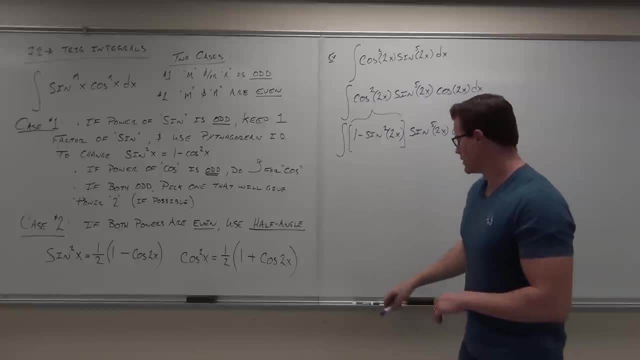 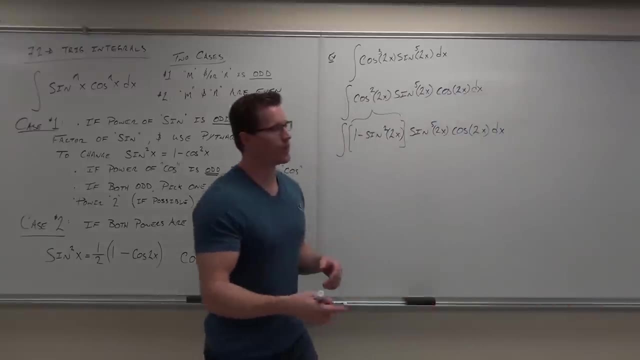 Have we done any calculus yet? No, it was just trick, just some trick. Just some identities actually. Now, here's the cool, here's the awesome thing: As soon as we do this, check it out. This is why we stripped off one of the cosines. 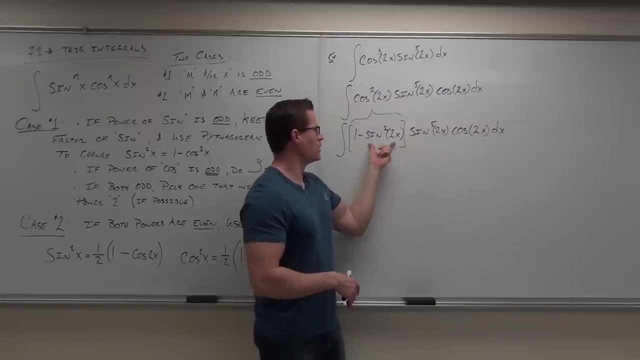 and left it over here. watch: Imagine u equaling sine of two x. What's the derivative of sine of two x? Two cosine two x. because you have a Chain rule. that's right. Do you see a cosine two x over here anywhere? 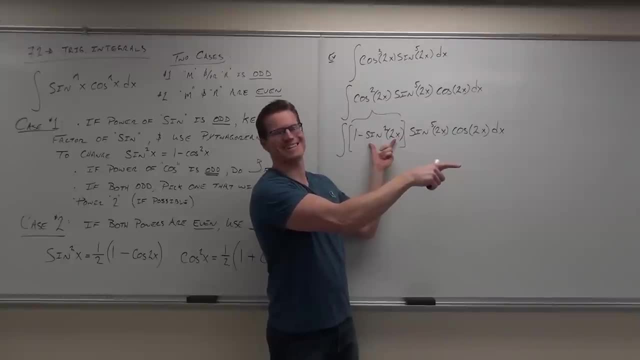 Awesome. that's why we do it. So when we get this, check this out, see how this works. You don't have to distribute this right now. Don't be crazy. Leave it just like this. This is the derivative of sine of two x. 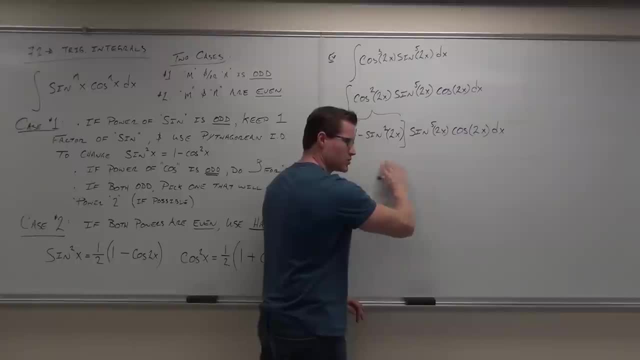 What's the derivative of sine of two x Negative? Just like this Watch. here's why, If I pick u equals, look, don't pick with substitutions. With substitutions, you go through the whole process. Is it in the integration table? 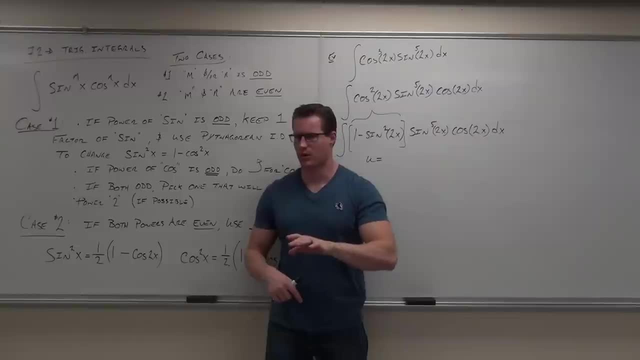 Heck no. Can you do a substitution? Yes, Don't go to integration web parts. Don't start doing crazy things. if the substitutions work right now, Pick the substitutions. Substitutions are typically on the inside of something. Remember talking about that. 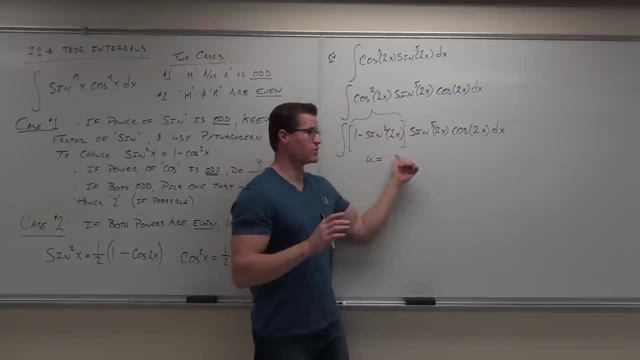 Inside of something. So it's not going to be to any power, It's just going to be sine of two x. If the derivative is there, your substitution is going to work. So pick u equals sine two x Du. 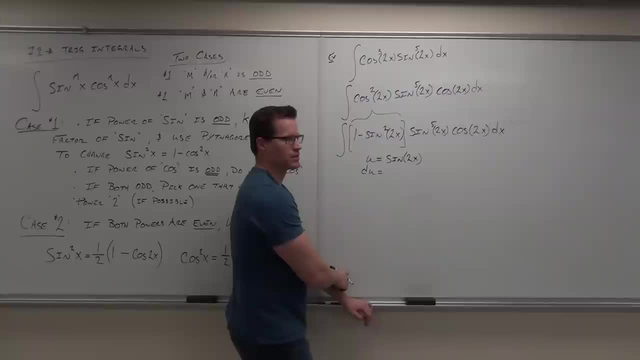 We all should be pros at this right now. Derivative of sine of two x is Two cosine of two x, Two cosine two x. Where's the two coming from? The chain rule, The x, The chain rule. I know many of you have done substitutions two different ways. 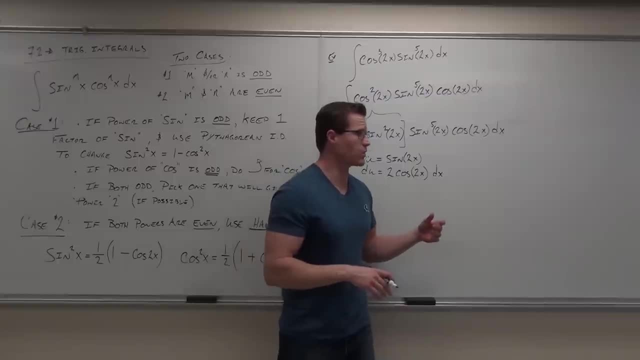 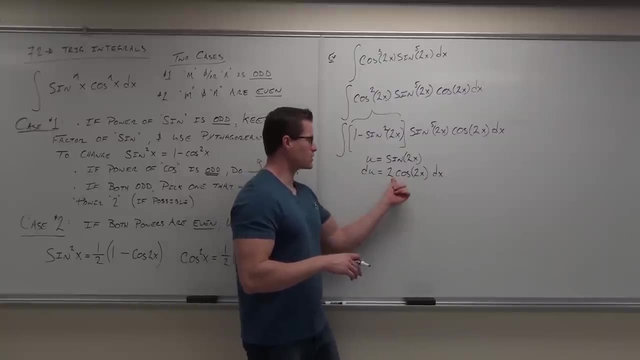 Since I've been teaching you two different ways as well, I'm going to stick with that. There's two ways to do this. You can solve for dx completely and get du over two cosine two x. Or you can just divide by two and get du over two equals cosine two x dx. 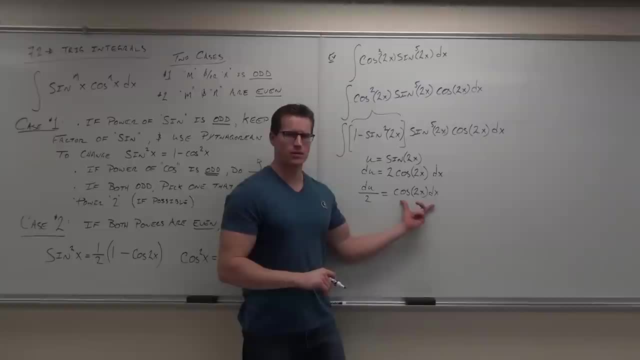 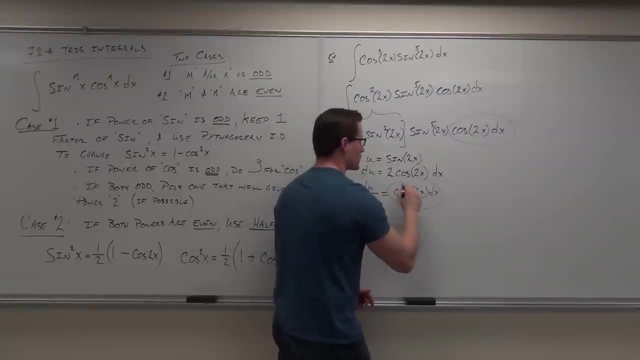 Hey, do you see this anywhere in our integration? Yes, That's why we put it last. Put it last because it sticks out like a sore thumb. This thing is right here. What that means for us is our integral is going to get really, really pretty right now. 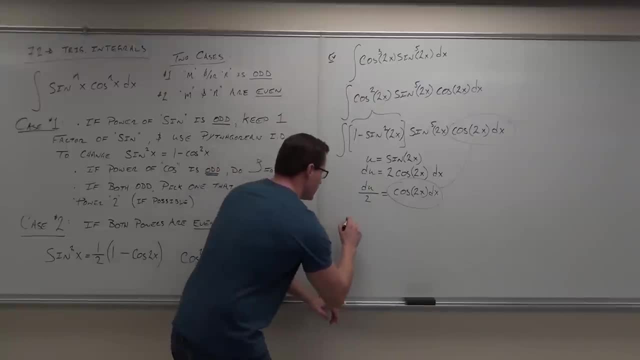 Let's see what we've done. Do we still have an integral? Yes, Do we still have a one? Hello, are you with me? Yes, We still have a minus Instead of sine of two x squared. what's this whole thing going to be? 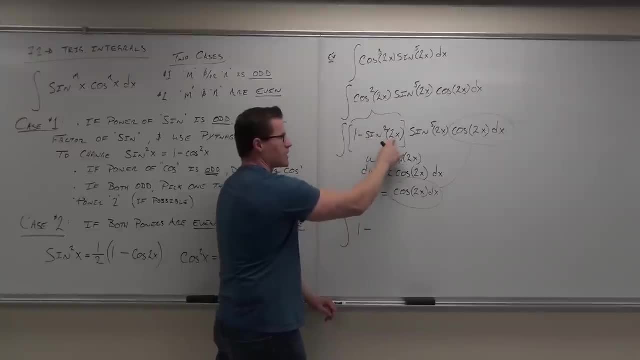 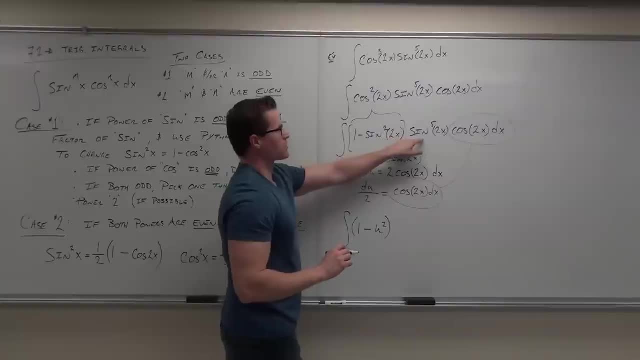 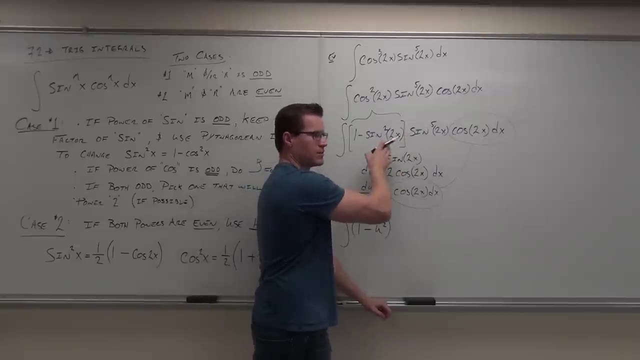 Brackets. Now they're number one AND number two. This is what you're going to have. I need to show of hands, if that makes sense to you. Now, that's beautiful. Here's why it's so nice. What do you do with the 2?? 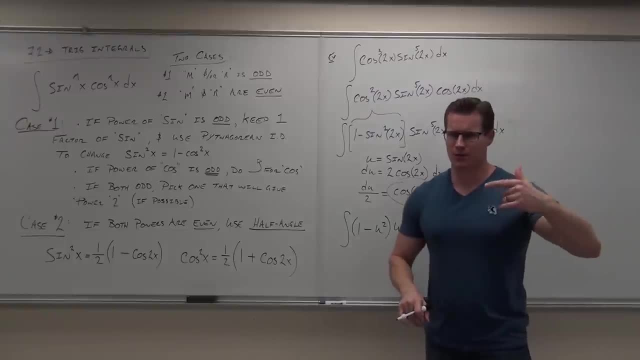 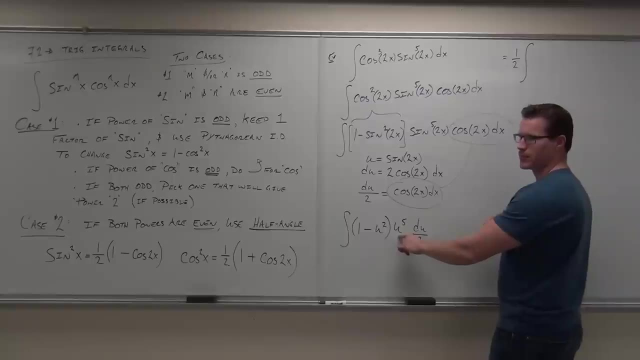 Does it become a 2 or a 1 half, 1 half, Careful on that. So 1 half integral. What are you going to do here? Distribute. This is why we wait to distribute here. We don't do it here. 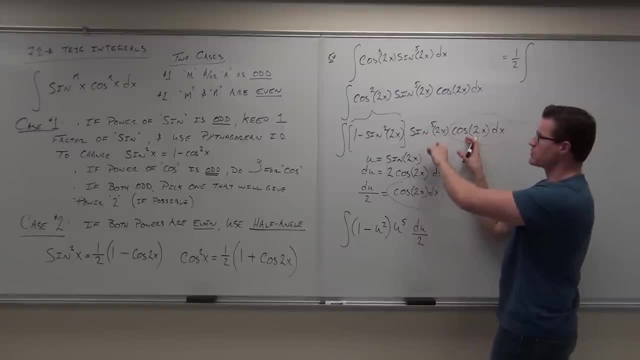 This is crazy. okay, If you had to distribute here, look at this, If you distributed here, you'd have this whole thing, and then you'd have this thing again. right, That's silly. You do two substitutions and it would work, but it's going to make it way harder, alright. 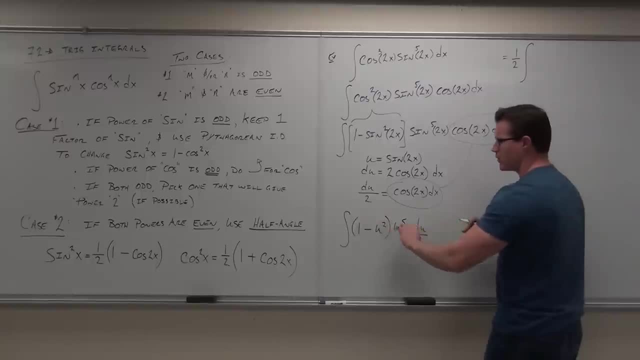 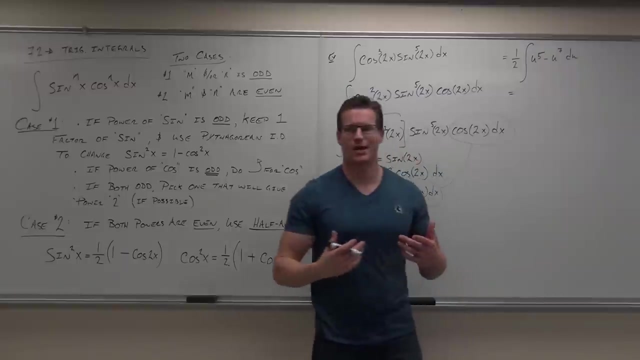 We just wait until here, so it's so much nicer. Now we can do our distribution and get u to the 5th minus u to the 7th. du Man, that's like the first type of integral you saw in Calculus 1.. 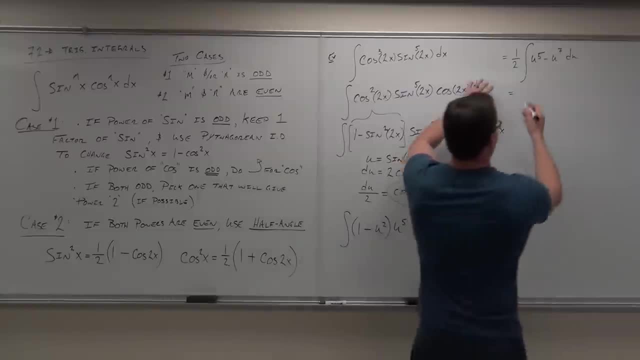 Exactly. That thing is easy. We've got a 1 half. Put your bracket there. Don't let yourself make a mistake of not distributing this later. We've got what is this anyway, U to the 6th over 6.. 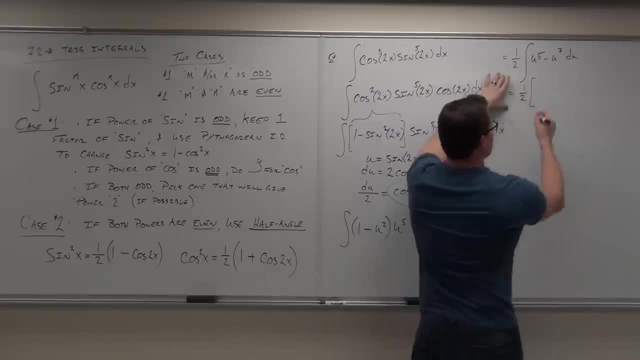 Perfect Minus u to the 8th over 8.. Are we done? No, We're almost done. We're going to do two things. What is it Distribute? We're going to distribute, So we're going to have 1 12th and 1 16th. 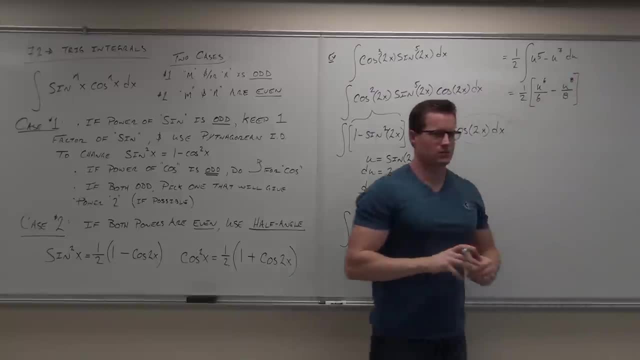 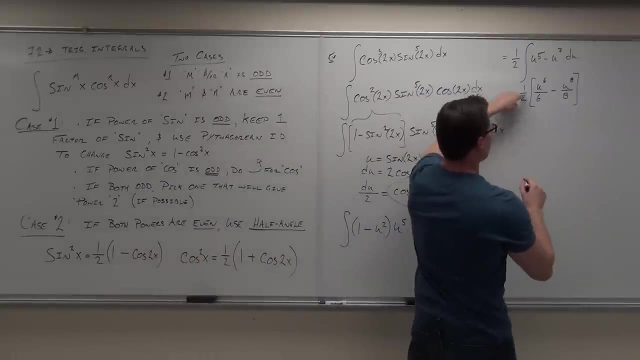 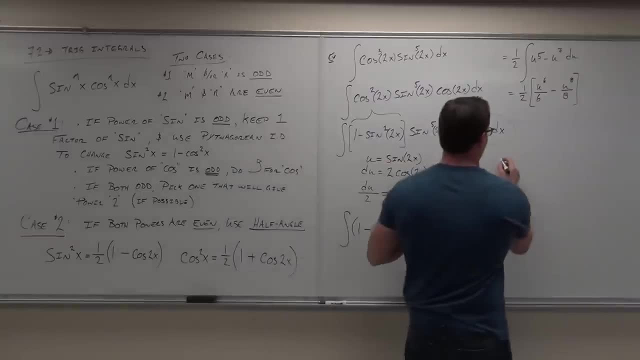 What are we going to do? Distribute, Distribute, Distribute, Distribute. Here's our u. So we're going to have here all the way down here. You can write it a couple of different ways if you want to. 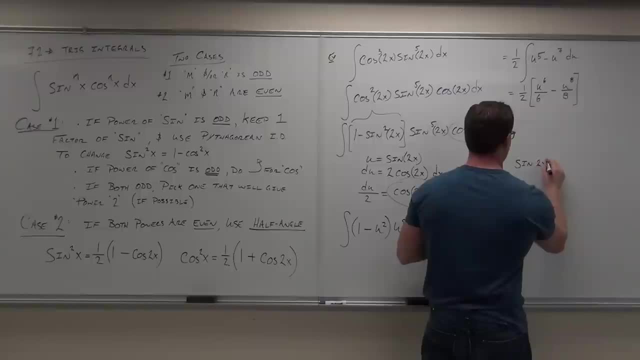 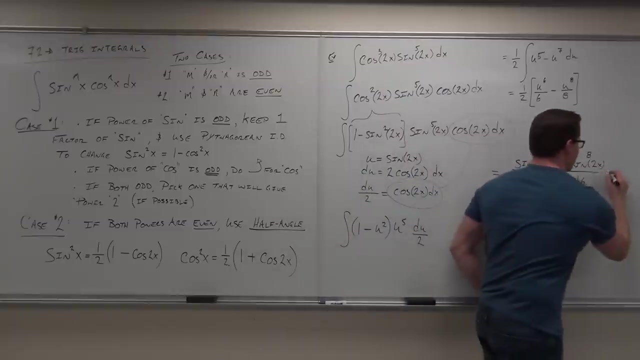 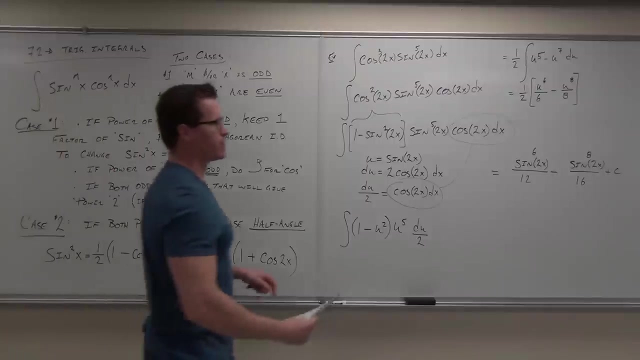 Here's one way You can do: sine of 2x to the 6th, power over 12, minus sine of 2x to the 8th, power over 16 and plus 8.. Plus c, Of course you could do. if you don't like the over 12, you could do 1 12th. 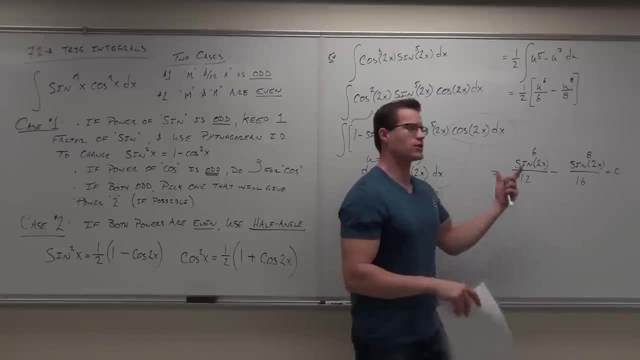 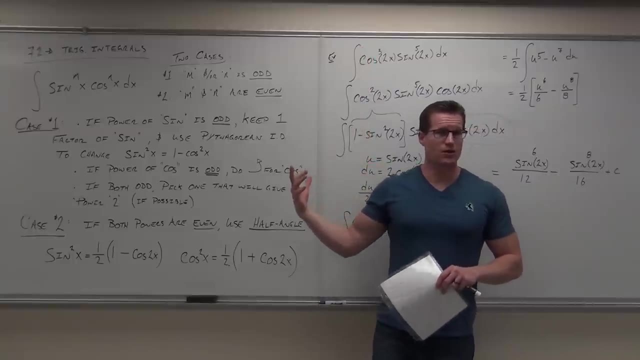 You could do minus 1 16th of 2x plus c. You could factor if you really wanted to, But this is what I'm looking for from you: Show of hands, if that actually made sense. Is it that hard? No, 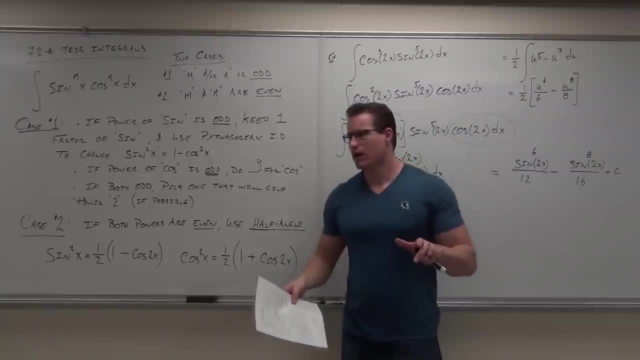 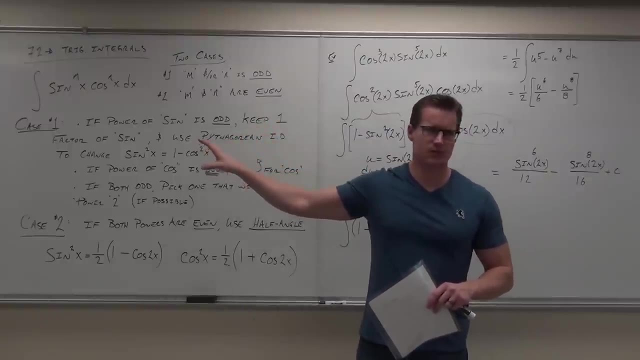 No, But here's the thing, The math here. I promise you it's not hard, It's just you've got to follow the steps precisely and you've got to be able to identify what case you're working with. The first step here is the hardest. 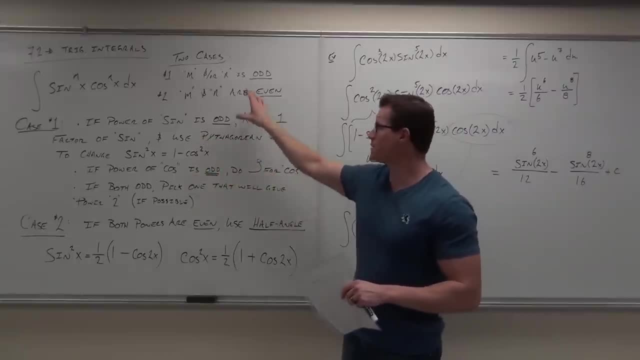 Not the hardest, It's the most important. So the first step of doing this correctly is really really key for you to get the correct answer here. If you strip off the wrong thing, it's going to take you either 10 times longer or it's. 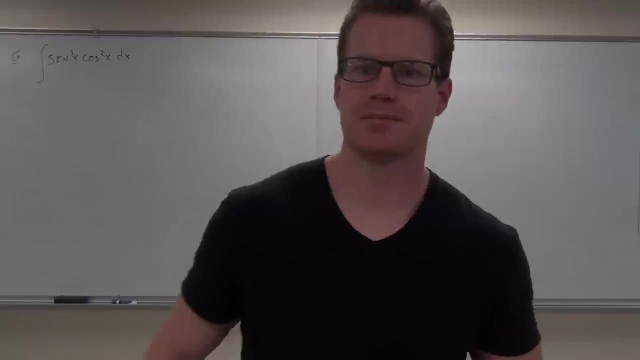 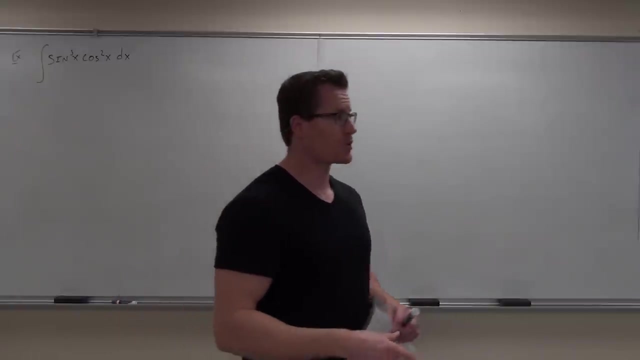 not going to work out for you, All right, So let's get started. So, what we're working on? we're going to continue working on some of these trigonometric integrals And, yeah, they get pretty hairy, But we have some cases, some ways to deal with these things that make it at least a 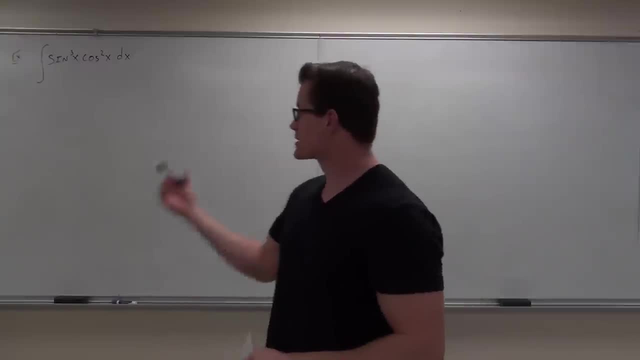 little bit nicer. We're going to use a technique, a method to go through this. So let's consider some of these. We'll gradually make them a little bit more difficult so you can see some different ideas that we have to work with. 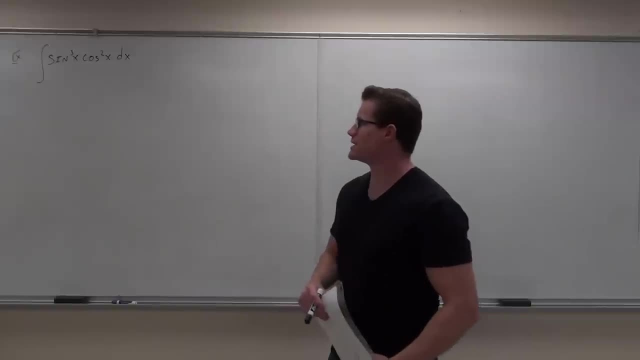 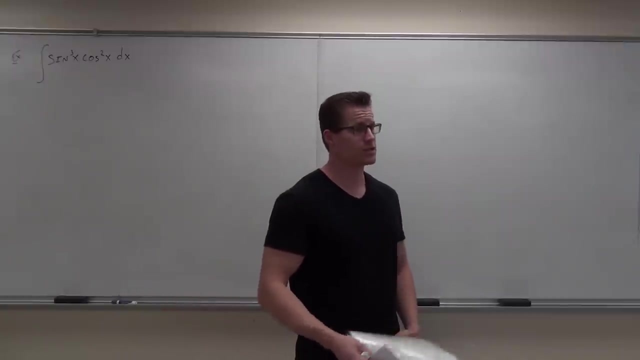 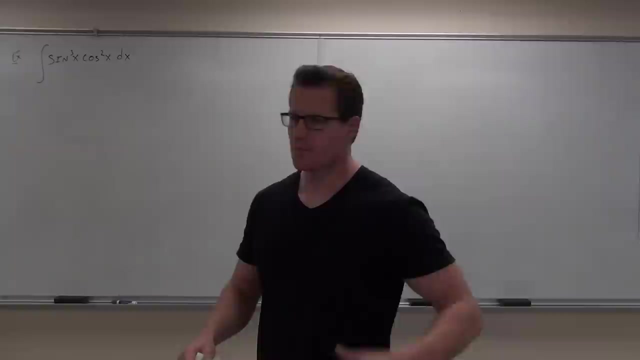 Let's look at the integral of sine, cubed x, cosine, squared x, dx. Now I gave you some cases. What I said was there's really two of them. Either you have at least one odd power or you don't. If you have case one, if you have at least one odd power, the goal is going to be split. 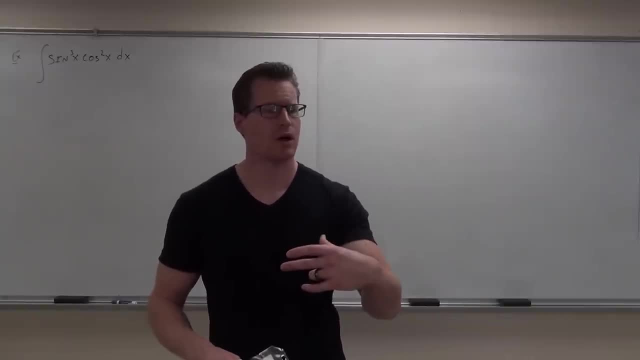 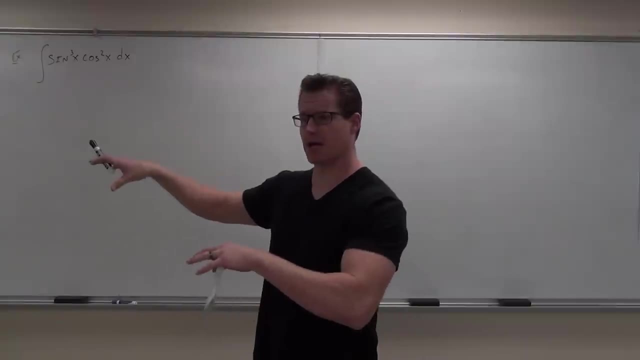 off either a sine or a cosine of that odd power And then use a Pythagorean identity. If you can use a Pythagorean identity, you change it from sines and cosines to either all sines or all cosines. Does that make sense? 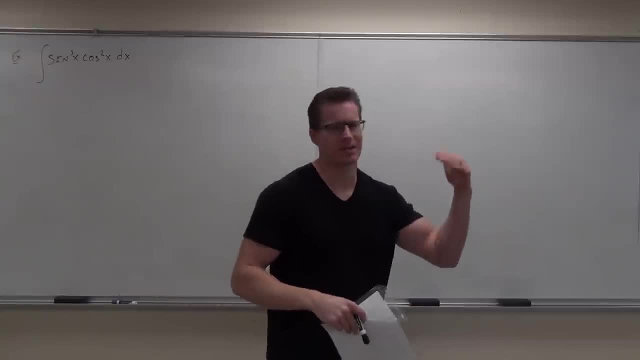 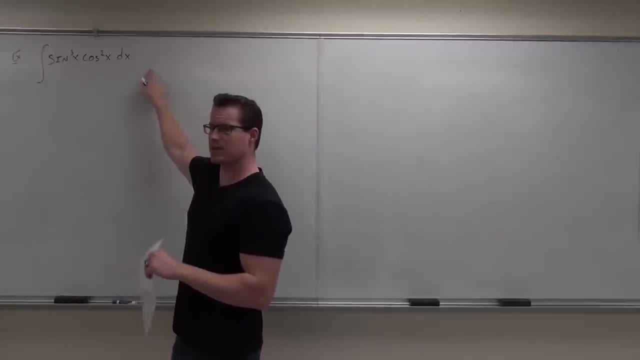 That's the idea here. So I want you to get familiar with what you're doing. Don't just follow this like a pattern. Really understand what we're trying to do. We're stripping off one of these things. firstly, so that we can make a Pythagorean identity. 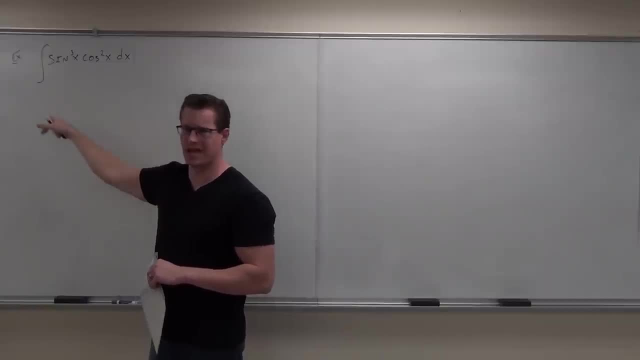 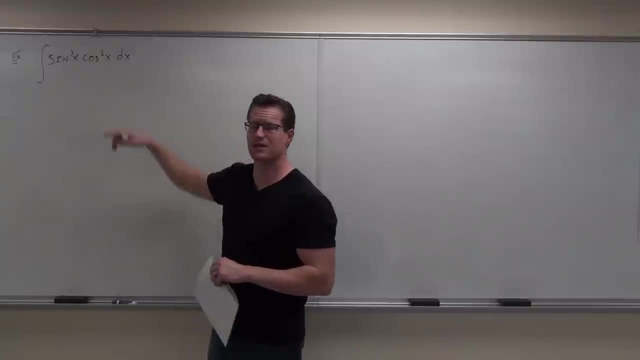 substitution and then we'll have all of one type of function, either sines or cosines, with the exception of that one thing we stripped off. The reason why we need that one thing we stripped off is because then a regular u substitution will work. really, really nice. 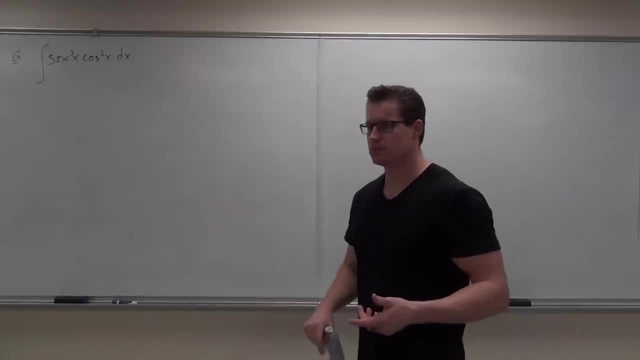 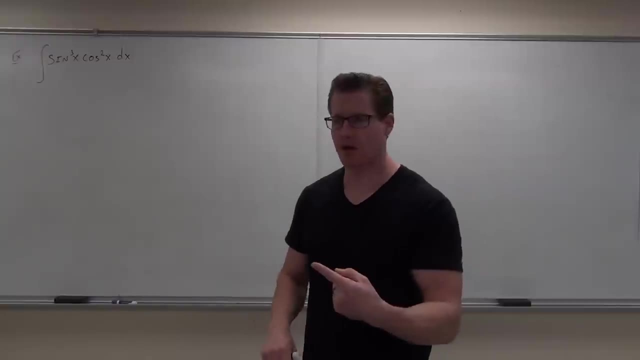 So let's look at our problem. Do we have an odd power? Are they both odd? No, Okay. so if one's odd, that kind of makes our choice easy as to what we're going to do. If there's one odd, we're going to strip off one of those factors and use the Pythagorean. 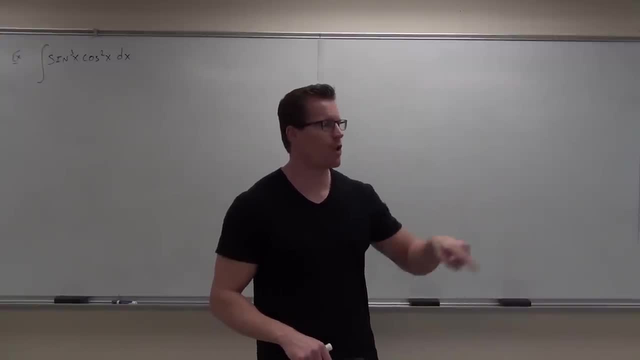 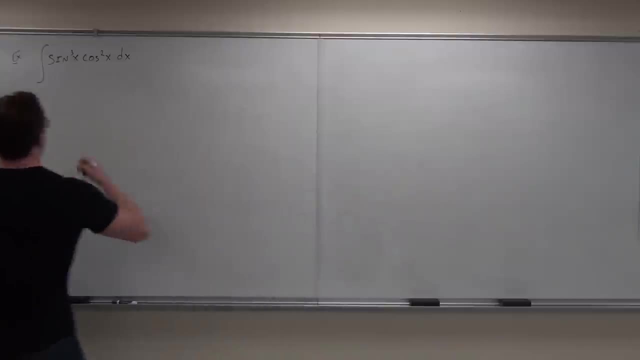 identity. If they were both odd, we typically pick the smaller power, because that will usually give us a Pythagorean identity easier. Does that make sense? Does that make sense to you? So for us, what are we going to pick for the thing that we're stripping off here sine? 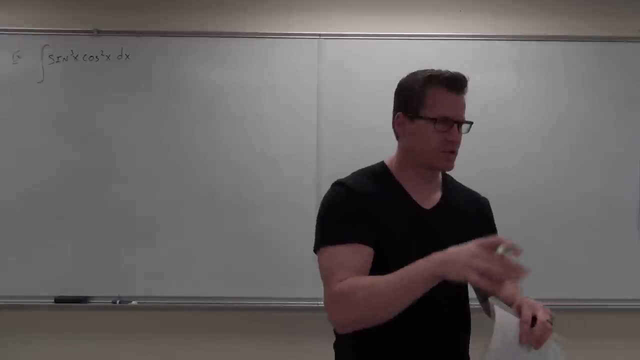 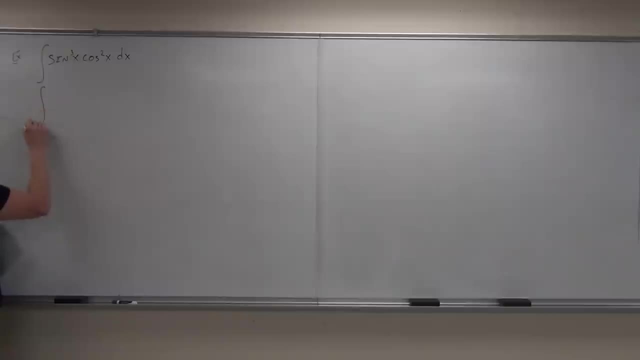 or cosine Odd. And why are we picking that? Because it's odd. It's odd, And if I strip off the sine, I'm going to get sine squared. That's the Pythagorean identity I'm looking for. So here we're going to write this, and I typically write it this way. 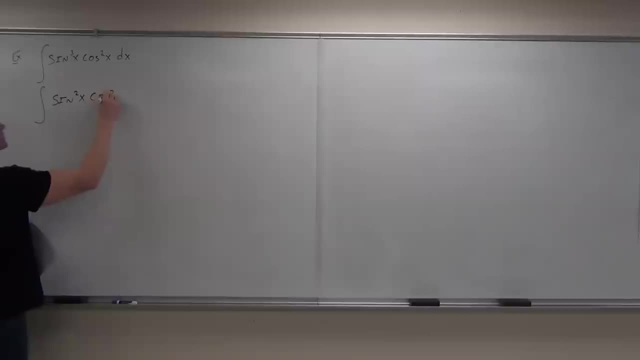 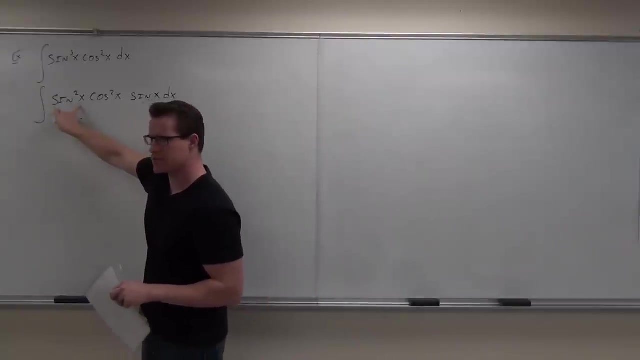 I'll write my sine squared x first, and then my cosine squared x, and then I'll put my sine x in the very back. Whenever you strip off right there, you put it in the back. The reason is because what's going to happen again? the idea here: use this to get a Pythagorean. 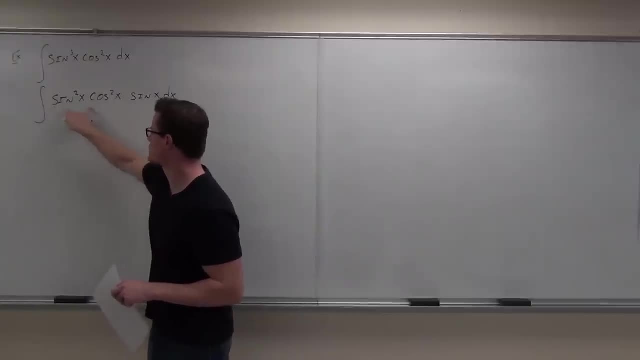 identity. That way, sines become cosines. These will all be cosines, And then I can make a substitution. Hey, what's the derivative of cosine? Sine, Sine, yeah, So that's the idea We're trying to get to that. 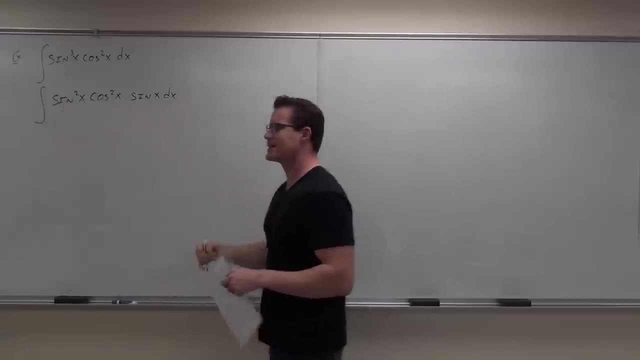 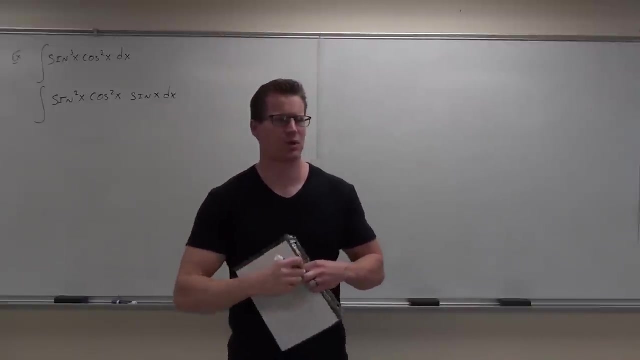 We're trying to get back to this going away. So, by the way, some people ask at this point: well, wait a minute, why don't I use the Pythagorean identity? Why don't I use the Pythagorean identity on this one, right here? 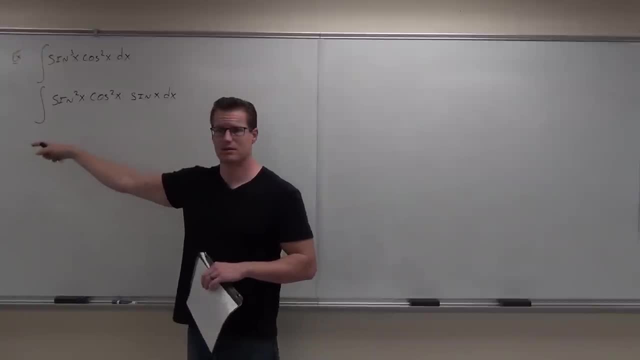 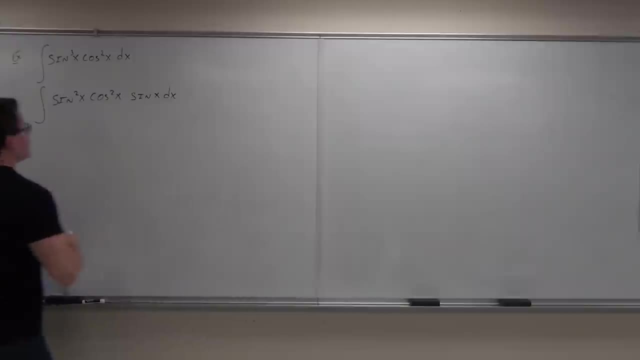 Well, if I do, then I'm going to get sine to like the fifth power somewhere, And that's not a good thing either. We want to be able to make that substitution and get rid of this. So as soon as we get our odd power, we strip off one of the factors. 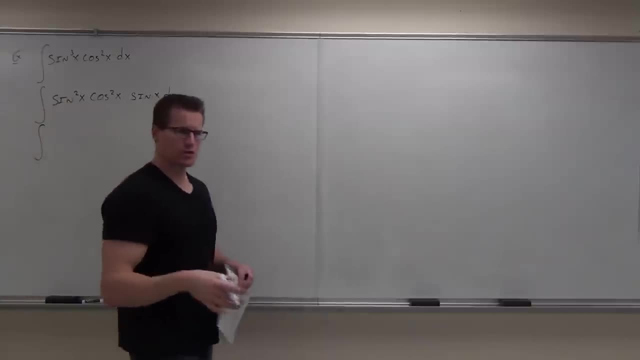 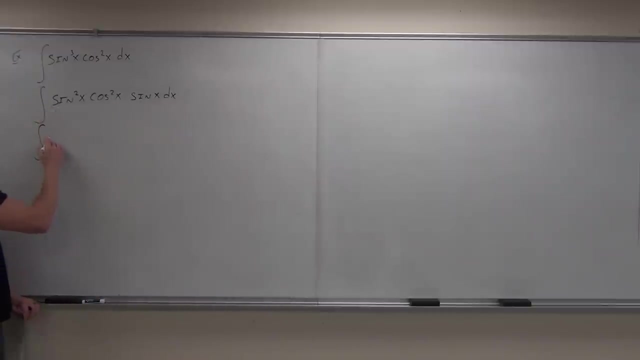 Then we go ahead and say: well, the method I gave you said: change one of those things by the Pythagorean identity. Whatever you stripped off, that's what you're left with. So this thing is going to be what is it? 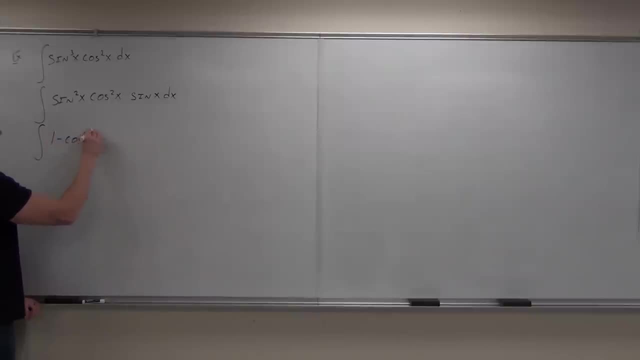 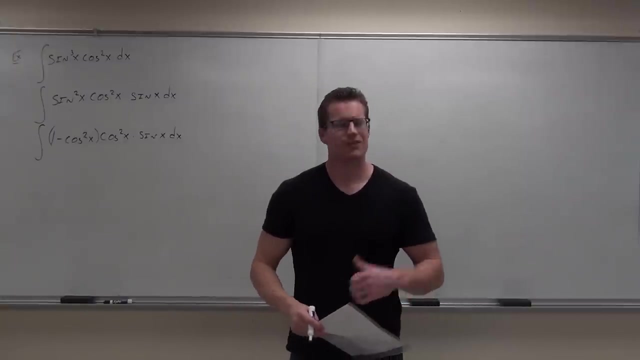 The rest of this stuff is still here. The rest of that is right there. Quick head nod if you're okay with it. so far, If you're going, why does that help us? Well, why it helps us is because right now I don't want you to distribute. 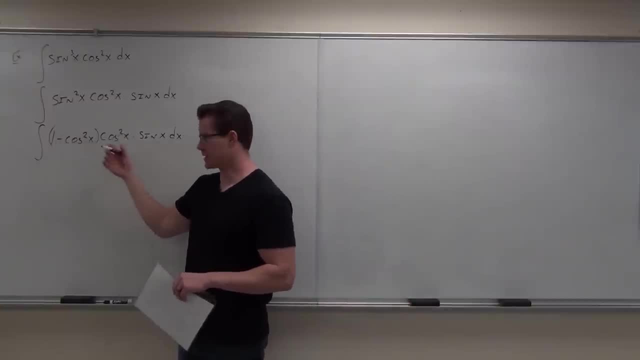 That'd be silly, okay, Because this whole thing we'd have to go here and here You'd have two inning rules instead of our one. We want to make this easy. Right here, we're going to have two inning rules. 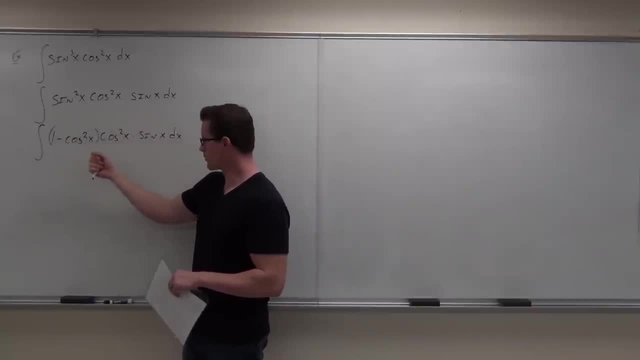 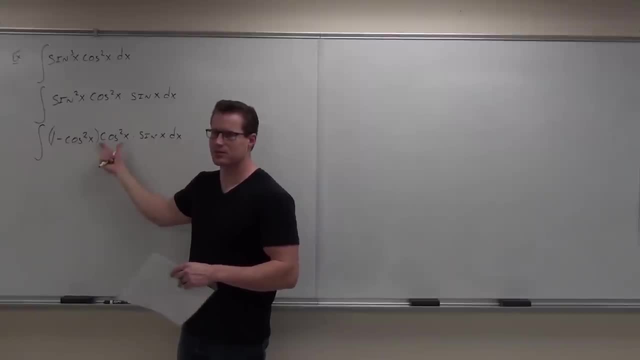 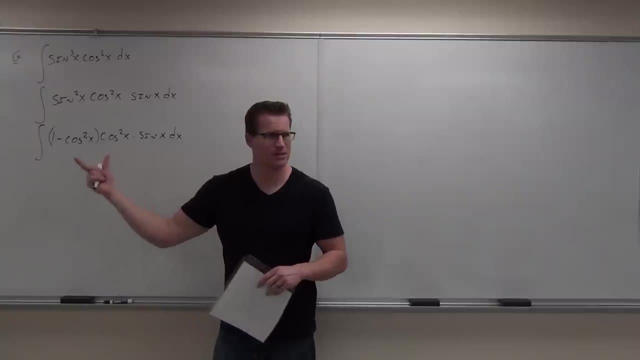 of cosine again: Sine, Sine, Negative, Close. What is it? Negative, Negative, Negative, Negative, Negative. That's going to go away. Yeah, my integral is going to change to a negative, but that thing is going to go away. 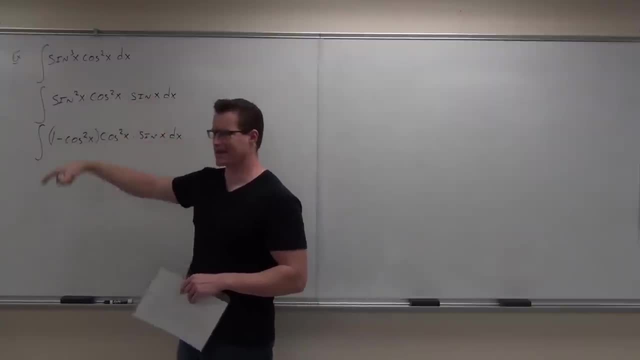 Does that make sense? This is the idea: If you have an odd power, break off one factor, Use an identity, Make a substitution. That's how it works often with this stuff. So here we go. Wow, this is really nice. 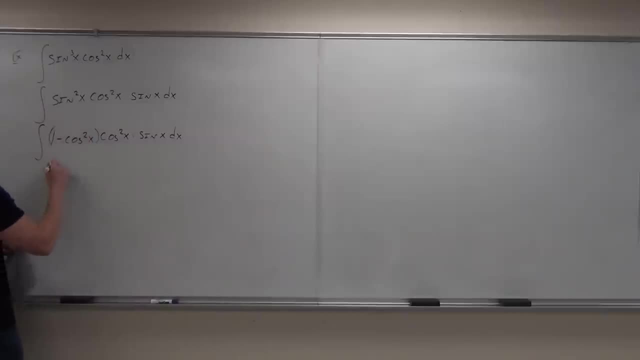 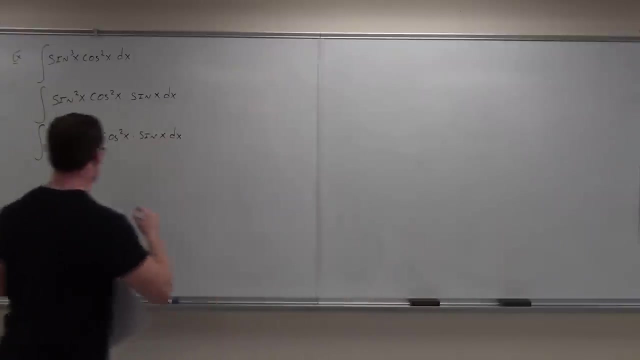 As soon as you see this to be about distributing or anything, because if we do a basic substitution for cosine, do I want cosine squared or just cosine? What do you think? Cosine, Yeah, just cosine. If I have cosine squared, I gotta do the chain rule. 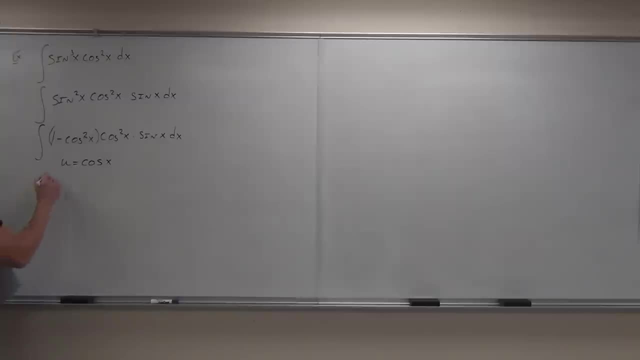 and that's really annoying because I'll have cosines and sines coming up at us and we don't want that. So du equals negative sine, x, dx. When I'm doing my substitutions on a lot of these trig integrals, I won't solve it for dx. 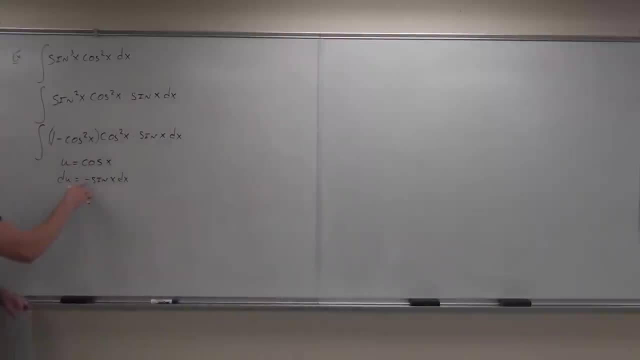 I know I showed you that sometimes- Sometimes I don't- What I typically do is just move this sine or any constants over. So, negative du would equal sine x, dx, because- and this is why we put this at the back end- Do you see how this piece matches up perfectly? 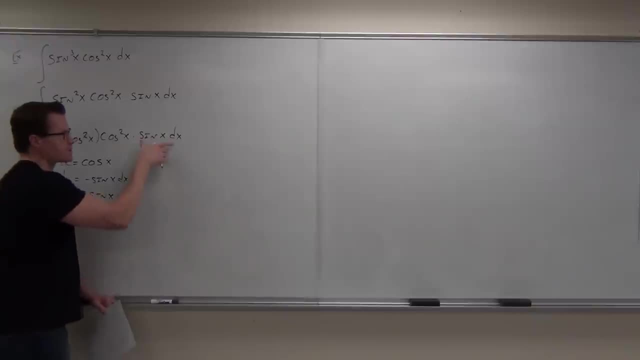 with that piece. You see what I'm talking about. That's what we want. So I move this at the back end, because this is now a really nice easy substitution Right there. Okay, so why don't you tell me what's gonna be on the inside of our integral now? 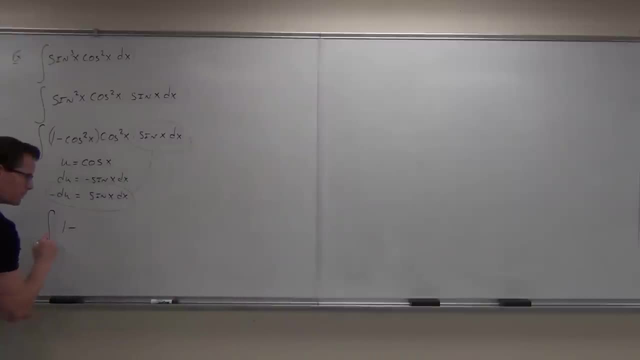 What do I get U squared? Okay, good, We got the one, Minus what now? U squared? Cool, Cosine is u So cosine squared. is u squared? Excellent, What else? Times u times sine x. Times u times what? 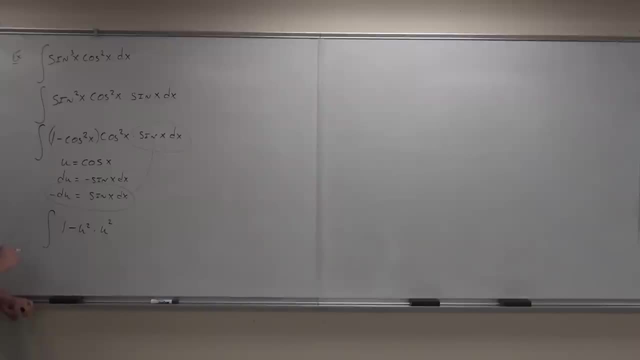 Times: u Oh du, now We got rid of the sine x- U squared. Okay, so we got one, I got minus. I got u squared. I got another u squared. There's something a lot of you love missing. 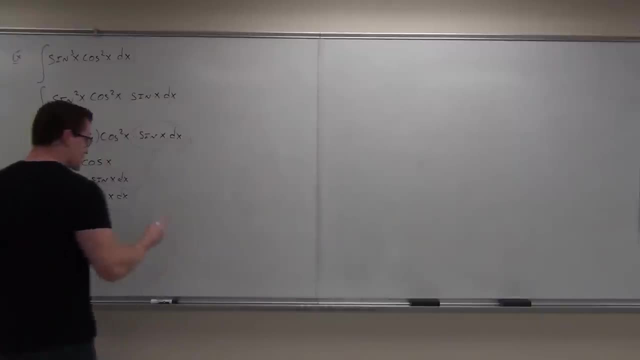 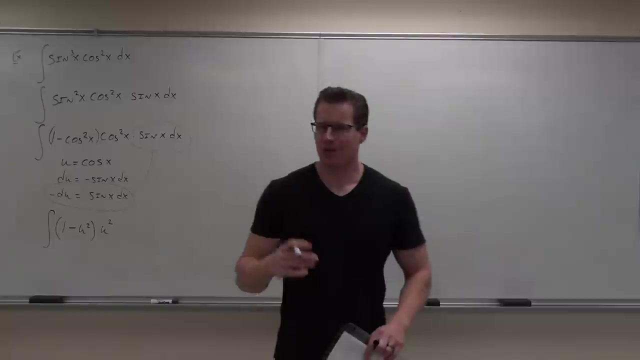 What are you missing right now? Negative du. Oh, besides that, Missing parentheses, Missing parentheses, Uh-uh, That's important. Why is that important? To distribute? To distribute. For some reason, some of you guys have the tendency to miss parentheses and still distribute. 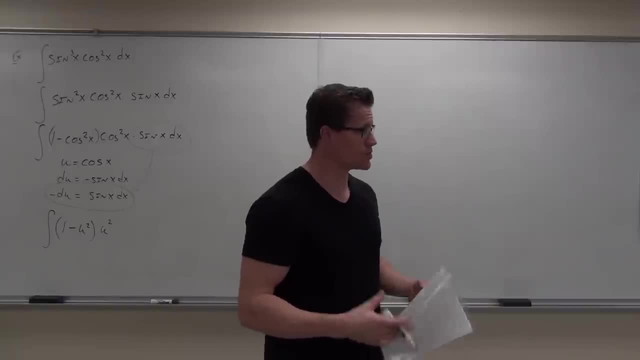 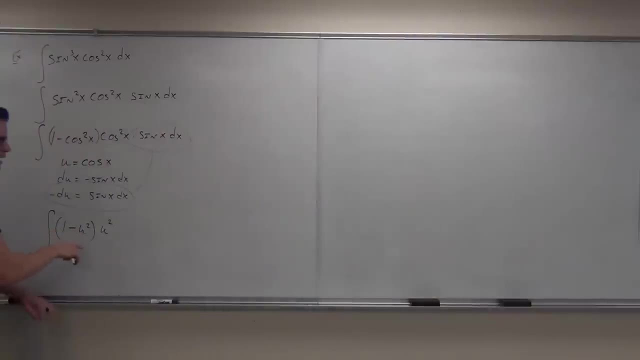 because in your head you like know they're there or something. It's really important for you to put those. You need them to say: this is what I'm doing, Otherwise this math kind of falls apart. You need to show that. So these parentheses are not trivial. 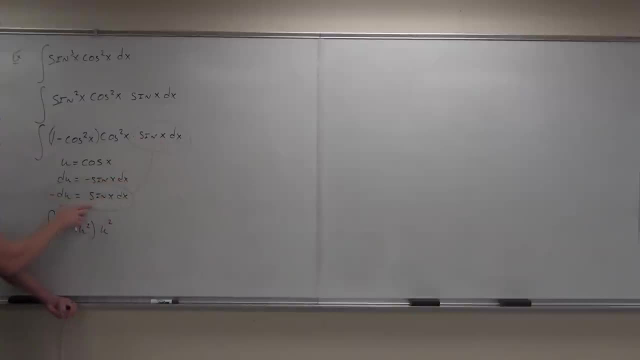 And then now sine x, dx is the same thing as what Negative u. Okay, we don't want to forget the negative du. Negative du, Negative du, So times negative du. What are we going to do with this thing right now? 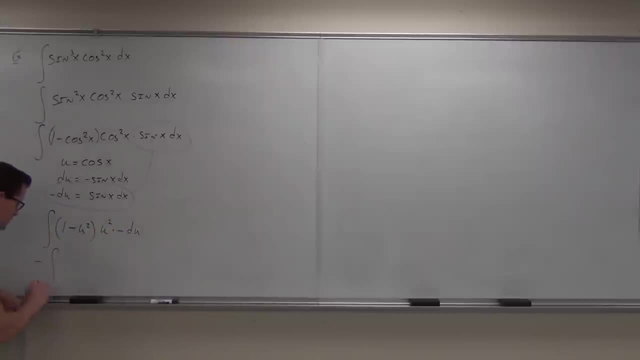 What do you think? Pull the negative out. Pull the negative out, Okay, so negative integral. What else are we going to do? Distribute, Distribute. That will be u squared minus u to the fourth. Don't forget the du. 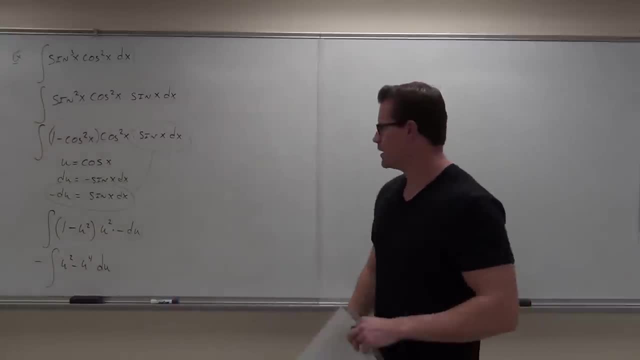 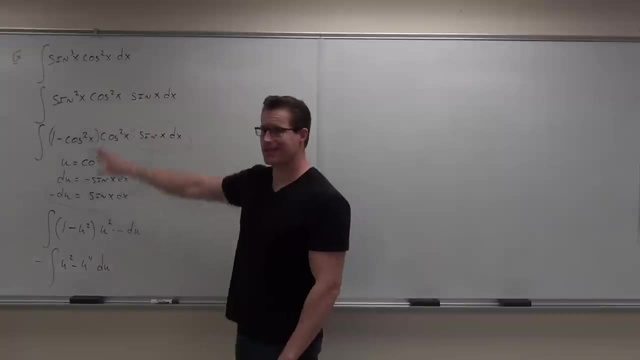 Don't get sloppy with this integration. You've got to show all this stuff. None of it is trivial, You guys? okay with this so far? Yeah, We just changed a really nasty integral. We go, man, how am I going to do that? 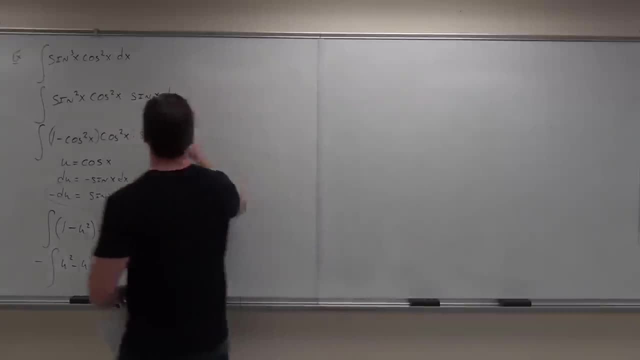 Something really, really easy. This is brilliant. This is nice. We'll have negative. What's the integral of u squared u, thirds over three, Minus what? u to the fifth over five? Would it be positive? Well, you tell me. 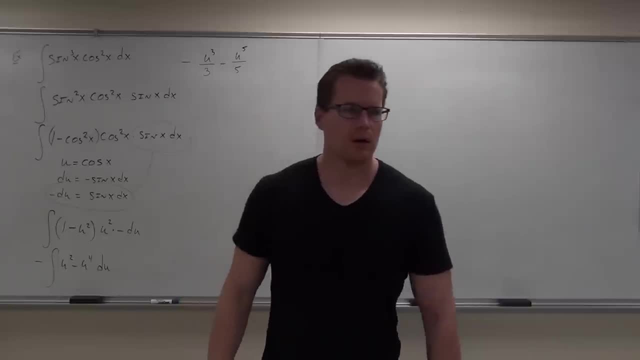 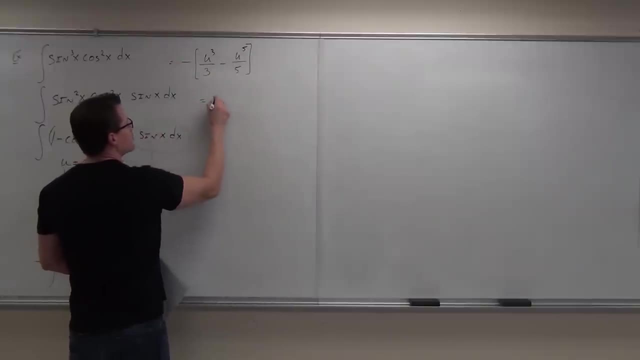 What am I having wrong here? Negative, Negative. Okay, so if I don't have my brackets, then this is wrong. If I do have my brackets, then we have negative. u cubed over three plus u to the fifth over five. 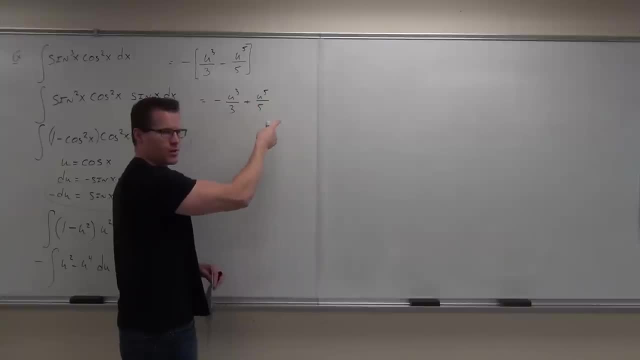 Naturally you can do that. You could write this in the reverse order. It might be a little bit nicer to do: u to the fifth over five minus. u cubed over three. Now we don't want to stop there. What's the next thing we've got to do? 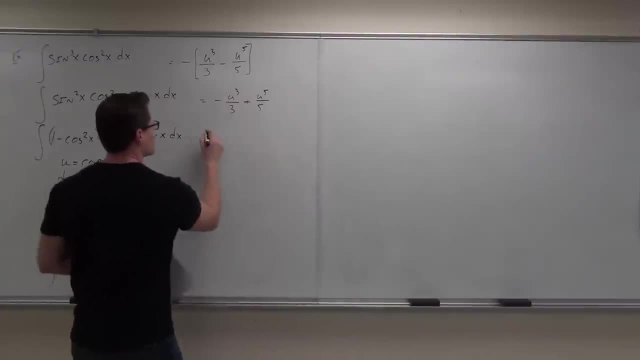 Plug your u back in there. That's very good. So, whatever our u is, we'll have – and I'm going to reverse this right now. So I'll have cosine to the fifth power of x over five, minus cosine to the third power of x over three and – 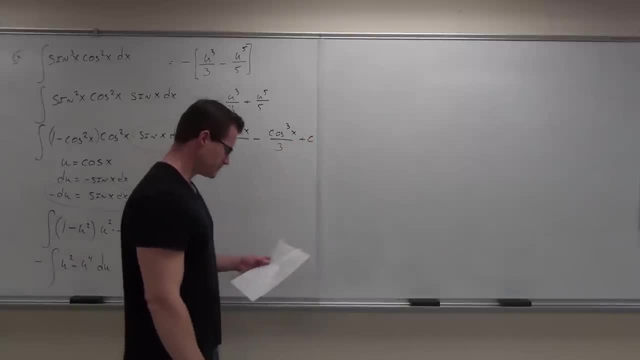 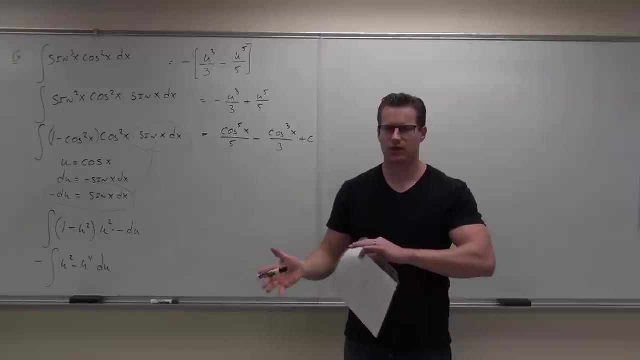 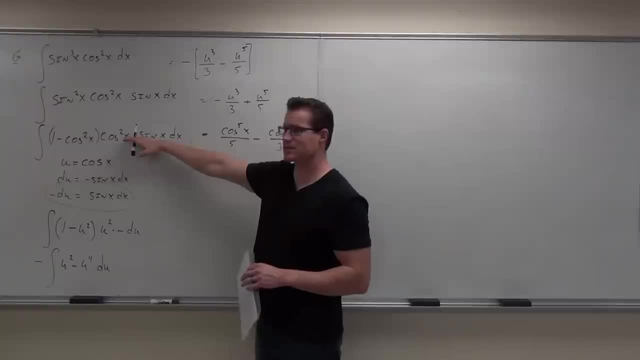 easy, medium hard, What do you think? Kind of medium right. This part – as soon as you see this – this is easy, This should be easy. at least This part is the part that people struggle with. How do I do it? 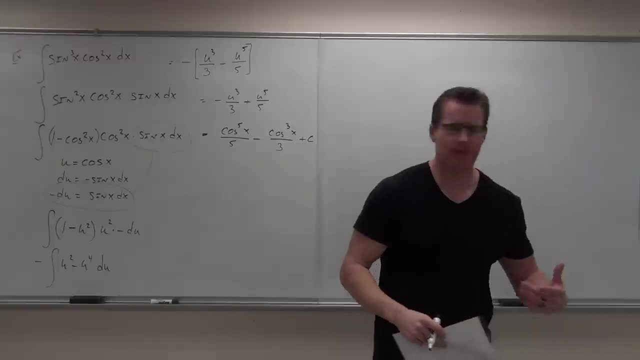 You got to get used to seeing these things following the pattern. You know what I mean. That way you go okay. hey, look at this odd power. That's an even power. I'm going to strip off one of those things. 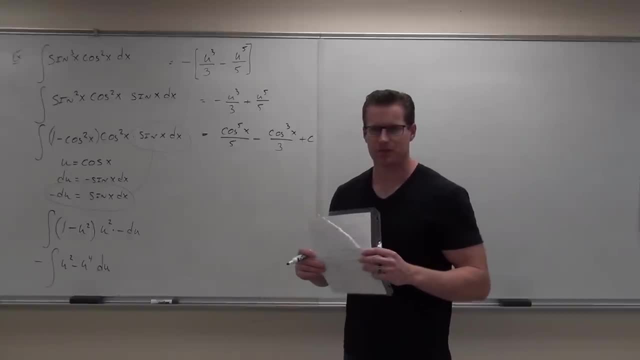 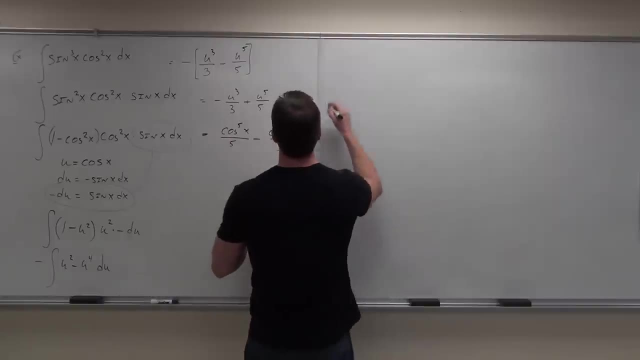 That's the idea here. Shall we do another one. Yes, So far I think I've given you two odds and I've given you one odd. Let's see how it works with this example. You know what I'm gonna need some more room. 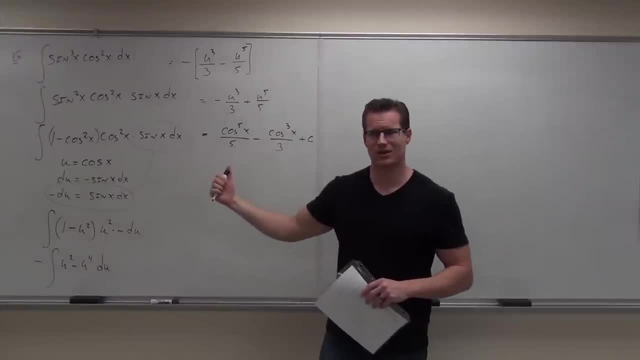 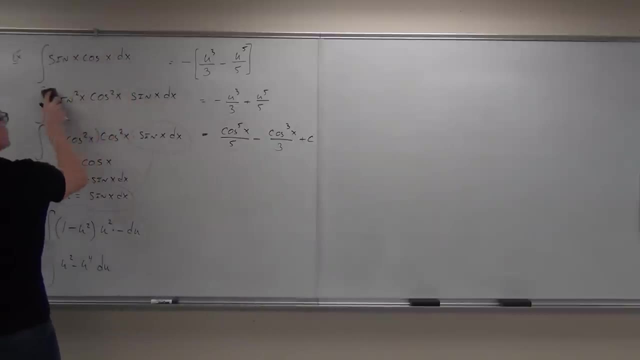 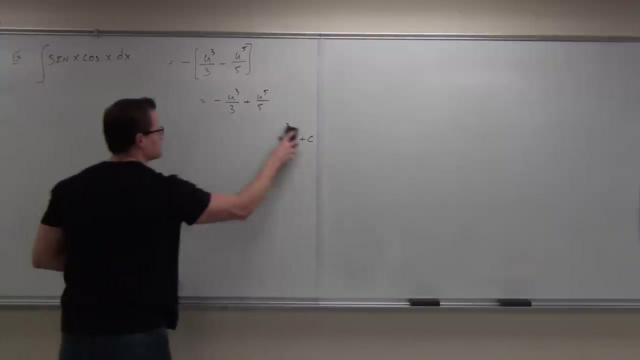 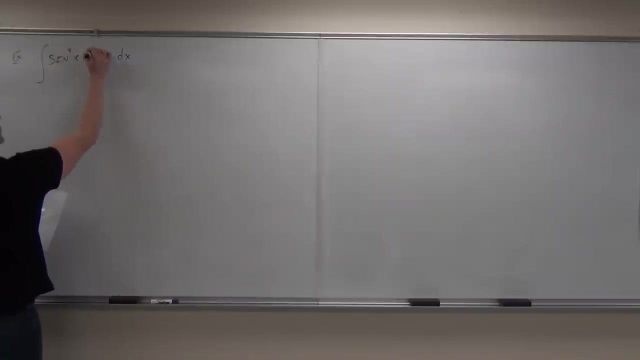 Do you have any questions on this? Because I'm gonna erase it. Some of these things take a while, Okay, so now we're gonna do sine to the fourth, cosine to the fourth. So as soon as you see this problem on a test. 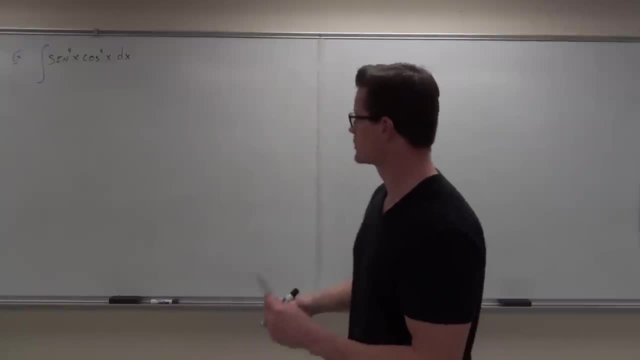 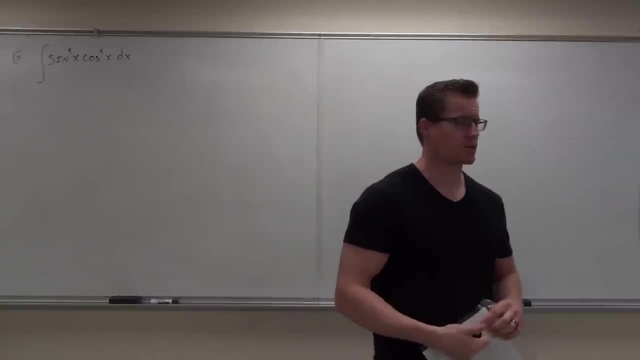 yes, you're gonna have something like this on a test. As soon as you see this on a test, you go all right, cool. How in the world are we gonna do that? Well, go through the pattern. Do we have at least one odd power? 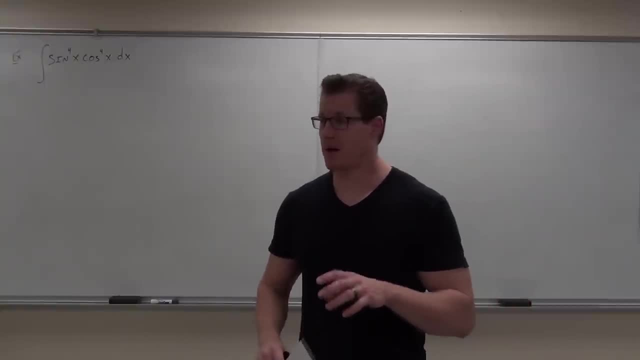 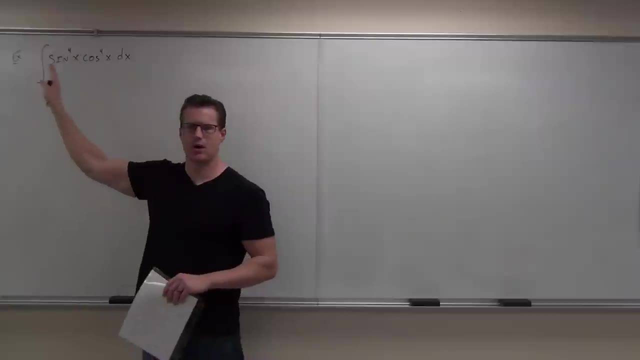 Okay, so they're both. even If they're both, even the idea of Pythagorean identity goes out of your head. Because if I do this, if I strip off either a sine or a cosine, I'm left with an odd power. 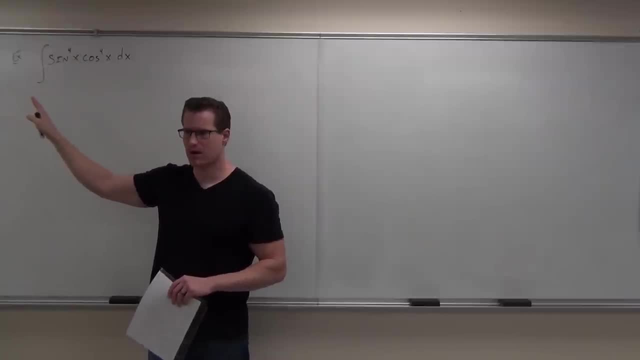 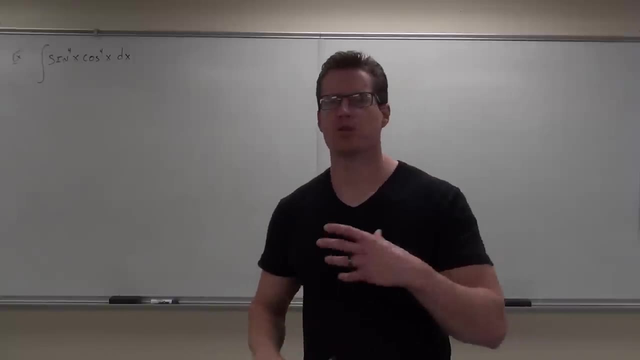 Does that make sense? Yeah, The Pythagorean identity's not gonna work with an odd power. Your substitution won't work because you'll have an extra sine or an extra cosine somewhere. That's not a good idea. So if you have both evens, the idea is you're gonna 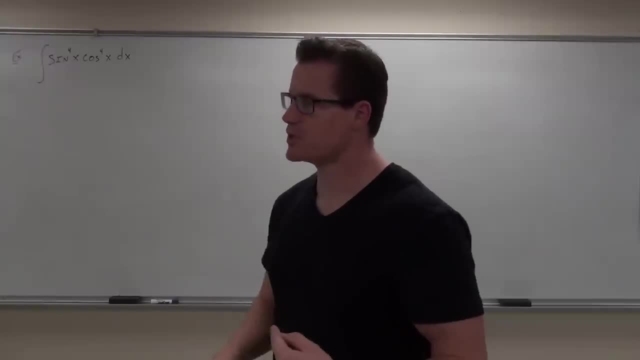 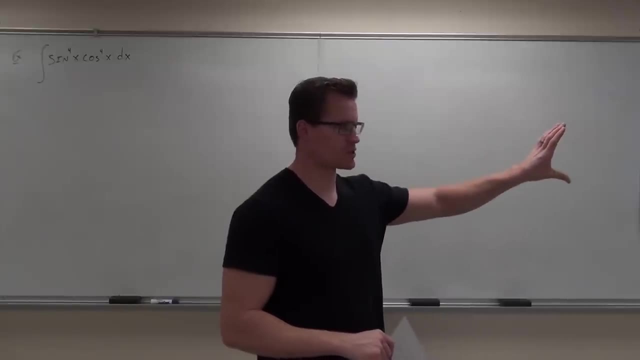 manipulate this thing a lot. It's gonna be a lot of work, But what we're gonna be using here is the half angle formulas, where we have: sine squared equals one half one minus cosine two, x and cosine squared equals one half one plus cosine two. 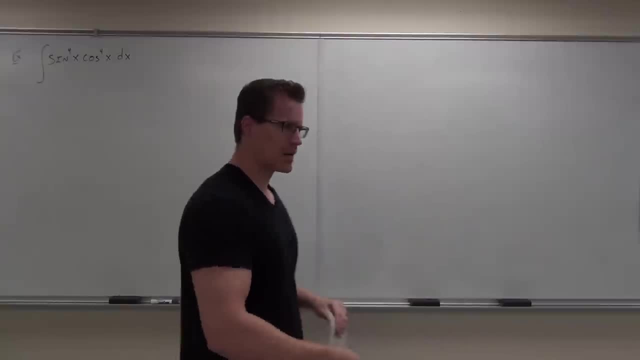 Very good. So we're gonna be getting down to those things here in just a minute, So let's work on how we might go about doing this And there's a few ways to do it, okay. So here's what I'd do. 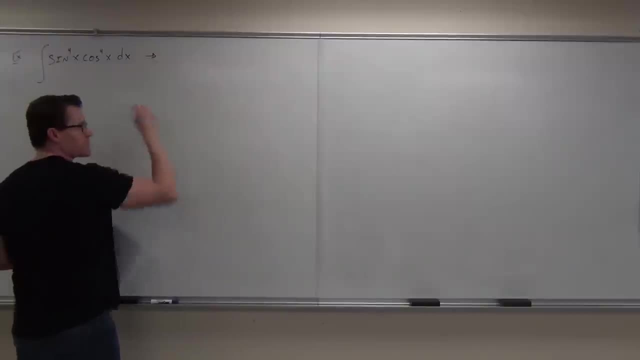 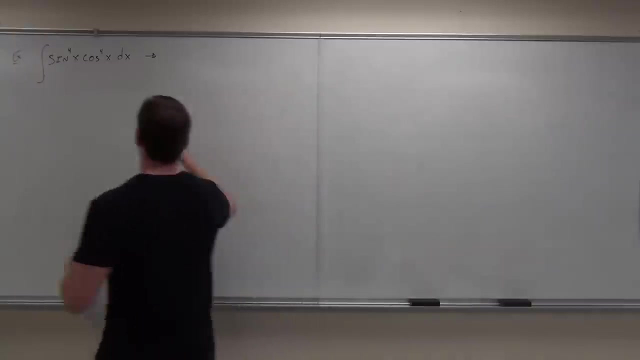 If I'm working on this problem, the first thing I'm doing is I'm gonna try to make this either all sine or all cosine. If I have the same power like four, four, we can typically do this. Check this out. 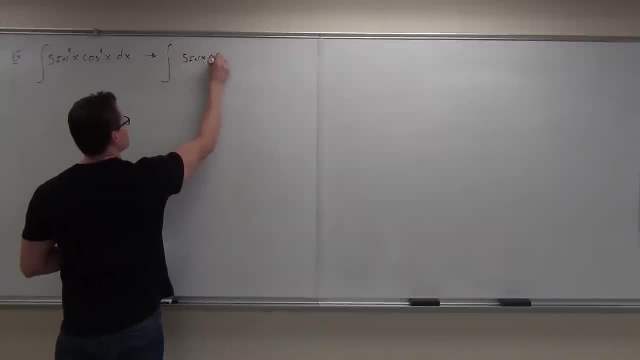 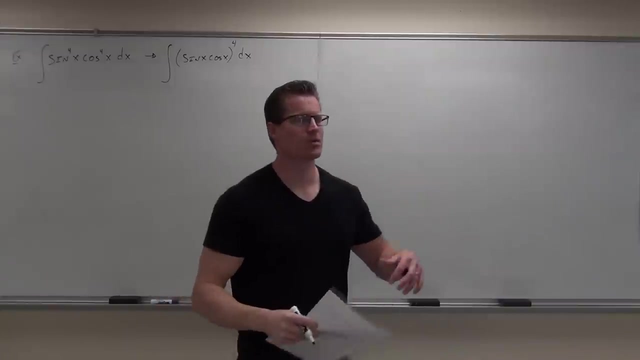 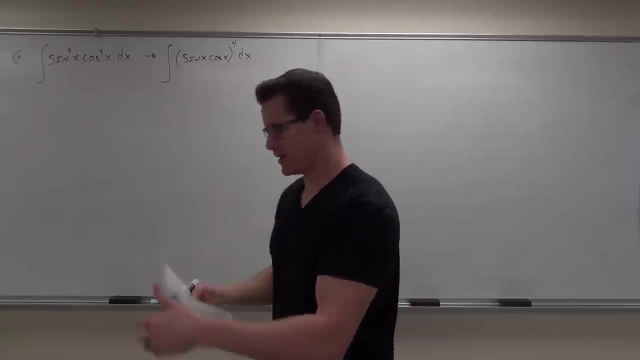 Well, I could make sine x, cosine x, x. All to the fourth. Is that true? Yeah, Sure, I could do that. My idea right now is to combine my sines and cosines with some sort of an identity. Right now, if you don't know it, I can actually do that. 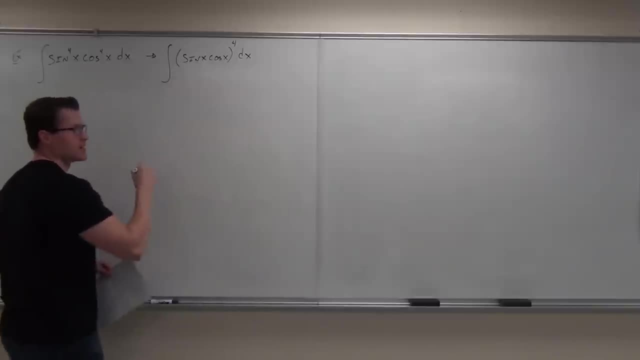 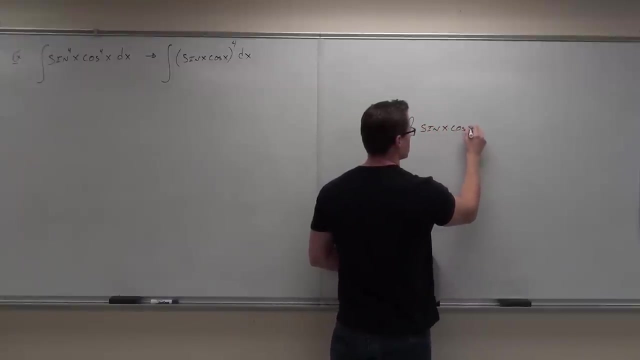 So if I'm looking at sine x, cosine x, I'm gonna use this identity over here. Do you know this one? Do you guys know that one? Is that a sine? Yeah, That's a sine, That's a sine, That's a sine. 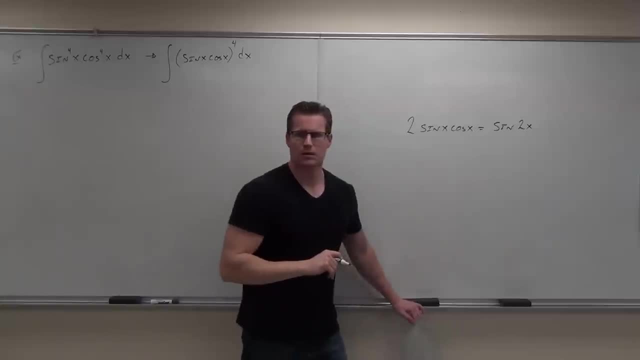 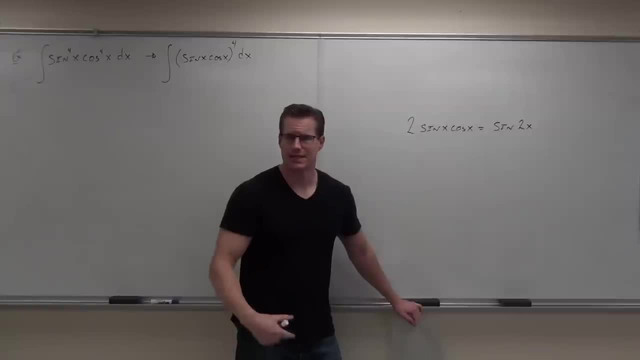 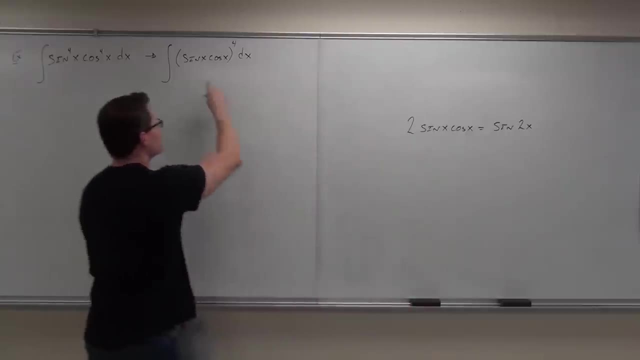 Okay, Well, check it out. We can manipulate identities all the time. If we know they're true, we can manipulate them. So, if I take this, this thing looks a whole lot like this piece, don't it? Yeah, Well, I'm gonna make this be exactly like this. 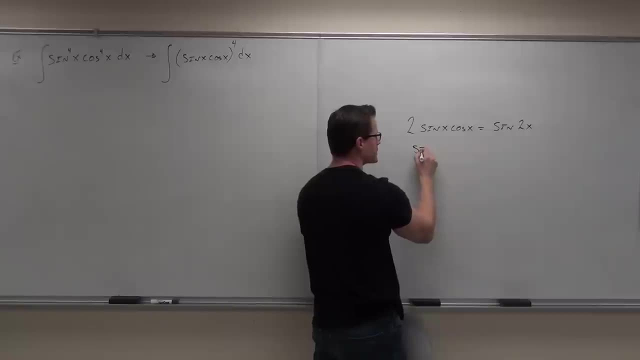 I'm basically just gonna divide by two. Then sine x, cosine x equals one half sine x. Yeah, One half sine two x. Oh, look at that, We okay with that. Yeah, Show of hands if you feel. okay with that one. 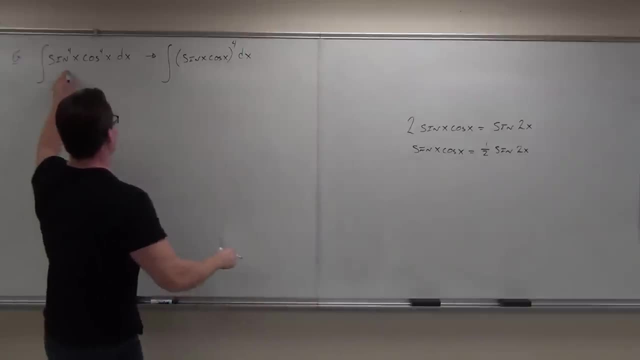 Well, what that means is: hey, look at that, I can make it sine x, cosine x to the fourth. Of course, this is a special case, okay, Where they're both exactly the same power. If they're not exactly the same power, then naturally this won't work. 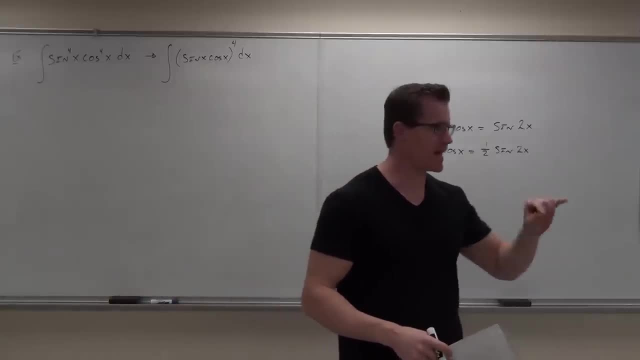 But I want you to see this at least once, Where they're both the same power. You got me, Yeah, So we can do this. Okay, Then this piece is one half sine two x, So our integral is integral of one half sine two x. 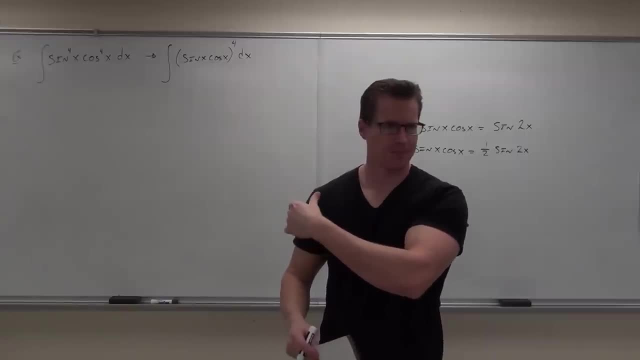 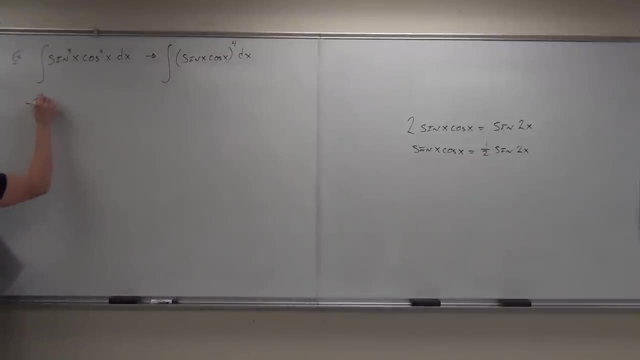 Okay, So this piece is one half sine two x, So our integral is integral of one half sine two x. Okay, So we can do this. Okay, Then this piece is one half sine two x, So our integral is integral of one half sine two x. all to the fourth power, z x. 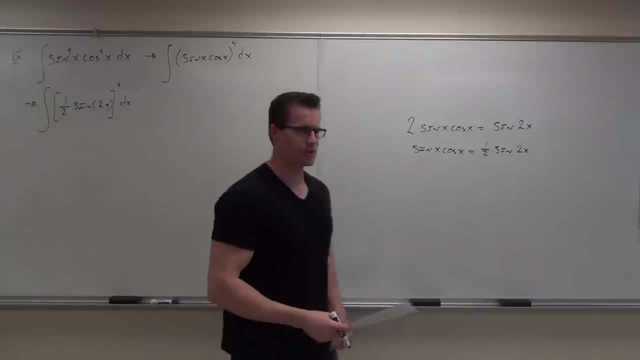 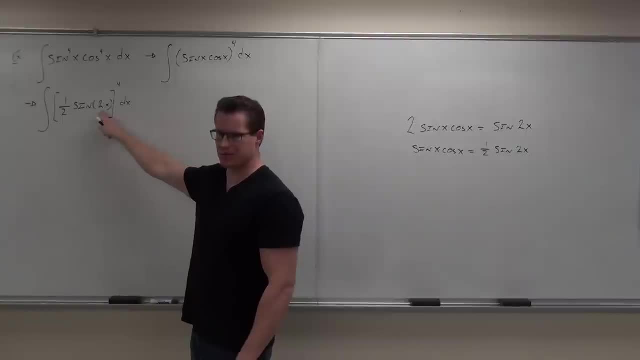 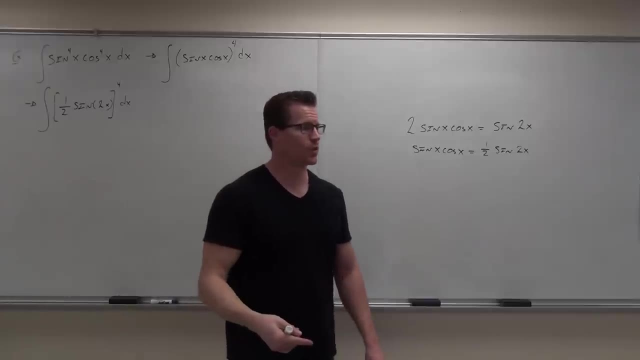 I don't want to do it. I don't care really about this. u substitution. I really don't, Because it'd be very trivial. U equals two x. You'd have a one half. Sure, Don't worry about that. We can do that basically in our head. 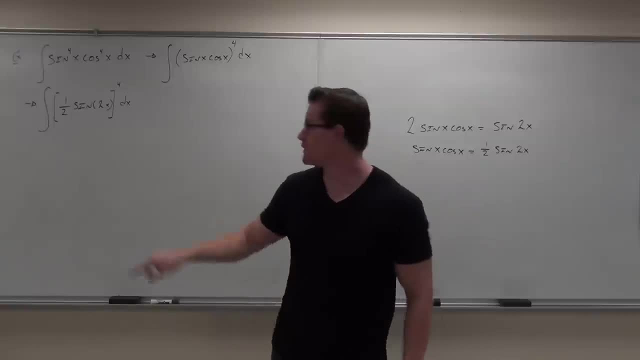 What I'm worried about, and we're going to be changing things. So if you do this, if you do a u substitution on this now, you're going to have to do it later again too. So don't worry about it until the very, very end, when you're actually evaluating integrals. 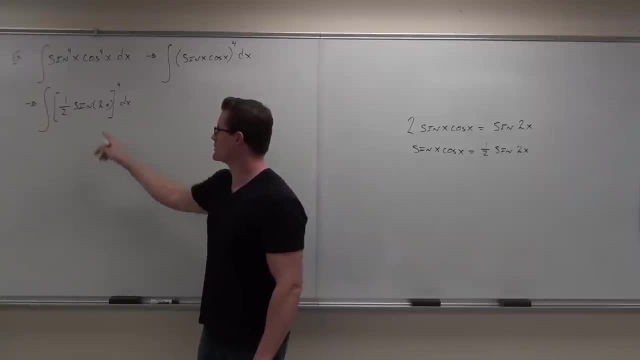 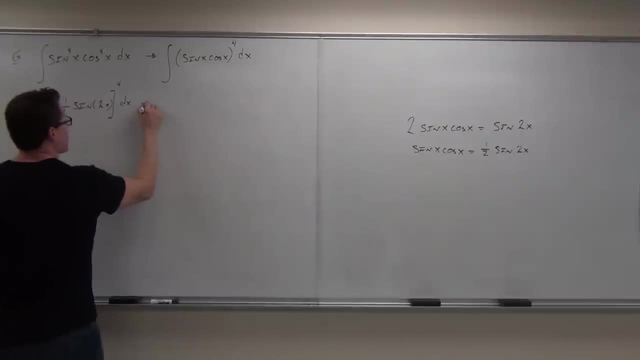 Does that make sense? Don't worry about it right now. What I do want to get rid of is: this looks kind of nasty to me. Can I take this to the fourth power and this to the fourth power? Yeah, OK, Let's do that. 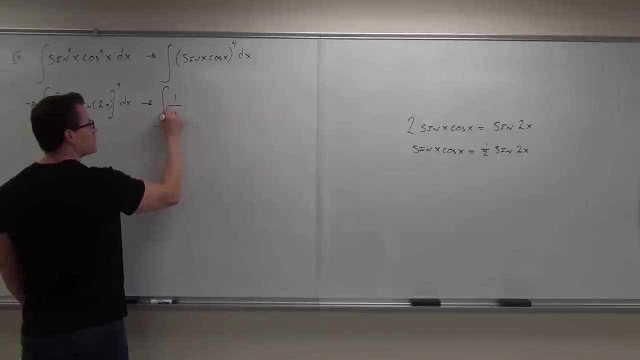 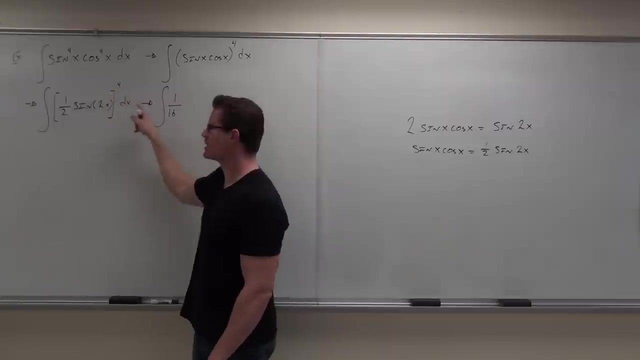 So I'm going to have the integral of what is one half to the fourth power One, 16.. You know what people do when they're just learning this or when they're going too fast on a test or their homework is: they'll forget about this guy and they'll give me. 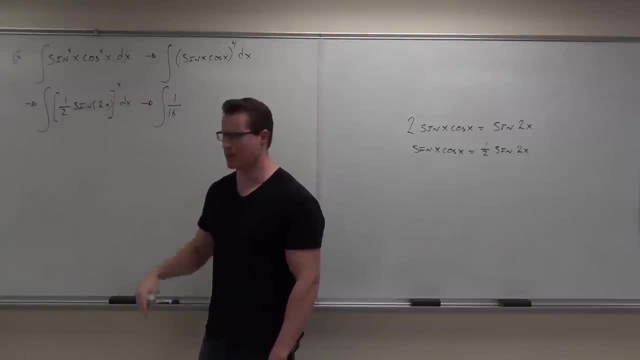 one half again. Do you see how common that might be? When I'm grading papers, I see that a lot. Where are they getting one 16th from? I'm getting one half all the time. My goodness, Well, you might not be taking that to the correct power. 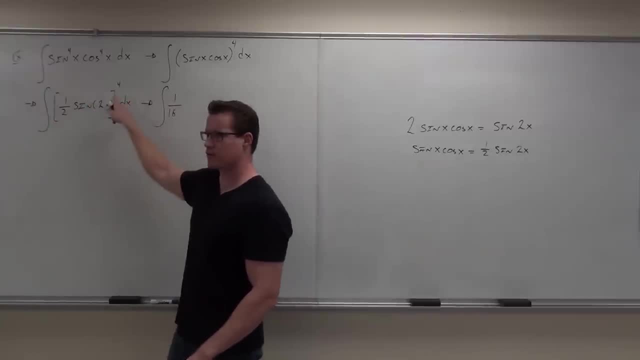 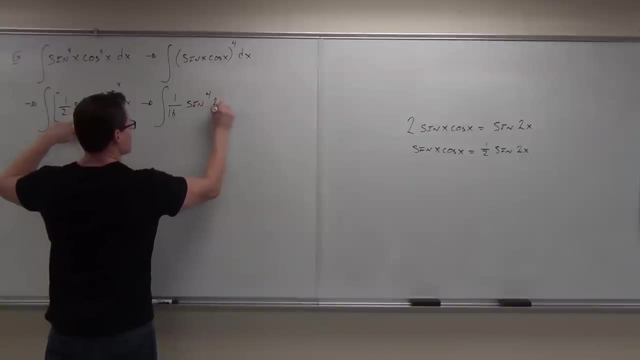 So be careful with this stuff. This whole thing is being raised to the fourth. not even if you understand that concept. OK, Then I've got sine to the fourth. power of 2x dx Looks a little bit nicer. What's the next thing I'm going to do? 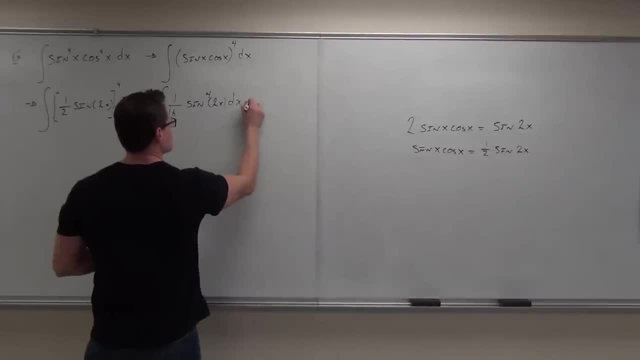 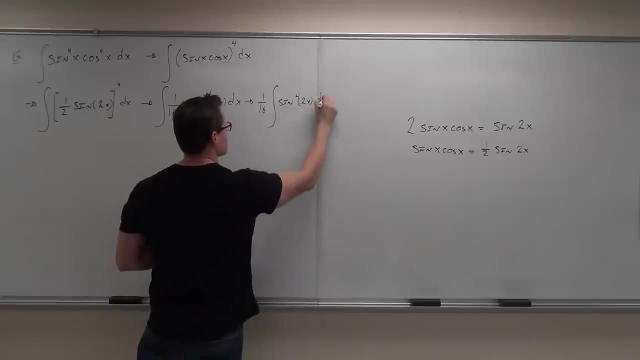 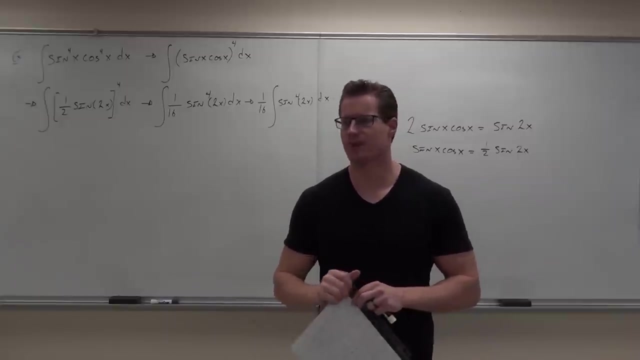 Move on to that concept One, 16th, integral sine to the fourth, 2x, dx. Now stop for a second. If you were so inclined, thinking about what I taught you back in the last section, what could you use Here? 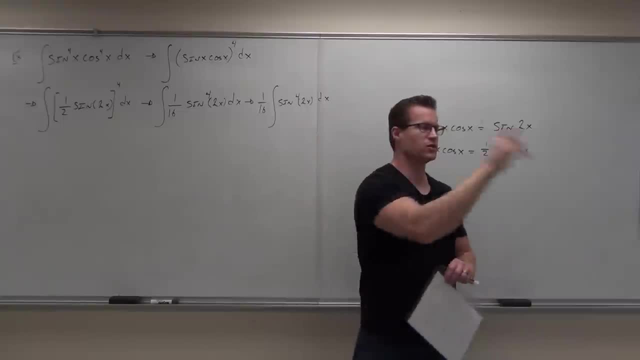 Reduction formula. You could use the reduction formula. It would absolutely work right now. Do you guys see why? Oh yeah, Well, there's no why I know, But there's a sine. Look at the sine. It's to the fourth power. 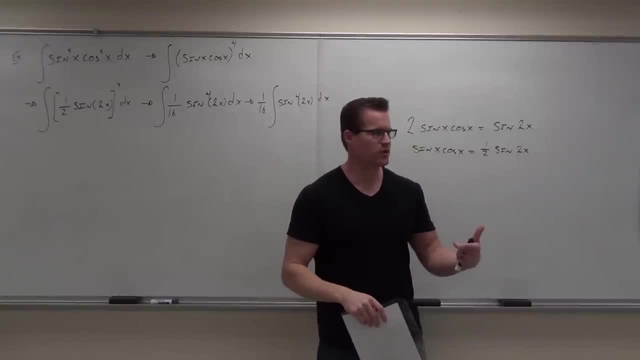 That power is greater than 2.. Greater than or equal to 2.. You could use reduction formula right now. In fact, we did sine to the fourth in class, just like two days ago. Remember? Well, two days ago you took a test. 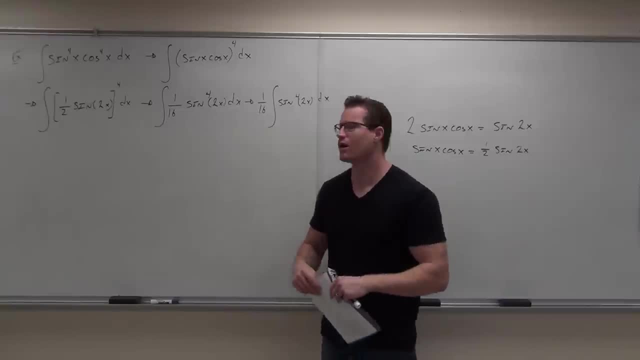 But three days ago- Remember doing that. It was the last thing we did. You could do it right now. You could just make a substitution. This is where you do it. You do it. U equals 2x. Do you ever do? 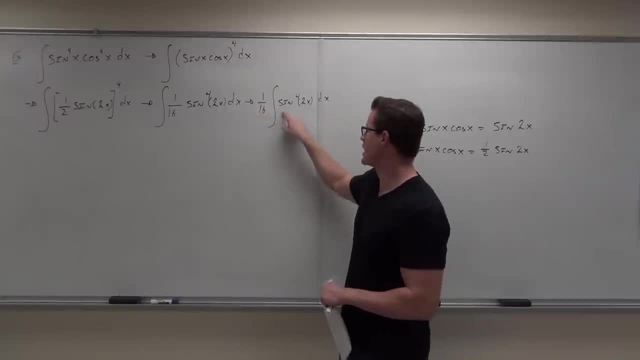 This would be 1 over 32.. You got me, Then you got sine to the fourth of udu And you do reduction formula, like I think it's two times. You do reduction formula twice And you'd be done with this thing. 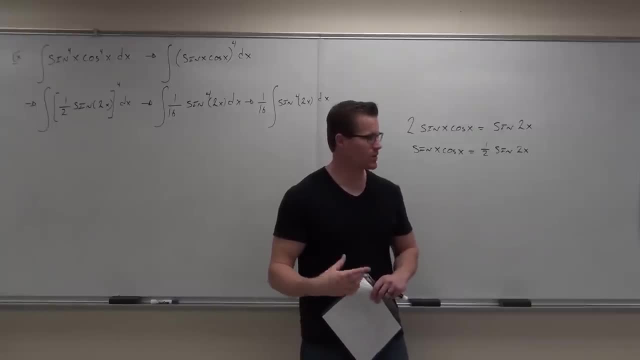 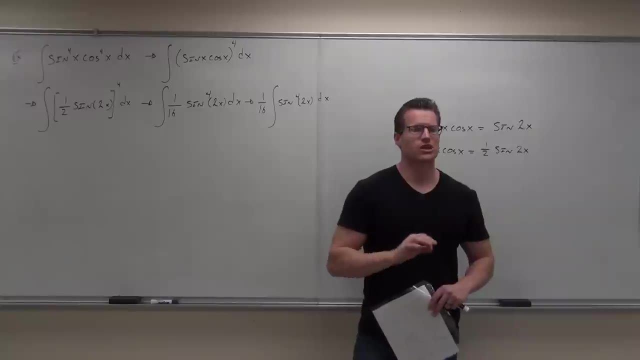 Do you guys get what I'm talking about? Look back in your notes or watch the video from the last section if you don't remember how to do reduction formula. Now what if you don't see reduction formula? Is there another way to do it? 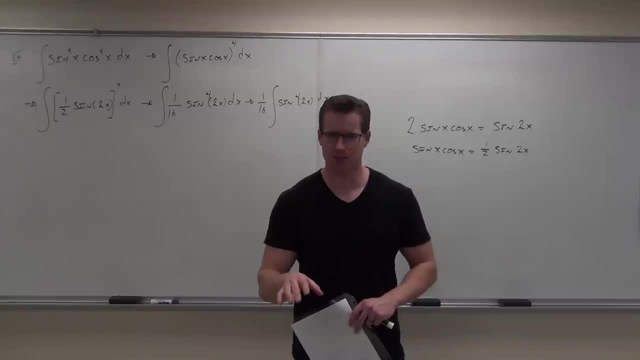 The answer is yeah, Which is really interesting, because what's going to happen is what happens, Because what's going to happen here is we're going to get our integral evaluated and it's going to look different than if we had done this with reduction formula. 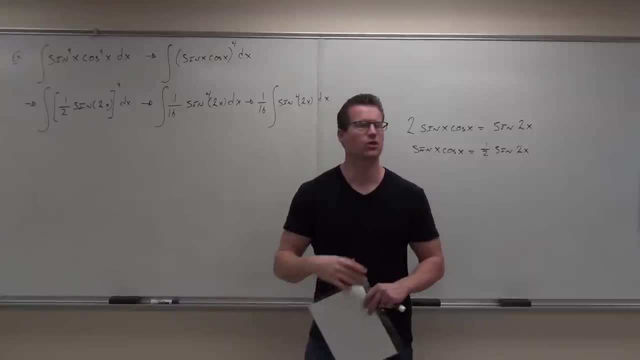 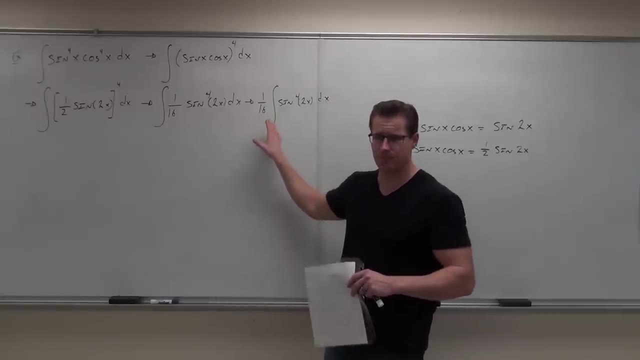 Reduction formula will work. It will be equivalent, but it's going to look different. Does that make sense? Now, I don't care how you do it. If you see this, I've already taught you reduction formula right, You can do it. 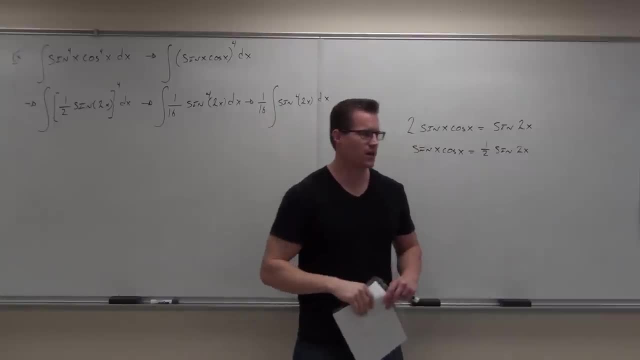 That's fine Anytime. If it's sine to some power, go for it. Some of us have. a few of you have proved the reduction formula for cosine. Go ahead and use it. Your answers are going to look a little bit different than if you do it this next textbook. 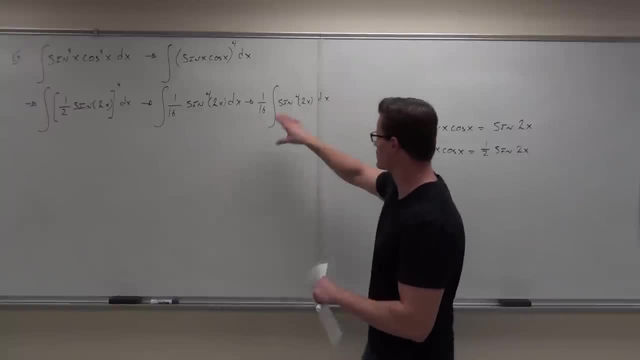 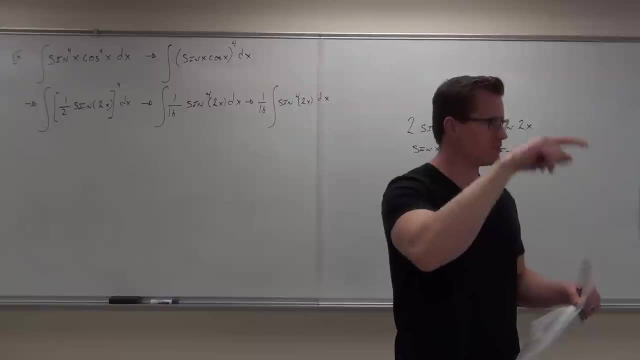 So technique one, You work it all down, You go: hey, I see reduction formula, I can do that. It's sine to a power greater than or equal to two. No big deal. Remember that one It's the one over n's and you have sines and cosines and a minus and n over n minus. 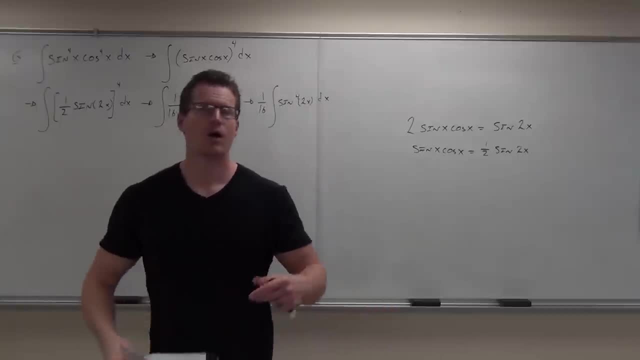 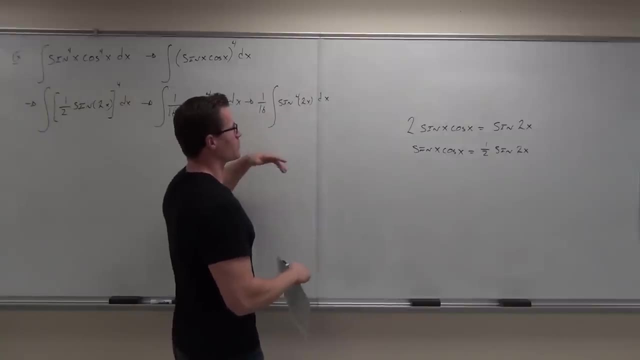 n minus one over n integral and it reduces it for you. Well, let's say you don't see it. Is there a different way? And the answer is yeah. If there's not a reduction formula possible or you don't see it, we can still do this. 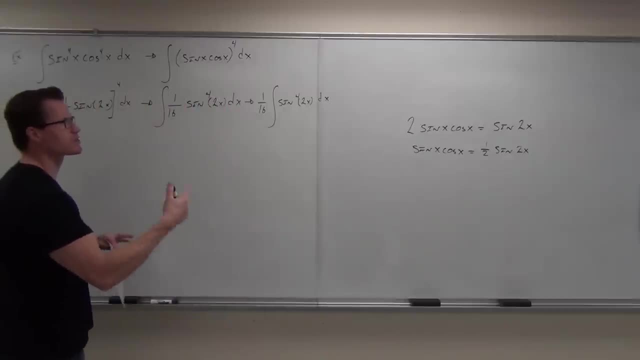 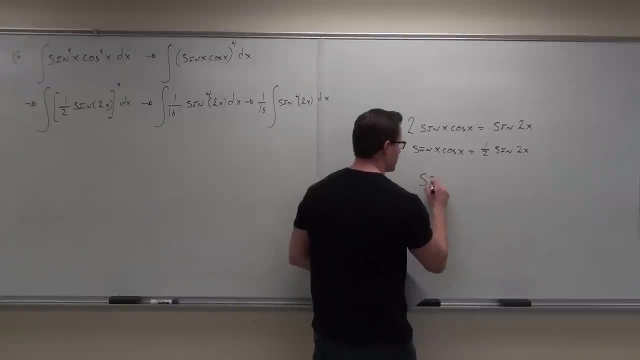 with those half angle formulas, And here's how you'd work it. Instead of thinking of this as sine to the fourth power, what we need to do is we need to find something that will allow us to make this substitution. We need this basically. 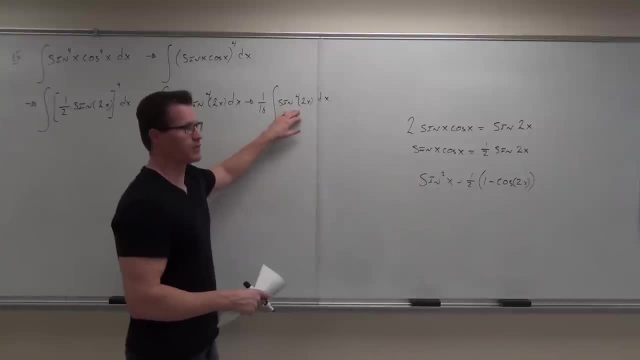 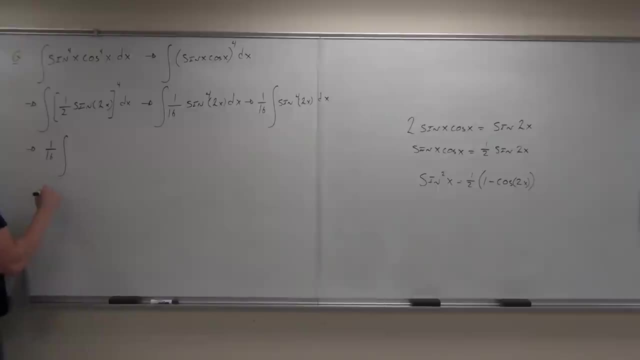 So when we get down to here we go, man, how do I do it? Reduction formula. If you don't see reduction formula, you're going to have to rewrite this again. So how we're going to rewrite it is one-sixteenth integral. 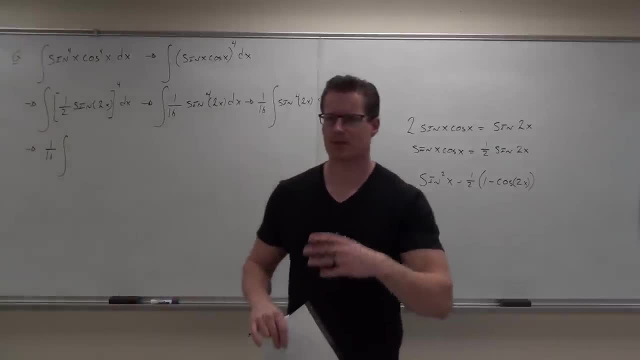 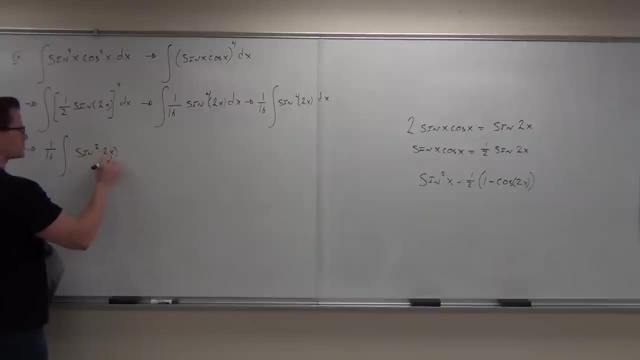 Let me rewrite sine to the fourth power. How am I going to write it? as something like sine squared. What do I do? Sine squared two x times sine squared two x. I'm going to change what you said just a little bit. 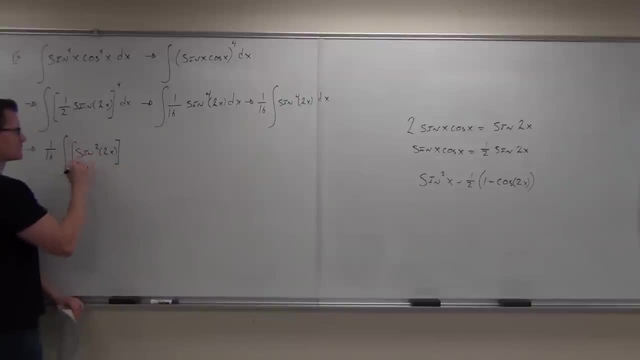 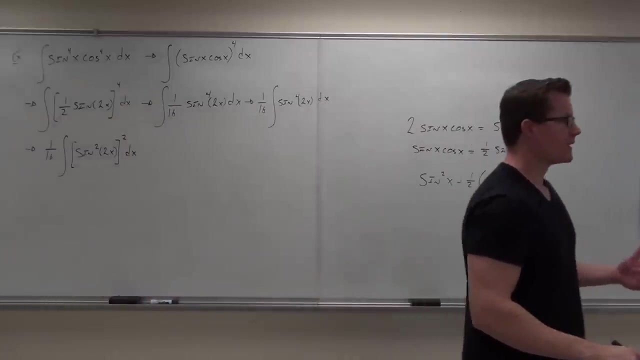 I want sine squared two x to some power. What is it? Square root of four. You all right on that one. Yeah, Now, as soon as you do that, as soon as you go- well, wait a minute, Here's some even powers. 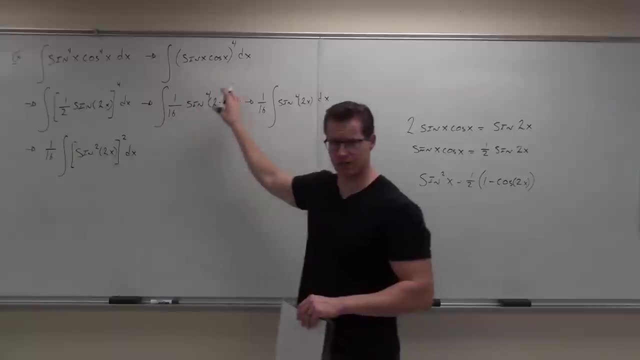 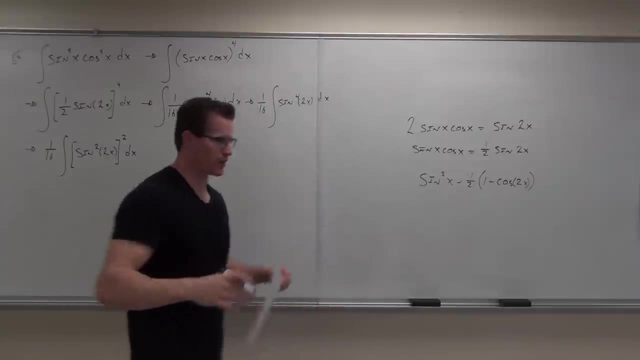 I know I'm going to be using half angles somewhere. Unless I do a reduction formula that works out that nicely, we can do that, But if we can't, then we're going to have some sort of a half angle formula coming up somewhere. 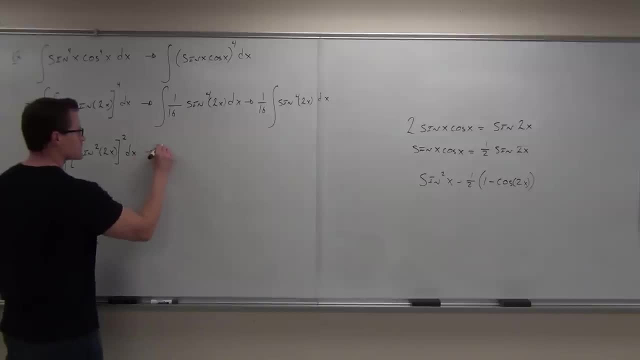 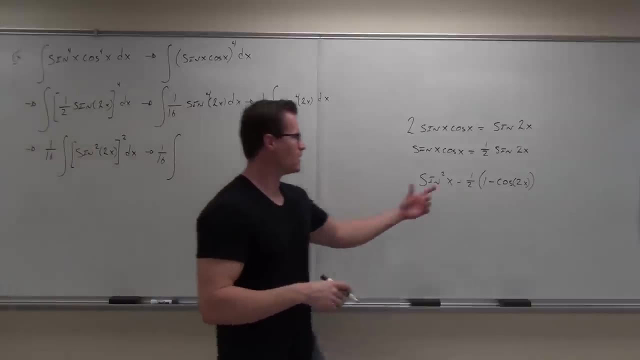 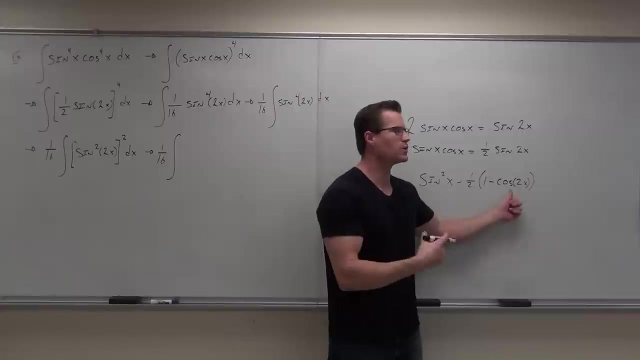 And here's where we go with it. So from here we still get a one-sixteenth Sine squared. Let's do sine squared two x. Let's make it into the cosine. Here's why we do it. If we take sine squared and we change it to one-half, one minus cosine, maybe you don't know why we're going to do this. 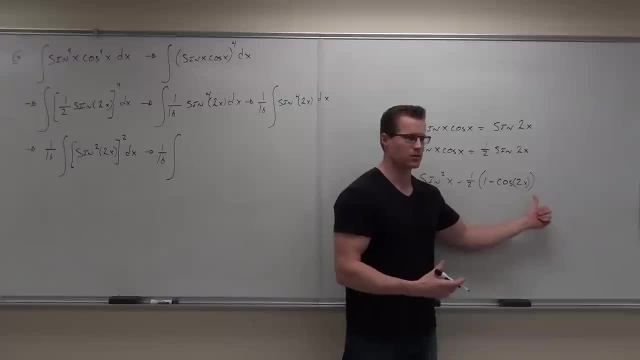 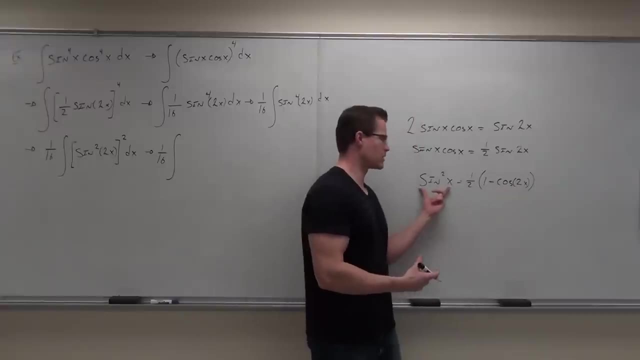 What's the power here? Two: What's the power here? One: What's the power for you? Does that make sense? Two: You can do the integral of cosine to the first power. You can't do the integral of sine to the second power the way it is. 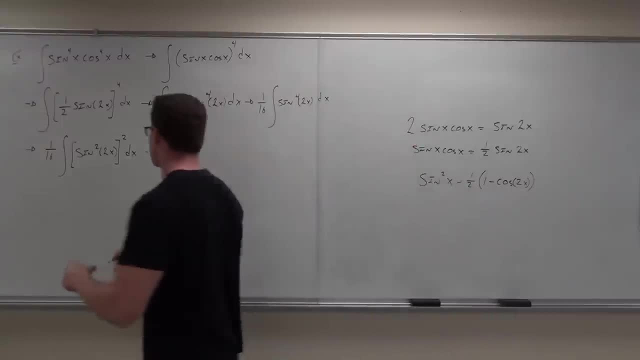 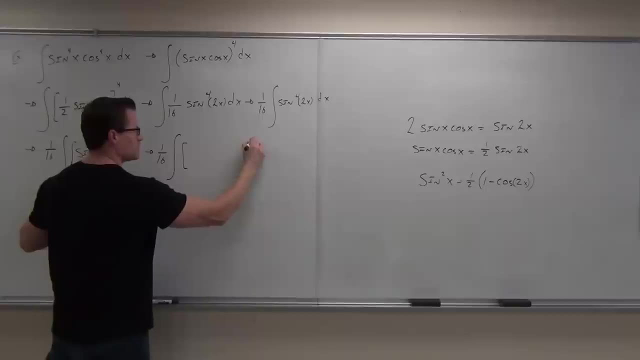 You need reduction formula or you need to make the substitution, So we're going to do that using identity. Now, let's be real careful with this. Don't lose your stuff. What's the power going to be up here? Two, 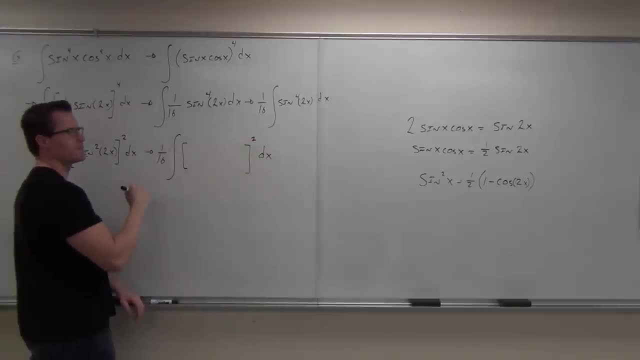 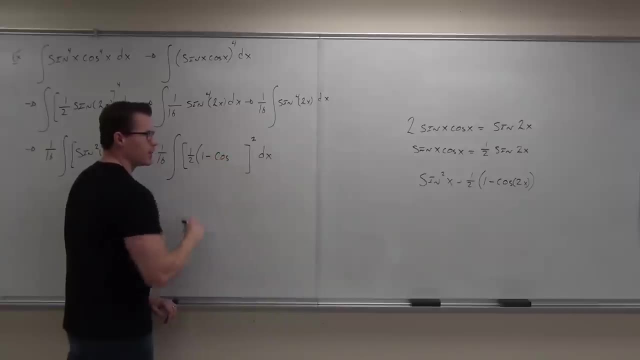 Two. Okay, And then inside, let's do that. What's it going to be? One-half parenthesis, one minus cosine, One minus. Okay, I like that. One-half, one minus, and then cosine. for sure, Be very careful. 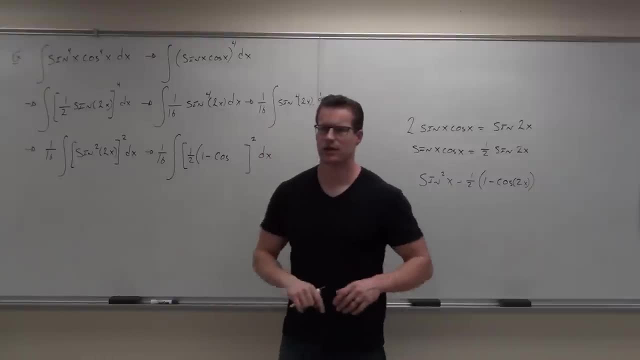 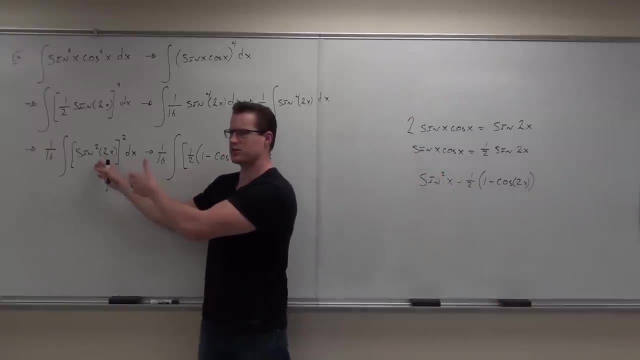 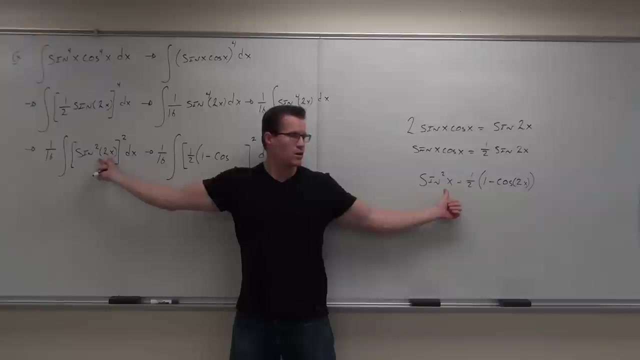 Don't lose pieces of this thing. Two x, It's not two x. Explain why is it not two x? Because it starts from two x. What's the argument of our sine function here? Two x And this says: whatever your x is, you're going to multiply it by two. 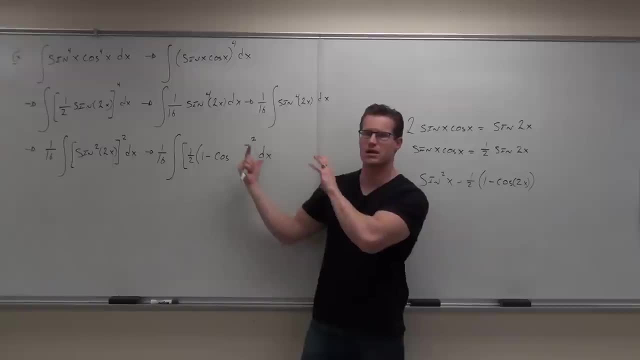 So if we have x, yeah, it's two x. If we have two x, it's going to be Four x. Do you see how common of a mistake that's going to be for some people in here? Yeah, Okay, don't make that mistake. 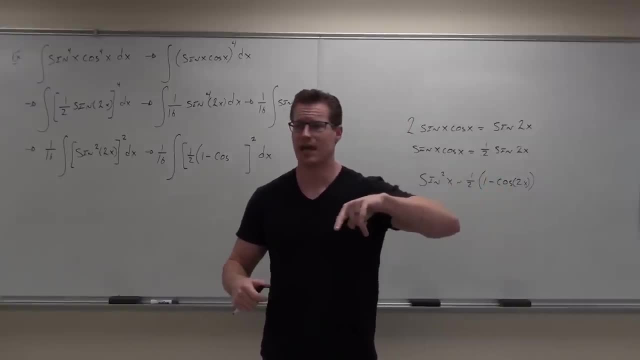 Because then when you do your substitution, you'll have a one-half when you should be having a one-fourth. Does that make sense? Or a one-eighth or something? So this is going to be four x. Be careful, Be careful with your math. 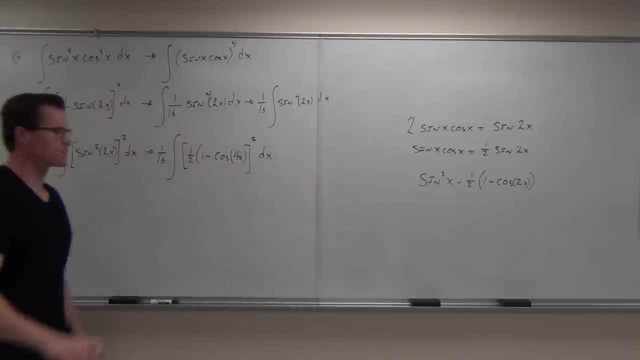 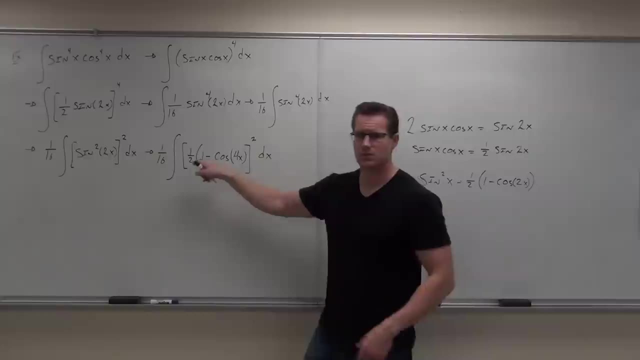 Show of hands if you're okay with that. so far, Good deal. Okay, Now what, Goodness gracious? Well, if we're doing it this way, we can't do a substitution, Because if we substitute for cosine, is there a sine anywhere to be had? 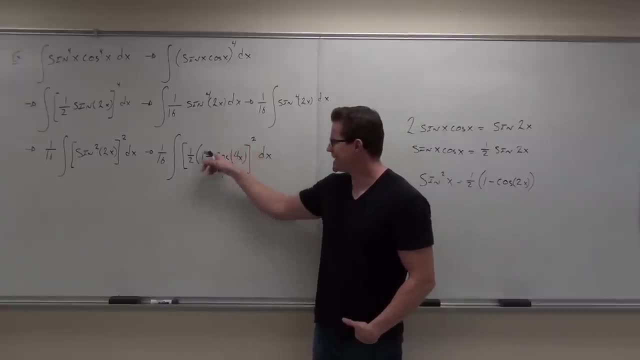 We can't do it. The only thing we can do here distribute all this junk. So what I'm going to do? same thing I did here: I took one half to the fourth. We're going to take one half to the second. 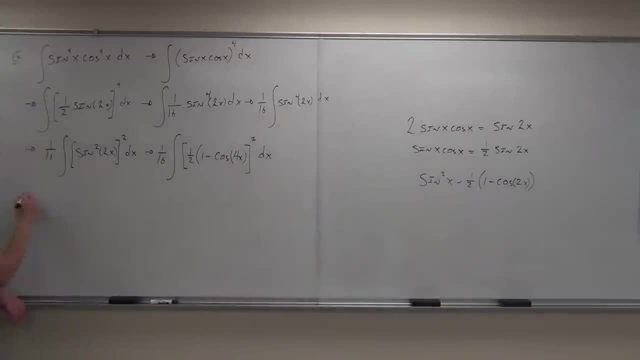 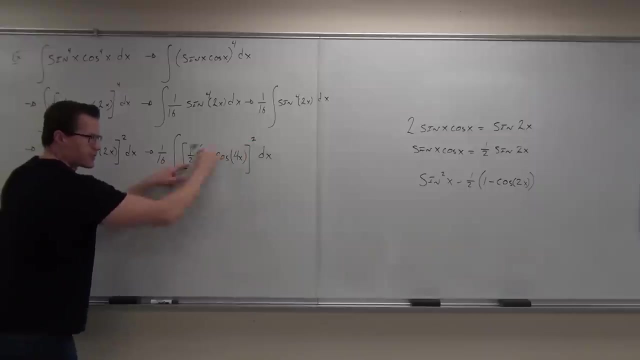 How much is that going to be? One-sixth, One-fourth. So I've got a one-sixteenth out front already. This is going to give me a one-fourth. don't forget about that guy. You need that. 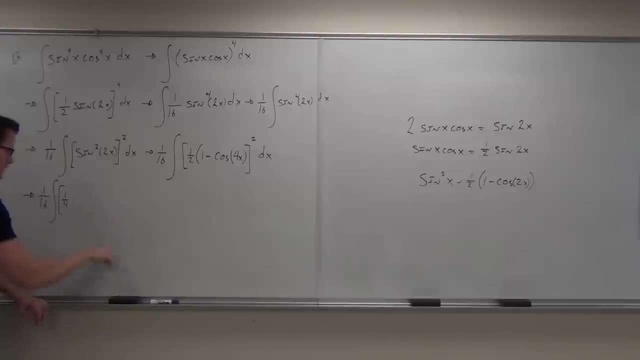 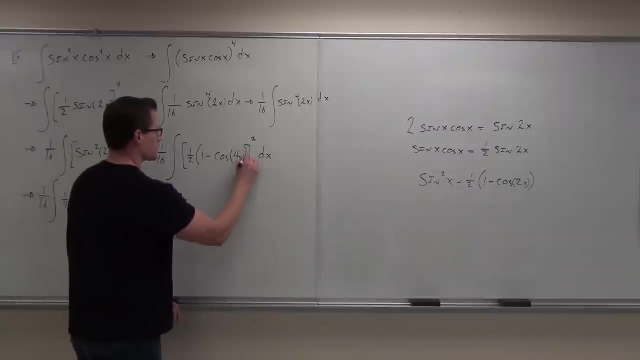 So one-fourth. you know what I need? that bracket. I hope you follow the notation here. All we did was we took 1 half squared, it's 1 fourth. We took this thing now, this thing- now it's this thing- squared 1 minus cosine 4x to the. 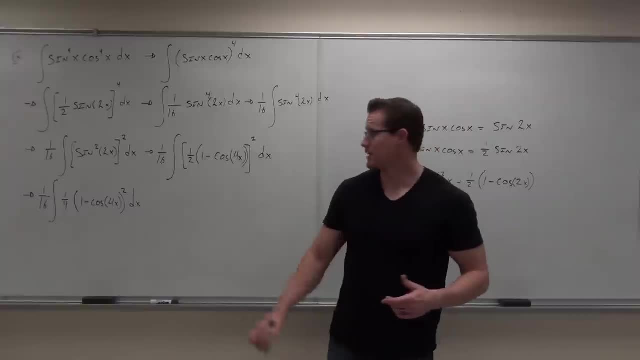 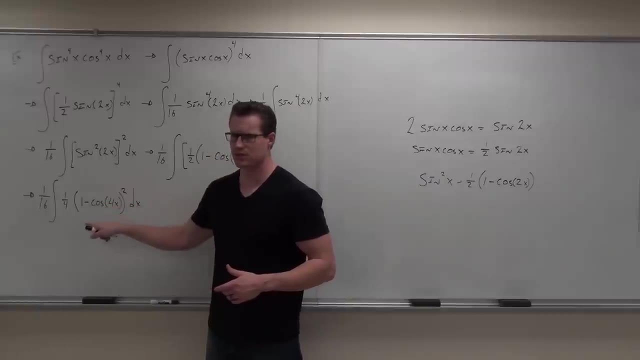 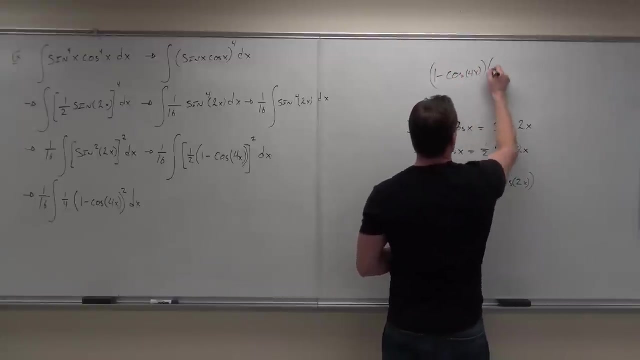 second power: Click head nod. if you're okay with that one, Can you guys distribute this? Are you just going to square this and square this? No, Please, for heaven's sakes, don't do that. Remember that what this means is 1 minus cosine 4x times 1 minus cosine 4x. 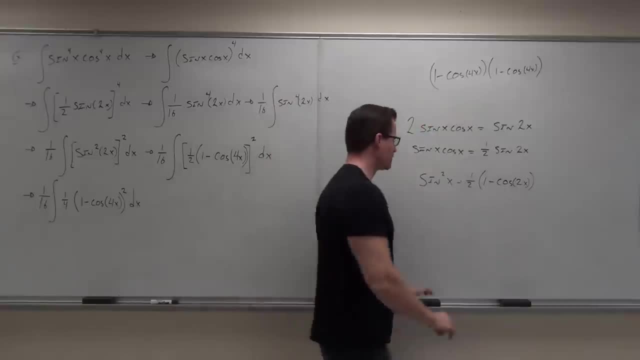 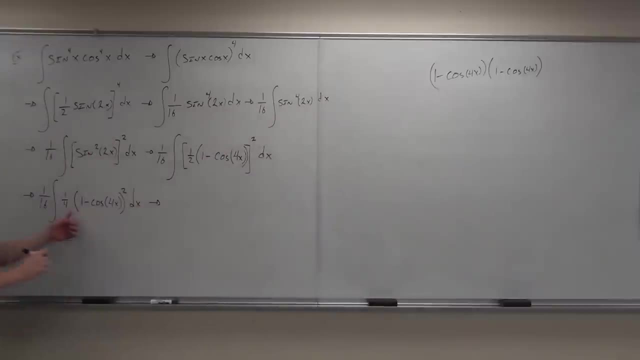 Would you please spend some time to distribute that for me? Go ahead, go ahead and distribute that for me. What I'm going to do is I'm going to pull the 1 fourth out front. We have a 1 16th. we now have another 1 fourth. 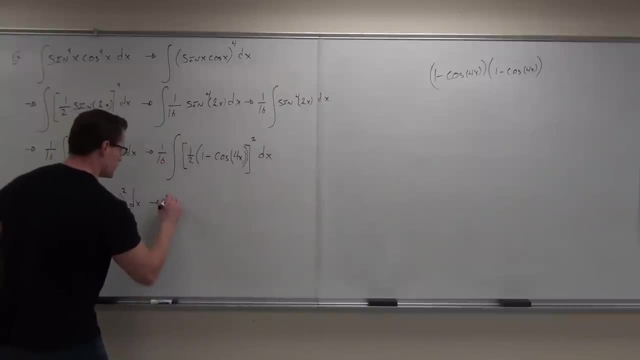 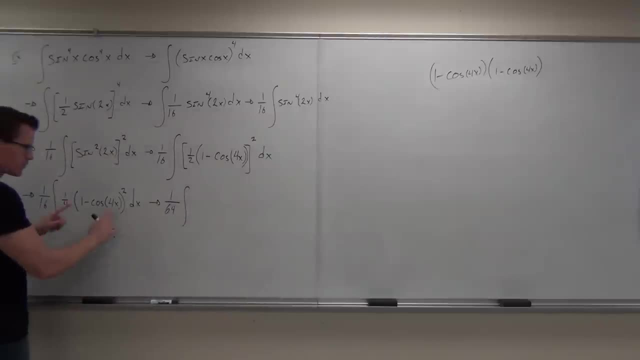 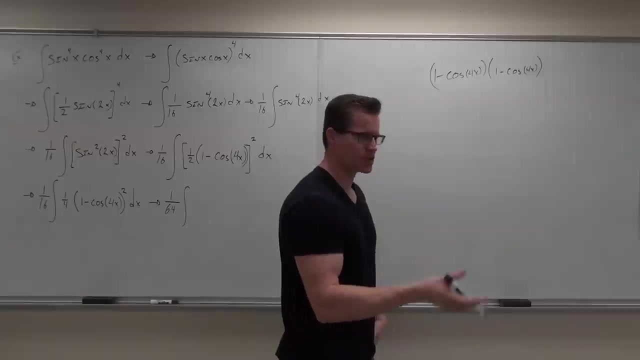 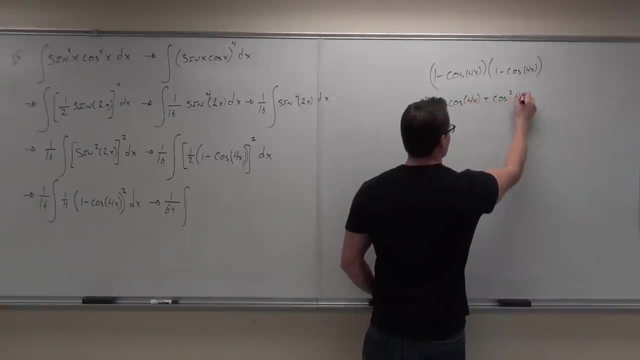 1 16th Then, so this now combines to 1: 16th. You guys are distributing this right now for me, so hopefully you get this. It's usually not very hard. You guys know how to FOIL. This is 1 minus 2 cosine 4x plus cosine squared 4x. 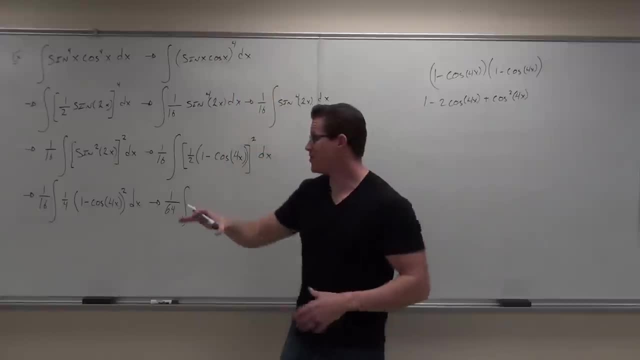 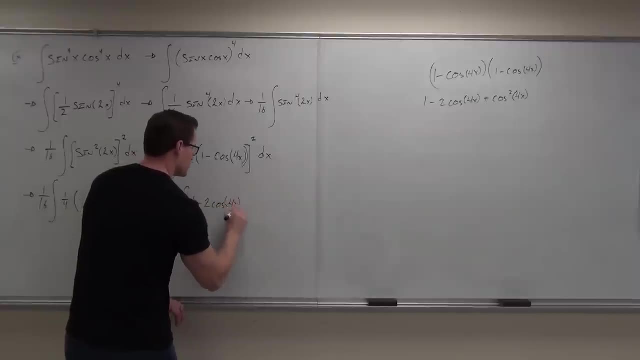 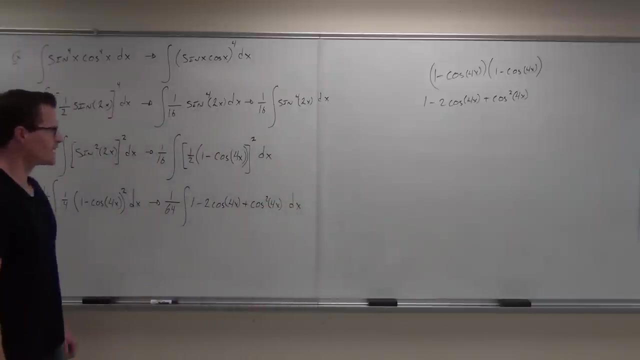 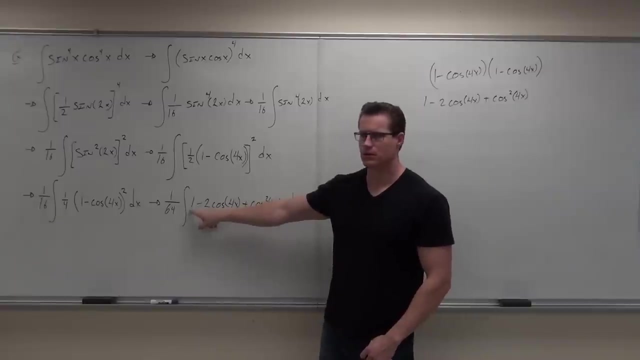 How many of you got that? Perfect, That's what goes here. Let's take a real close look at our integral and see what we've got going on. If I asked you to, could you do the integral of 1?? Yeah, no substitution, that's a piece of cake. 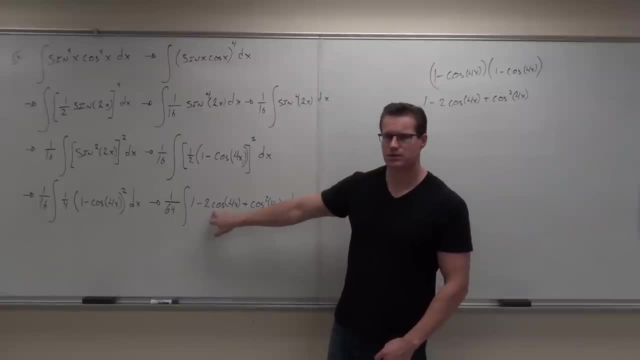 Could you do the integral of cosine 4x? Yeah, what's the integral of cosine? Now you'd have a 4x that would be over 4.. You'd need a little substitution. I typically do those in my head. 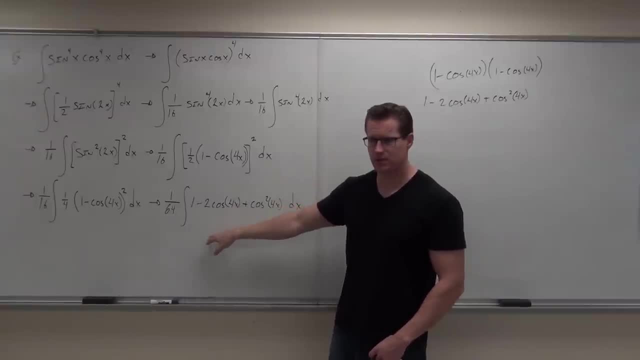 U sub on that would be over 4.. Does that make sense to you? Now? can you do this one? Okay, let's try this again. Integral of this. could you do it Easy? Integral of this: could you do it without a substitution? 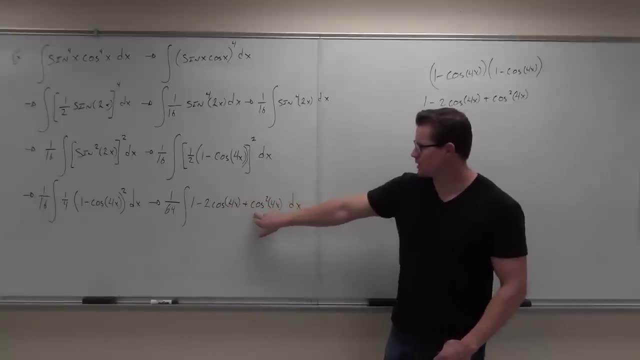 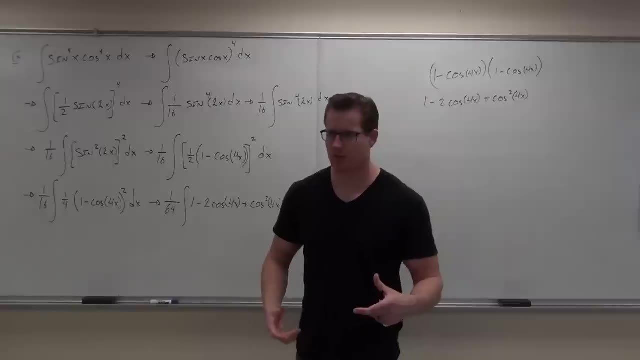 Little substitution, but that's easy. Can you do the integral of cosine squared? Is that anywhere in your integration table? No, no, We've got to go over again. So we start from the very beginning with our trig stuff. What power do we have? odd or even. 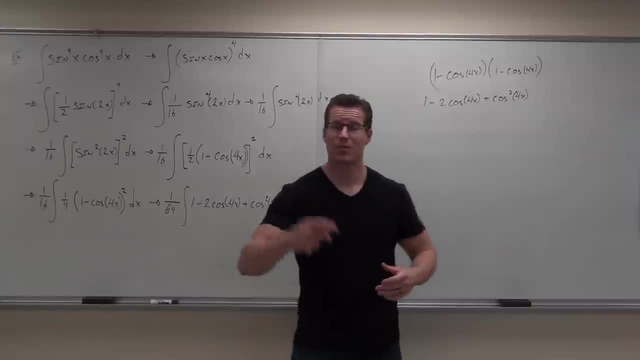 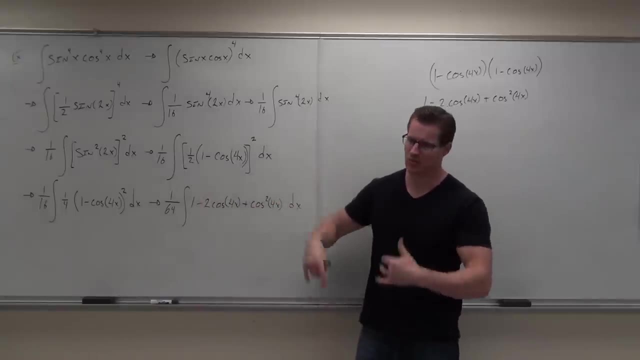 Even power With even powers. we use what Pythagorean identity? or half angle? Which one Half angle? Ah, do we know a half angle for cosine squared? Yeah, we do That. lets you break that down again. There's lots of steps here. lots to this. 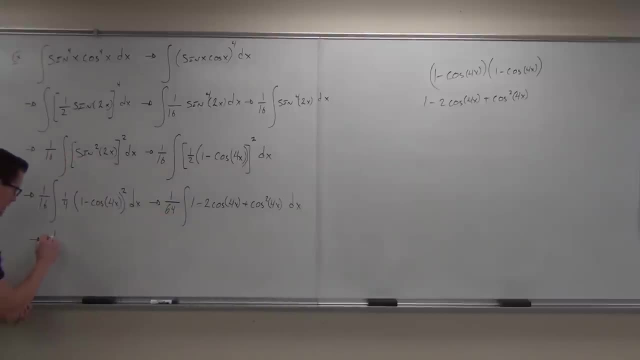 Be very careful. write these all out. I know some of you don't like to write steps and I'm going to say two is stinking bad. do it anyway. You've got to write this. you've got to be able to do this. 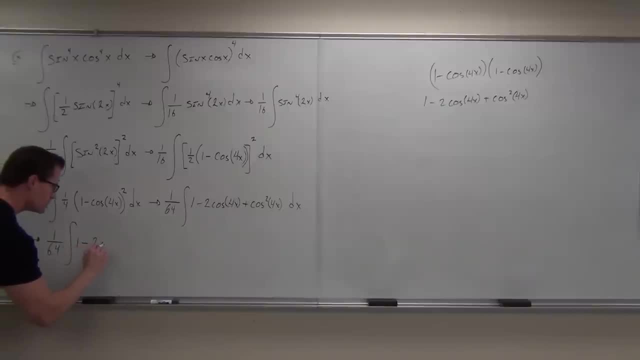 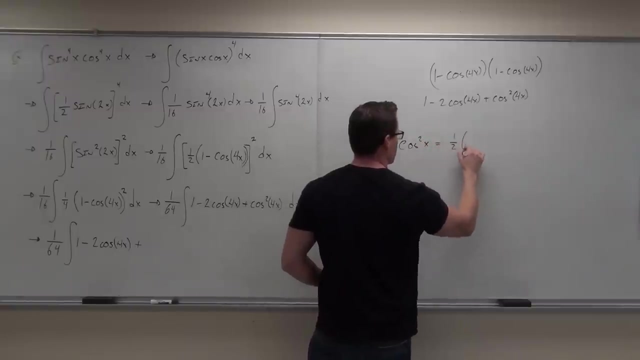 And make no mistakes on it. So we have 1.. We've got minus cosine 4x. We've got a plus. let's look inside here. Remember that cosine squared x equals 1 half 1 minus cosine, oh sorry. plus cosine 2x. 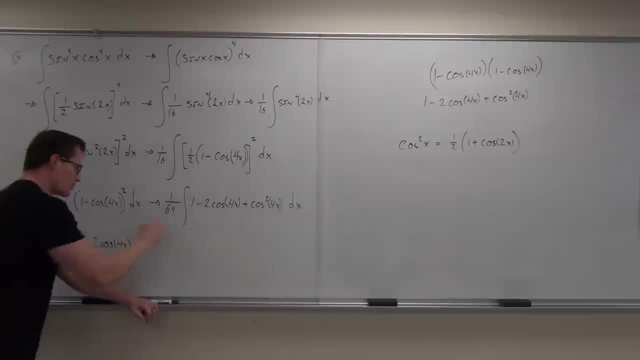 Hopefully we're familiar with that one. Let's apply it here. I've got the 1,. I've got the minus. cosine 4x: I've got the plus. What am I going to write next? One half, One half, got it. 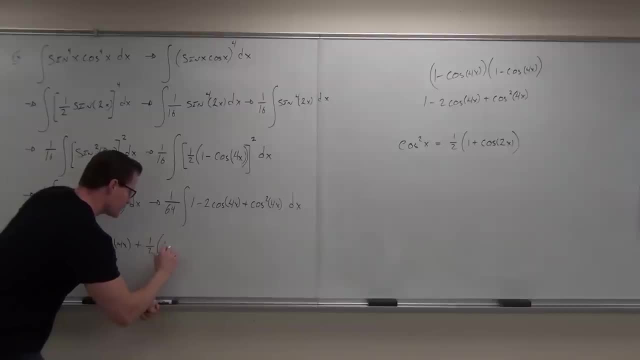 Keep on going. Come on, tell me 1 plus cosine 2x, but don't forget the first Oh 8.. No, 2. Okay, now you all need to be careful on what the argument of that thing is going to become. 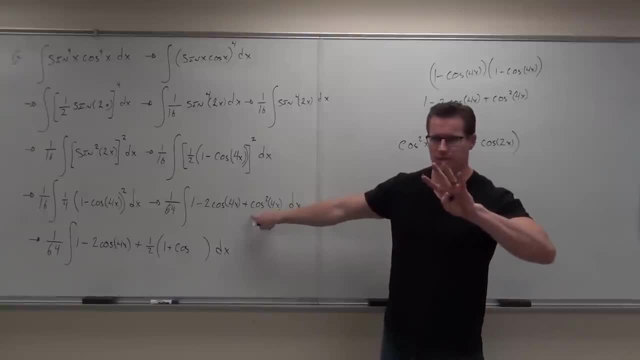 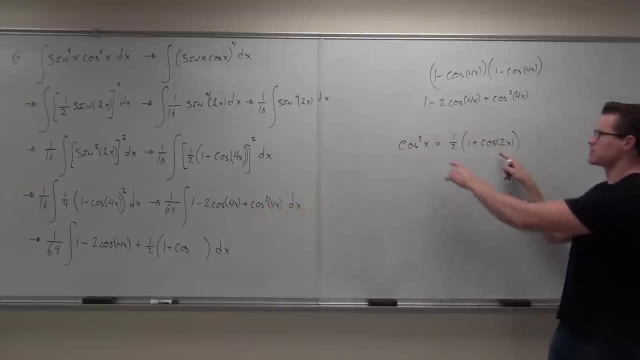 Listen, we're starting with cosine squared of 4x. If cosine squared x gives me cosine 2x, cosine squared 4x gives me cosine. remember you take the argument, you multiply it by 2.. What is it? 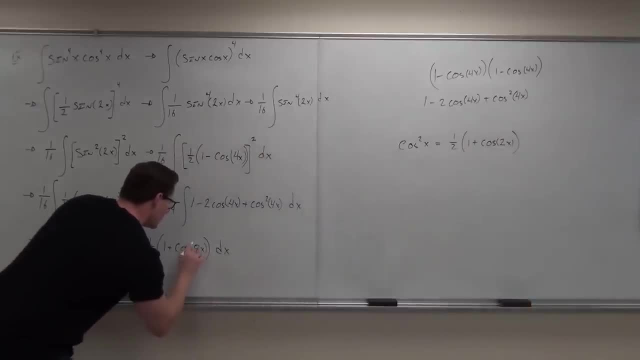 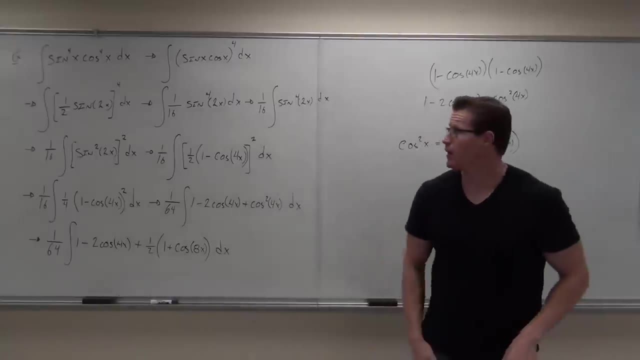 Perfect, Okay, I'll tell you what we're almost done. I want to do about a 10-second recap to make sure you guys are good with this stuff. You okay with the? maybe I'll do the fourth power, Yeah. 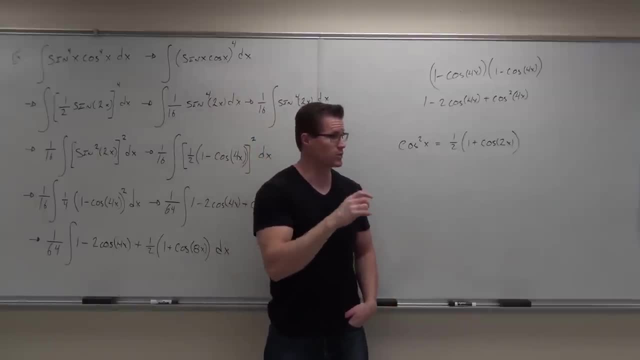 It's a special case and I get that You're not always going to have the same power there, But when you do, man, try something like this, It's kind of nice. Use an identity. Are you going to have to know your trig identities? 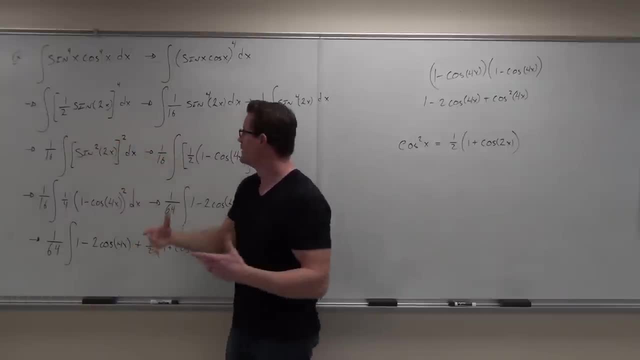 Yeah, otherwise this stuff doesn't make sense. You've got to have that down. People take calculus 2 to finally fail trigonometry. People take calculus 1 to finally fail algebra. all right, But this is this is trig. 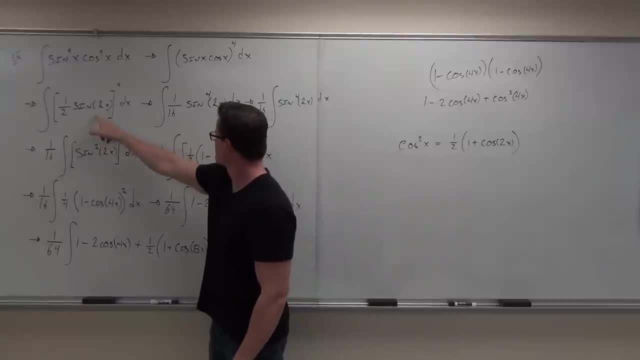 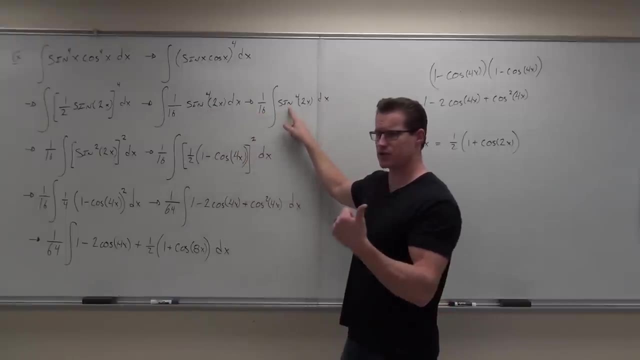 I mean, my goodness, we're going to use a lot of trig. Then we go, Okay, well, that's cool. You know what? We can just take it all to the fourth power. We recognize this one as either a reduction formula that we could do. 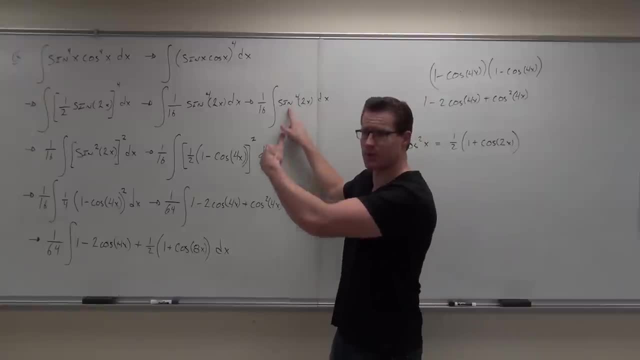 which probably would be a little bit quicker than this. to be honest with you, Sometimes you won't be able to do reduction formulas. Sometimes you will, Or we go. well, I didn't remember that, So let's practice doing the whole, even power thing. 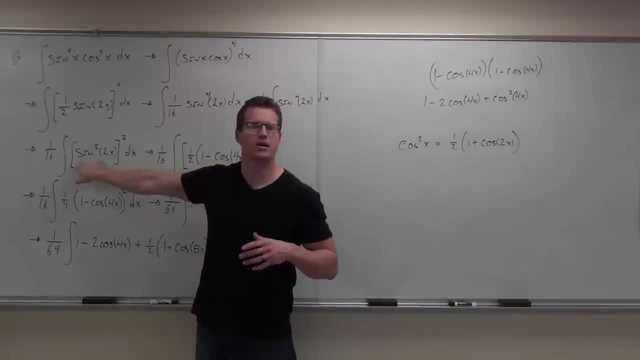 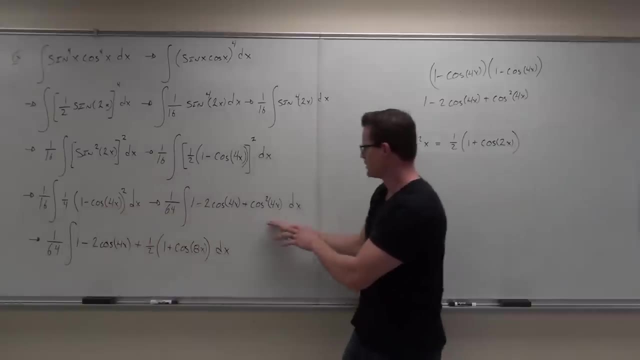 The even power thing is: make it a sine squared or make it a cosine squared somehow. Then use a half angle, Cool. Then distribute it. Look for any more squares. You're basically reducing this with a half angle formula. It's like an inherent reduction formula. 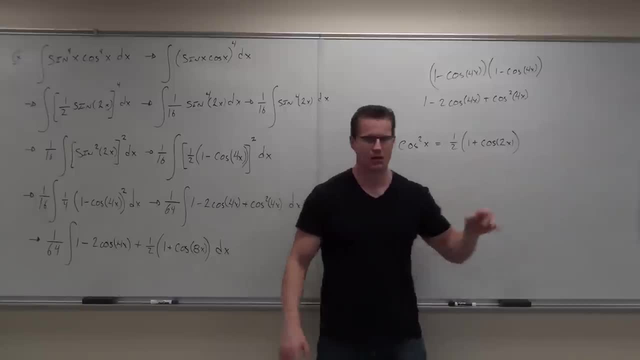 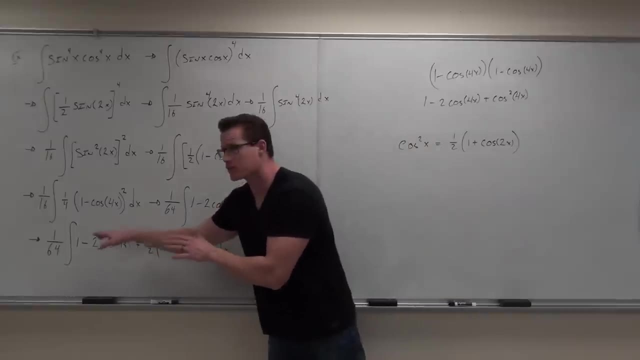 The half angle formula always reduces your power. Do you get what I'm saying? So we look again. We go okay. well, we've got to do it one more time. Half angle again reduces the power. one more time Now we have everything to the first power. 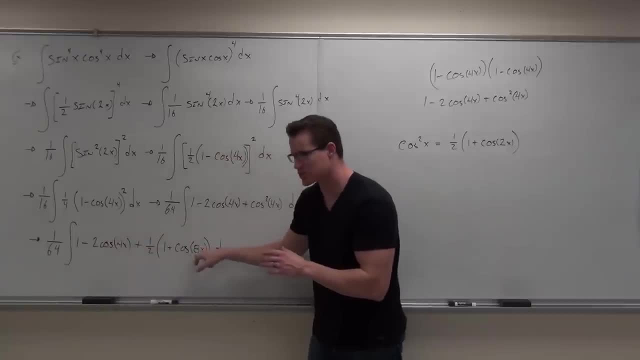 We've got 1. No big deal. Cosine to the first. We're going to distribute this in just a bit. Cosine to the first. Let's pretty this thing up a little bit. What are you going to do here? 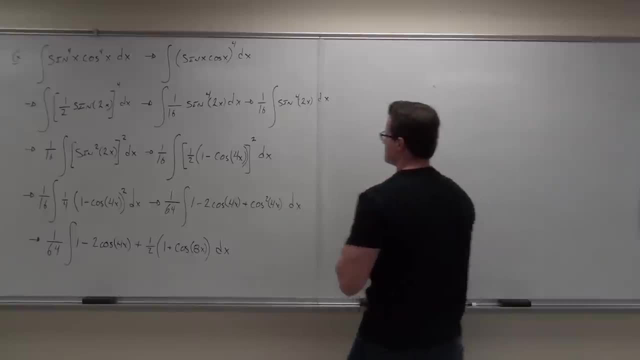 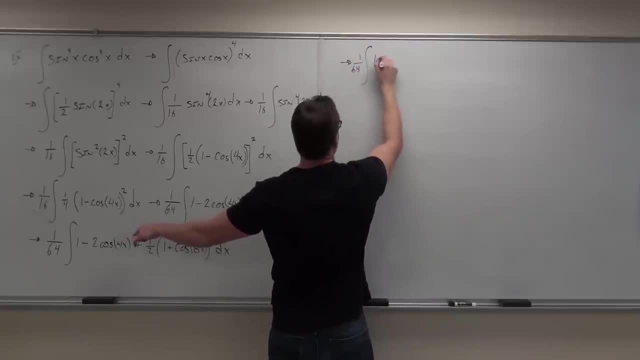 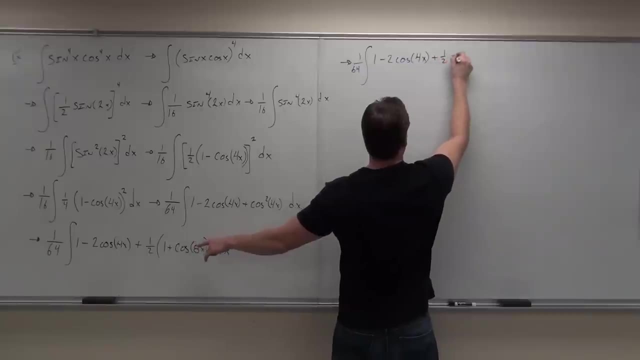 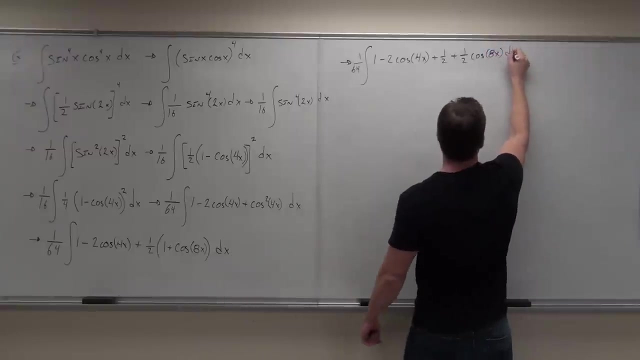 So we've got 164.. We're going to have 1 minus 2 cosine 4x- Don't lose track of that- 4x Plus 1 half plus 1 half cosine 8x dx. Okay, I'll tell you what. 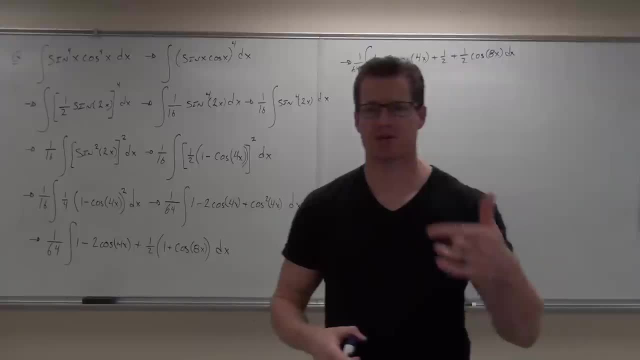 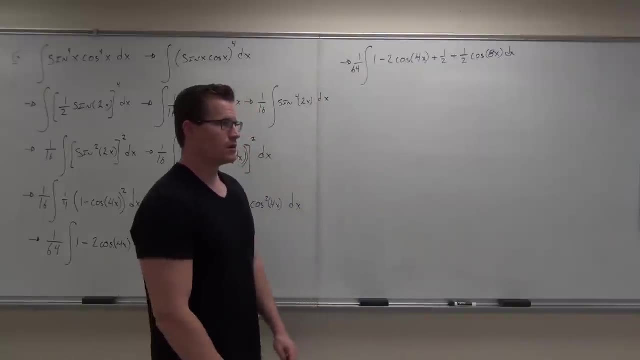 Whenever you distribute an algebra, the one thing that you should probably do after you distribute is check for what That's right like terms. Do we have any like terms here? Yeah, Yeah, just combine those numbers. This is 1 and 1 half. 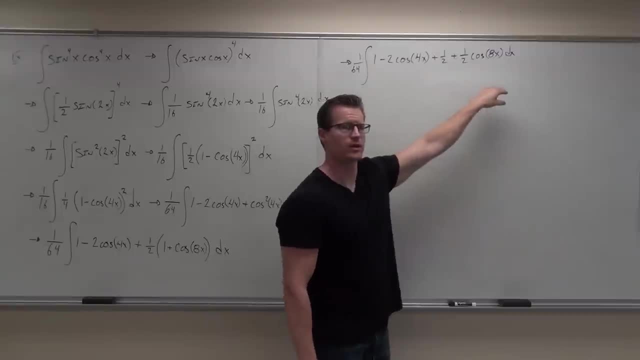 That's 3 halves. That will make you integrate one less term here, which is kind of nice. Combine your terms if you have any. Can I combine cosine of 4x and cosine of 8x? No, That's a no-no. 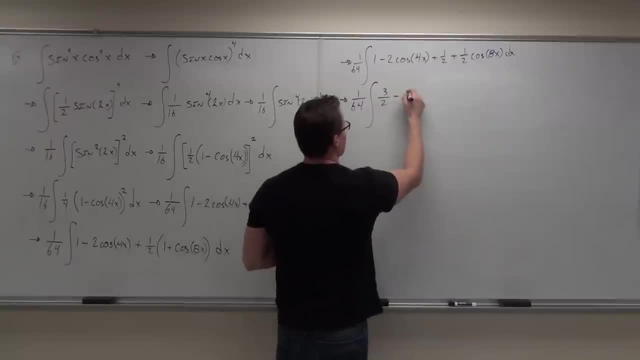 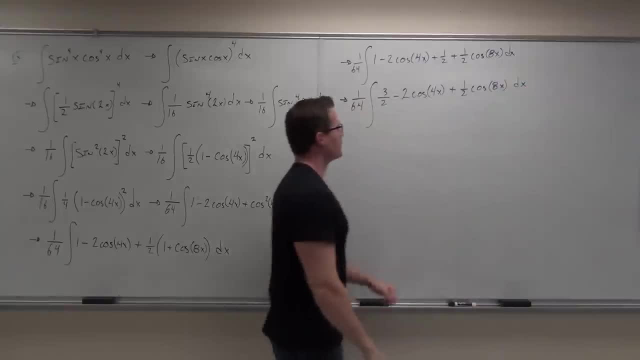 That's 1 half of cosine 4x plus 1 half cosine 8x dx. My goodness, that's a lot of junk. I want to make sure that we're all good to go. Do you guys feel OK on what we've done so far? 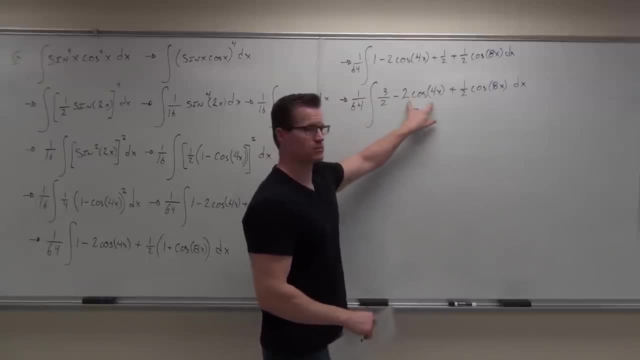 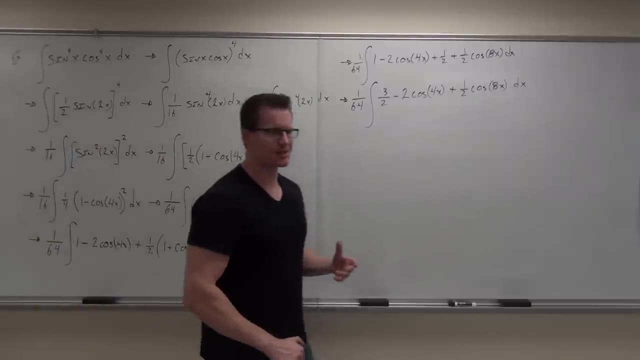 Yes, No, Nope, Nope. OK, Can we integrate that little piece? Yes, This one, Yes, This one. It's the same thing. It's integrated When you do it, just be real careful with your constants. That's typical. 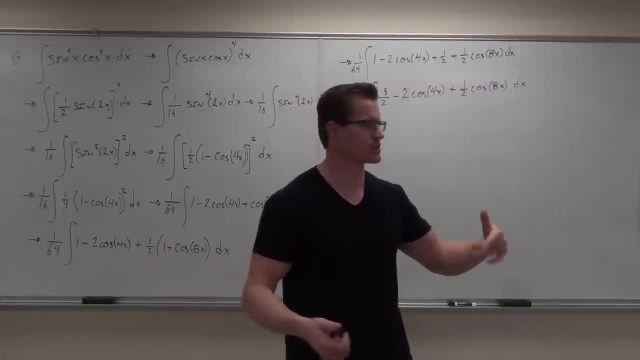 I mean almost nobody, Almost nobody. Oh no, it's sine, It's the constants that are going to get you here, so don't lose track of stuff. We're going to have 164.. We're going to have a big old bracket here. 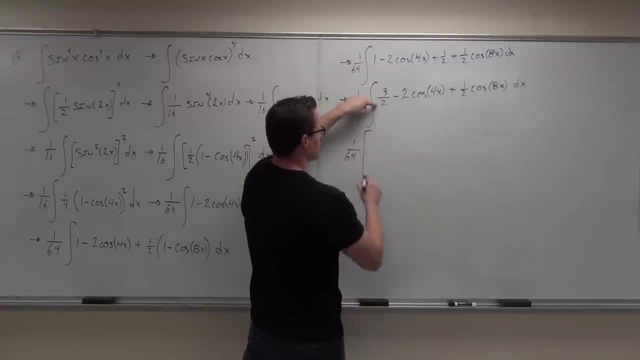 Let's integrate piece by piece, Integral of three-halves: Three-halves x, Three-halves x. very good, Minus. here's how integrals work. If you want to do these in your head, this is the way I do it. 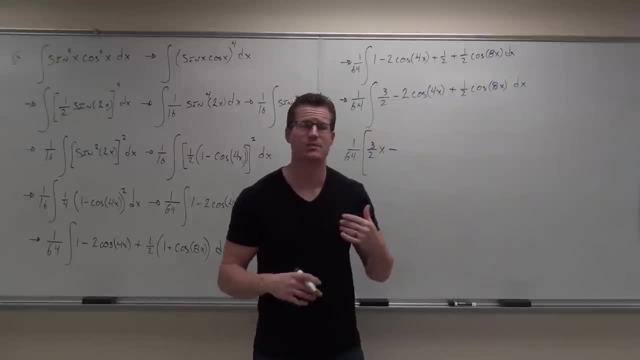 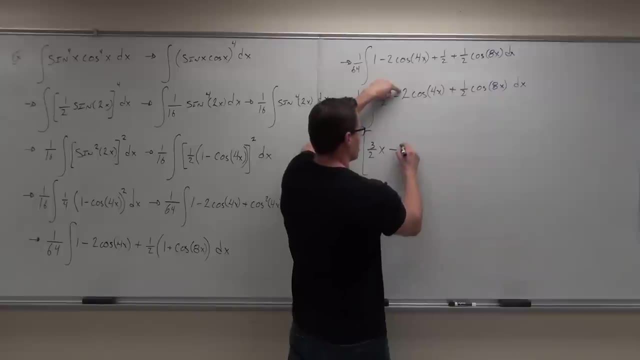 I do little substitutions in my head because I don't want to waste my time. So watch, Watch. here's what you do. The two is a constant, correct, Yes. Integral of cosine. It's sine. It's sine four x. What's the derivative of four x? 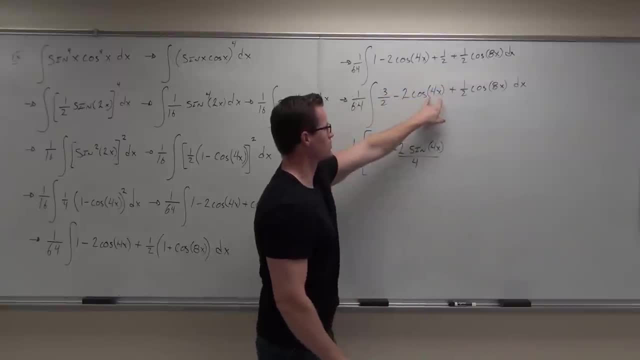 Four Over four. That's how you do it. So derivative of this thing- that's a basic substitution. when you just have constants, It'll typically work with those arguments. You should put it over, whatever the derivative is. If you notice, this is coming from the du over four that you would get. 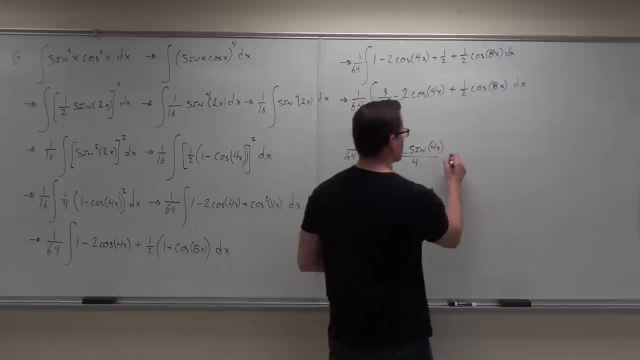 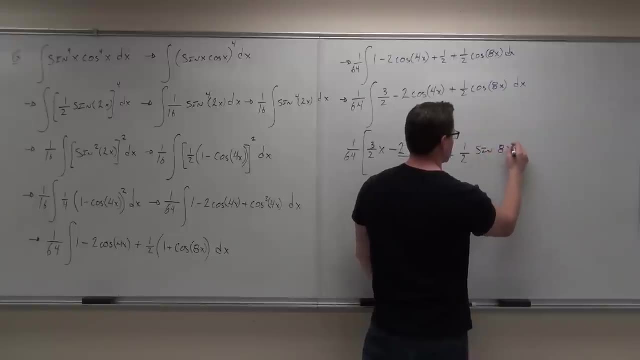 Does that make sense? So that's where it's coming from. Let's try the next one. What's the next thing I write One-half? Next thing: Sine eight, Sine eight x, Sine eight x Over eight. 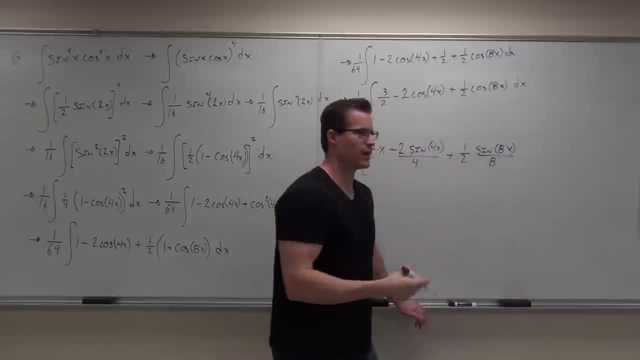 Perfect Over eight. Now we're able to do those without actually having to write a special substitution on that, because that takes a little while. right, You have a substitution here. You have another substitution here. That takes some time. Can that two and four cancel out? 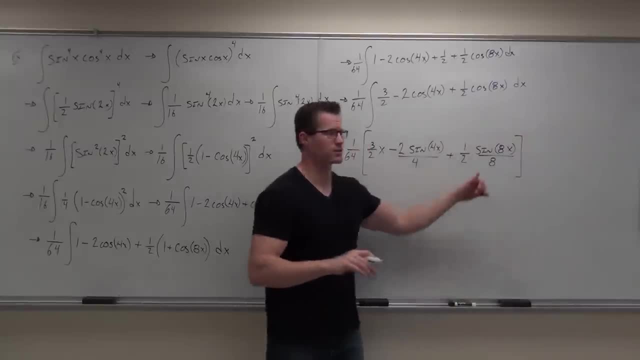 Well, we're going to talk about that right now. I want to make sure you guys are good on this so far. Show your hands if you are Okay. so yeah, a few things are going to happen. Of course, we're always going to look at simplifying. 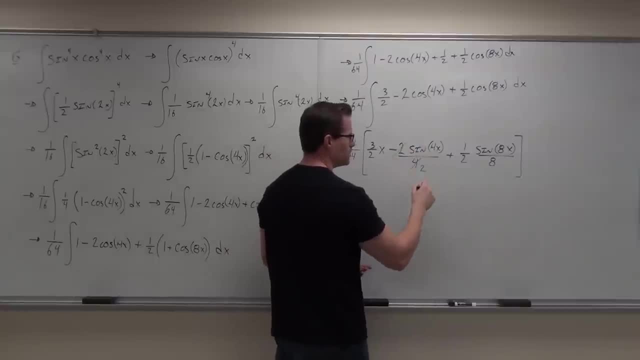 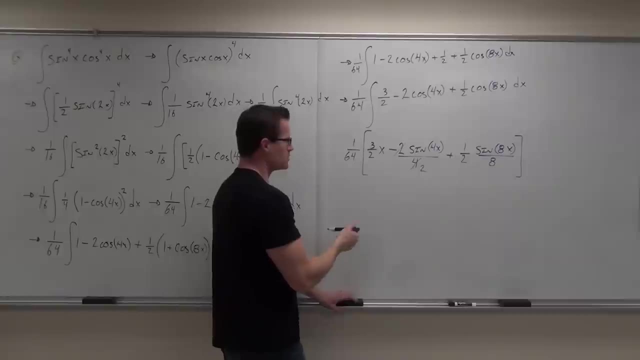 Two with four done, This becomes what? Sixteen? Okay, and then maybe we'll distribute, Maybe you won't, It kind of depends. I'm going to distribute because I want to, So we'll have three over one hundred twenty-eight x. Oh goodness. 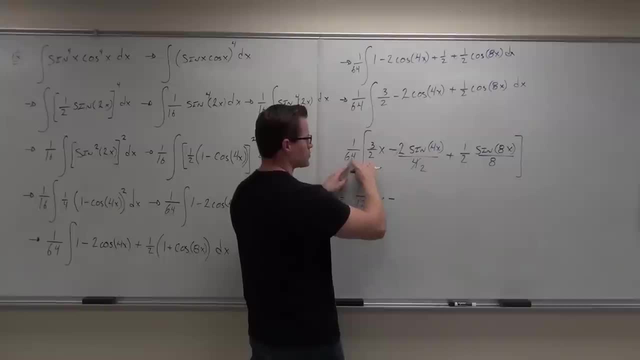 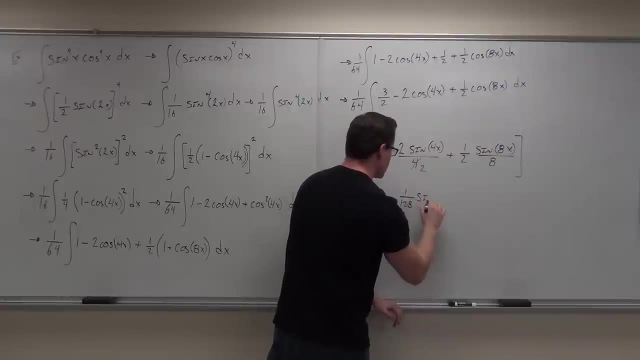 We'll have minus. what do we distribute? Notice, this is a one-half, Yeah, One over one hundred twenty-eight sine of four x plus wow, what's this going to be Sixteen. So basically you have sixty-four times two times eight, or sixty-four times sixteen. 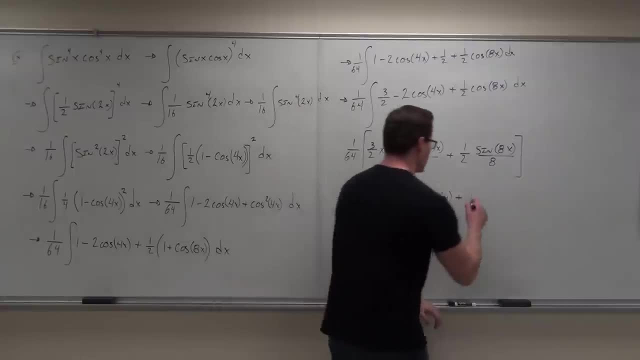 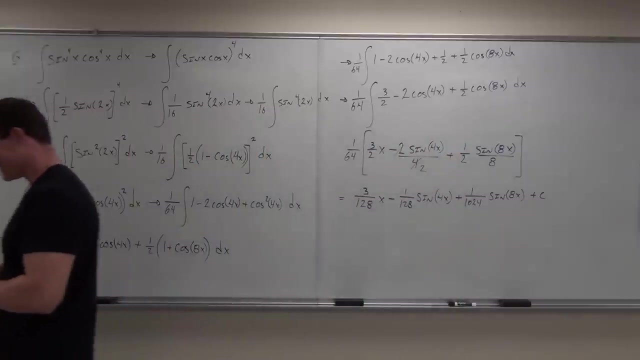 I don't even know. You tell me what it is. Thousand twenty-four Sounds good. I'll take your word for it. Sine eight, x and finally Plus c, Plus c, Yeah, Wow, Wow, that was a lot of work. 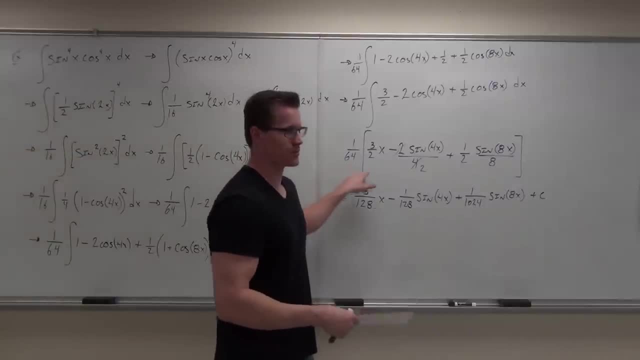 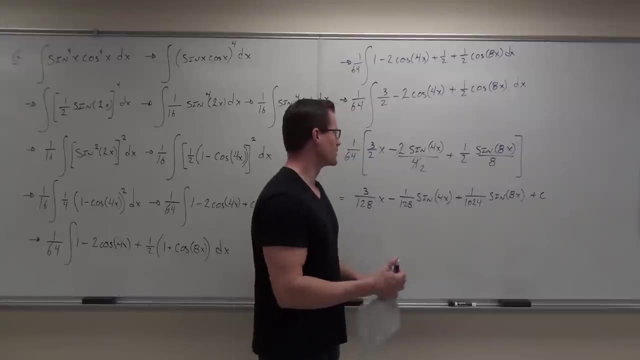 It wasn't bad. Could you have left the sixty-four? Absolutely No problem. You could have just left it. You could factor out something else. Steve question Totally: should have just factored out a one-half. Yeah, you could have. You could have factored out a one-half and made it one, twenty-eight and then three x. 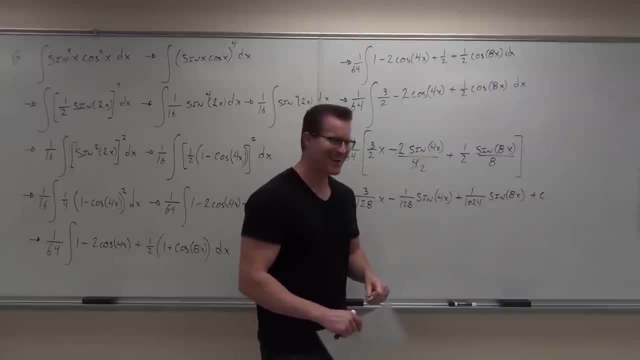 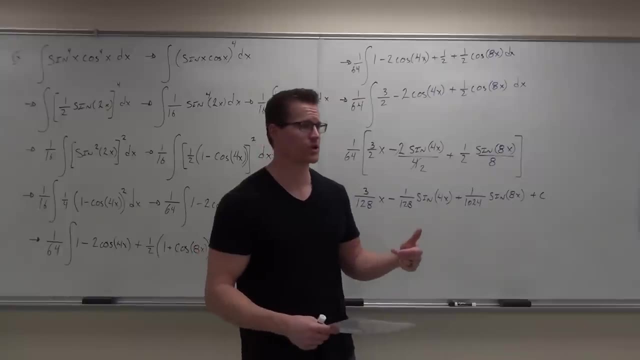 Should have just done reduction. Should have just done reduction. That's right. But you know what? There's times when you can't right. So I want to get you really practicing this. The next one. you see that we're going to be able to do that as well, but I want to see you practicing this method. 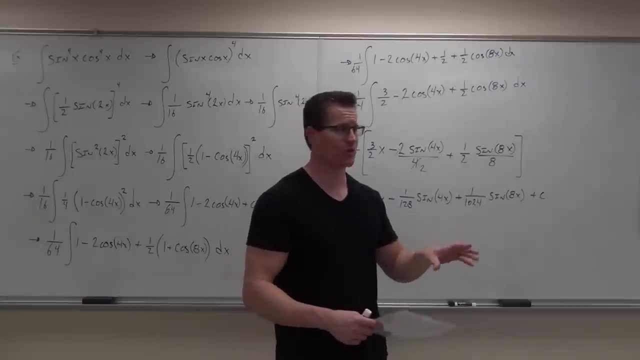 Does that make sense to you? Yeah, So I get it. If the reduction formula works, that's what I would do. Notice that this is going to be a little bit more concise than the reduction formula. Reduction has sines and cosines in it. 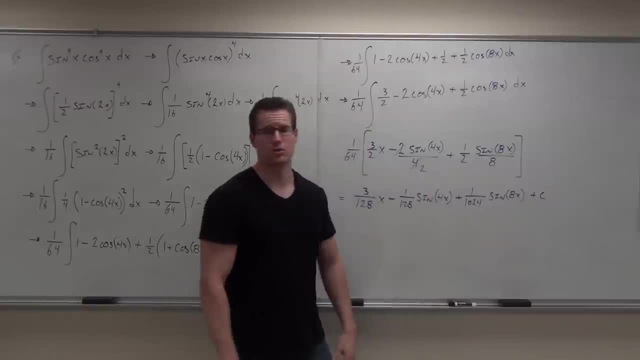 So this would be a little bit nicer in my opinion, but you could do it with the reduction formula. Are you guys ready for the next one? Yeah, Okay, the next one's going to be some work. Question: If we were to use the reduction formula, is it possible that we could get something that looked different but was equivalent to that? 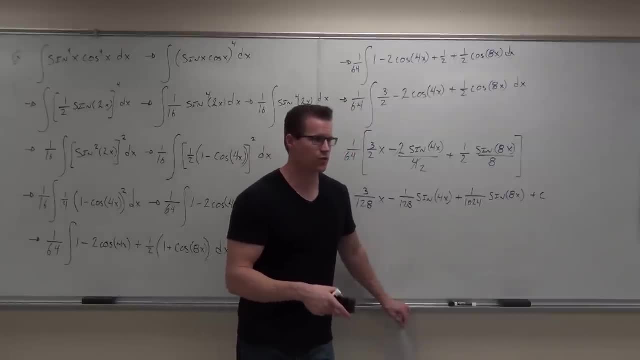 That's actually just. what I was saying is that when you do reduction formula, it's going to have sines and cosines. The integral will be equivalent And you can get the same thing with identities, but it's going to look different. 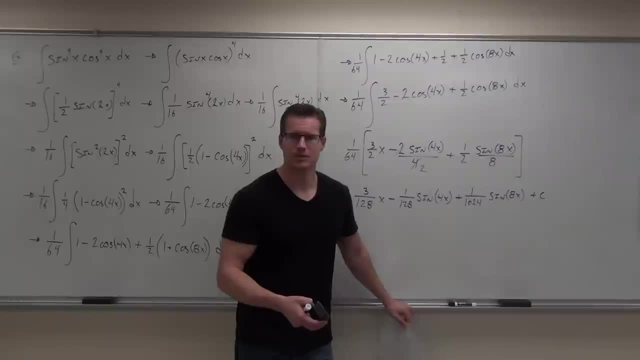 Okay, Well, how can you know? it's the same thing. You do the identities to prove it, Like all those times in trig where it said: prove this identity. That's how you do it, That's why they had you do those. 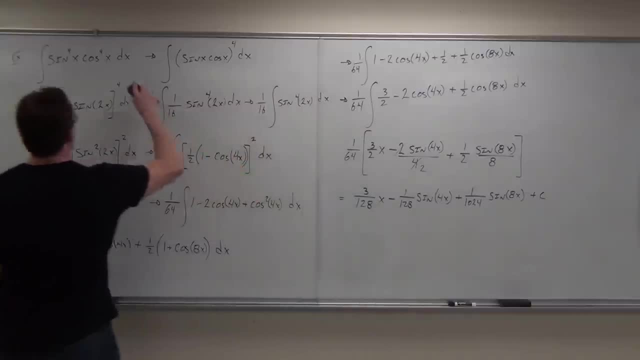 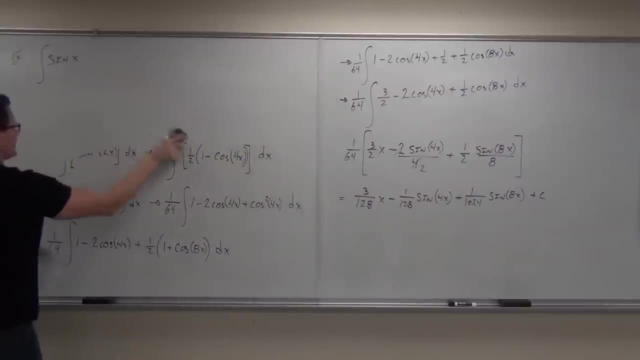 That's why they had you do those. So anyway, let's continue. Let's do this one: Integral sine. Yeah, Okay, there's no dx there, so I drew this one wrong. You just say can't do it. 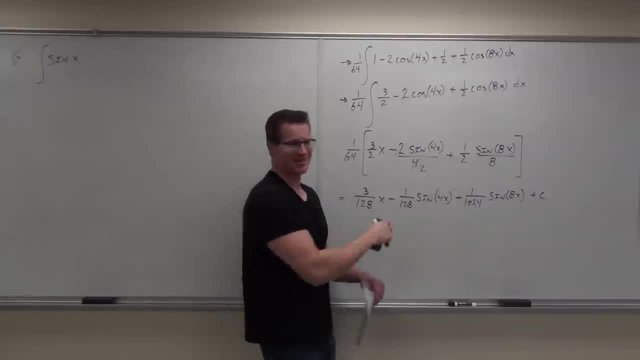 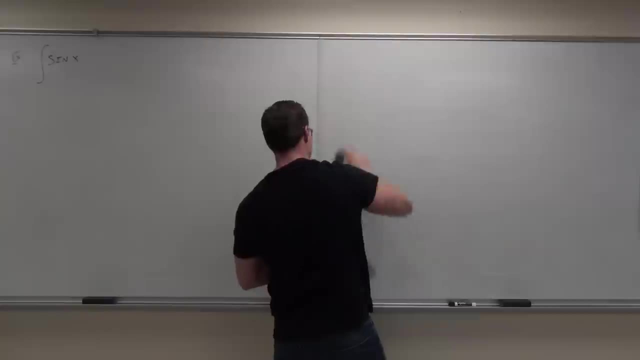 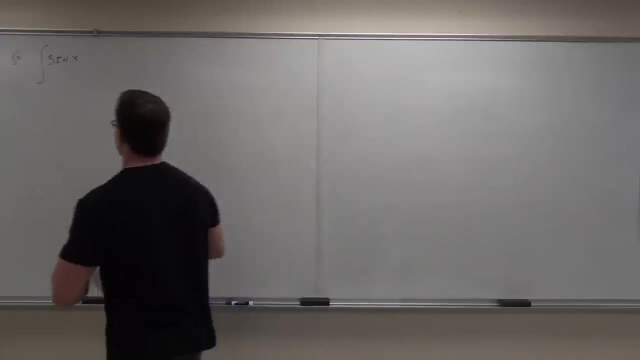 Oh yeah, Did you have any questions on that? Pretty good, Just watch the video. That's right, Watch the video again. Okay, there you go. Questions Too bad, Just joking. Let's make this sine to the sixth dx. 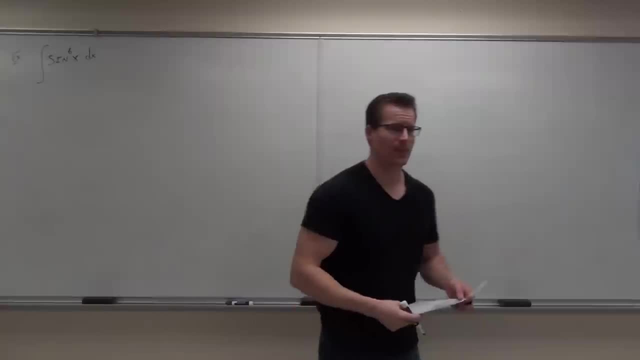 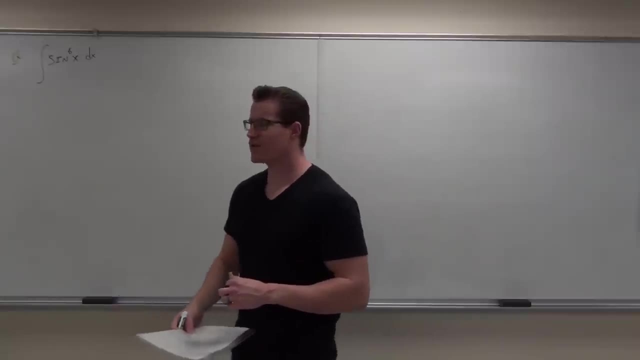 Now, what would you use here? I would use reduction formula. What if you didn't know the reduction formula, forgot it, just missed it? or just want to practice, like I do, on doing it differently? Can we do it? Yeah? 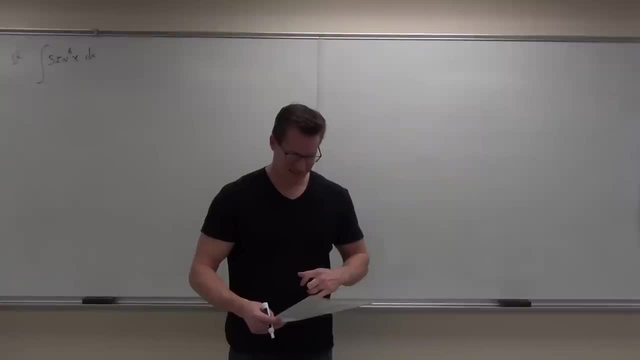 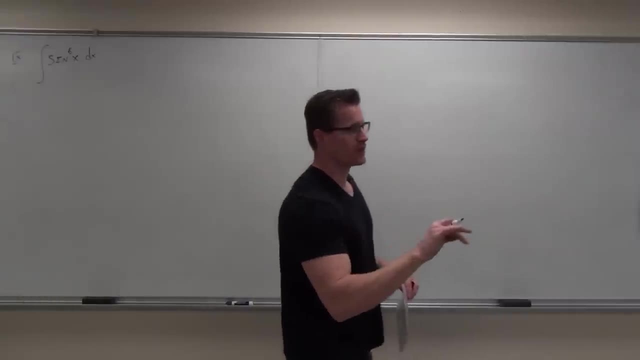 Of course we can. Is it going to take a lot of work? Yeah, Yes, Yes, it is. So how would you do it if you didn't have the reduction formula Sine of x to the sixth power, Sine of x to the? oh, you're close, but no. 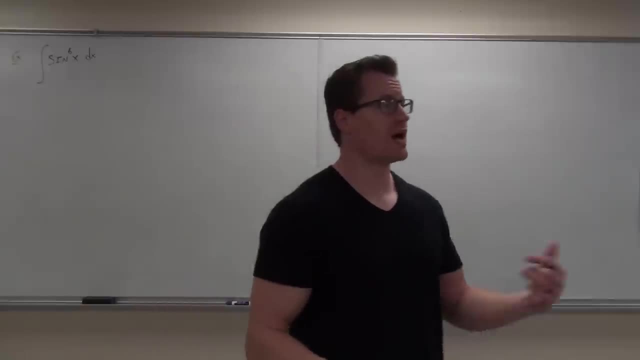 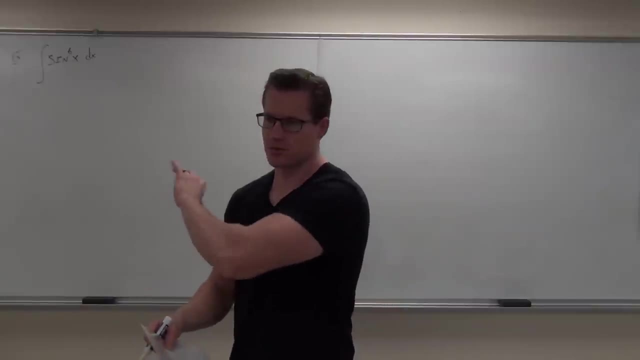 You see, if I have even powers, let's look at the powers. Do I have odd powers? No, I actually have two even powers. If you don't think there's two of them. kind of Cosine is zero, so it doesn't really count. but I have sine to the sixth power. 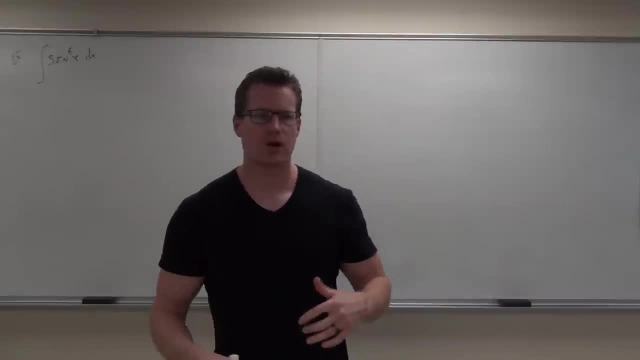 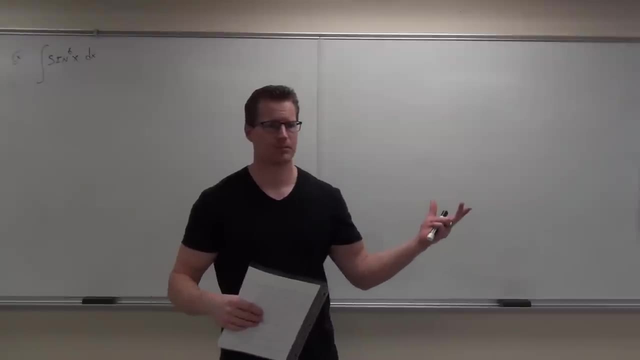 That's my only power. It happens to be even. So, what are you going to use, ladies and gentlemen, when you have all even powers? Will you use Pythagorean theorem or half angle, Half angle, Half angles? So we need to make this a half angle. 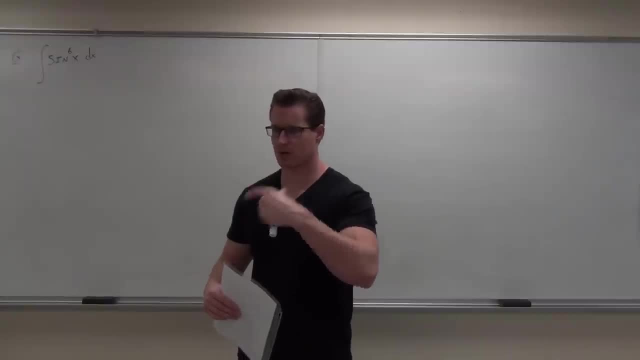 Half angle only works if you have sine squared or cosine squared. So somehow I want you to rewrite that with a sine squared. Go for it And don't write out sine squared times, sine squared times, sine squared. okay, You could, I guess, but it's going to be the same. but it just looks sloppy. 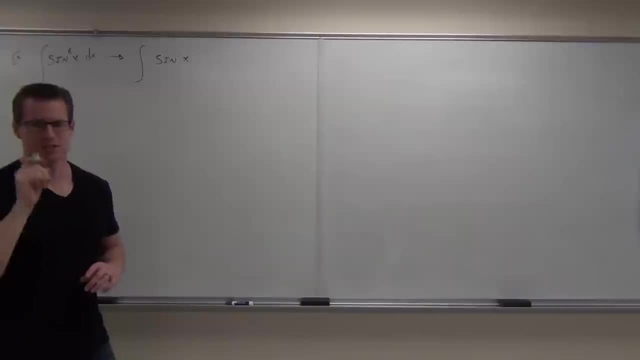 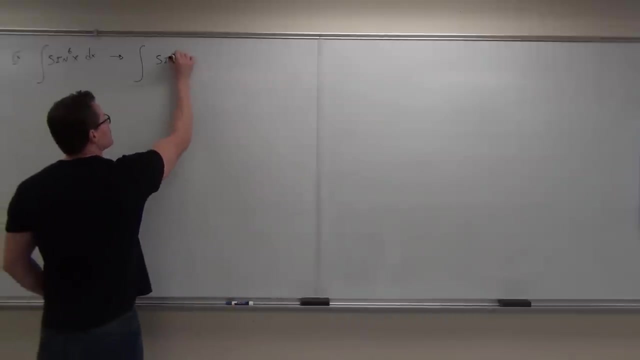 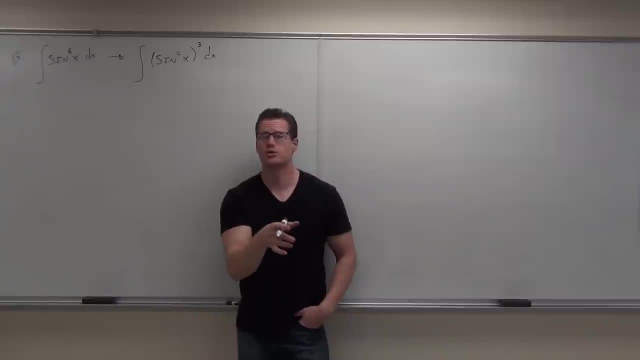 Yeah, Okay, I want to see if you understand the reason why we just did that. What are we trying to use when we have even powers? Even powers only work when you have sine to the second or cosine to the second. but we don't have any cosines. 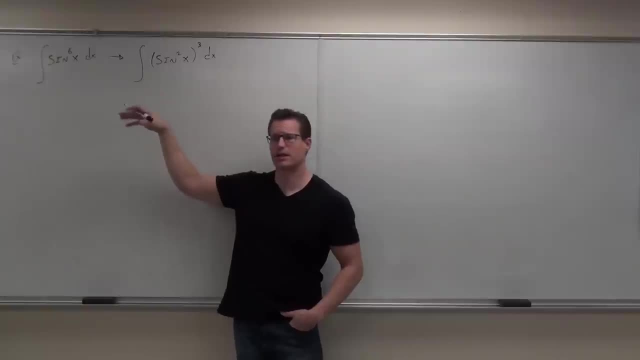 So that's the only thing that's going to work for us is to do sine to the second and then do the third power. Are you guys with me? Yeah, Do the next step. Do the formula here. Yeah, Do it. 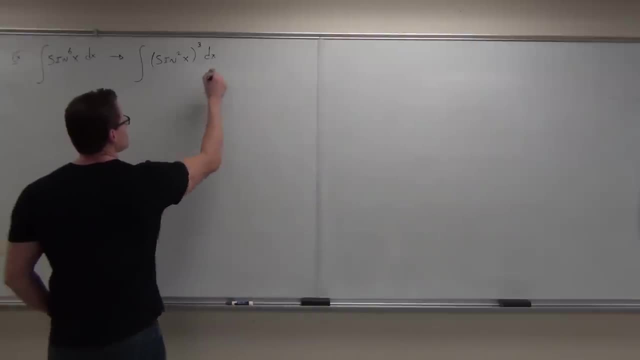 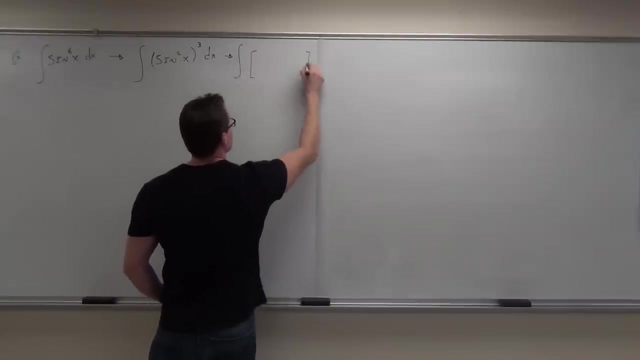 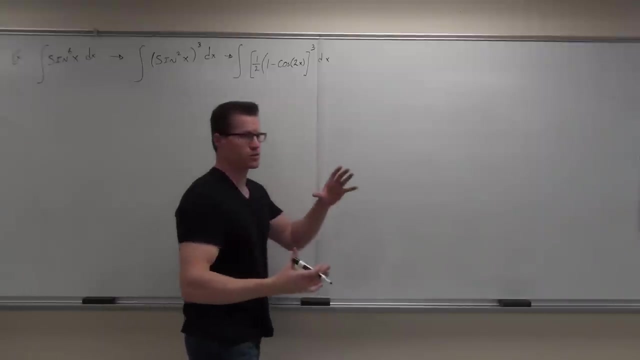 Cosine 2x. Let's see if you all got it. Did you get 1 half times 1 minus cosine 2x, and then all of that raised to the third power with a bracket? Yeah Cool. Next thing you're going to do: 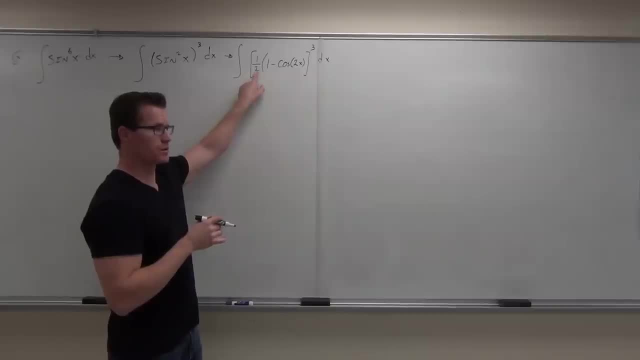 Let's do it. What are you going to do? Distribute that x from it. Yeah, you are. This is going to become how much? 1 eighth. 1 eighth is going to be pulled in front of my integral. You follow. 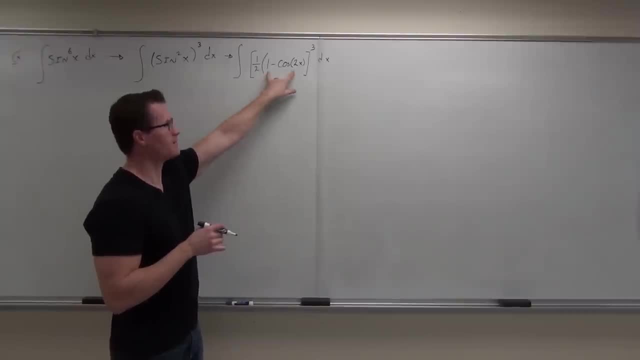 Yeah, Now what do you have to do with this thing? Just keep it that way. Foil x 3.. I know what I forgot Something, Sorry. You're going to have to distribute that, Oh yeah, So if that was to the. 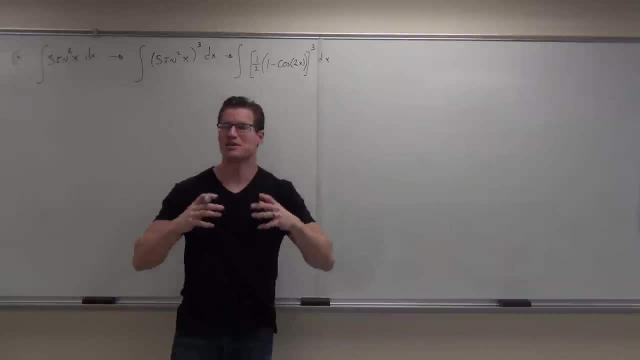 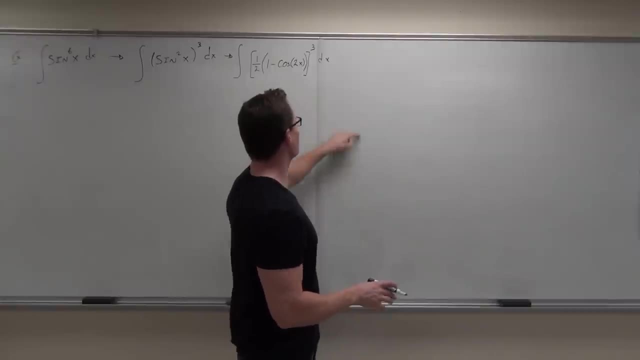 Oh my gosh, If that was to a higher power you'd have to distribute even more. So yeah, You have to. If you're going to do this method without reduction formula, you actually have to distribute that. So on your own, right now, off to the side, do 1 minus cosine 2x times 1 minus cosine 2x. 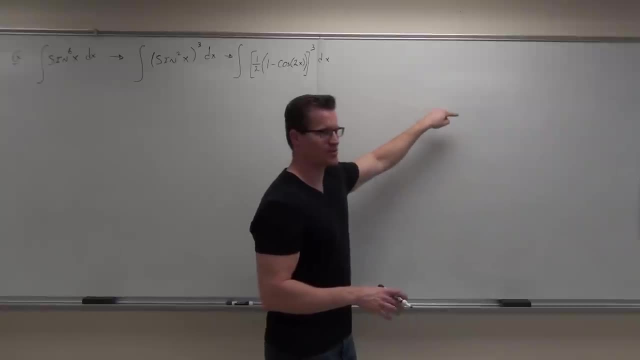 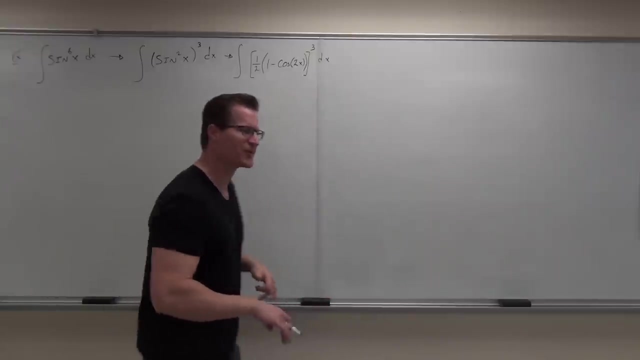 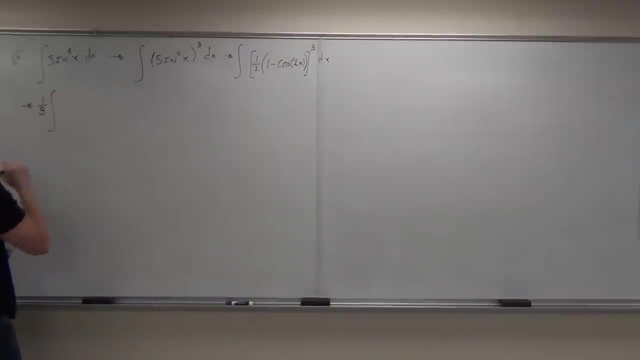 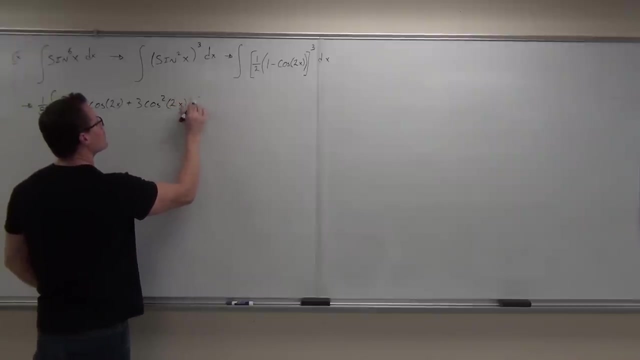 times 1 minus cosine 2.. You're going to have to distribute that. I'll let you do that for about 10 minutes. I'm going to write it on the board here. You're welcome. I think that's right, if you want to check. 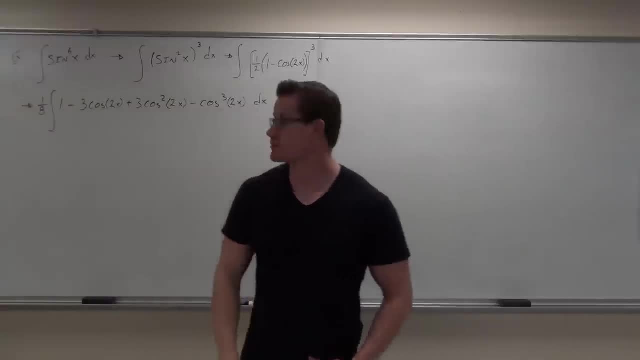 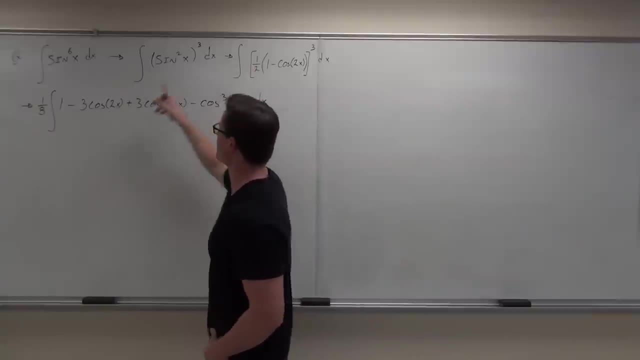 There are easier ways to do binomial expansion. That's one of them. If you know the Pascal's triangle 1, 3,, 3, 1, and you know alternating signs with a minus, plus, minus, and you know powers reduce- sorry, powers gain- 0,, 1,, 2,, 3,, you can distribute. 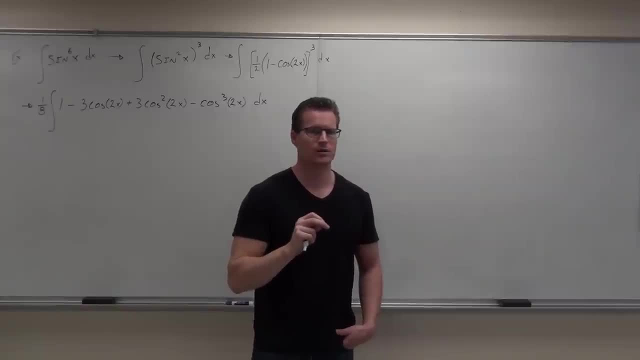 things like that very quickly, Very quickly. So if I did like to do the fourth power, basically it would be the same. it would be 1, 4, 6, 4, 1.. And then you can, if you know the binomial expansion, you can do that. 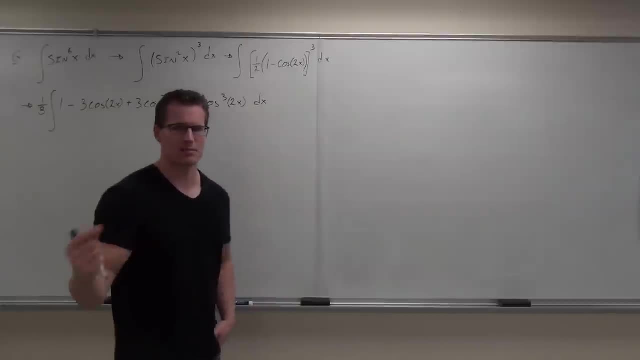 So, anyway, this is what you should have if you distributed it and combined like terms. Did you all get that? Yes, Are you just going to trust me that that's right? Yeah, Probably Okay, that's right, Let's continue. 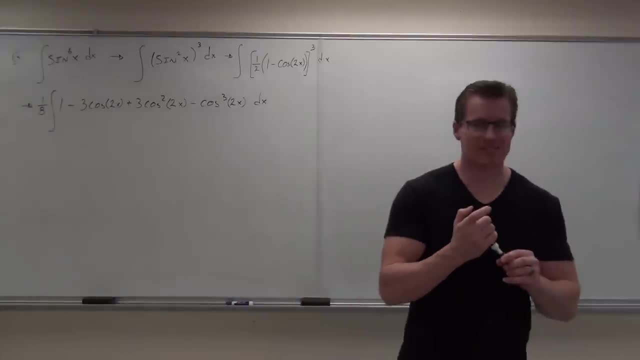 Now, after you distribute, after you do that, you really do have to look at your problem. See what's going on here. folks Check this out. Can you do the integral of this? Yeah, Then you're going to leave that. 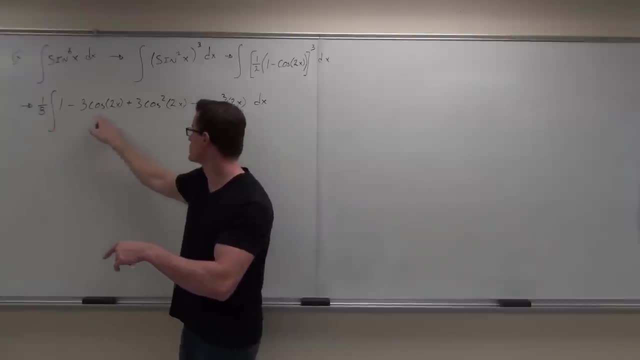 Don't bother changing that. That's a good thing, Remember, you could separate this into 1,, 2,, 3, 4, more integrals We're not going to. We're going to do it in our head, But you could. 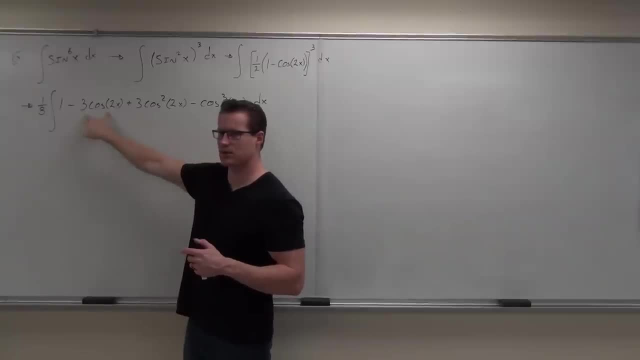 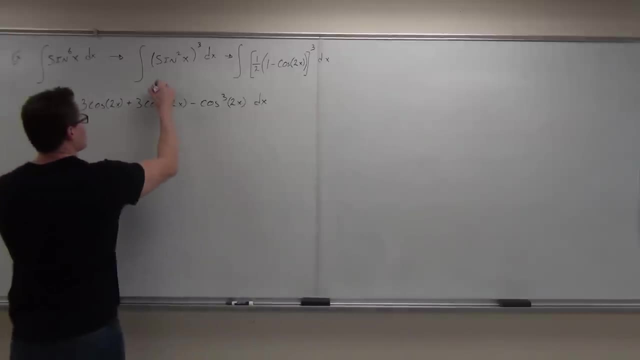 So leave this alone. Leave this alone. Can you take the integral of cosine? No, Yeah, Leave that alone. Can you take the integral of cosine squared? No, So this is something we've got to work on. Okay, let's see if you're paying attention. 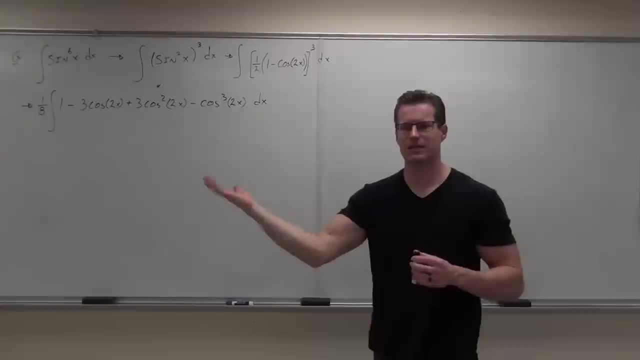 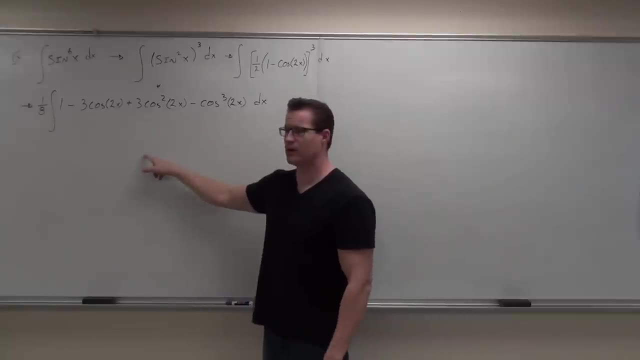 With cosine squared, would I use Pythagorean identity or half angle. Half angle Why? Because it's cosine to the square. Bam, That's exactly right. So this is going to be a half angle right here. Now stop, We're going to do one more thing. 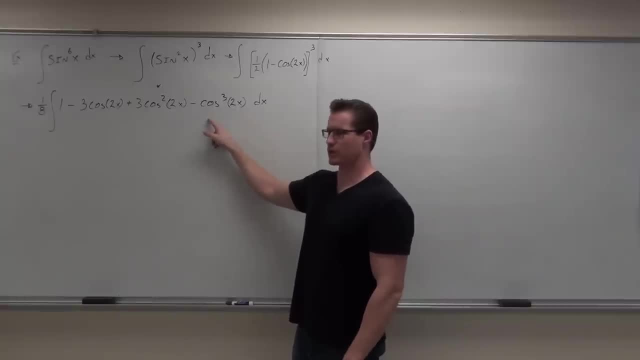 Cosine to the third. Can you do the integral of this right now? No, Change that one too. So this is another one. That's an ugly little star, isn't it? Yeah, Another little star, If you've got cosine to the third, okay. 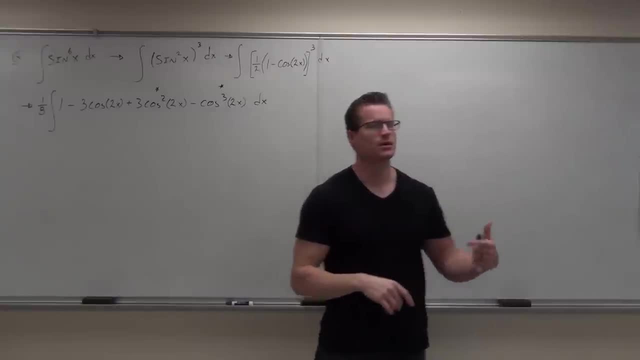 Let's think about this: Are you going to do half angle? Are you going to do Pythagorean identity? Pythagorean identity? Why? Because it's an odd Odd. That's right. That's exactly right. So let's go slow. 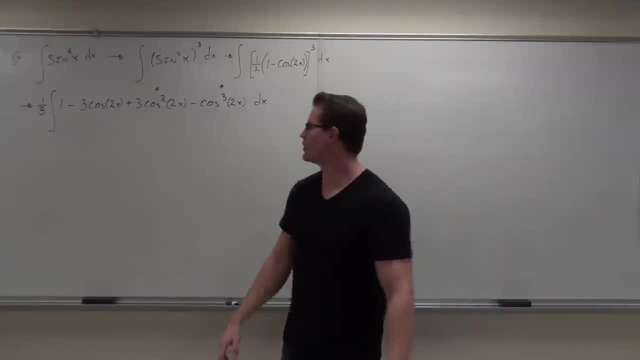 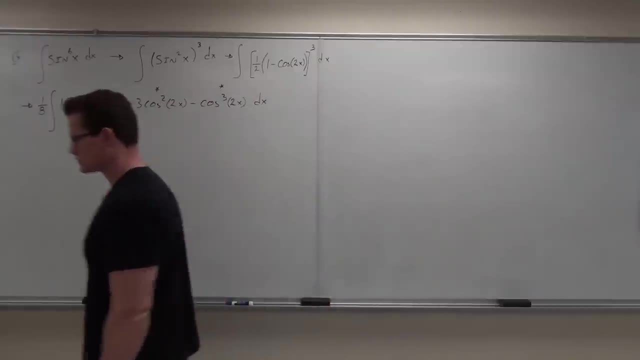 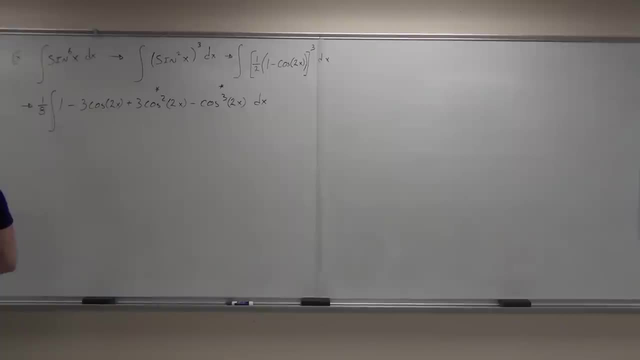 Okay, That's nice. so I know that It's an odd. Okay, So let's do 3.. Texan, Texan, izer, Pass the second. Can we split that? I will count the numbers. Now what did you do? 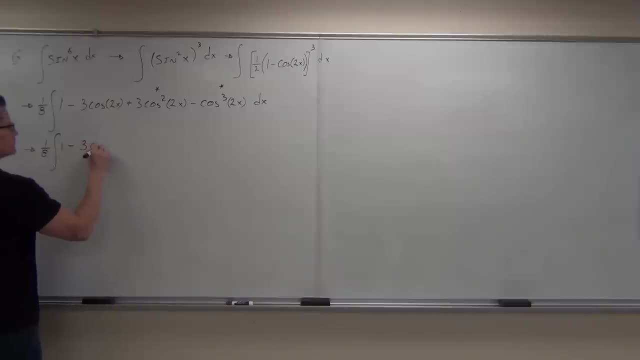 You divided and you got 3.. All right, Let's see. Well, I know, two plus 5 minus, Well, 10.. Oh, come on, You're only going to see it there. Okay, So we need to subtract that away. 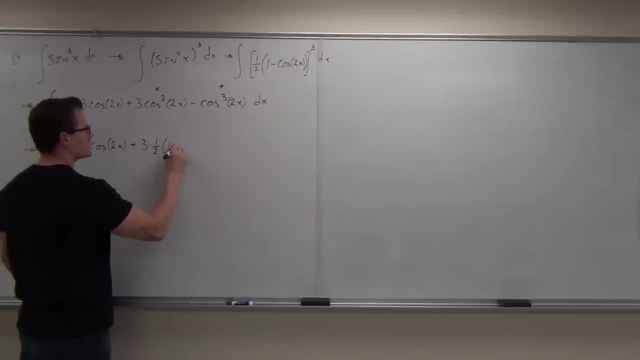 Here we go. Let's see Here: 3 minus 1 plus 3.. Yeah, Let's see. Okay, This is this part right, here is one half one, plus cosine Four x, Brilliant four x. 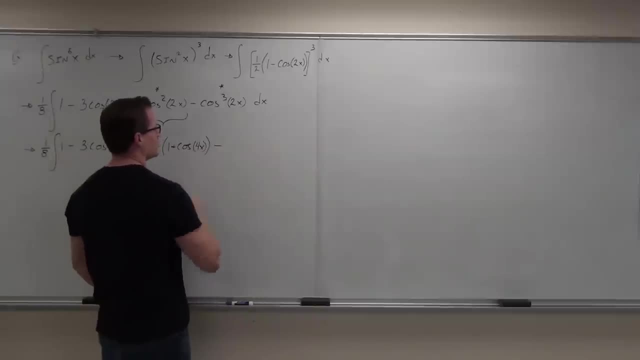 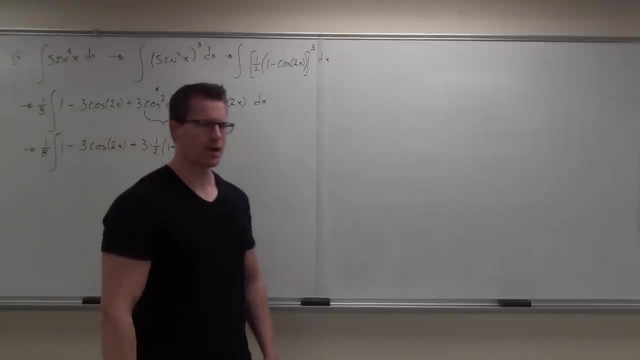 Did y'all get the four x? Yes, Good, Minus. Let's talk about this one now. If I've got cosine cubed of two x, you're right that stands for that's an odd power. So what do we do with odd powers? 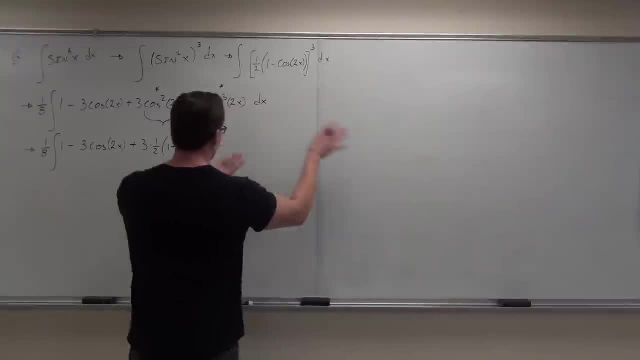 Pull one off. Pull one off. very good, We strip off a. we get the stripper, We get the stripper. Ah, that's right. So we strip one off here. cosine two: x, D x. Oh, look at that. 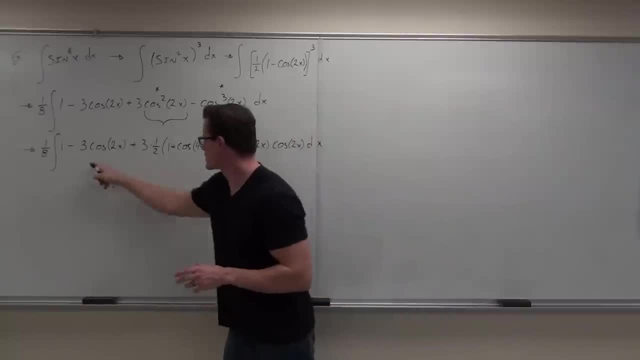 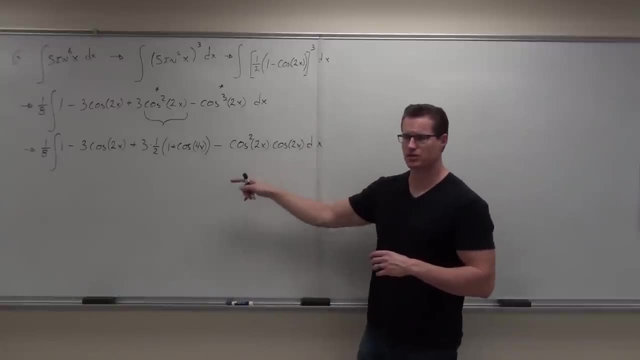 We're gonna do a couple things at once, okay, So don't get lost on me here. I'm gonna leave all this stuff the same. I'm going to distribute this because that's nice, we want to distribute that. I'm also going to start changing this guy. 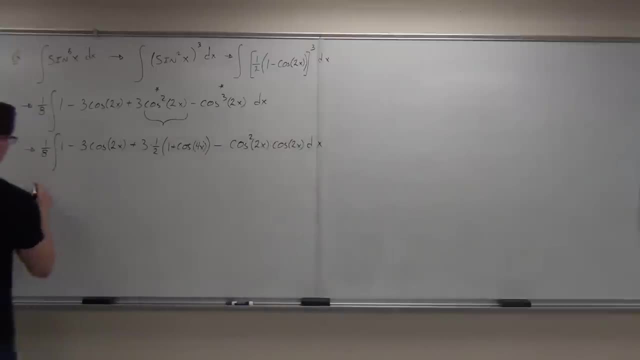 Chopin's feel okay with this. so far, Alright. so we've got a one eighth, We've got an integral, we've got a one, We've got a minus three, We've got a cosine two x. We've got to check this out. 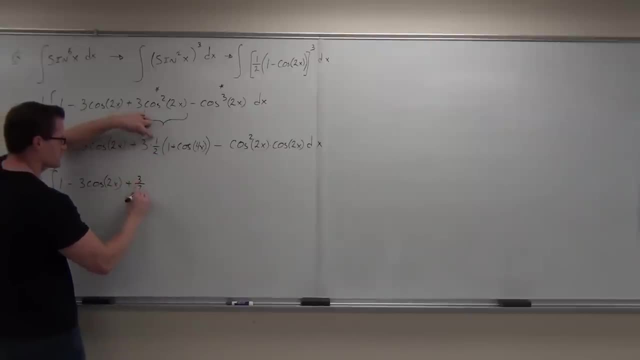 This is three halves times one is three halves. Three halves times cosine four x is three halves cosine four x. So this is exactly the same. All I'm doing is distributing three halves. So we've got those two pieces. Quick head knock drive with that one. 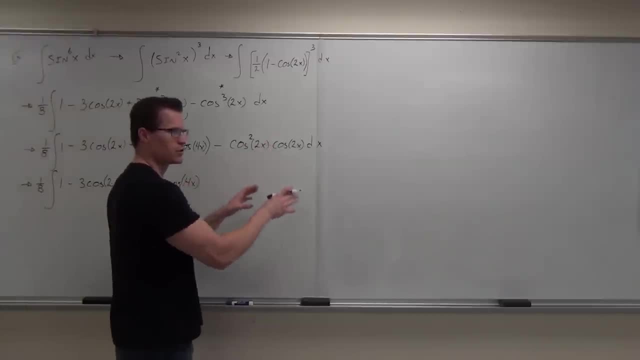 Now, when you're working with this stuff inside of an integral, you can do two things. What does that have to do? You can do this if you want to. You can go wait a minute. this is too confusing for me right now. 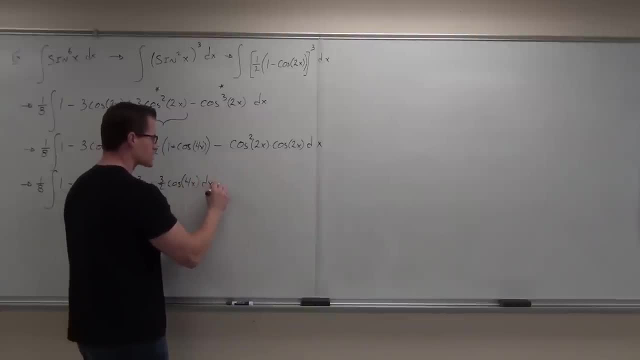 I don't want to deal with this here. You can write a dx and split off another integral. Does that make sense? Do it off to the side. Just don't forget it's a minus. You're going to have to have a bracket. 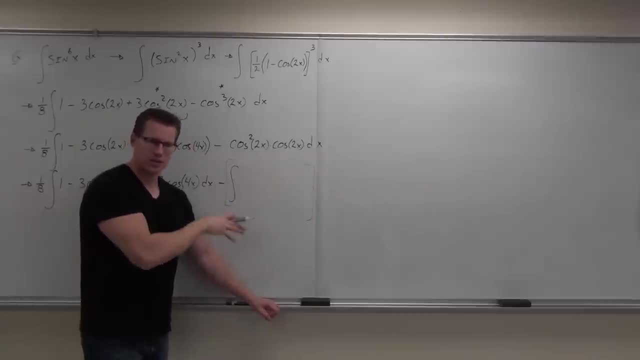 around all the junk that you do right now. Does that make sense to you? Yeah, You can do it in here too and do the substitutions, or distribute and make things a little bit nice for you. That's what I'm going to do. 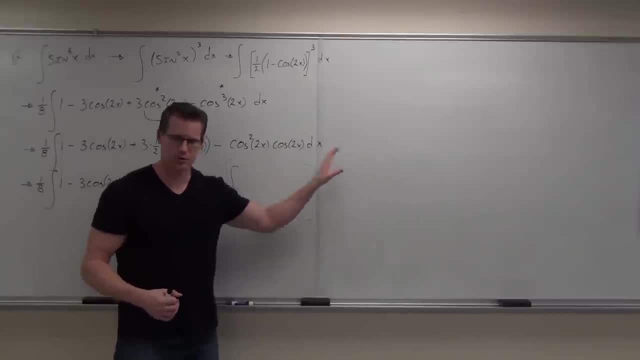 So either you're doing this off to the side, no problem, or you're doing it the way I'm going to show you. You guys, okay with this so far? Yes, Okay, so this is like its own little problem, right here. 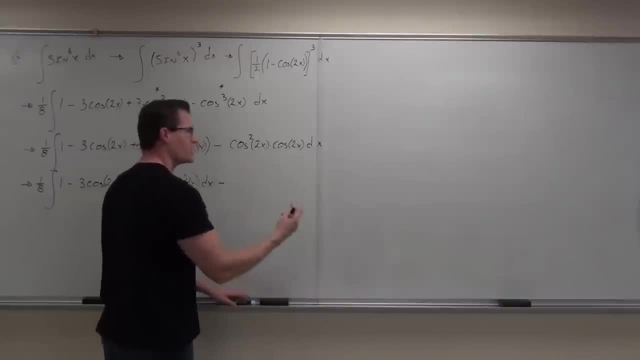 Here's how I would choose to do it. I'd say, okay, well, you know what This right here. this is the same. What are we doing here? Are we doing half angle or Pythagorean Half angle? Because it's connected with this, you do half angle. 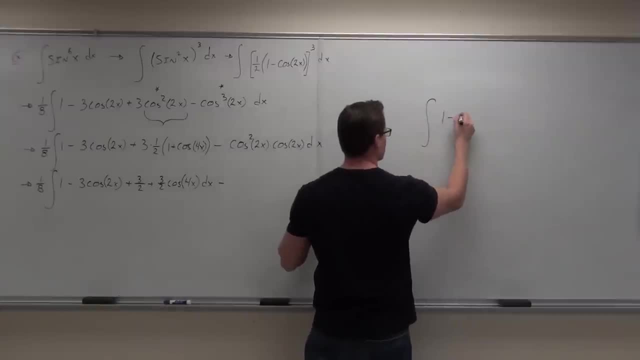 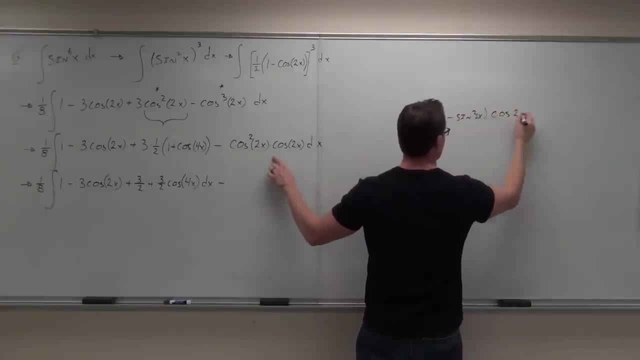 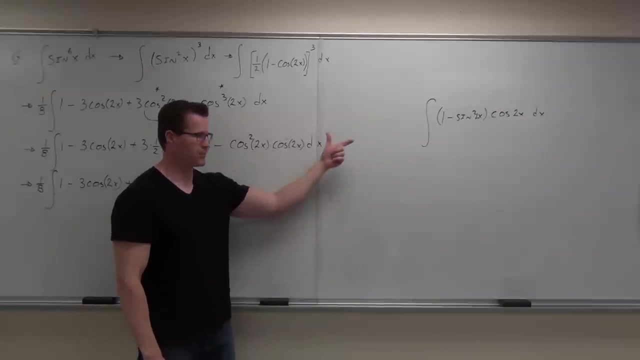 So again, you would have this integral. so Pythagorean Off to the side. if you chose to do it, This would become 1 minus sine squared. You want Pythagorean, not half angle. That is cosine 2x. 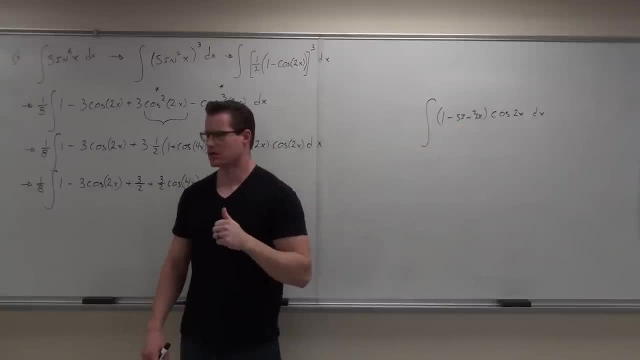 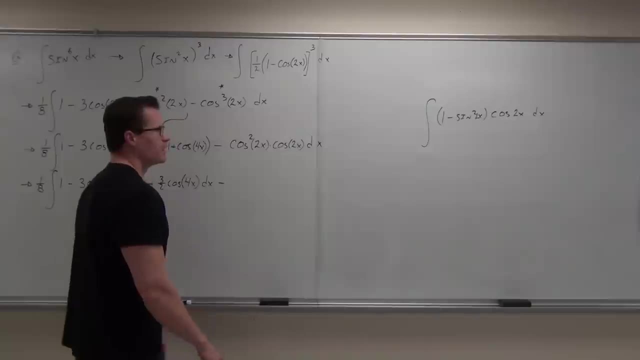 That's supposed to be a little 2 there, And then you do a simple substitution and you're practically done with that. You guys? okay with that one? Okay, maybe I'll do both, just so you see that it works out the same. 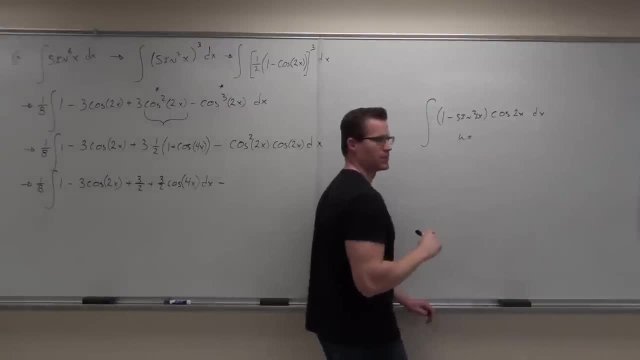 Over here. what would your? u become? U cosine sine Cosine or sine Sine Sine? It's usually inside of something Sine. of what Cosine Du? Those people who hate to do the chain rule? don't mess this up. 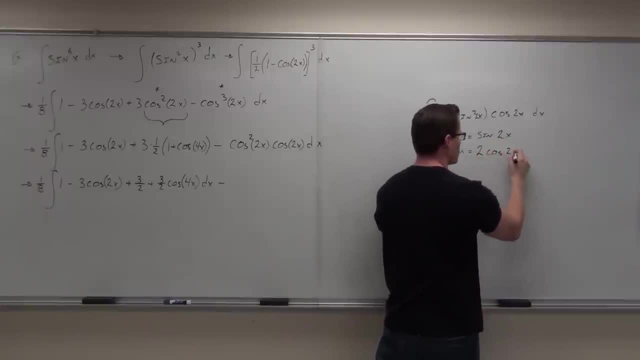 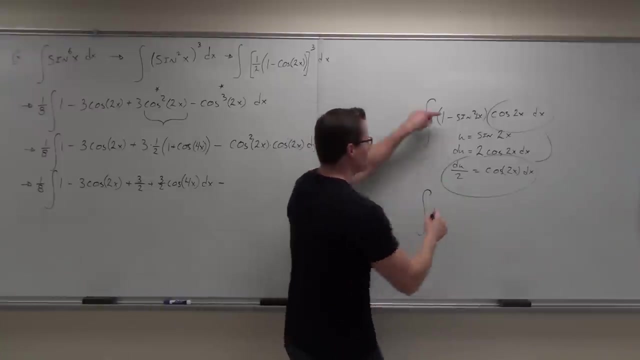 What's this going to become? 2 sine over 2x Or du over 2 equals cosine 2x dx. exactly what we have here. I know I'm working quickly, but we've already done something very similar to this. 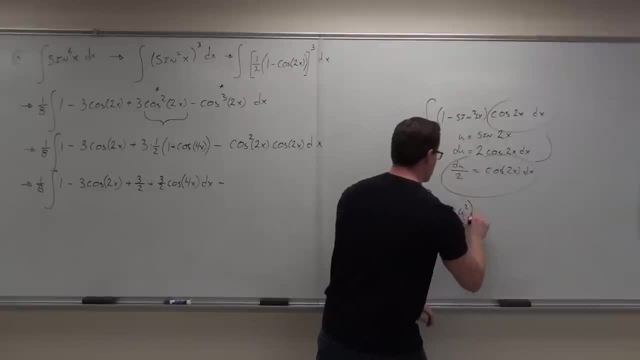 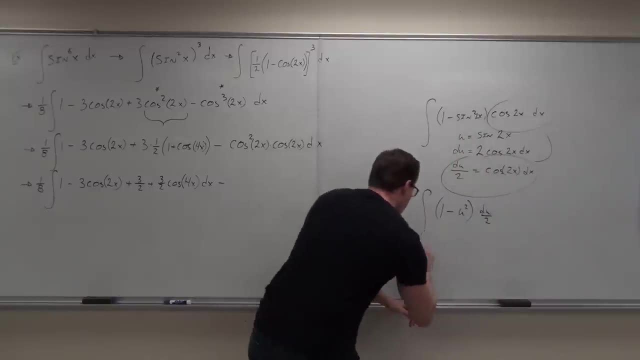 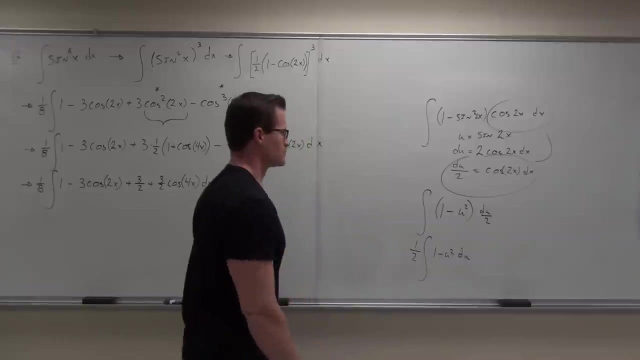 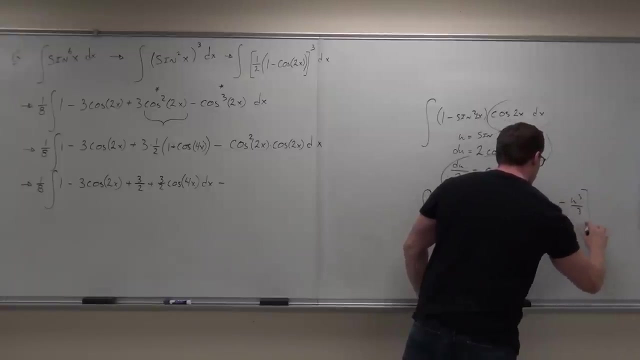 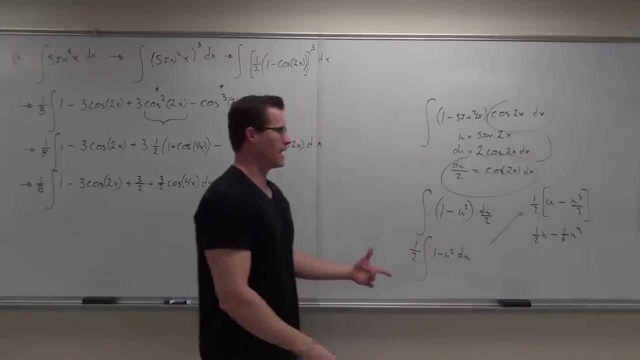 This is 1. Minus U squared, This guy is du over 2.. Or in other words, this is 1 half integral of 1 minus u squared du 1 half u minus uq over 3.. 1 half u minus 1 sixth uq. 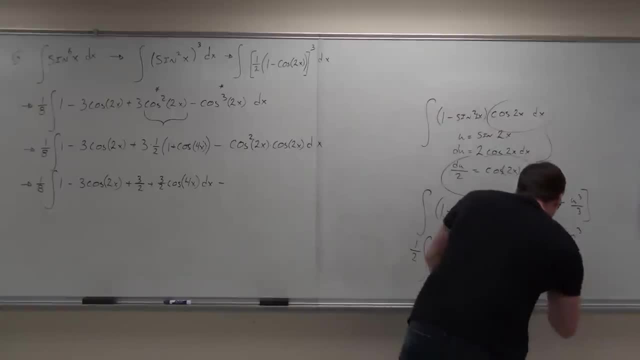 And lastly, we do our substitution back in. We'd add 1, half. what is it? what was our substitution anyway? Minus 1, sixth, sine q, 2x. Okay, I know I did it fast, but I want to know how many people could do this on their own. 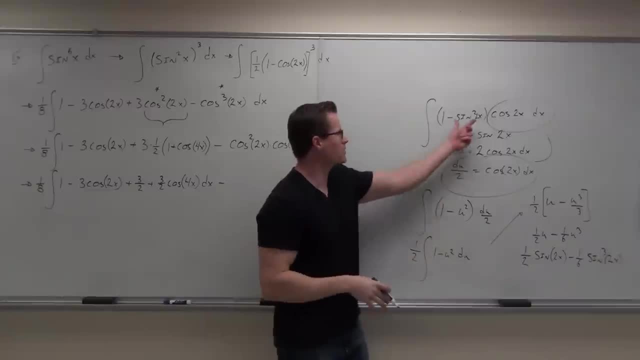 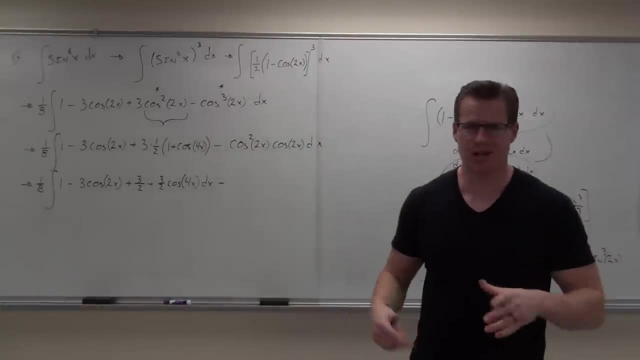 at this point It should be pretty much all of you, Because we all know how to do a substitution. This was the only big thing is seeing just really, have you noticed how the hard part about this is seeing what to do? 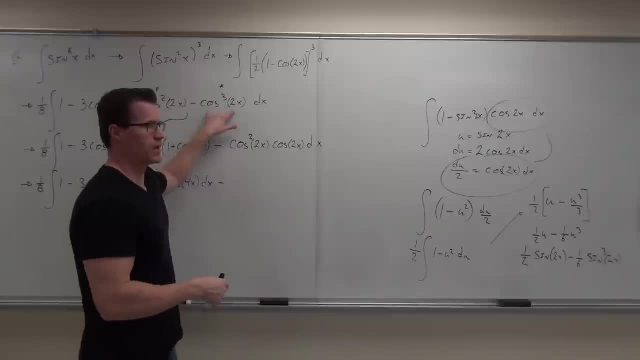 It's not actually doing it. It's going: oh wait, I've got a cosine q. Is that half angle, or is that Pythagorean? It's odd, so it's Pythagorean. This was even. therefore, it's half angle. 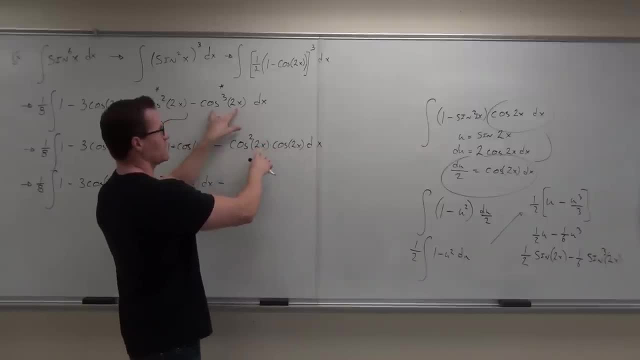 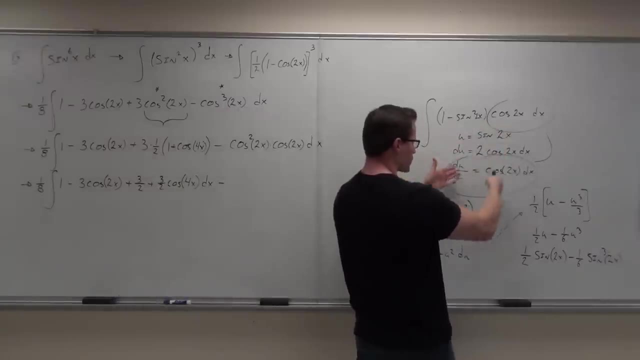 So well, separate it so that you can do Pythagorean. So q, no, no, no, no. Strip it off. we've got Pythagorean, we've got that Pythagorean identity. do a little substitution. It works out pretty nicely. 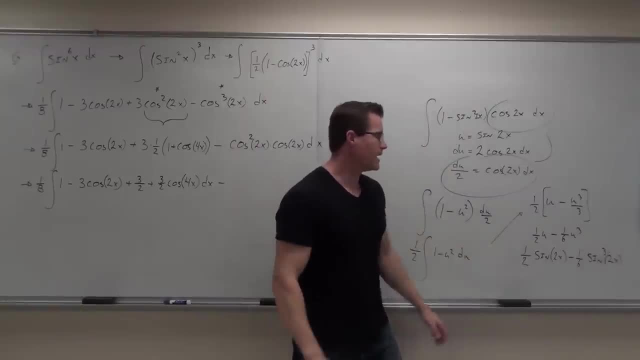 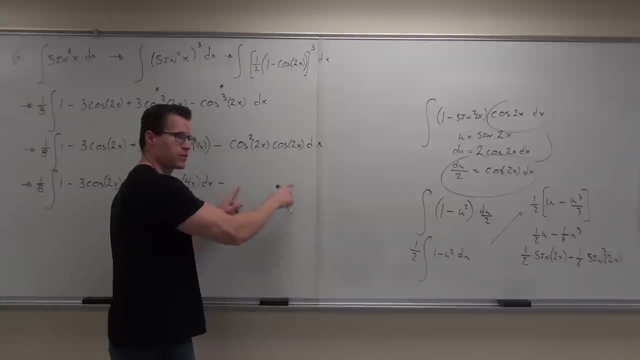 Show of hands. if you have the same thing on your own and you're okay with that one, Cool. Now notice something: This integral is done, So this is what you plug back in right here when you're done with the integral. 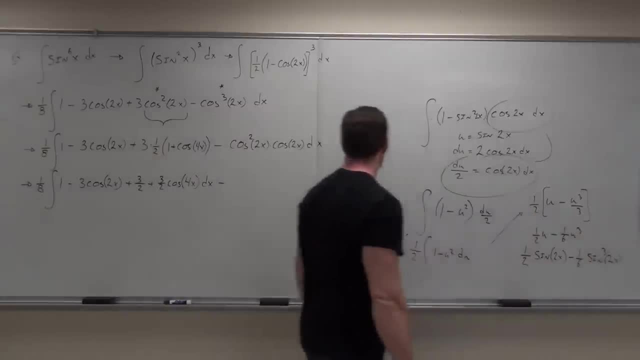 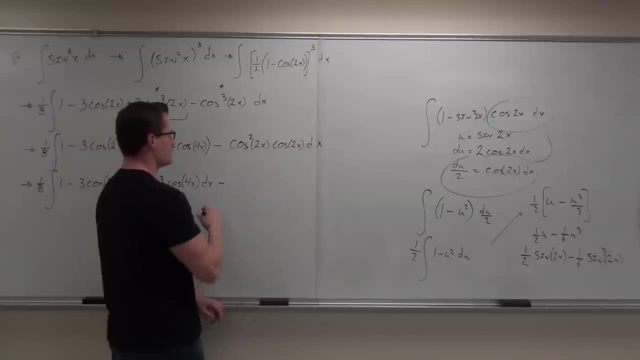 Does that make sense? Yeah, It'd be minus this whole mess of crap. Now, if you do it the other way, I don't even know if I want to show you the other way, now that we've already done it. it's going to take some time. 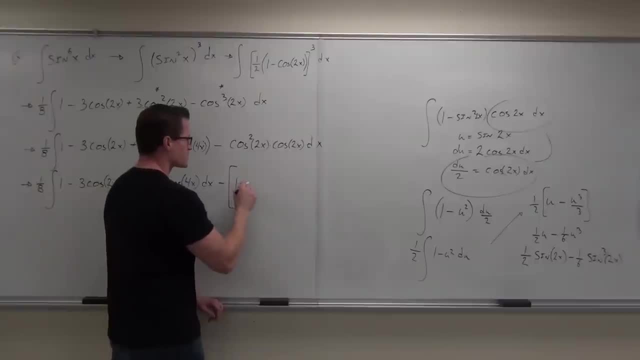 If you do it the other way- basically just put a bracket here- you do the same thing sine squared: 2x, Cosine 2x dx. You would distribute it, so you would have a cosine 2x here. 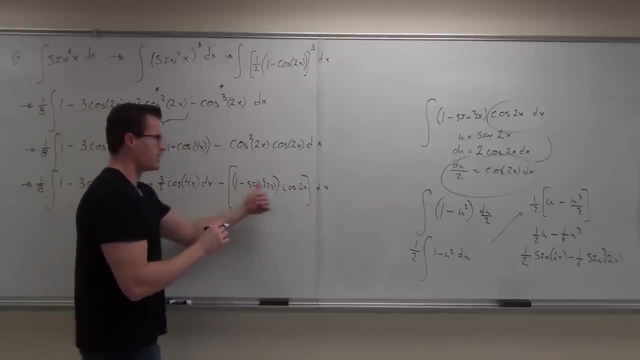 I would probably combine that cosine 2x somewhere over here, and then you'd have the same substitution that you just did. Does that make sense to you? Yeah, So you do it one or the other way. I'm going to leave that. 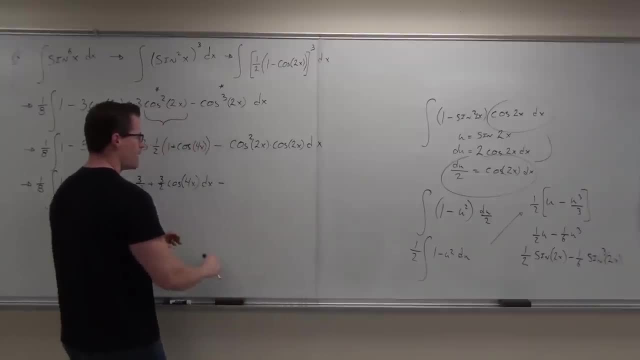 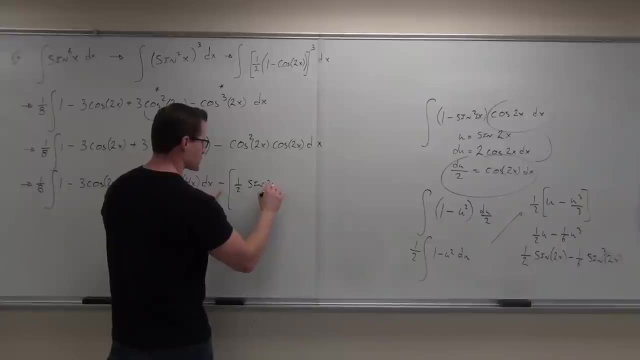 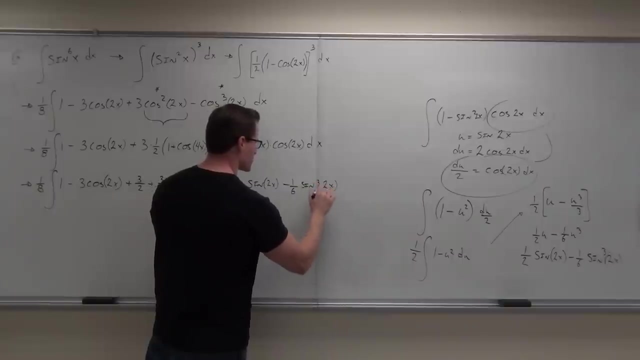 So I like that way, I like doing it off to the side. So this is going to be minus this stuff 1 half 1 half sine 2x, minus 1 sixth sine cubed 2x. 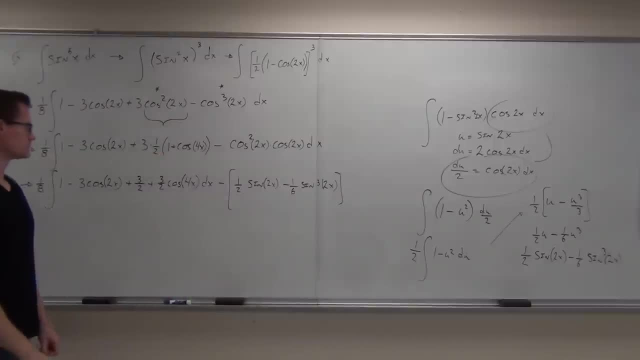 I'll put the plus c on the very end of my problem. I don't need to deal with it right now. Okay, so I don't want to lose you, I don't want to lose anybody, so let's check it out. 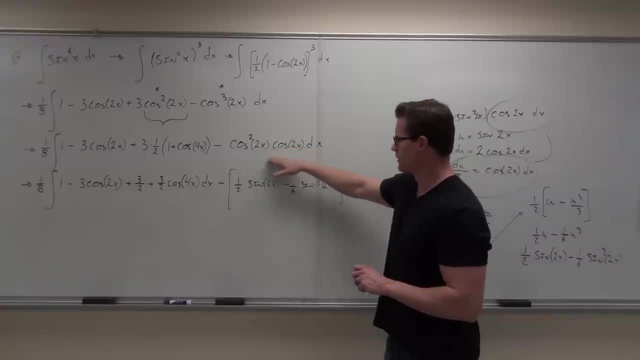 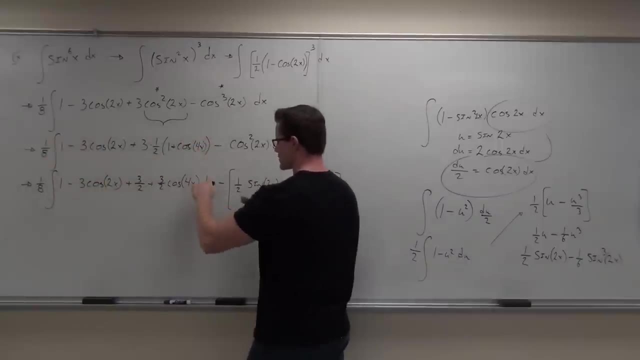 You guys are okay down to here, correct This one. we said no, no, no, Let's separate this. Let's call this one big fat integral. That's why we get the dx right here where there wasn't one before. 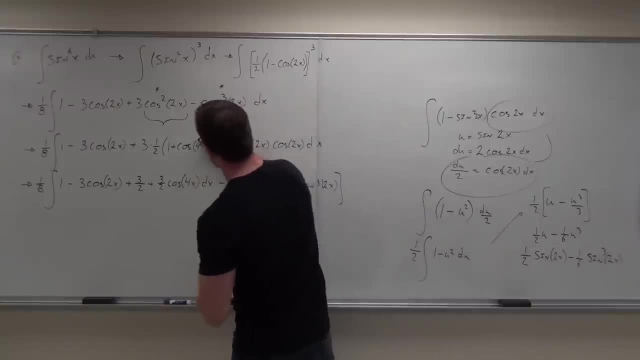 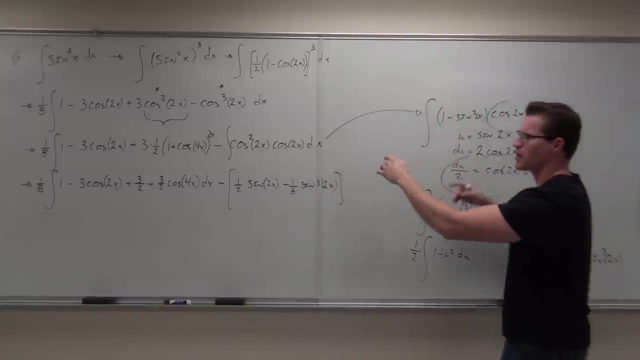 Then we're subtracting the integral of this guy. So we said: now let's make this a dx and we'll have the integral of this. So we move that over here, we do it off to the side. It's a problem within a problem. 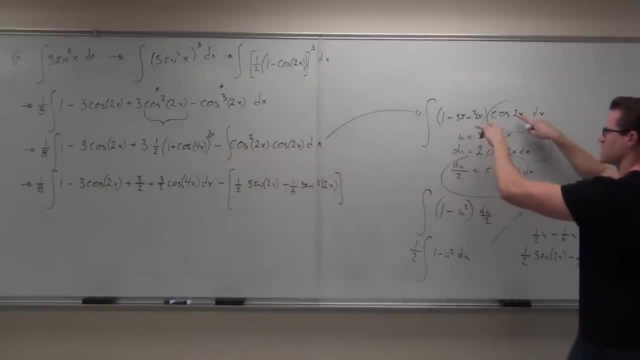 So 1 minus sine squared, 2x times cosine 2x. Do the integral, then put it right back. We get the same thing. So are we going to integrate this right here? No, Are we going to integrate this right now. 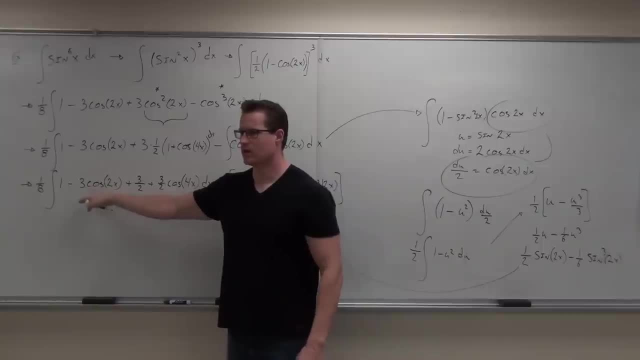 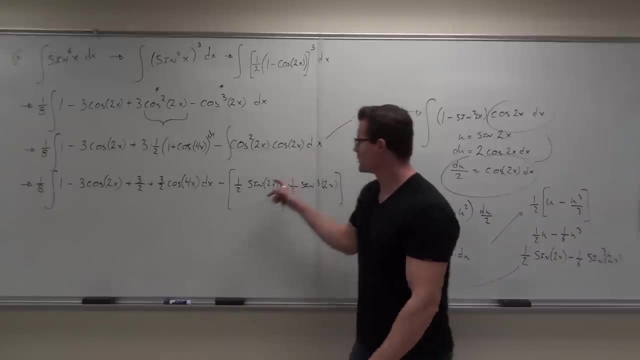 No, Heck no. Are we going to integrate this stuff right now? Yes, Of course we are. What might you want to do before you start integrating that? Combine the like terms. Combine the like terms. Yeah, that's right. And, in fact, if you would have done this the other way that I was about to show you, you. 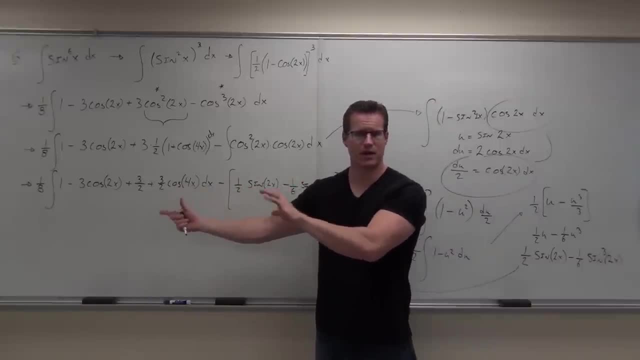 would have some more like terms to combine, so you'd have less terms. It's whether you want to combine them now or combine them later. We're going to do it at some point. What like terms do we have? Three hat, Three hat. 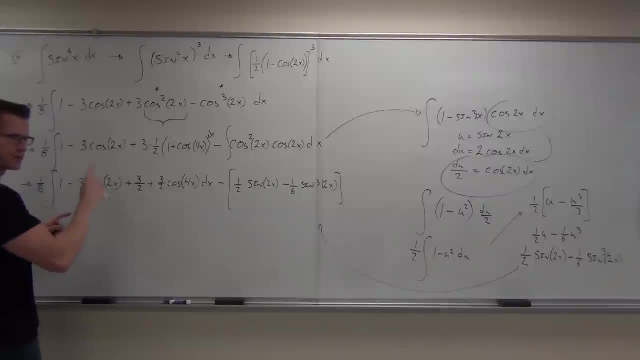 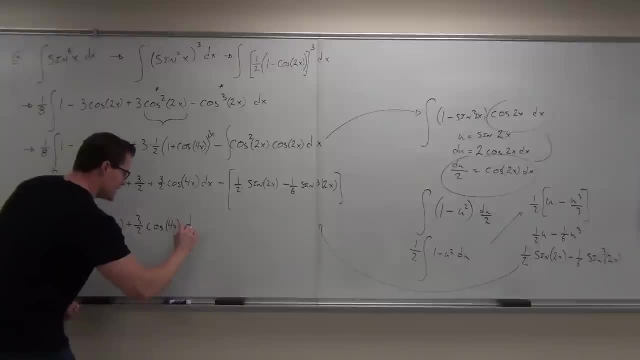 cosine four x, Notice dx. calculus ends here. This we've already done. Distribute: Yeah, you can do that. You can distribute that right now, if you wanted to. You want to do that. Yeah, You want to do that. 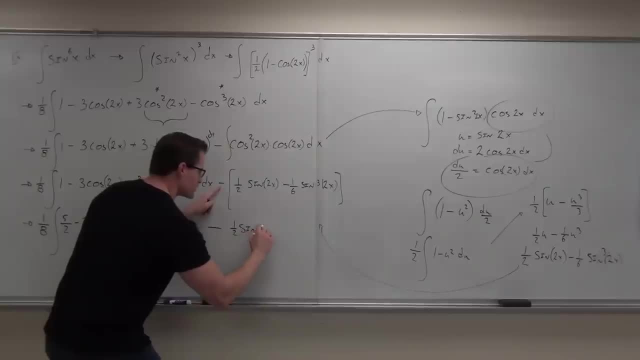 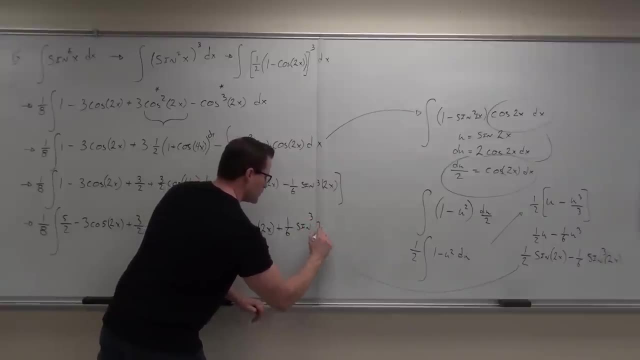 No, You're going to do that. Yeah, So minus one half sine two x, Plus one sixth, Good, plus one sixth sine two third power: Two x, Two x. Now let's work on the integral of this thing- Almost done. 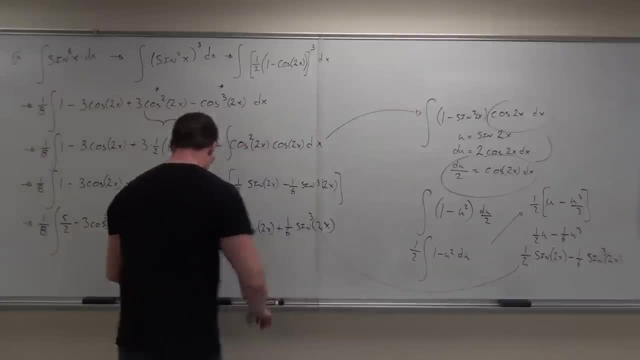 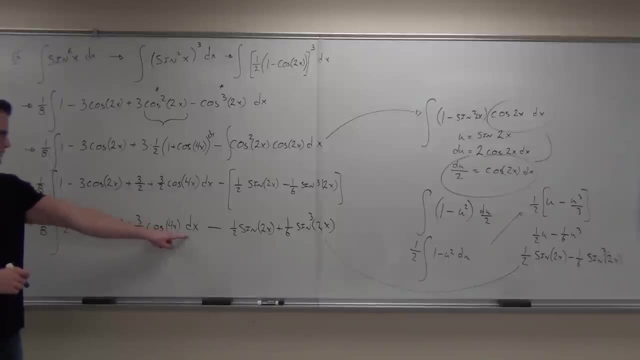 Wow, You're forgetting the dx on both of those. What dx? The whole integral, The extractor x. For the other one, The last extractor, There's a hit. It's already an integral. Yeah, There's a head, There's a head. 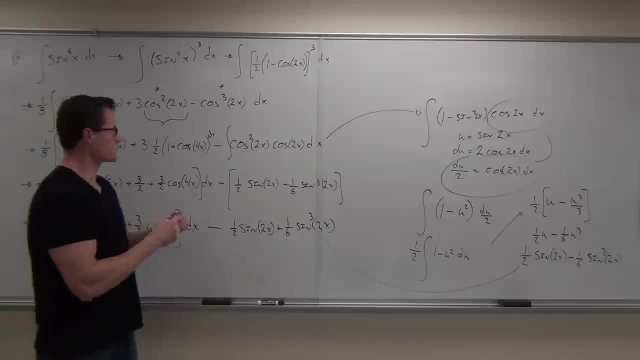 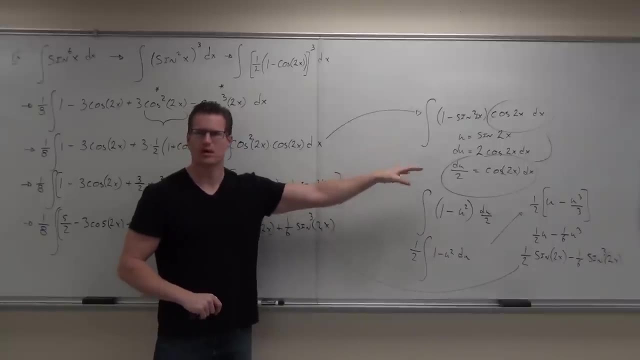 Oh, you split it. That was kind of the whole idea was right: here we split this and we did this integral separately, that way we could use substitution And go: yeah, yeah, you know what, let's do this separate. 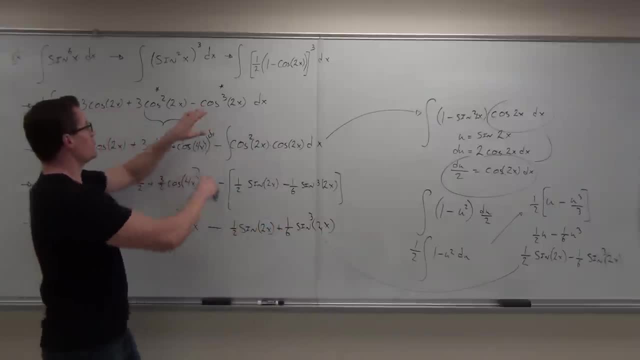 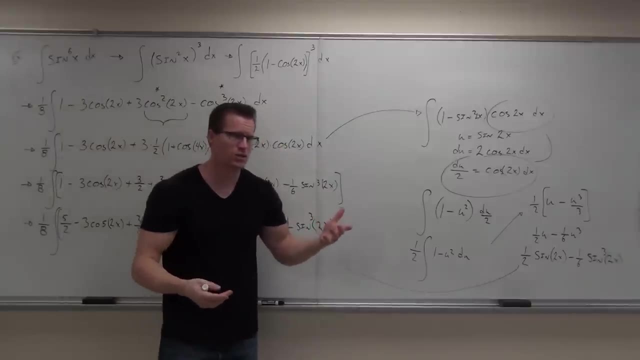 We have it back in terms of x. Now we can put it back. So this was all one integral, This one. I said no, this is too hard for me to do right here, or you can- You actually could, not a big deal. 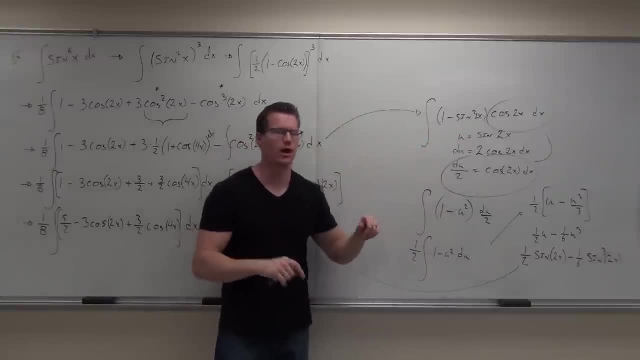 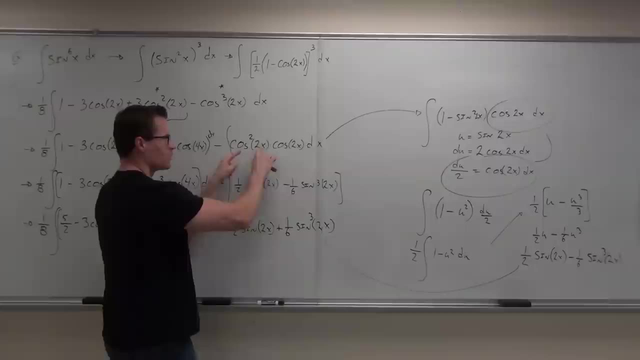 Or you could do it separately. I just wanted to give you that option. So either way- and I don't care how You pull that off- make sure you get all the way done. then you plug it back here. but notice we've already done the integral. 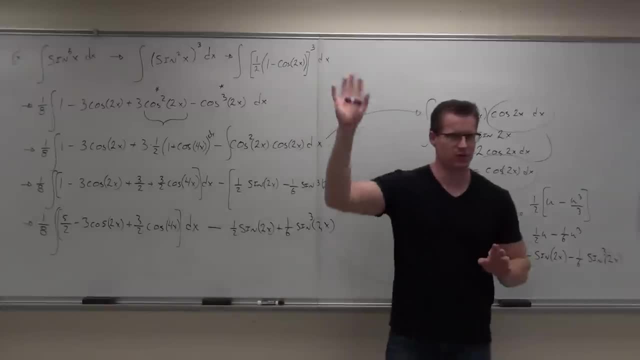 There is no more integration to do here. I really do need you to understand that Show of hands. if you do, you feel okay with that Question. Someone looked like they had one Question, You sure? Okay, Okay, almost done. 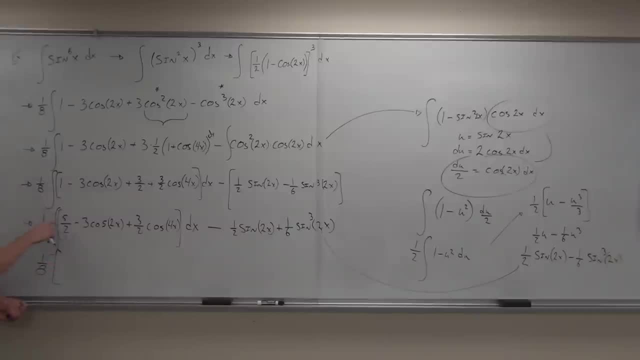 So one eighth times some nasty stuff. Let's do this integral. Can you do the integral of five halves? Yeah, What is it? Five half x Minus. be very careful with these guys. This is gonna be minus three. integral of cosine two x. 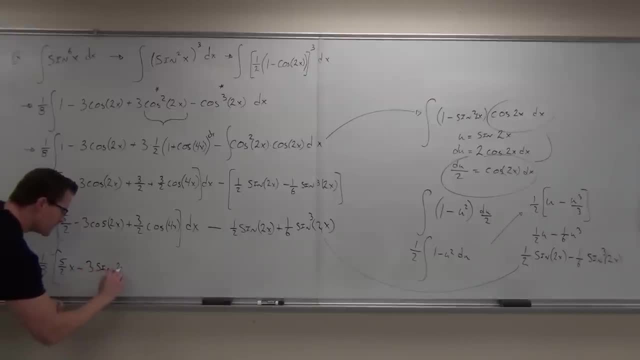 please Sine of two x times two. No, it's not times two Divided by two. Divided by two, When you're doing integrals, you're dividing by this derivative because you're setting this equal to u derivative of this equals du. 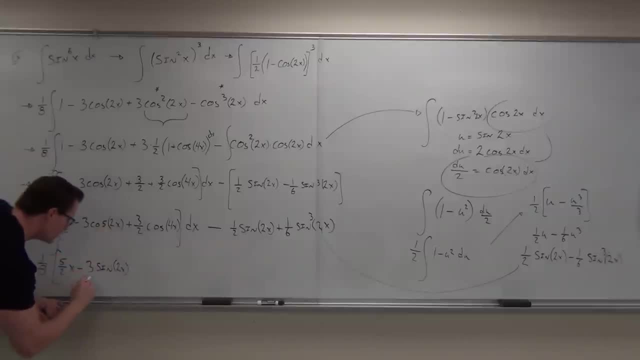 so dx would equal du over the two Plus three halves. Let's try this again, okay. Derivative of this one, Sine of four, Sine of two, Perfect Again. you're kind of doing those substitutions in your head. 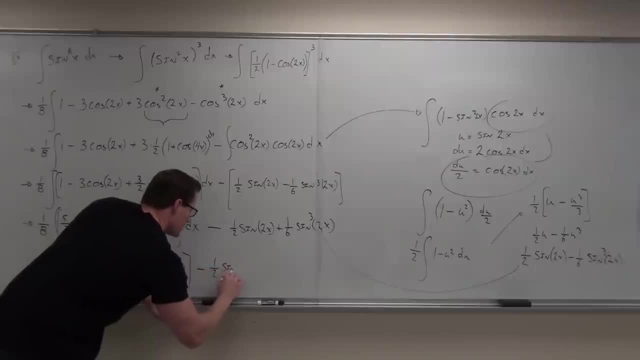 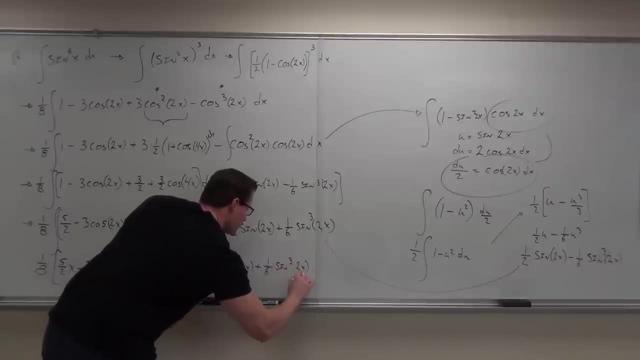 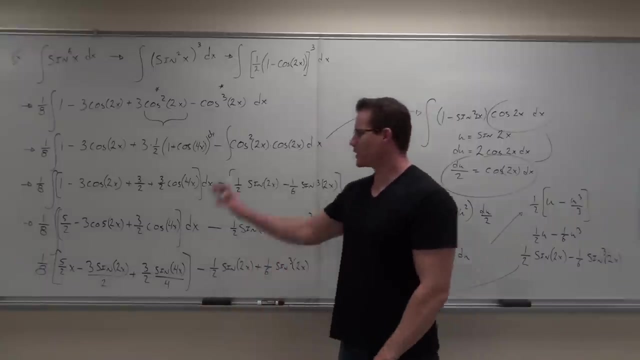 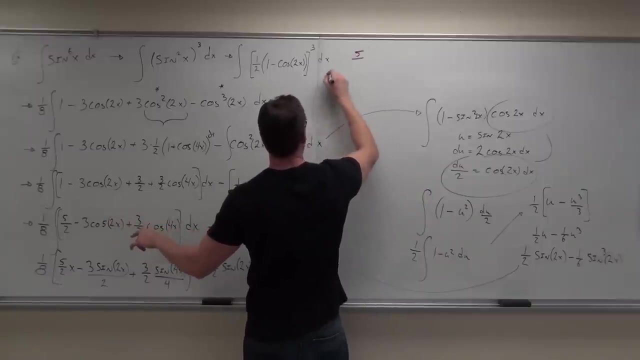 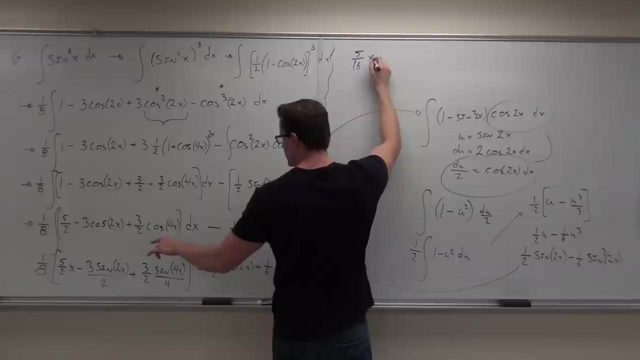 Minus all this stuff. Oh dear, It's fun, right A little bit. What now? Distribute to one eighth And combine that, So working from the very bottom, Five sixteenths x, Oh goodness, minus three sixteenths. 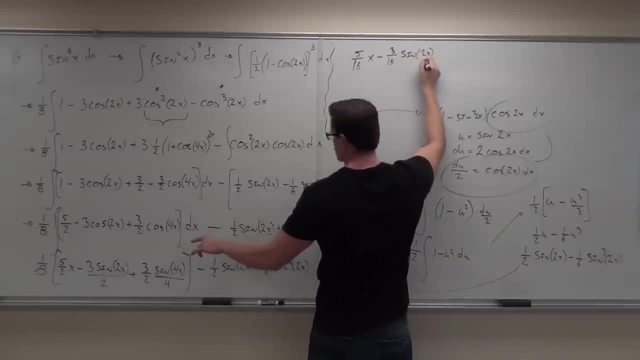 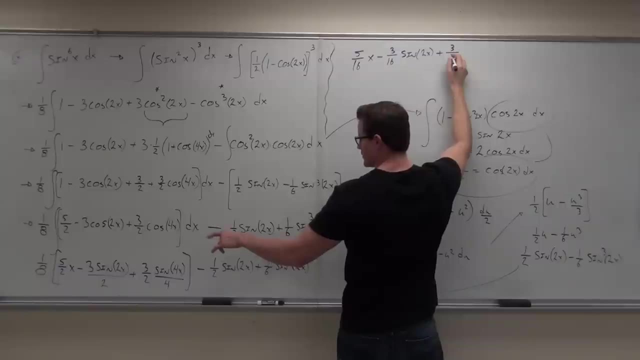 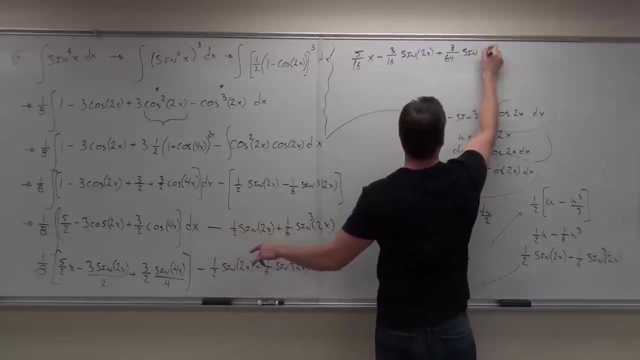 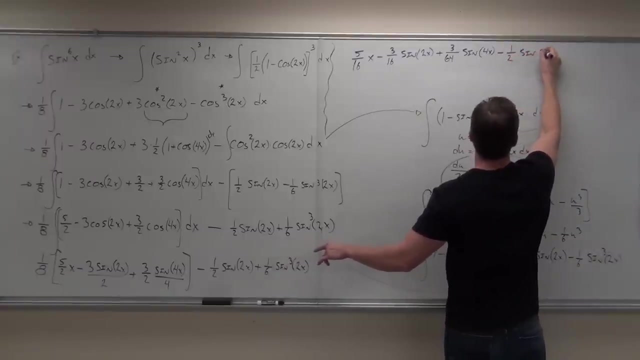 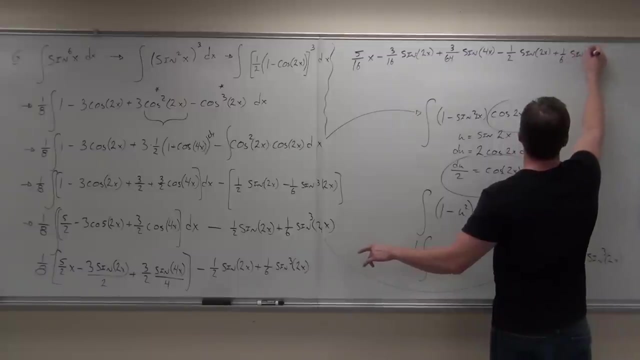 Sine two: Sine two x, I know right Three. Three. Sine four x Minus one half. Sine two x Plus one. sixth. Sine Q: Two x. Oh goodness, alright, Well, almost done. 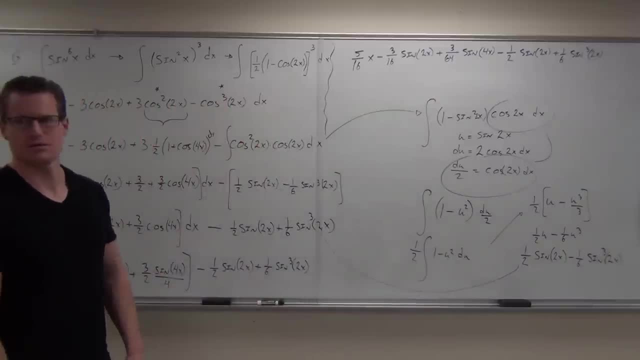 Listen, the last thing that we're going to do. Wouldn't you have to distribute the one-eighth on both sides? We did No, no, It also goes here. Yeah, you're right. This is a big bracket. Yeah, you're right. 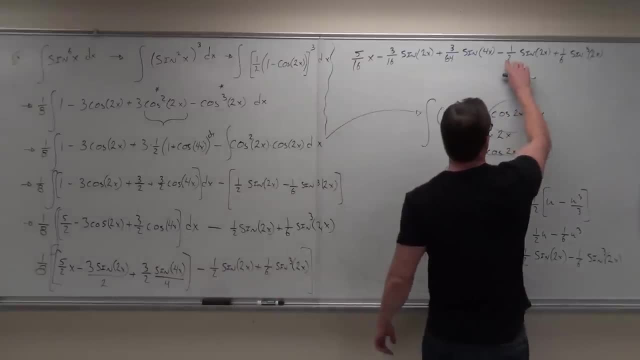 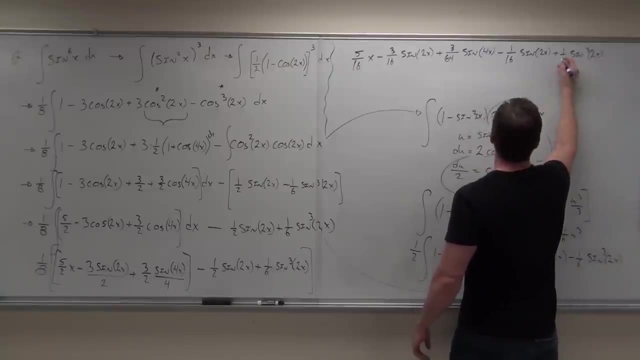 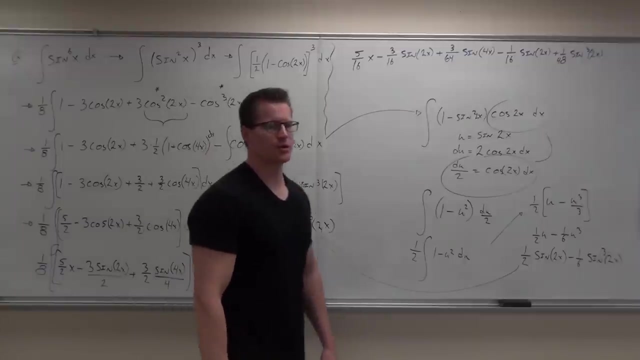 You're absolutely right. So if I distribute that, what's this change to 16 and 42. How much 41.. So one more thing we've got to do. We're looking for any like terms. So like terms. do you see any? 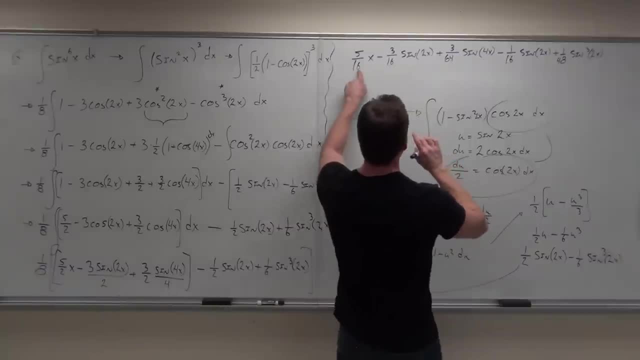 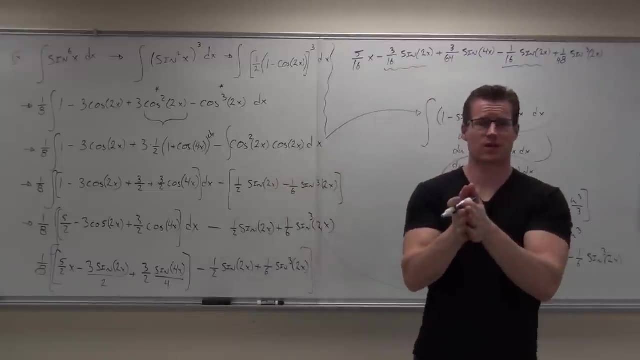 The sine 2x: yeah. This one, no, This one, yes. These two are like terms And, thankfully, because Patrick taught this, we distributed that and they have a common denominator right now, which is really nice. So we're going to have – I was just testing you, Patrick. 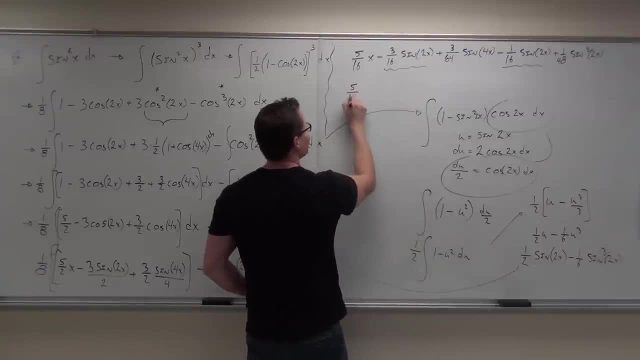 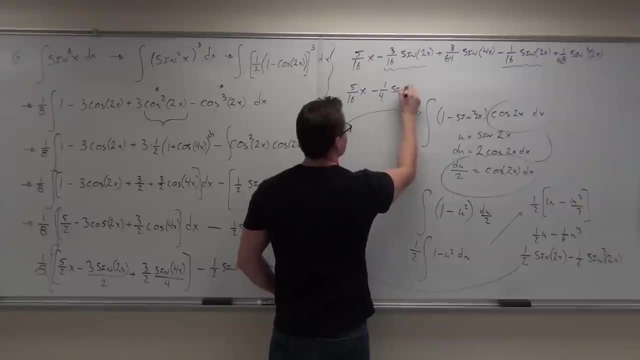 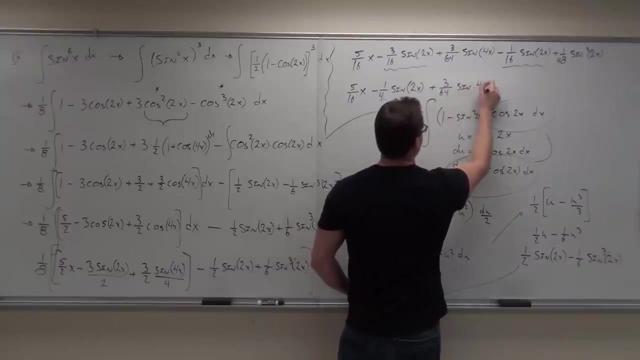 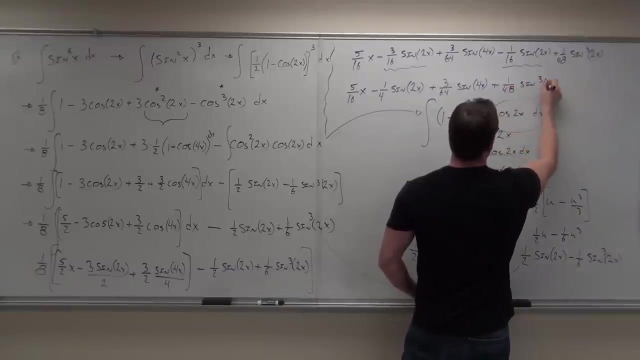 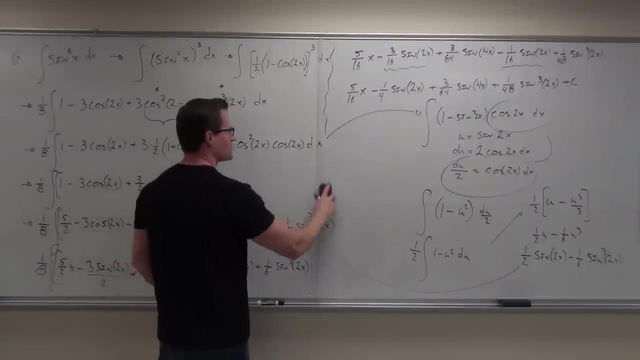 You passed Five-sixteenths. Five-sixteenths, How much is that going to be Four-sixteenths? And lastly, Plus C. Okay, I want to show you one more thing with this, If you didn't do the integral. 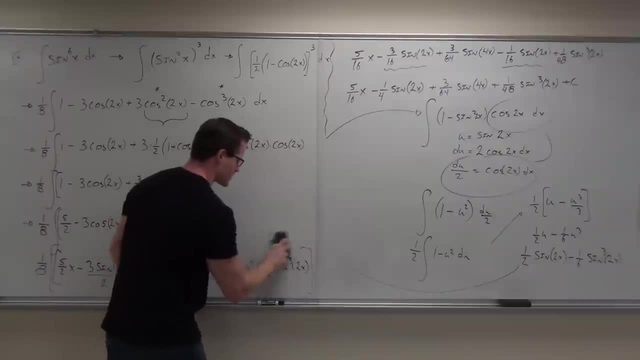 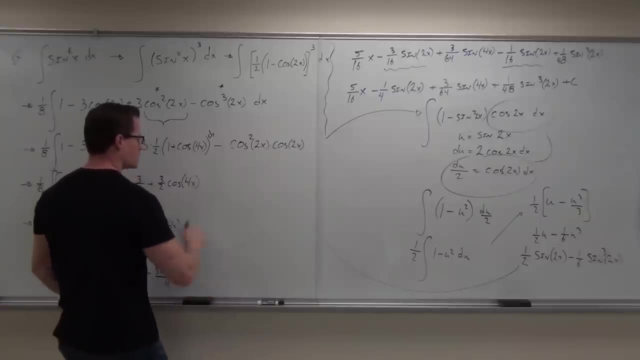 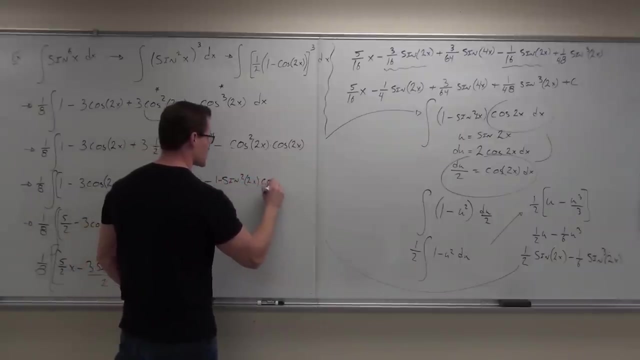 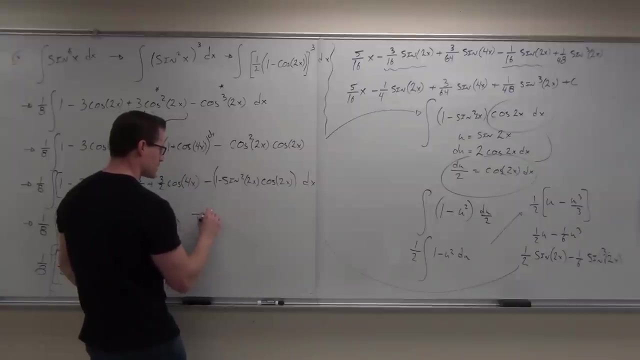 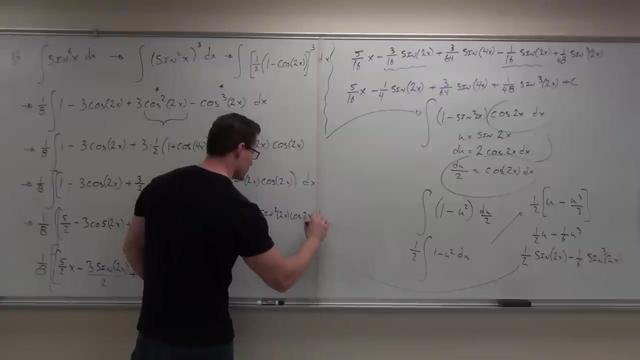 So I do want to prove to you that it does come out the same. So imagine you didn't do this right here. What you'd have is 1 minus sine squared 2x times cosine 2x all dx. You'd have a minus cosine 2x plus sine squared 2x cosine 2x dx. 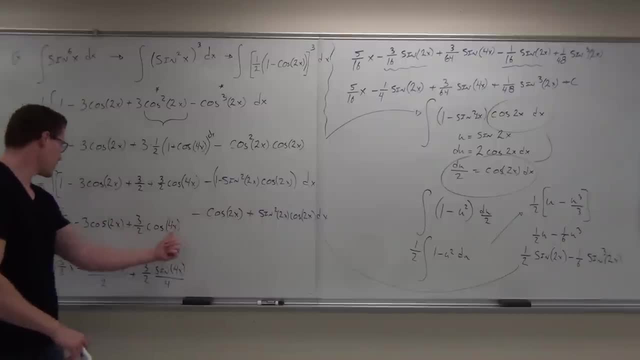 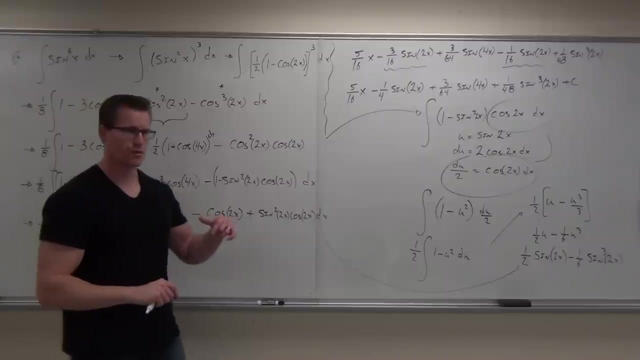 You would distribute this thing. This is what you would combine with this thing. It would be minus 4.. So when you look at that, this would become minus 4.. Minus 4 cosine 2x: If you do the integral of the minus 4 cosine 2x, you'd get minus 4 sine 2x over 2.. 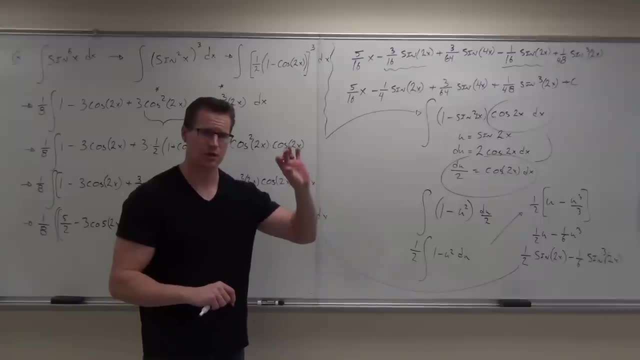 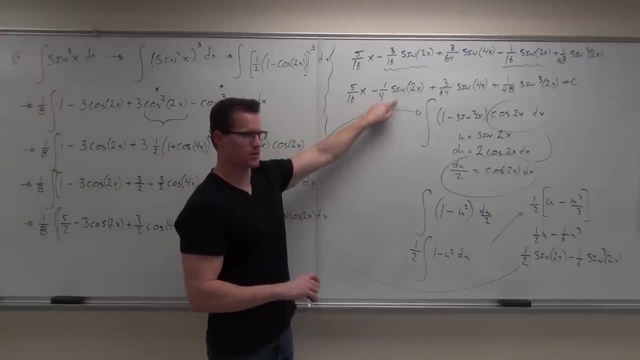 Correct, That would be the 2. You'd get 2 sine 2x. When you multiply by 1 eighth, you'd get the 1 fourth right there. Does that make sense to you? It matches. The coefficients are going to match. 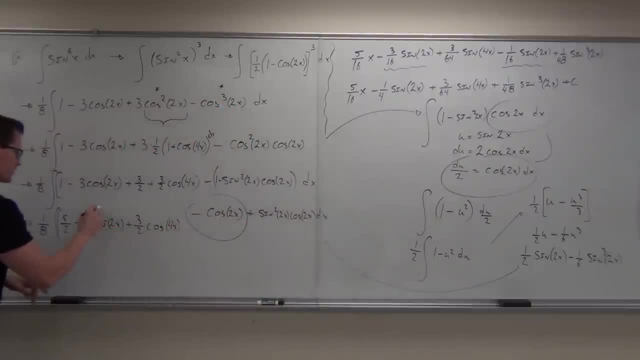 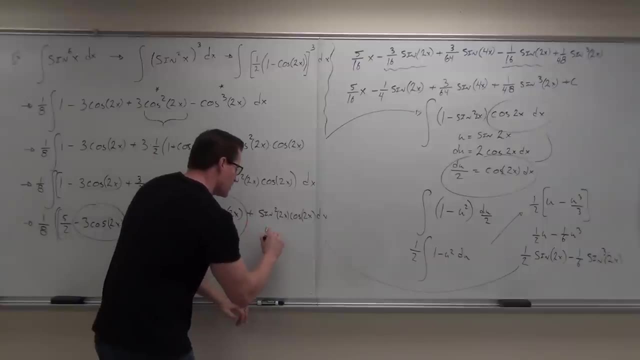 So this one would get combined with this one right now. This one, This one, This one is what you would do over here. You'd do the u sub on sine. You'd get du equals 2 cosine 2x dx. 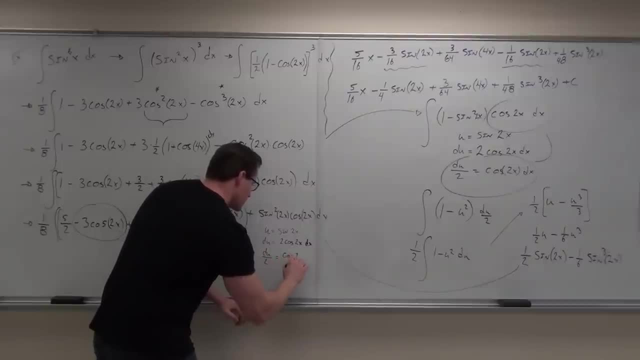 You'd get du over 2 equals cosine 2x dx. This is what would match right here. It would be a little substitution kind of off to the side, And what you'd end up getting is you'd get u squared over 2.. 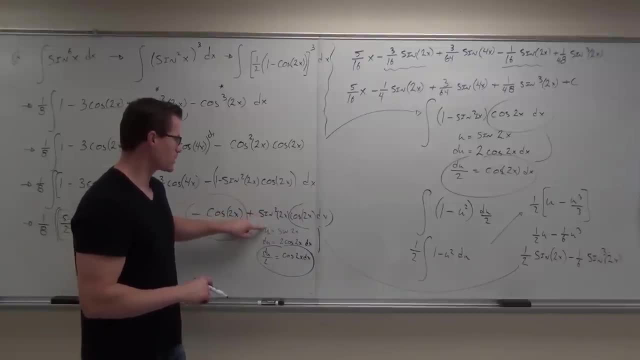 Does that make sense? u squared over 2.. So when you do u squared over 2, check that out. u squared over 2 would give you u to the third over 3 times 2.. That's 6.. 6 times the 1: sixth. 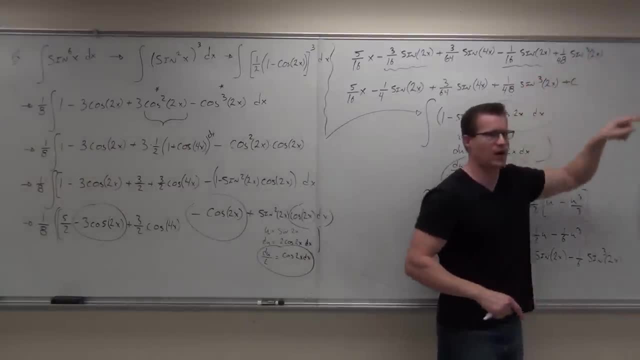 1, sixth times 8 gives you the 148.. Here's the u to the third power of the sine 2x. Oh my gosh, That's a lot of work. Either way, it works. I just want to prove to you that it actually does. 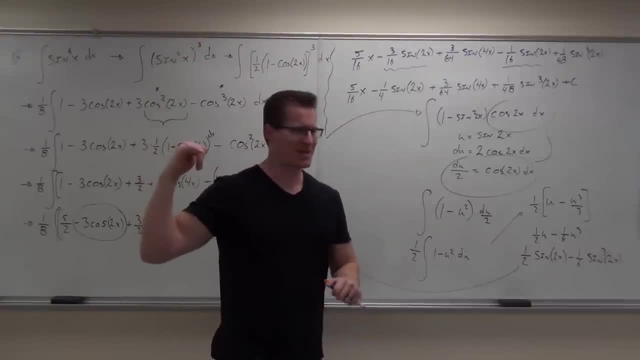 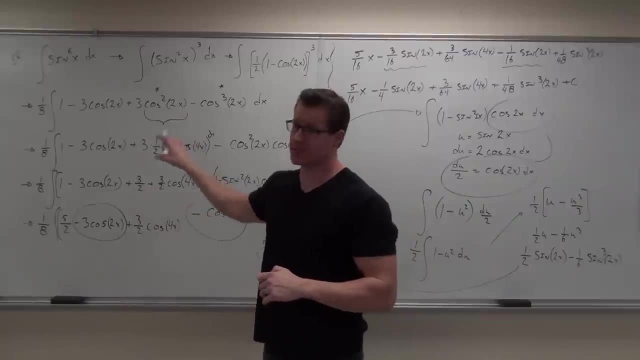 Show of hands. if that one made sense, Okay, that's hard right. What would be way easier? Not that, Not that The next formula would be easier, but if you don't have it or you can't use it, then this is what you have to do. 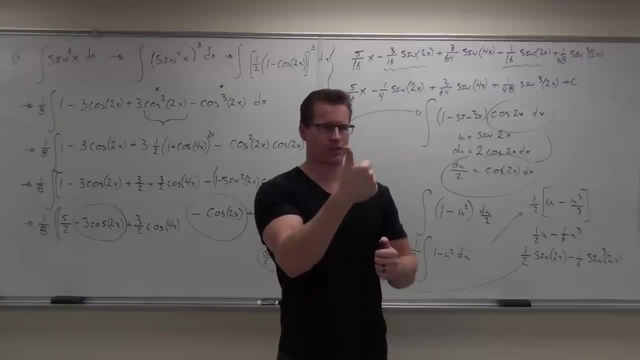 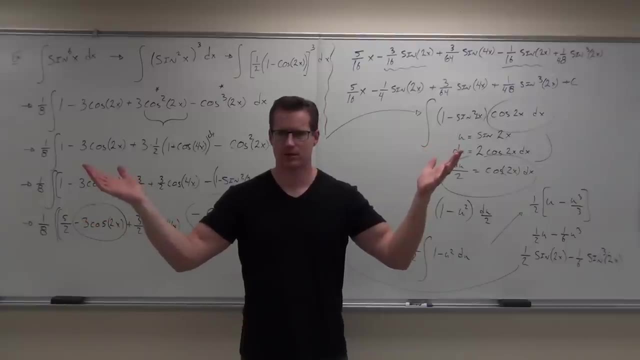 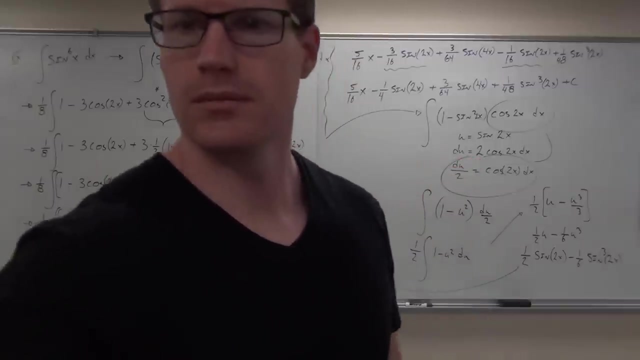 So what you should know at this point: odd powers, Odd powers. you use which identity, please? Everybody, Pythagorean, Pythagorean, Odd powers, Pythagorean, Even powers, Very good, All right, let's do our last example about integrals that involve sine and cosine. 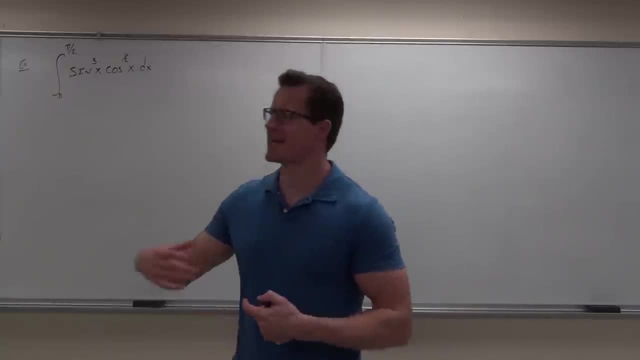 After this we'll talk about sine. There's some other types of trigonometric functions like tangent and secant, cotangent, cosecant, that stuff. I'll give you the rules on that after this example. but I want to go through one more. 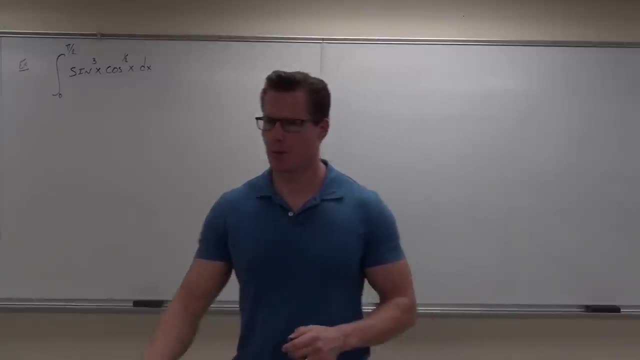 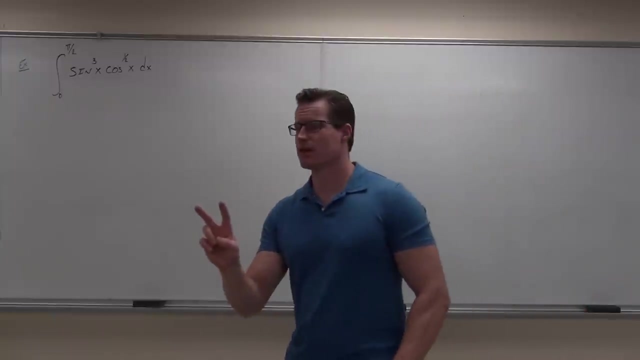 maybe when you don't have some whole number exponents. so you get a feel about what's going on Now. when we talked about our rules on integrating sine and cosine, there was two cases. There was the case where both powers are odd, where both powers are even, or where they 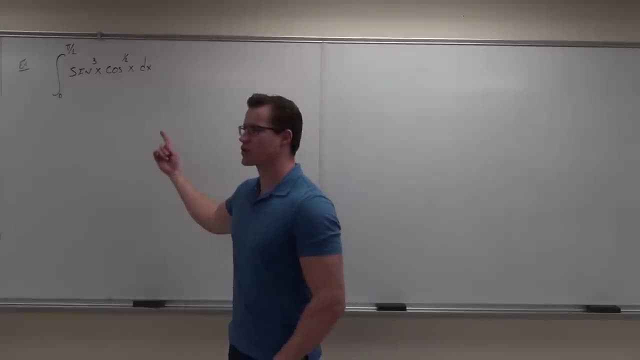 have one even and one odd. Wouldn't you have a fraction like this? Look at this. Look for the other one. This would be pretty hard to deal with. so we're going to look at sine to the third power. What case does this fall under? 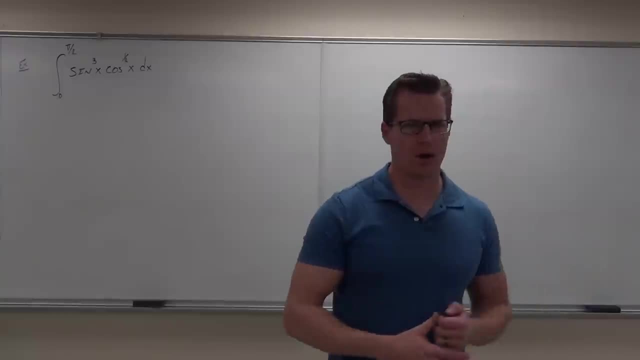 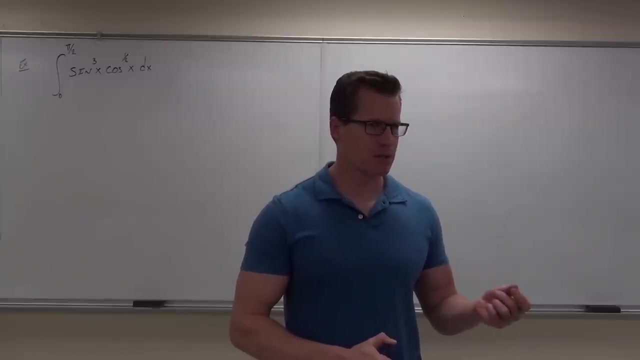 Does this fall under both, even both odd, or one of them being odd? One being odd, That falls under one being odd. Now, when we have that one being odd, do you remember what we do with that? Break one off. 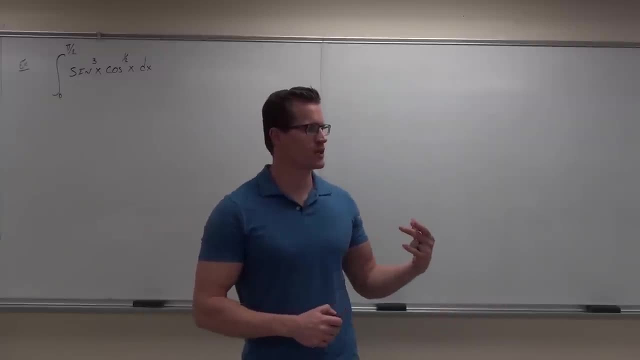 Break one off. That's right. We strip one off. Remember, We strip it off because what we're going to do is- oh, I hope you know- We're either going to do half angle or we're going to do Pythagorean. 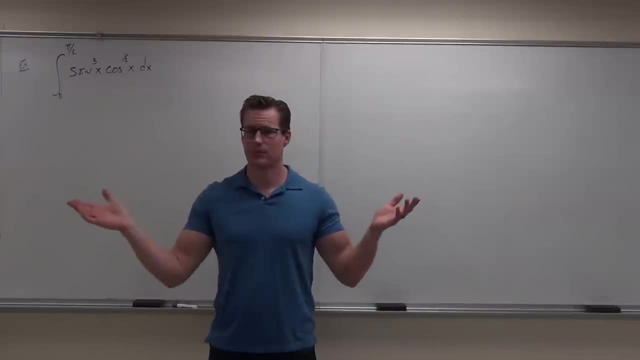 Pythagorean, Pythagorean. What's the case here? Pythagorean, It's going to be Pythagorean because we're going to strip one off and change the sine squared. As soon as you change the sine squared to a cosine, the reason why we strip off that. sine is because now a substitution will actually work. The derivative of cosine is basically sine with a negative. The derivative of cosine gives you the sine. It's gone, It's out of there and we're able to integrate the rest with a simple substitution. 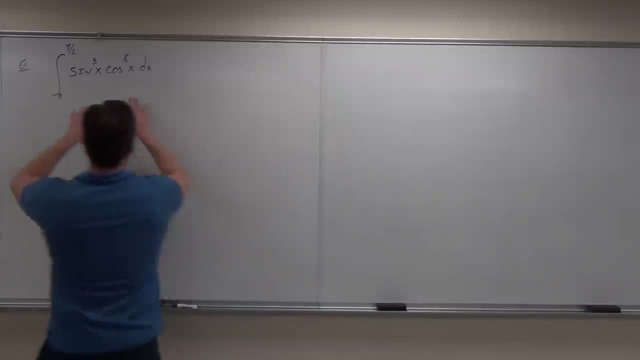 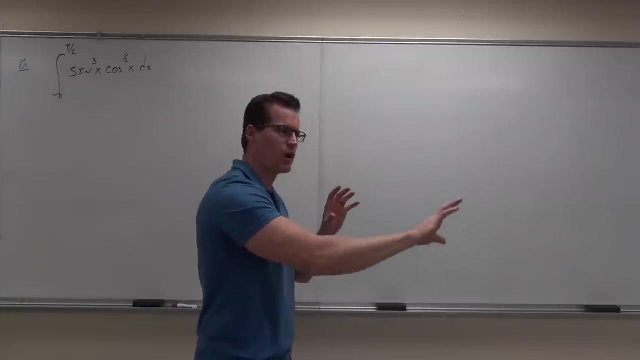 You ready? Let's try it. The first thing we look at: do we have odds or evens? That counts as an odd. Whenever you get an odd power of sine or an odd power of cosine, strip off the one that gives you a square power. 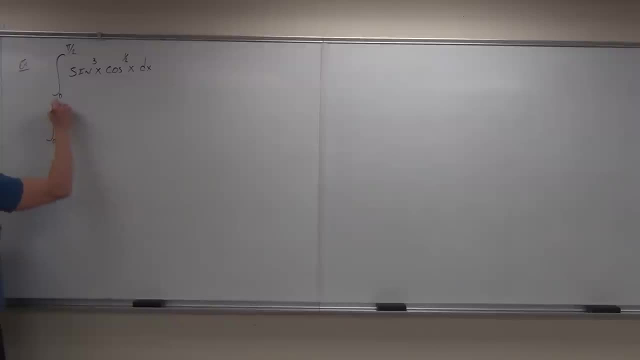 I don't want sine to the third. I'm going to write this as what? Sine squared x, Sine squared x. I like it: Cosine one half, Cosine one half. I like to write that one first because I like to strip off the sine and put it here, because 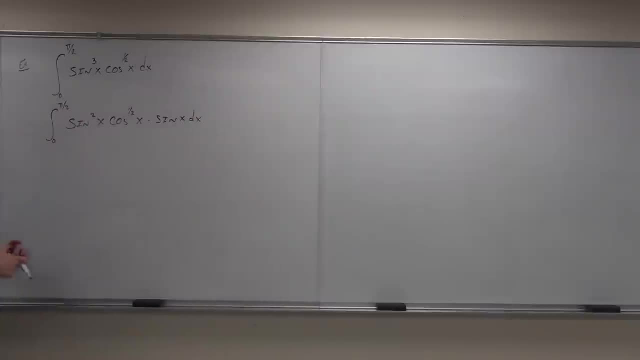 it makes our substitution look a little bit better. Again, here was the idea. We got an odd power strip one off, and then what are we going to do with the sine squared? What identity is that? Is that the half angle or the Pythagorean? 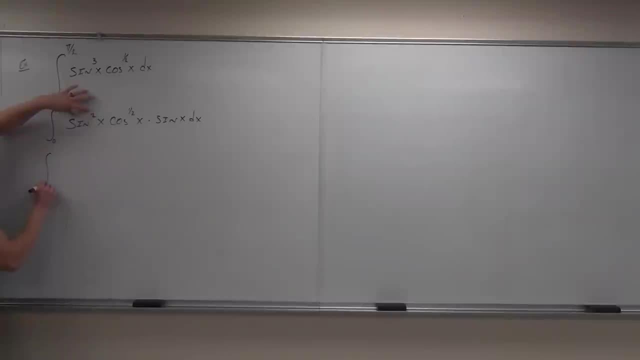 Use that one. So here we go. Okay, cool, I like this. We're going to do 0 to pi over 2.. We're not going to touch this until the very end. The idea again behind doing this is manipulate your integral so that you can use a substitution. 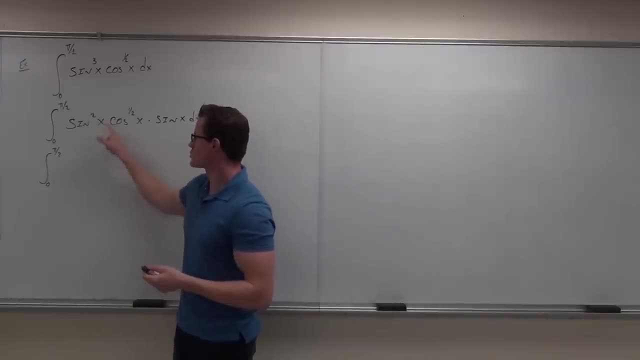 The way that we do, that is, we try to make these be the same trigonometric function. You have to make them the same And you have to make them the same So that when you take a derivative, it's this guy over here. 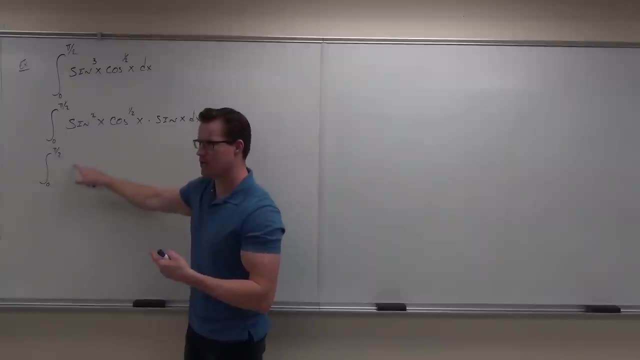 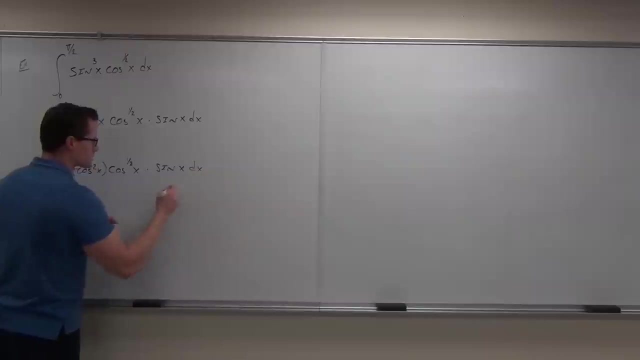 So use Pythagorean to change sine into a cosine. Then we'll have all the same stuff: One minus cosine squared x times cosine to the one half x times sine xdx. So when we have an odd strip one off, Now we use Pythagorean identity to make everything besides this guy into cosine. 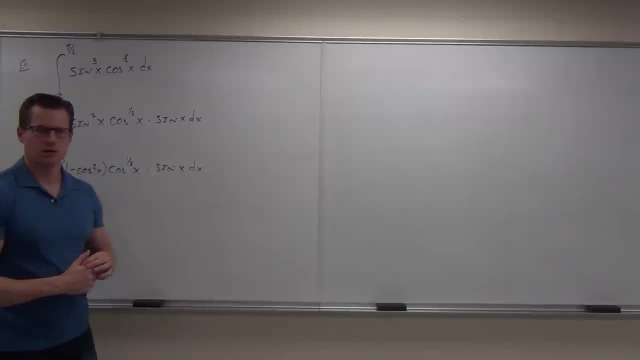 Once we do that, do you see a substitution that's going to work? Don't worry about distributing, You don't have to do that. Don't worry about that, Just make your substitution. What's your substitution going to be Then? du equal, oh, derivative of cosine x, what is it? 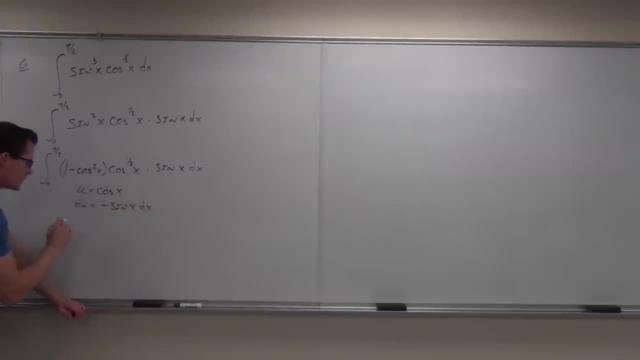 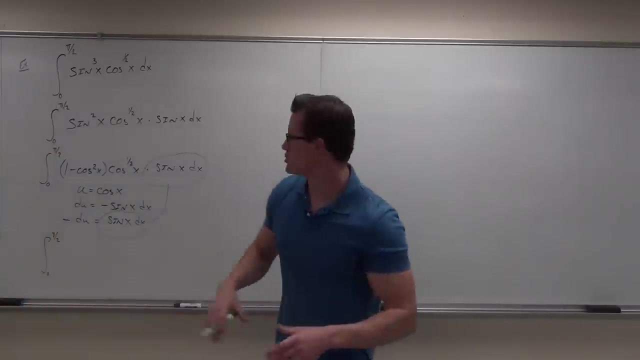 Negative sine. Very good, Okay, So we know that negative du equals sine xdx. That is what we have here. Let's keep on going. Can you all tell me what's going to be in my integral once I make that substitution? 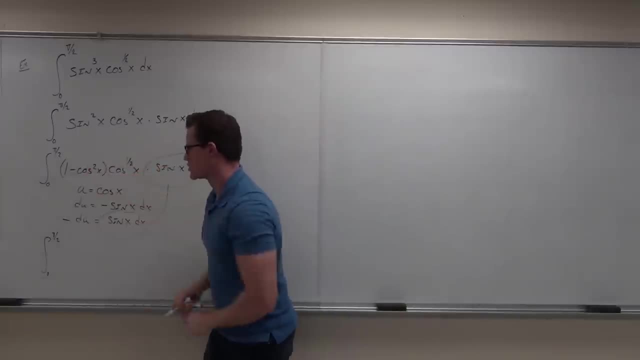 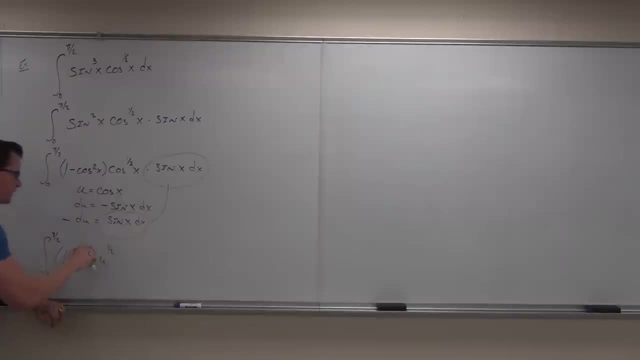 What next? U to the one half? Oh good, So we still have u cosines. u? u to the second. u to the one half. Negative du. Yeah, Don't forget that. negative, The sine dx, is negative du. 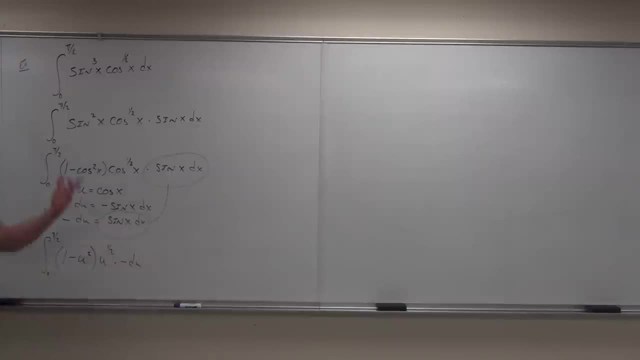 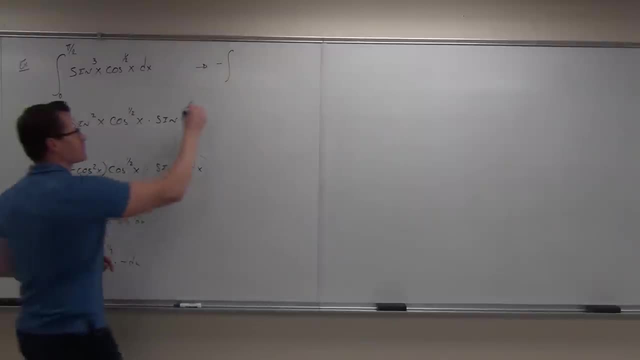 We'll move the negative out front. We'll move the negative out front. We'll keep our bounds of integration. Distribute the? u- Yeah, let's distribute the u. So right now, once you make the substitution, it's a lot easier to make the substitution. 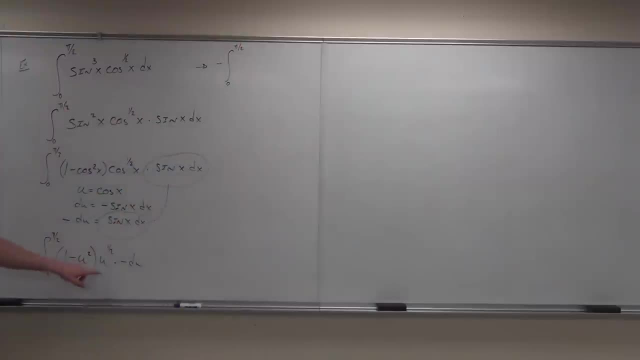 then distribute. rather than distributing, then make the substitution. There's less to have to deal with. So when we do our distribution we get u to the one half Minus u to the one half Minus one Minus u. 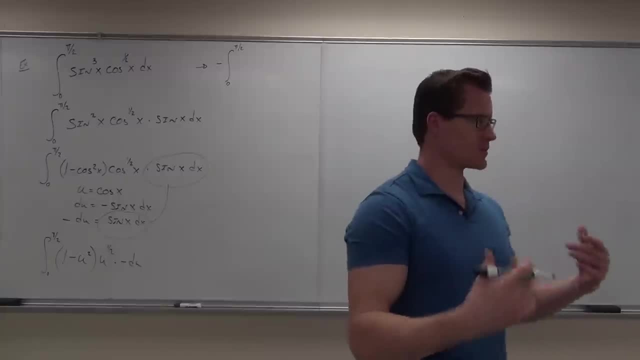 Minus o? U to the one half. When we multiply powers together, do we add them or multiply them, Add them, Add them. You add them. So u to the first Minus, u to the one half. Minus o. 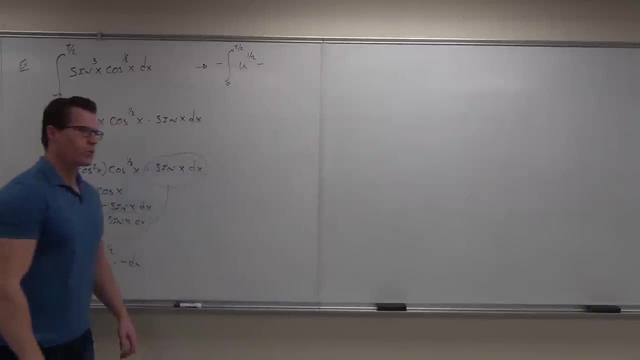 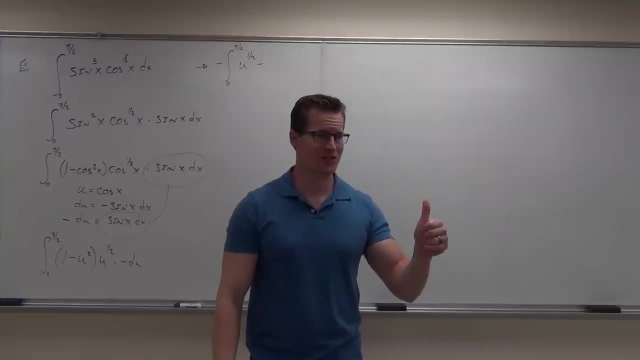 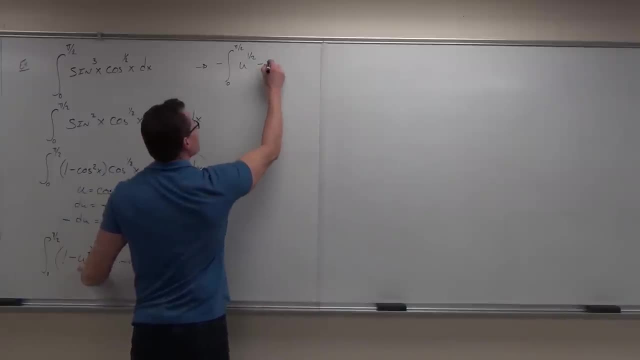 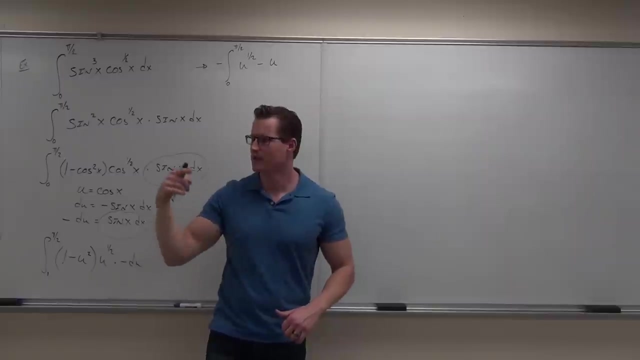 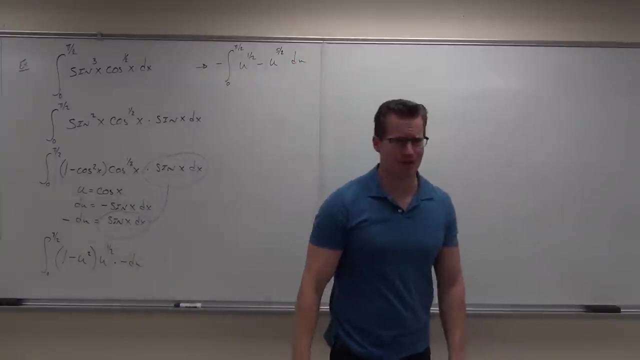 Four. Let's see Four over two plus 1 over 2, that's 5 over 2.. You will get five halves. I hate to say it, but use a calculator if you have to. I don't care, Get it right. 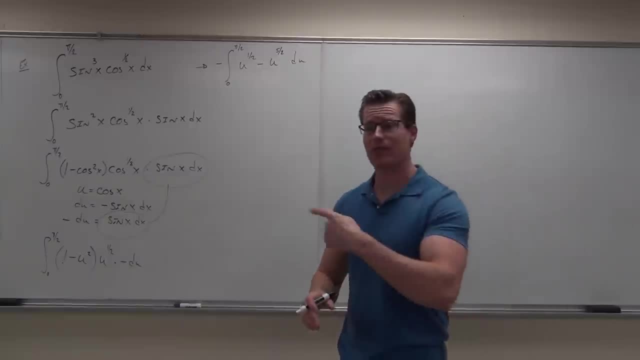 Ok, Don't multiply those and give me one, or I'll be like goodness. add the powers you have. two plus a half. well, that's two and a half. five halves, that's what that is, you guys. okay with that one. finish that off, go ahead. you would. if you added one plus a half, that'd be one and a half, that's. 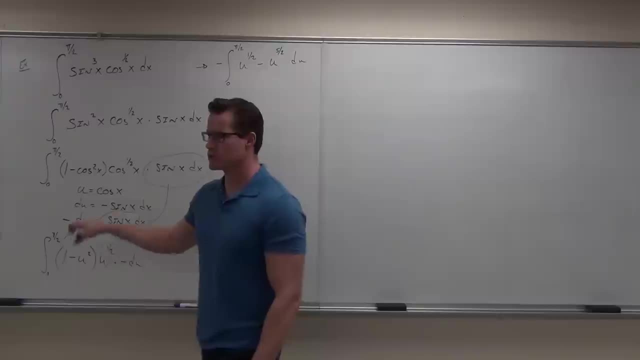 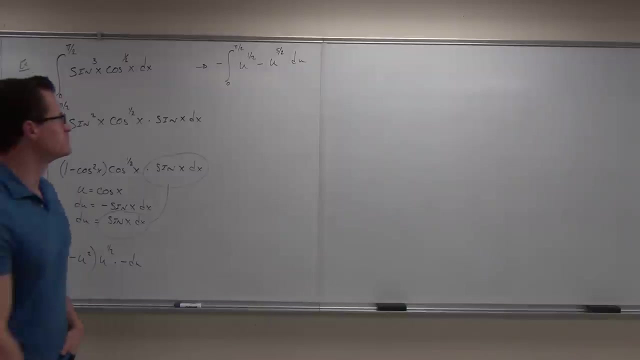 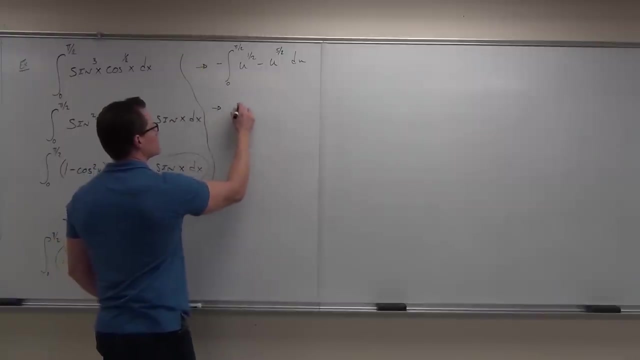 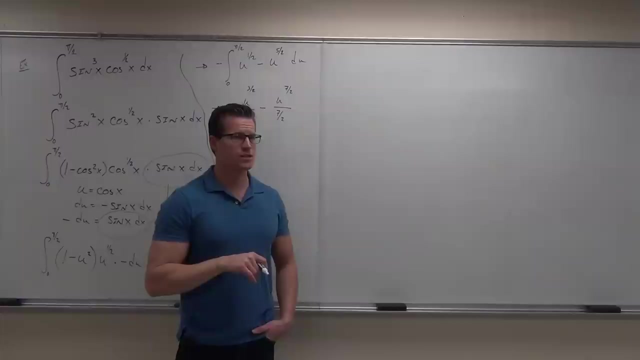 three halves, but if you add two plus a half it'd be two and a half, five halves. did you get three halves over? u to three halves over three halves? did you get you to the seven halves over seven habits? what am i missing, listen? do i need a? 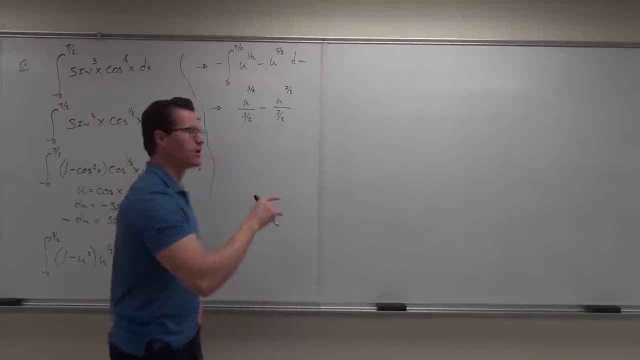 plus-c here. no is definite, okay, so good one. I miss a and front of the whole. do you guys have brackets? you should, because we're subtracting this whole integral. okay, so we're subtracting this integral overB,2i in g, x, y. 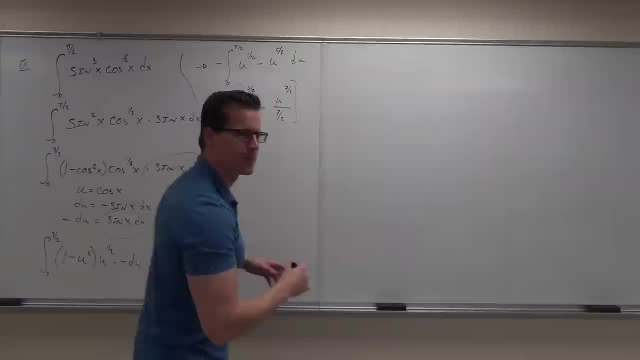 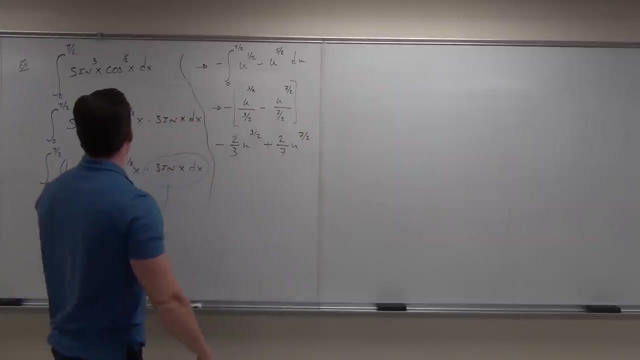 thing. what's going to happen here? let's simplify this. what's it look like? okay, so negative, negative. what two thirds U to the three-halves? okay, I like it. then what two seconds? would you want to change the balance on this line? that's a. 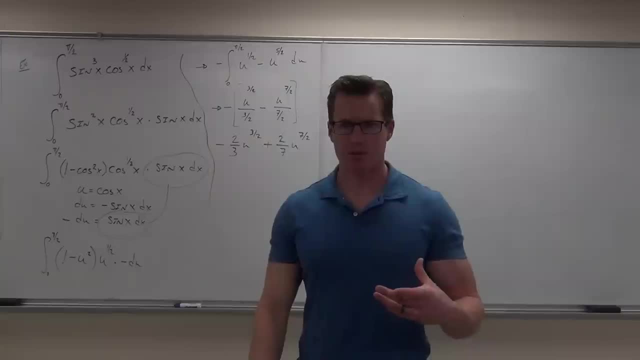 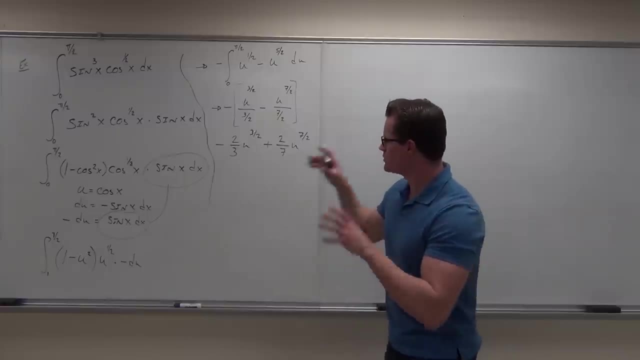 good question. that depends on you. if you want to change the bounds, then you should have already done it correct. yeah, if you don't, let's. let's say this: some of you guys made a little bit of a mistake on the last test. let's say you. 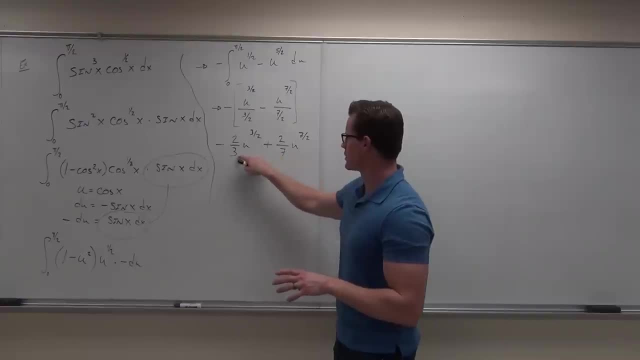 don't change the balance. do you plug in 0 and pi over 2 here? no, what do you put here? you'd have to put whatever you, this would have to be code. yeah, whatever you is, you have to put cosine back in there. then you plug in 0 to pi over 2. does. 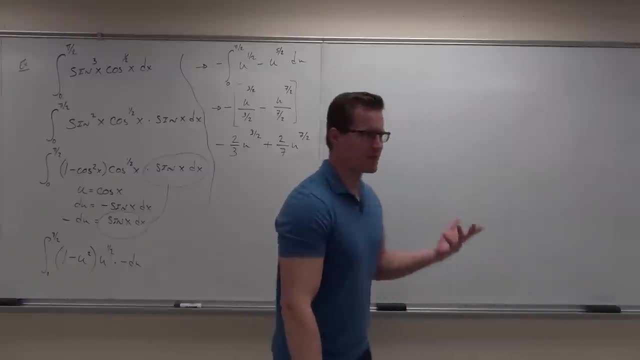 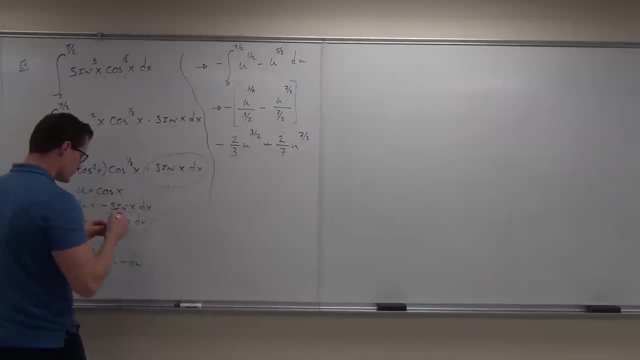 that make sense to you. if you go ahead, I like changing balance. personally, I think it's easier, or at least it's more straightforward. so, right here, what I would do is: it's okay, we start with X's. so if X equals pi over 2, then U equals, and if X equals 0, then U. 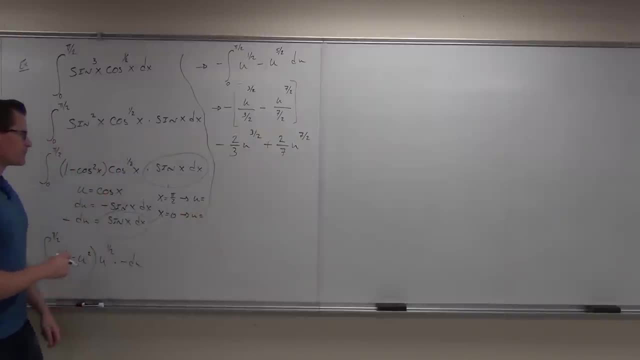 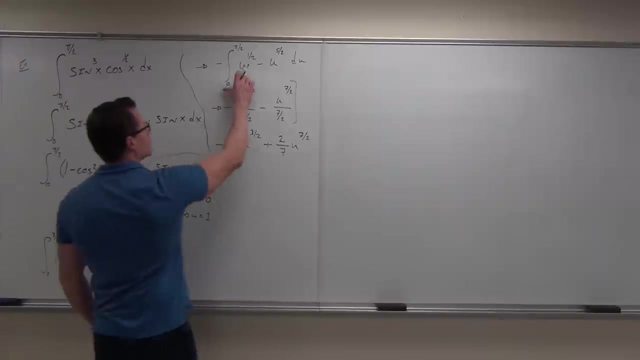 equals and we just plug that into cosine. so if we do that, we've got cosine of what's cosine of pi over 2? and if we plug in pi, let's see if we plug in 0, what's cosine of 0- 1? okay, the only problem that we're gonna have here if you do it this way. 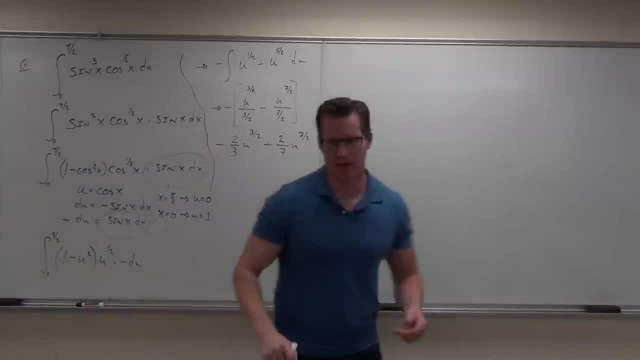 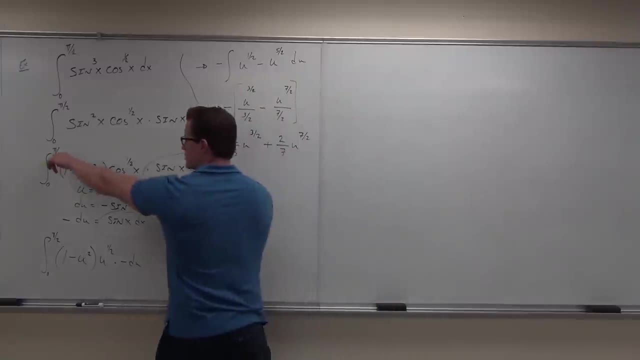 please be careful. this is probably good for you guys to see. this is why we're doing right now: where's the 0 go, bottom or top? the top goes on the top because pi over 2 got mapped to 0. does that make sense to you, okay? where's the 1 go from? 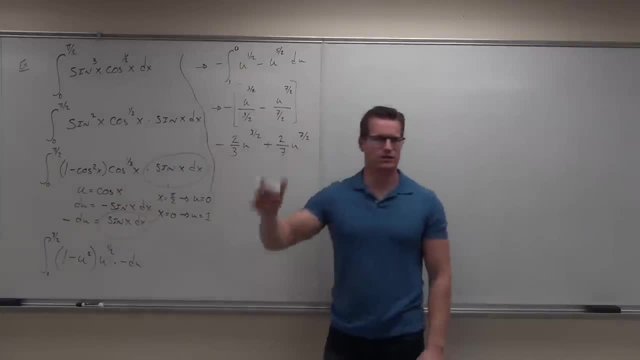 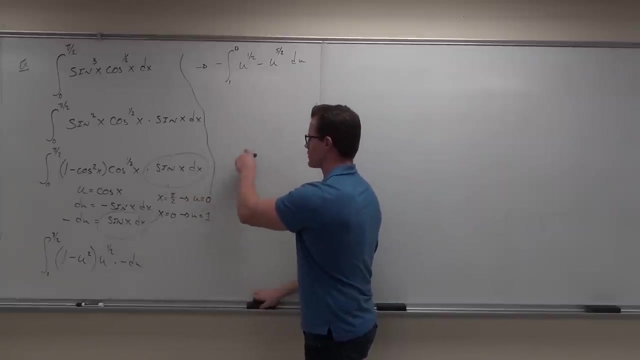 the bottom 1. so if hands are feel okay with that one, okay, if you do it this way, if you do it this way, what happens right here? so other way? if you had this, you'd have to do cosine for your U and then plug in the actual values. it's fine, you go ahead. 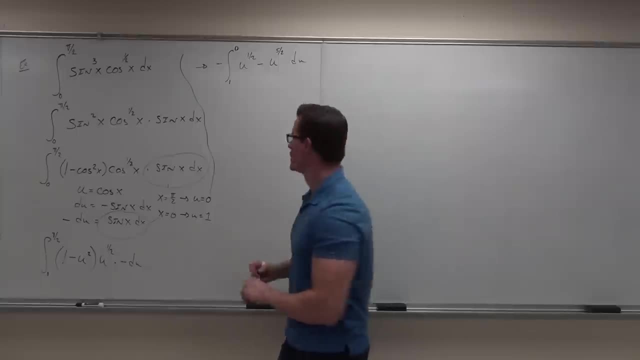 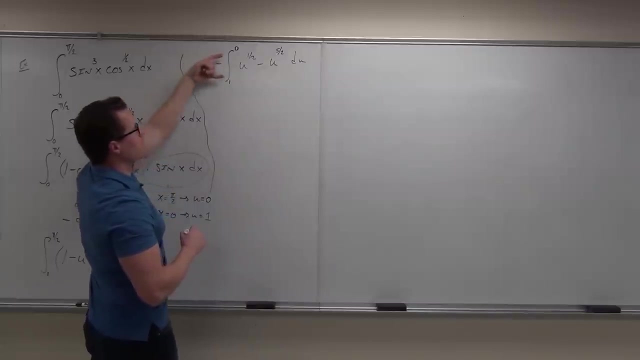 and if you, someone who had that on paper, go ahead and do it, make sure you get the same thing we did. if you do it this way, if you actually change bounds, you should have remembered from your calculus one that when you flip your integral, your Your sine changes. 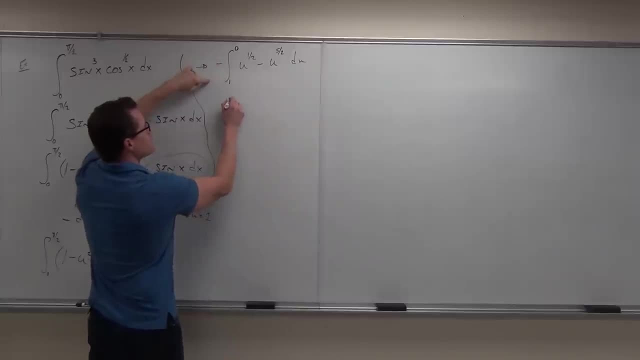 Do you remember that property? Yeah, If you flip this, you go: okay, let's make it from zero to one. Let's put it in the correct order. Negative becomes positive. It changes that. So eventually we'll be okay with that. 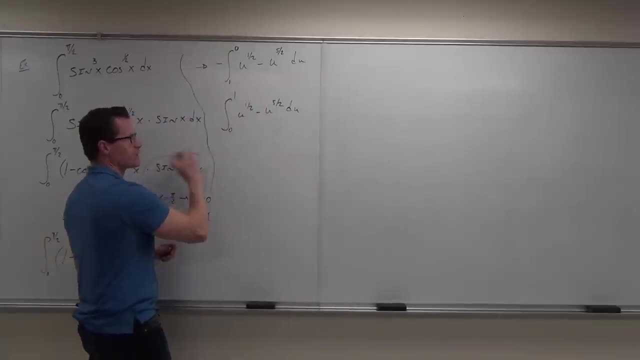 Okay, and now it becomes well something we can do. We don't have to resubstitute in that cosine, So this would be 2 3rds u to the 3 1⁄2 minus 2 7ths u to the 7 1⁄2. 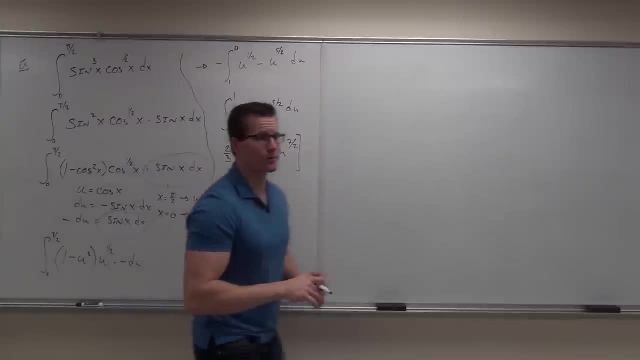 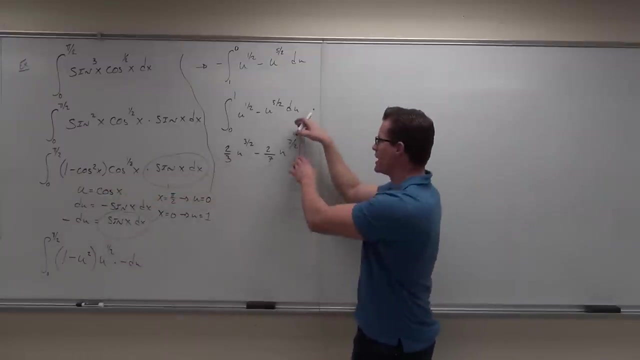 We already did that. Now let's practice this one. If I do this, if I change my balance, do I have to put cosine x back in for my u? No, No, change them. These are now in terms of u from zero to one. 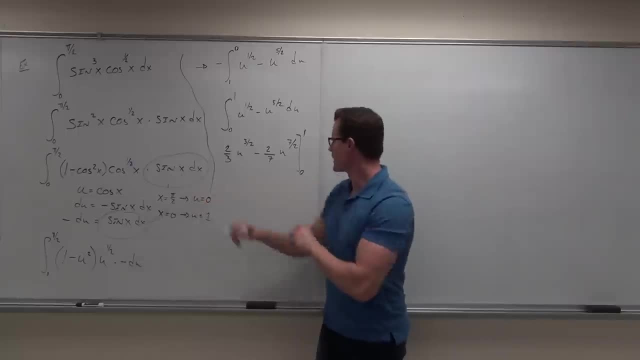 Those are u's now. They were x's, Now they're u's. We just showed that We get to plug in one, We get to plug in zero. We don't have to plug them into cosine because we already did over here. 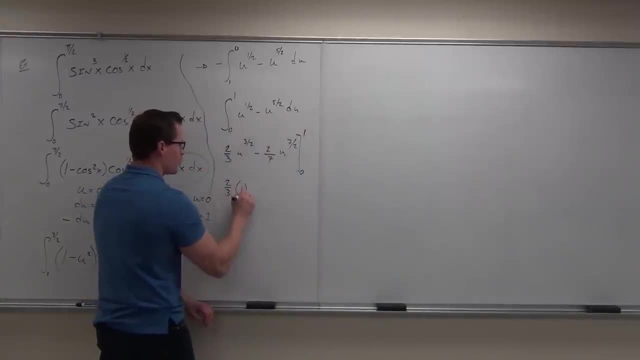 That's how we changed it, So we'd get 2 3rds 1 to the 3 1⁄2, minus 2 7ths 1 to the 7 1⁄2.. I always plug these in in case something funky happens. 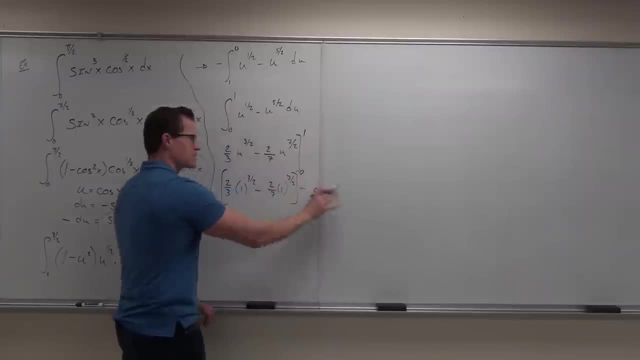 We get zero. Okay, that's gonna be zero minus zero, So nothing's gonna happen over here. One to any power is still one, So 2 3rds minus 2 7ths. How much is 2 3rds minus 2 7ths? 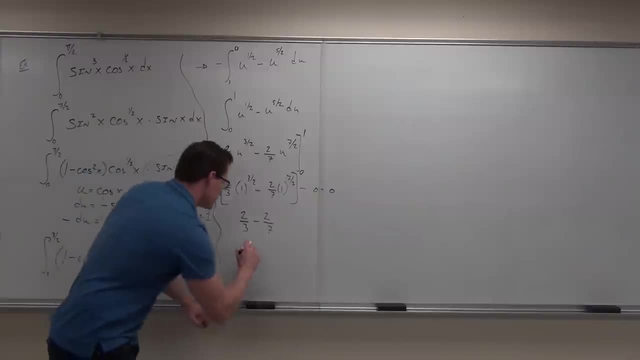 Eight, twenty-four, Eight, twenty-four, okay, Eight over 21.. Michael recovers. This would be negative, correct? But if you have a negative out front already, it becomes positive. That's the idea I wanna show you, if that made sense to you. 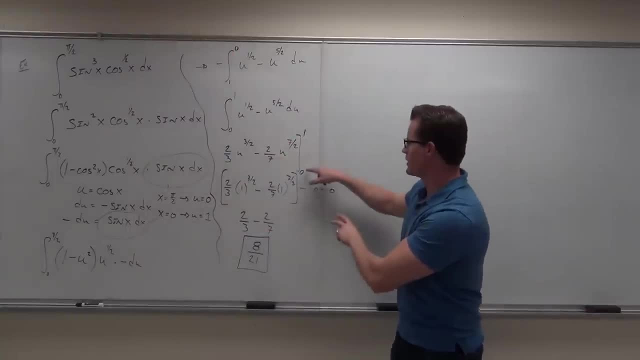 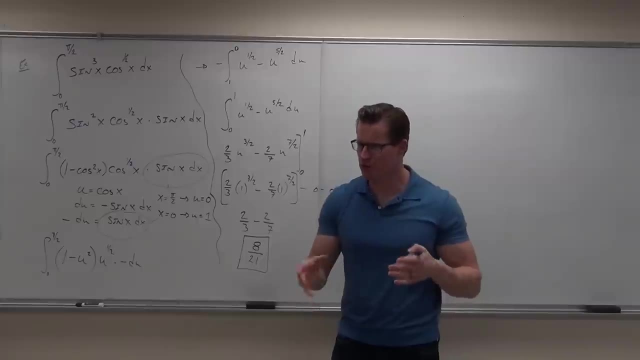 If you did it the other way, This would make sense to you. You wouldn't do this. you'd still have 0 to pi over 2, but you'd be plugging it into cosine here and cosine there. I want to make very, very sure that you're clear on that one. 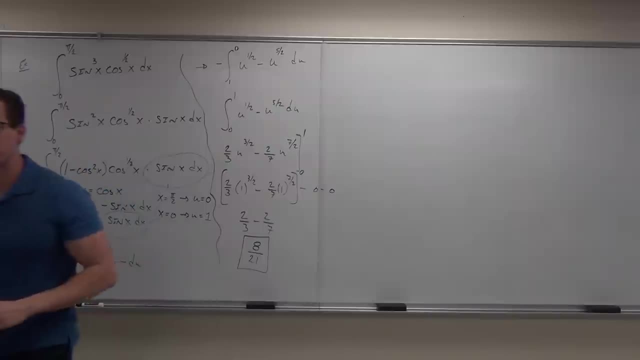 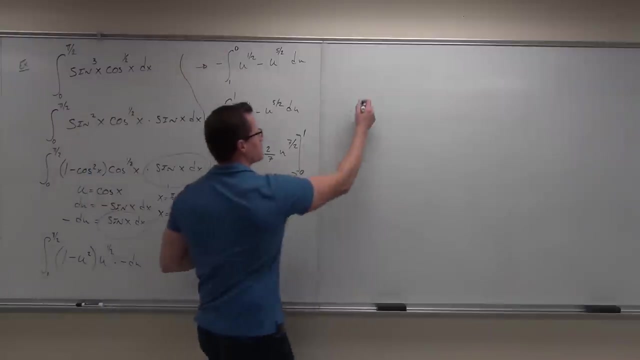 Are you guys clear on that? Yeah, It would be awesome. Say what You'd have to distribute the negative. Yeah, you would. If you didn't, if you left it with the original bounds, you would get negative 0 to pi over. 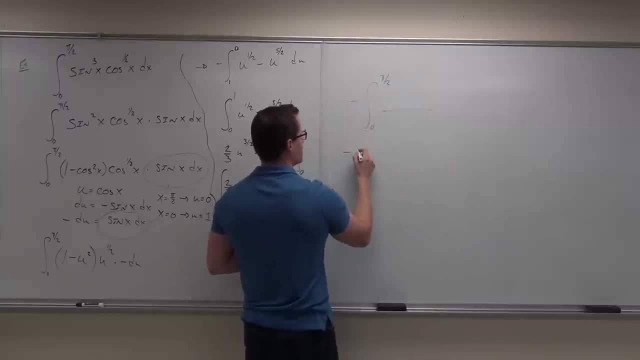 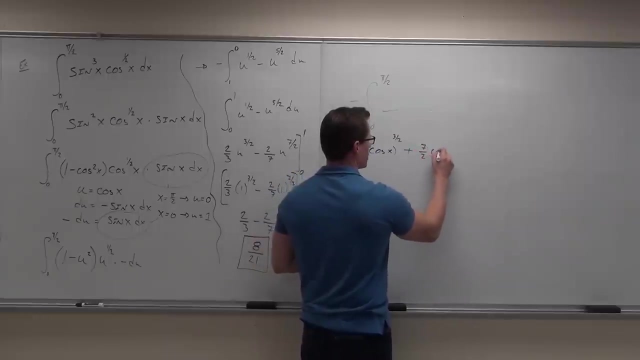 2, like that with all this junk, and then you'd have negative 2 thirds u, but the u would become cosine x, 2, 3 halves plus, because you would distribute the negative 7 halves cosine x to the 7 halves. sorry, I added this backwards: 2, 7ths and then you'd plug. 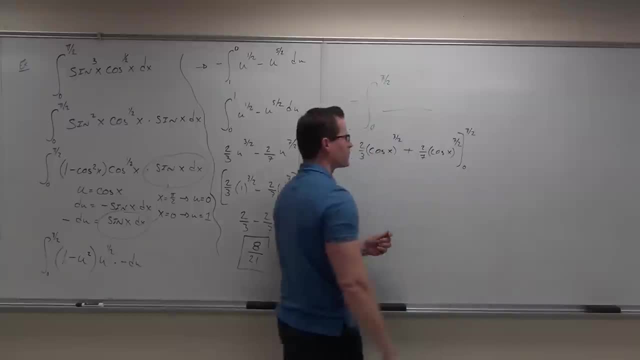 in not 0 to 1, you'd plug in 0 to pi over 2.. Well, if you look at that, it's going to be the same cosine of pi over 2, this is 0, 0.. 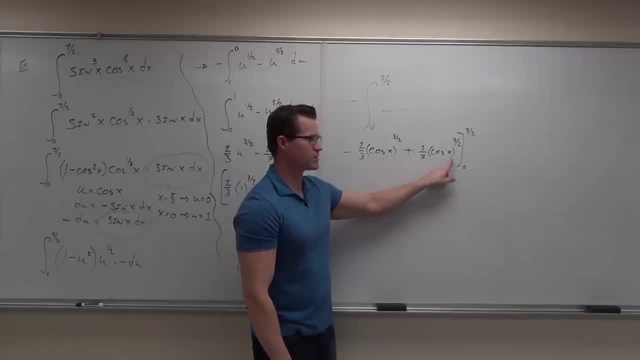 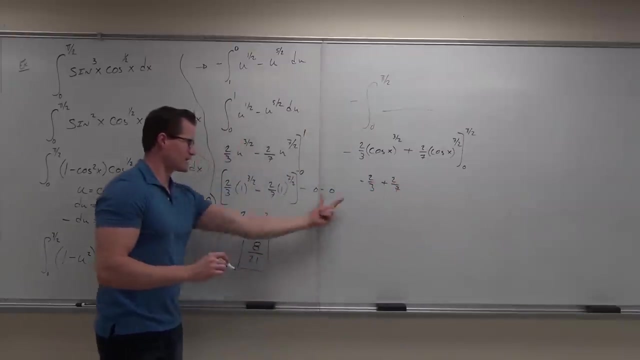 0.. 0.. 0.. 0.. Cosine of pi over 2, this is 0, but the 0's aren't 0, cosine of 0 is 1, cosine of 0 is 1, so this is negative 2 thirds plus 2 7ths. oh, look at that. it's exactly the same, just. 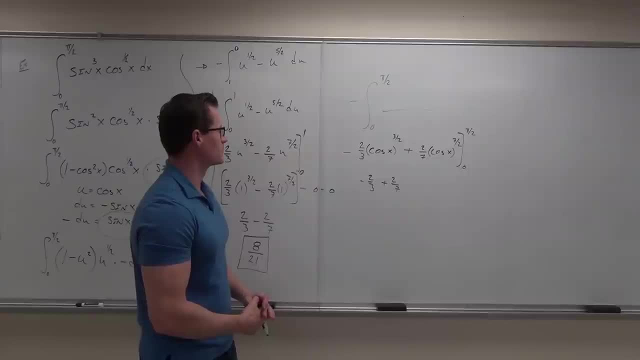 negative. oh, I missed something. huh, because we should, let's just subtract them. so it would be. Oh, I missed something, huh, because we should, let's just subtract them, so it would be: oh shoot. 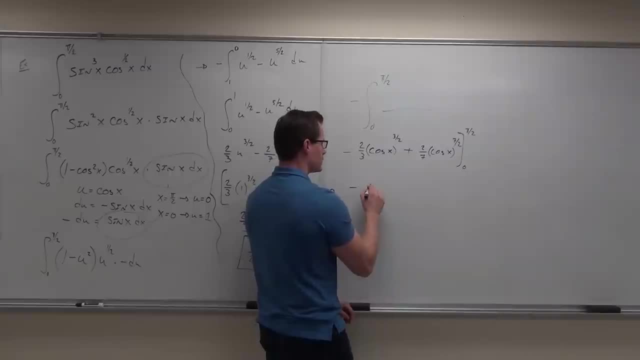 Oh shoot. Negative 0 plus 0, minus negative 2 thirds plus 2 7ths is how it would really look. Negative 0 plus 0, minus negative 2 thirds plus 2 7ths is how it would really look. 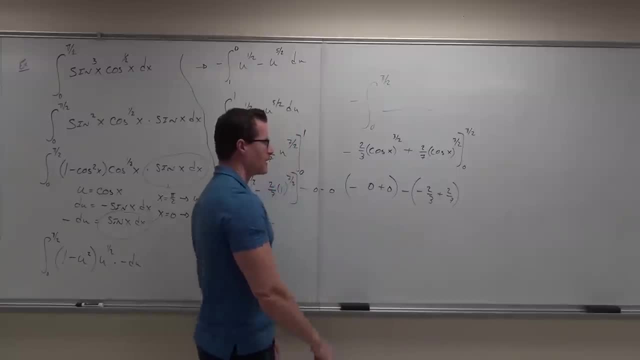 Negative 0 plus 0, minus negative: 2 thirds plus 2 7ths is how it would really look. That's the same thing. This, if you distribute at: 0, 2 thirds minus 2 7ths: that's the same. 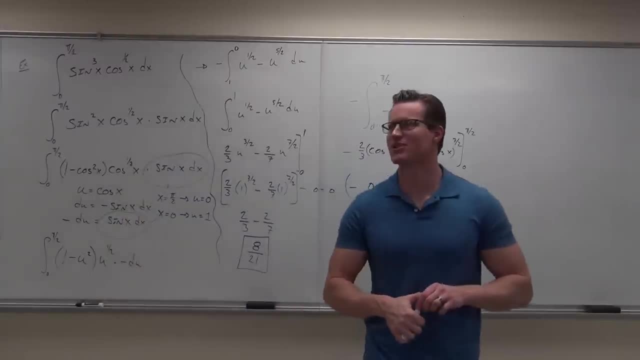 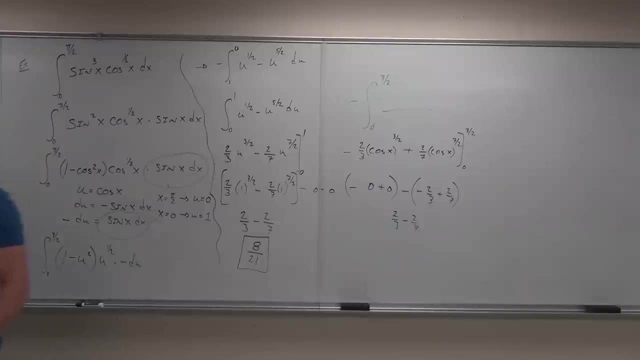 Same idea, exactly the same. Make sense, now Even more sense. I know it made sense before, but now it's like extra sense. Anyway, We're going to talk about one more thing in this lecture and I really want to talk about. 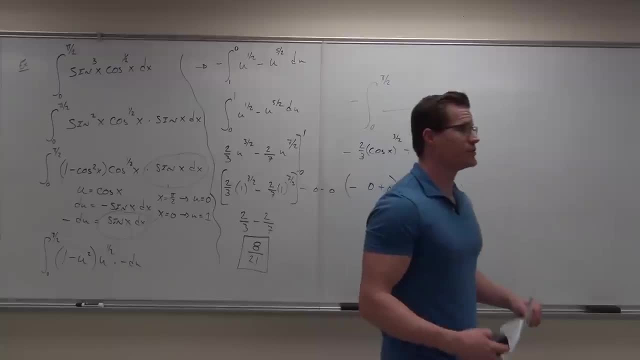 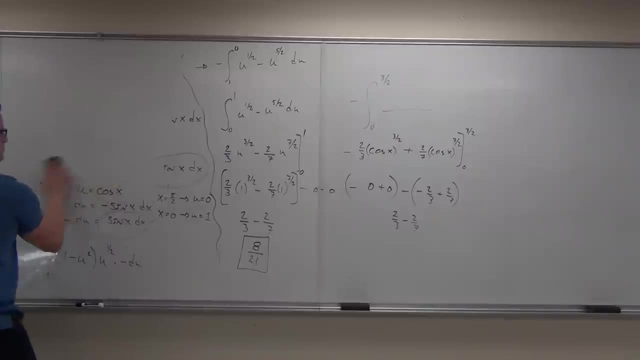 in this section how to do some integrals that maybe don't have just sines and cosines. We've been practicing with sines and cosines all day long, all lesson long. Let's look at something else. Oh, by the way, did you have any questions? 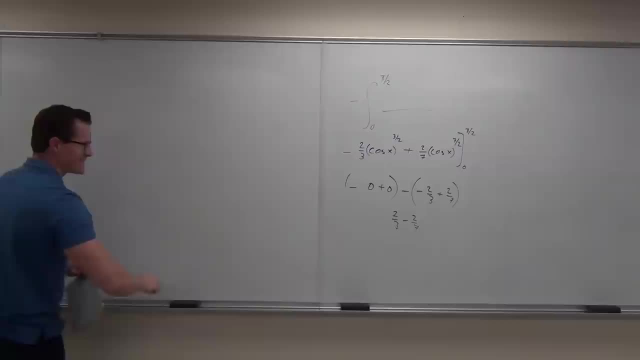 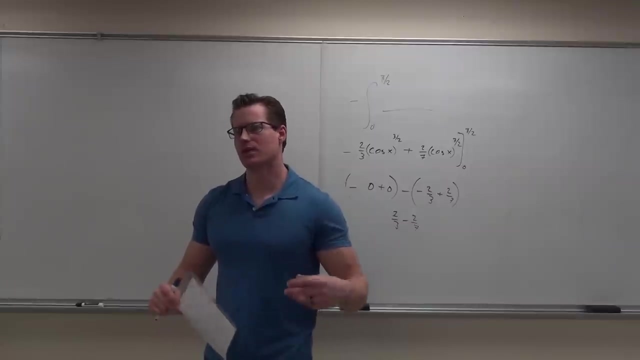 No, sir. Okay, all right, Good, Too late. So what happens if you have something like not sine cosine but tangent, and probably something else like secant? We group sine and cosine together, because the derivative of one gives you the other one. 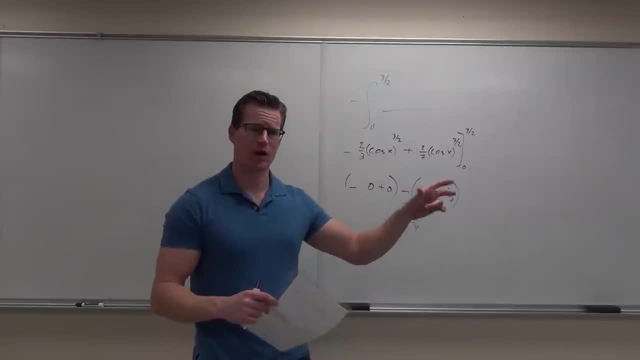 Does that make sense? And we group tangent and secant together because the derivative of one kind of gives you the other one, especially with like secant squared and things And cotangent cosecant. So those ones are grouped together because it's possible to do. 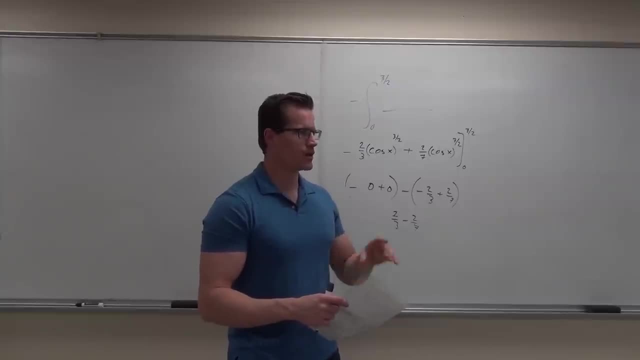 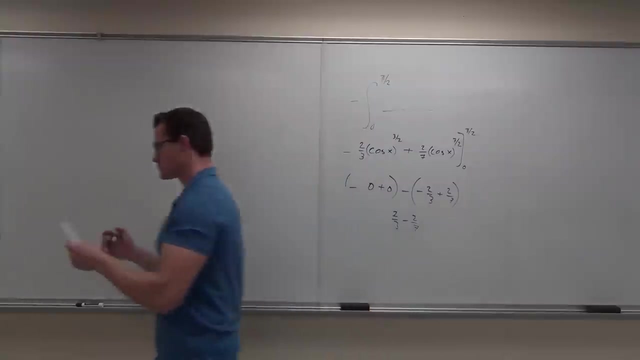 If you don't have that scenario, you have to change things to sine and cosine and work at it a different way. I'll give you that example much later, So like at least another day. So what about integrals that involve tangent and secant? 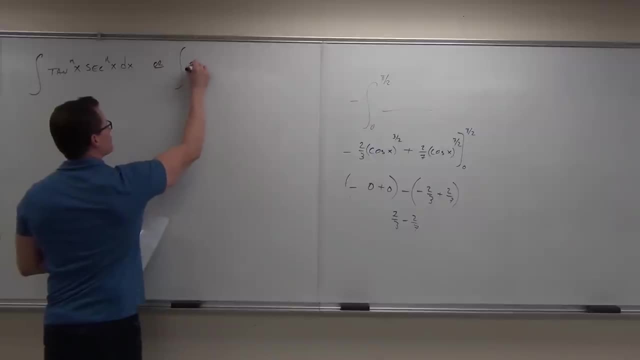 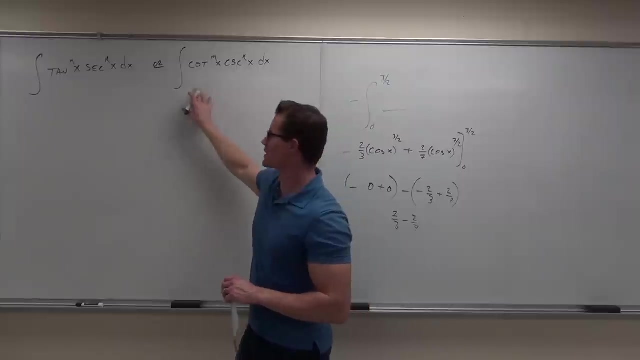 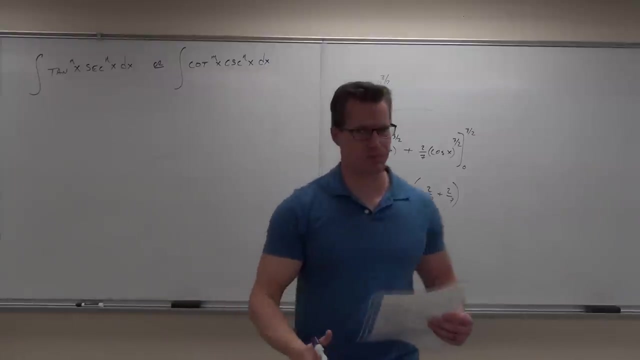 Or cotangent and cosecant. I'm hoping that you understand the ideas that we use here. We're going to use the same exact ideas here because the- The tangent and the cotangent, secant and the cosecant, they work really similar and the identities are very similar. 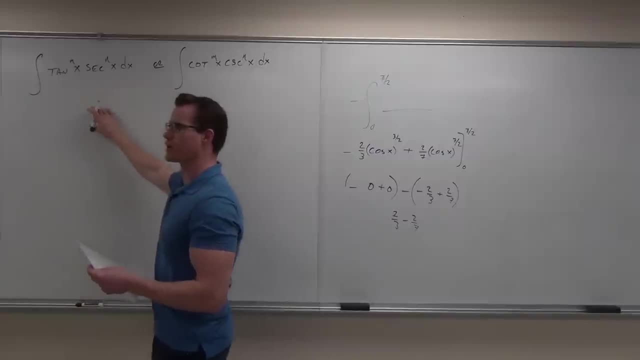 So let's take a look at what we do with this one, and we'll use a corollary for this one. So here's what we do. Just like we have rules for sine and cosine, we're going to have rules for tangent and secant. 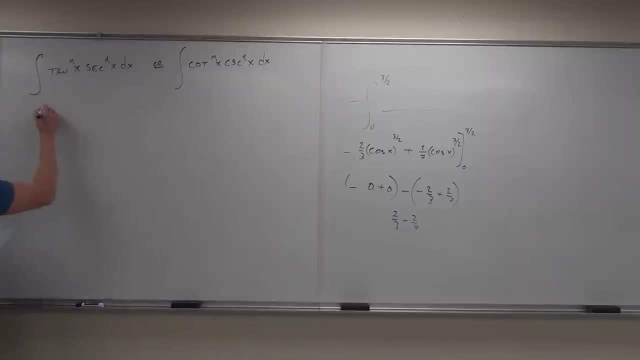 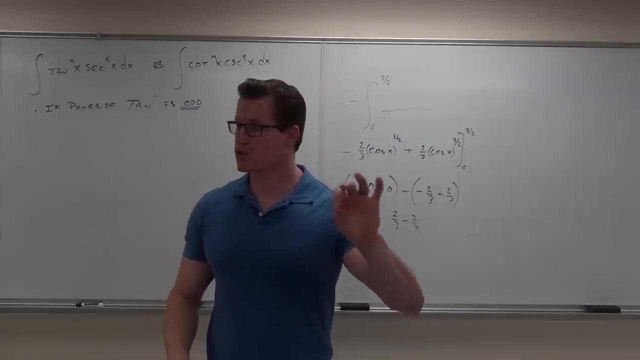 If tangent is odd. so if tangent is an odd power, If the power of tangent is odd, what we're going to do is something kind of fancy. We're going to strip off not only a tangent, but we're also going to strip off a secant. 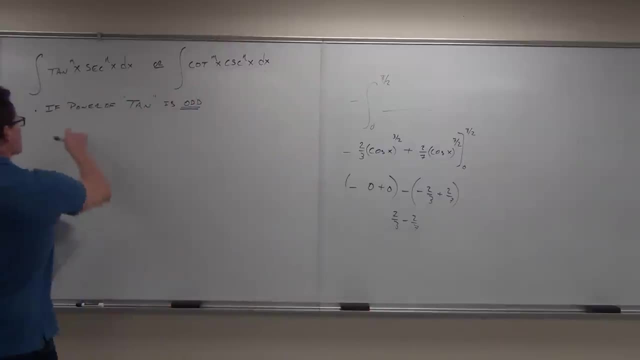 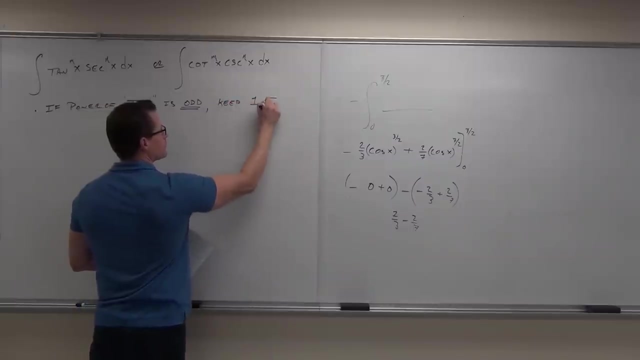 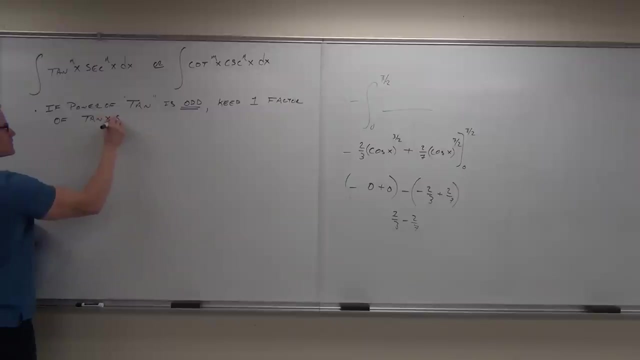 So we're going to keep a tangent and a secant. I'll explain why in a second. So if the power of tangent is odd, keep one factor of tangent X, secant X. In fact, I'm going to write it backwards. 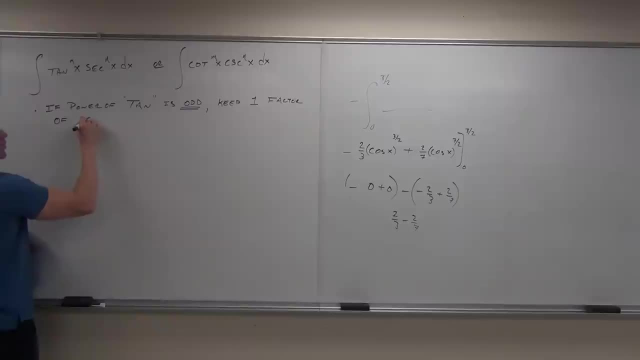 So we're going to keep a tangent. We're going to strip off both a tangent and a secant. Keep one factor of secant X, tangent X. I'm going to write it this way because it's going to make a little bit more sense right now. 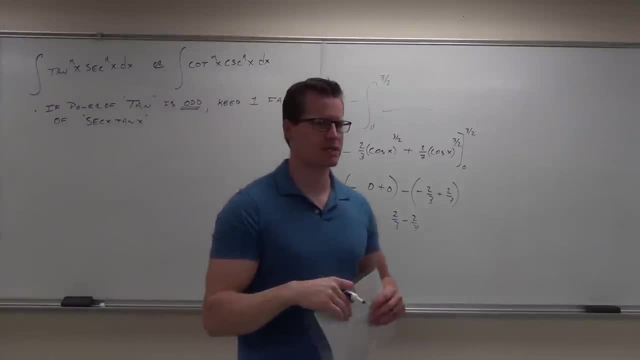 Remember the idea behind this? I hope that you do. The idea is that we're going to break off a little piece, right? Yeah, We're going to break off a little piece so that we can take the derivative. So if tangent is odd, if tangent is odd like 3,. 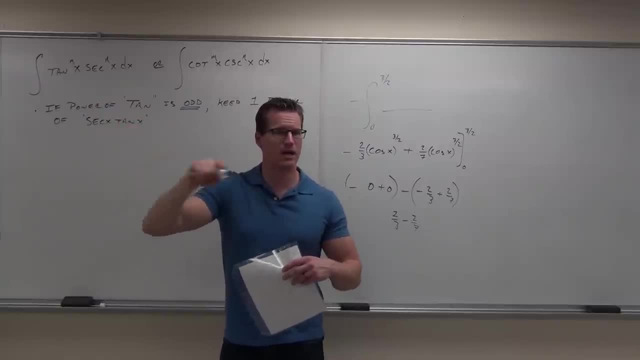 we're going to strip off a tangent That's going to make the remaining power a 2. Tangent to the second power has an identity: It's going to change into secant. Hey, what's the derivative of secant Tangent to the secant tangent? 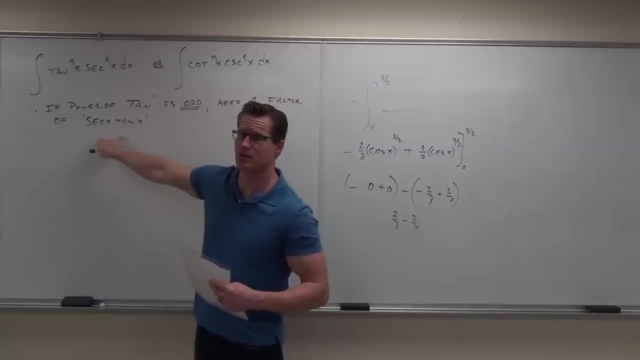 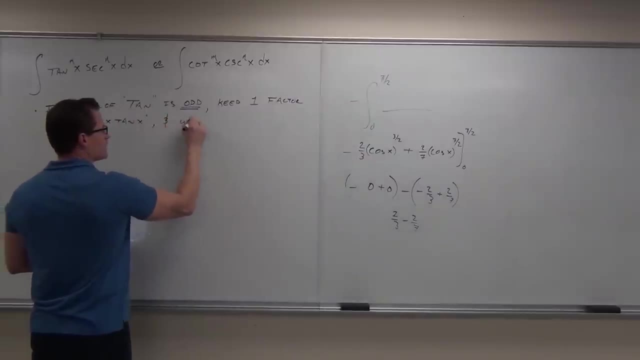 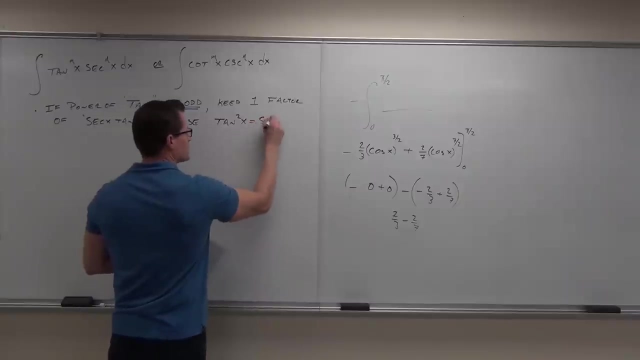 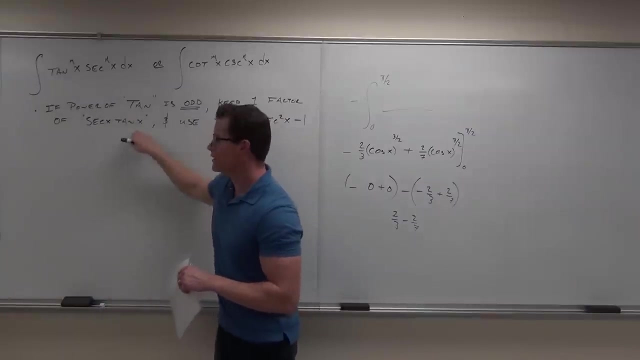 That's why we're keeping that, because this will allow us to do a substitution. So if the power of tangent is odd, keep one factor of secant tangent And you Use: tangent squared X equals secant squared X minus 1.. What that does? that changes all of this tangent into secant. 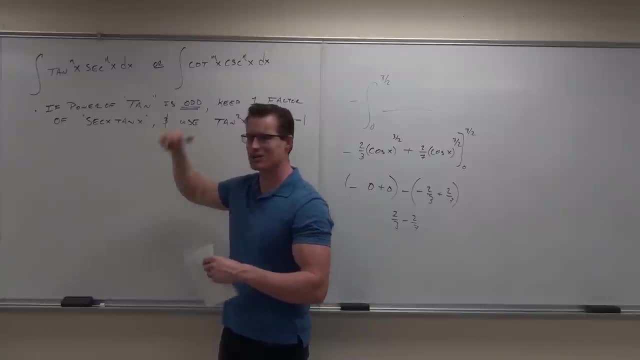 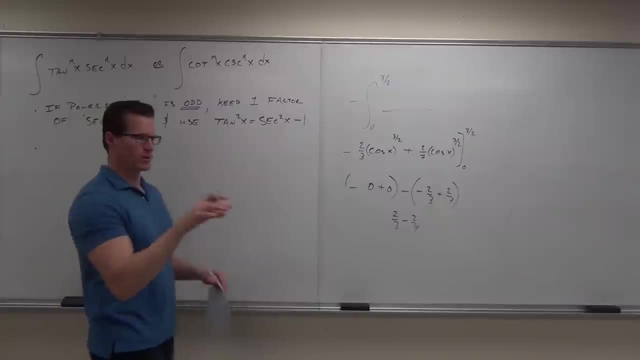 Then you can use a substitution. The derivative of secant is secant, tangent, and you're pretty much good to go. Now, let's say that the power of secant. So we check first the power of tangent. okay, If it's odd, you're good. 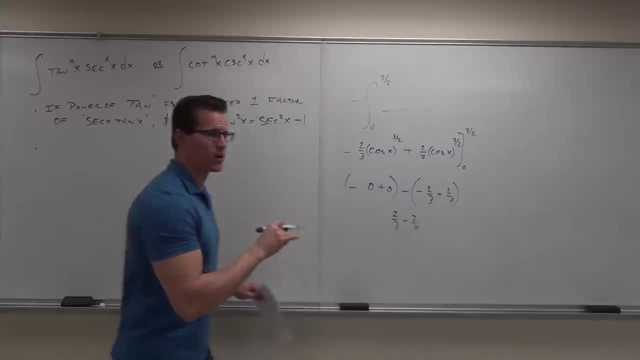 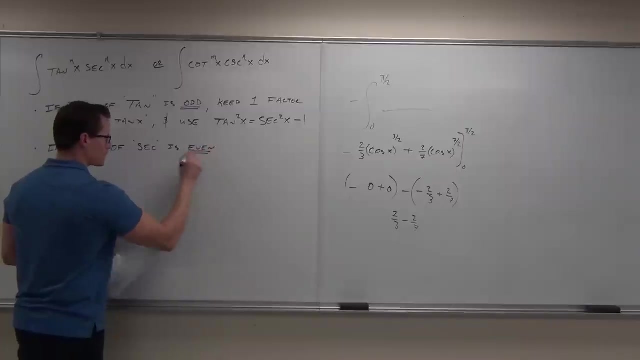 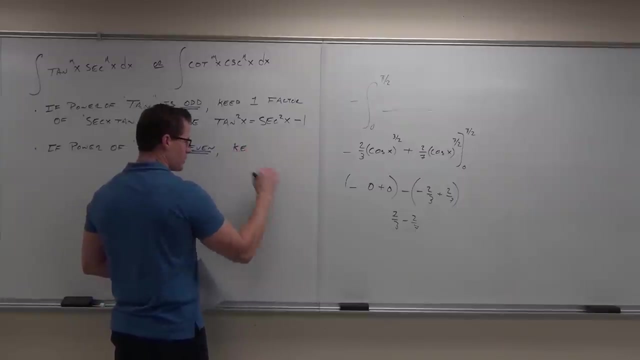 Then if it's not, We're going to. We're going to check secant. Let's say, the power of secant is even. The power of secant is even What we're going to do is we're going to keep or strip off a secant squared. 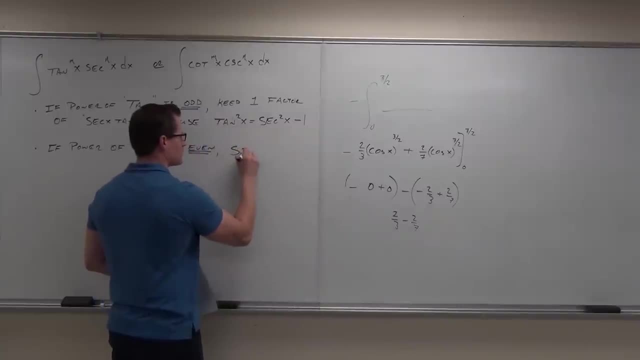 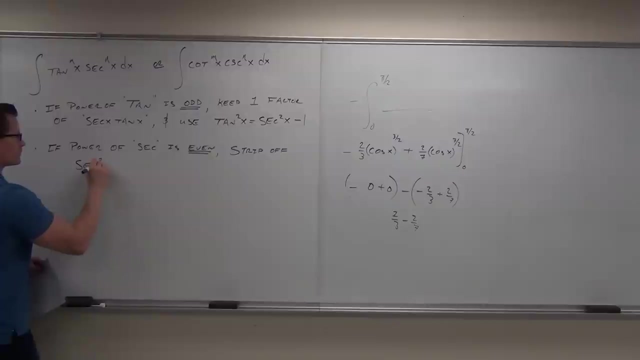 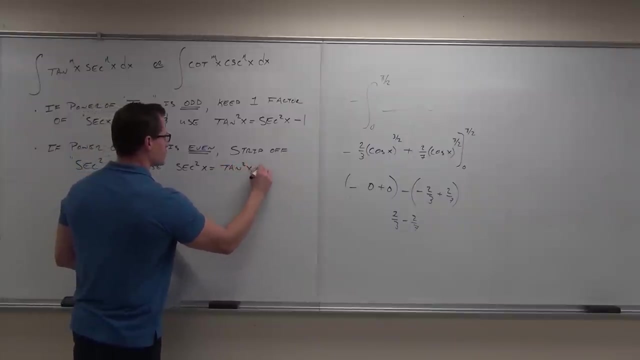 And then we're going to keep or strip off a secant squared And we're going to use secant squared X equals And use secant squared X equals. See what will that be? Tangent squared X plus 1.. If this is the case, 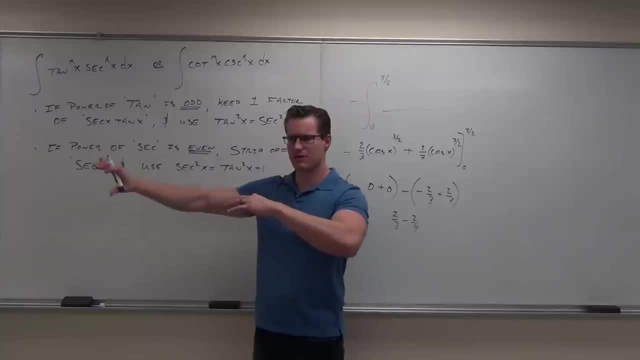 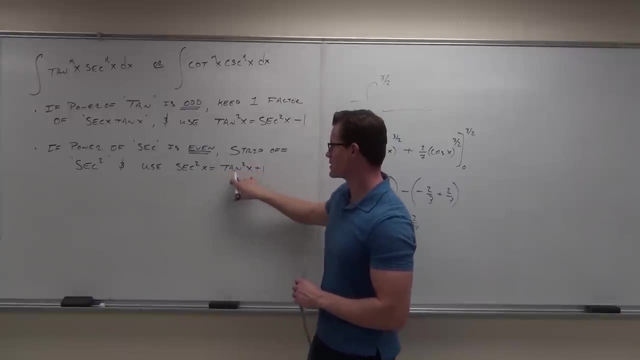 If we have an even power of secant, Well then we can do is strip off the even, the rest of the even, And keep a secant squared. If we keep a secant squared and use this to translate everything else into tangent, 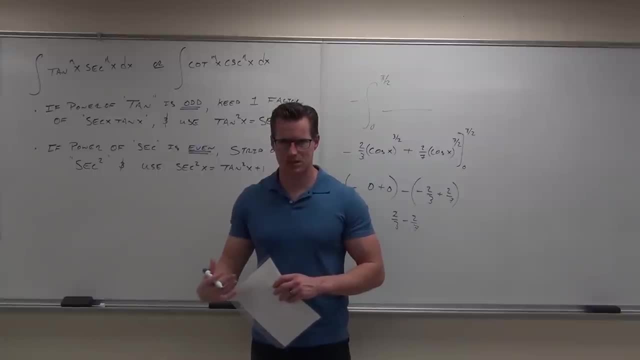 hey, tell me something. What's the derivative of tangent Secant squared? That's going to allow us to make a substitution. Tell you what I want to try, at least one of these right now, just to get it in our heads real quick. so this stuff makes sense, okay. 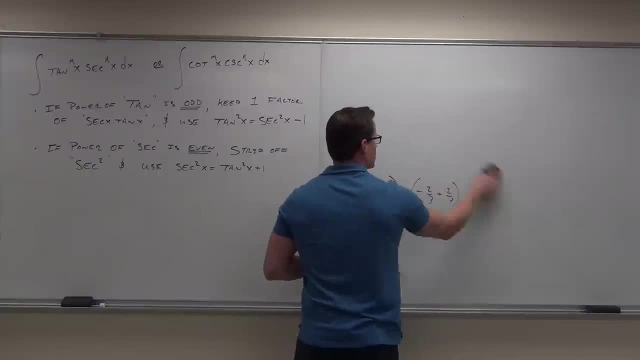 So you'll find a lot of similar patterns to sine and cosine. Same idea. It should be a little bit easier now that we have this stuff down. Question: Oh, so those two definitions, those work for either both of those, cotangent or cosecant too. 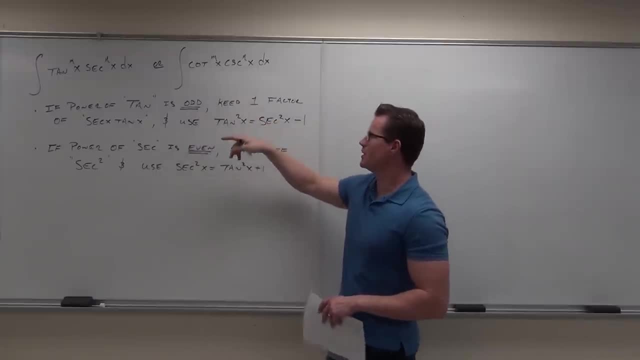 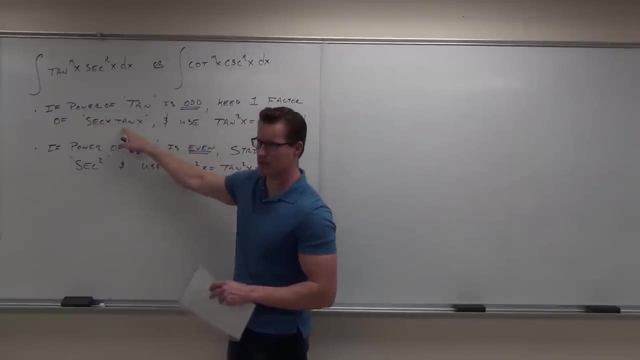 That's right. So if- and I'm kind of putting this up here for this one too- You could read it this way: If the power of cotangent is odd, keep one factor of cosecant cotangent and use: cotangent squared equals cosecant minus one. 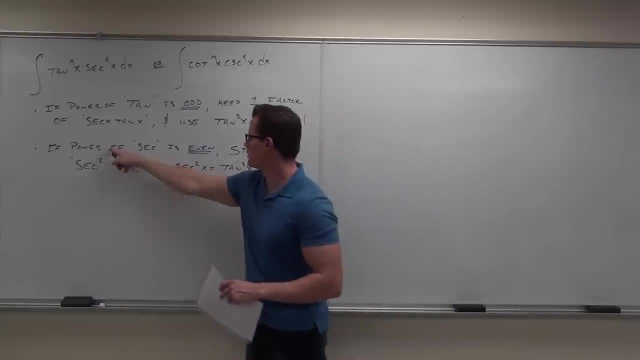 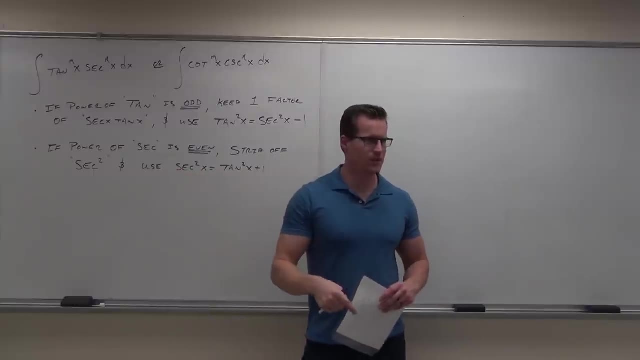 You'd use that one. Does that make sense to you If the power of cosecant is even? strip off cosecant squared and use the appropriate identity, Okay, Okay. So make sure your identities are good to go and we'll be absolutely fine. 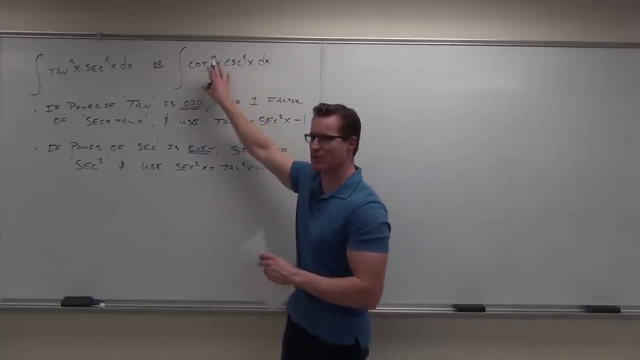 Very similar ideas here, which is why I'm not going over this one completely separate. They're the same, it's the same thing. Let's try one. I'll give you one in a while too, but let's try one with tangent and secant first. 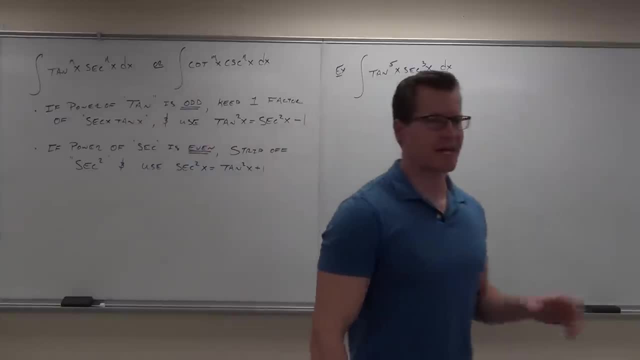 All right, let's go through the whole process here. We're going to look at the power of tangent first, And if it fits our paradigm we're good to go. If it doesn't, well then we've got to look at the power of secant. 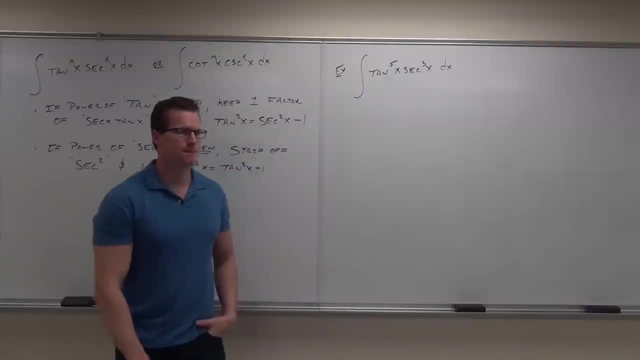 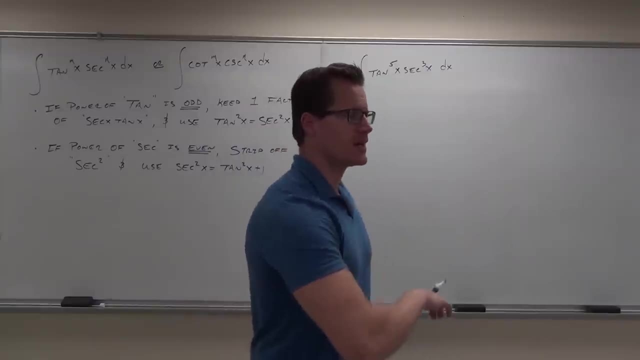 So let's look at the power of tangent. What do you notice about it? It's odd, It's odd And that's great. That fits right here. So what we do with the odd power of tangent? we're going to make it even. 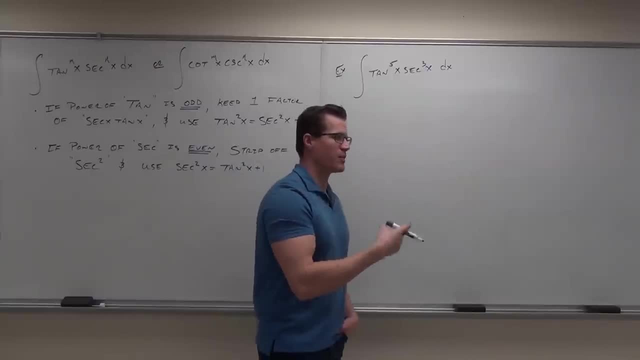 We're going to strip off a power of tangent, but we're also going to strip off a power of secant. So what am I going to write as far as the tangent goes? Tangent to the fourth, Yep, Tangent to the fourth. 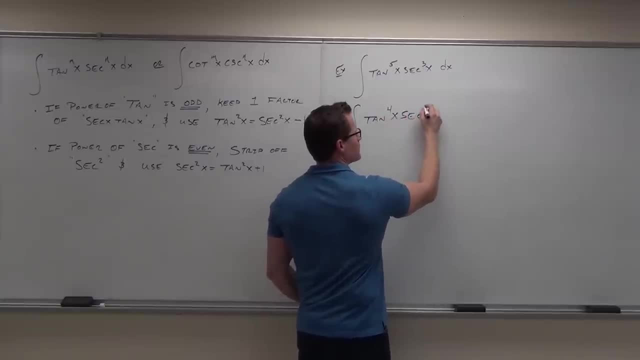 Tangent to the fourth And I'm also going to do- I'm going to do- secant to the Secant. Now, here's what we're going to do with that. We just stripped off the tangent. We just stripped off the secant. 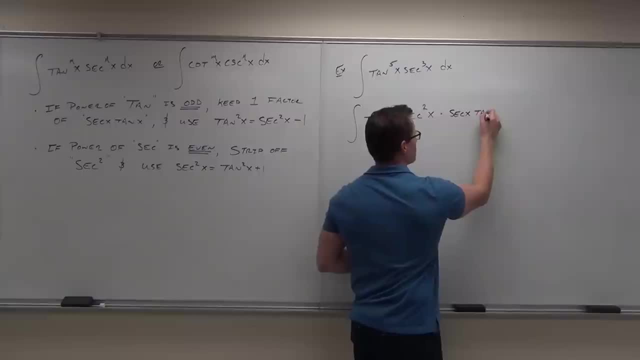 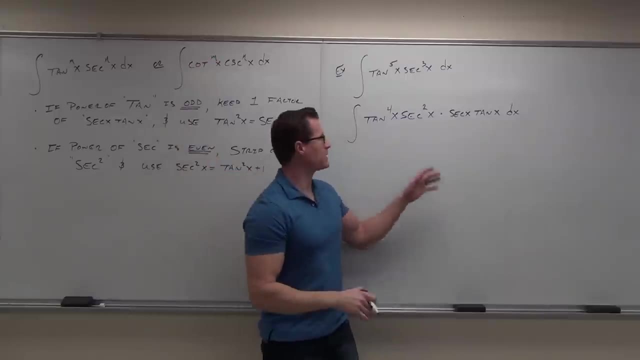 I'm going to have secant x, tangent x, dx. I want to make sure that you guys are all with us. so far, Where do you have your? Okay, we're done. It's just some algebra. It's just understanding that this is the same thing. 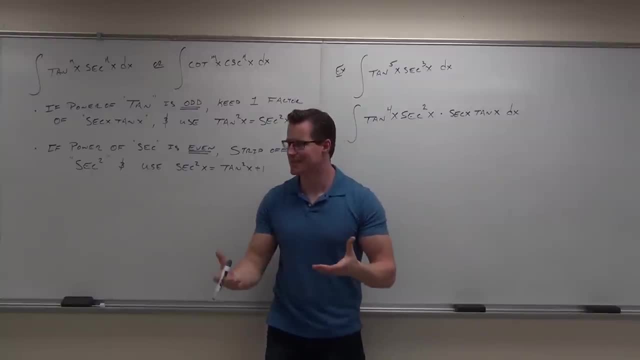 I'm just doing this on purpose, because right now I'm working to make a substitution. That's the idea. Now do I want to change secant squared? No, No, Some of you might be thinking: wait a minute, That's even. 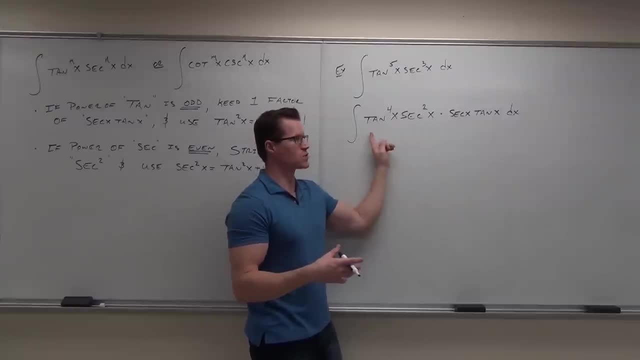 Should I do that? No, The idea here is: you're trying to make this so your substitution has this derivative. This is the derivative I want. If I change this to a tangent, I'd have a substitution of a tangent. What's the derivative of tangent? 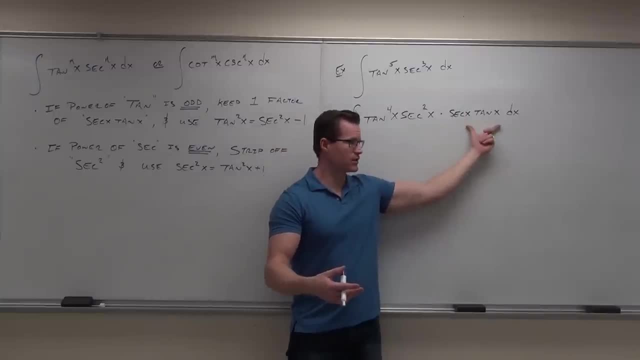 Secant. Is it this? No, If I change this to a secant, what's the derivative of a secant, Secant This? That's why we're going to go about it this way. Okay, This Not so much. 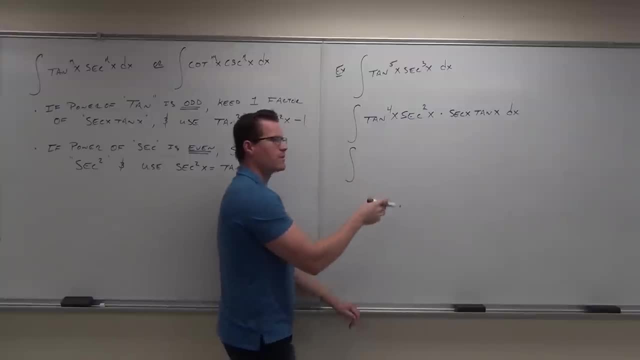 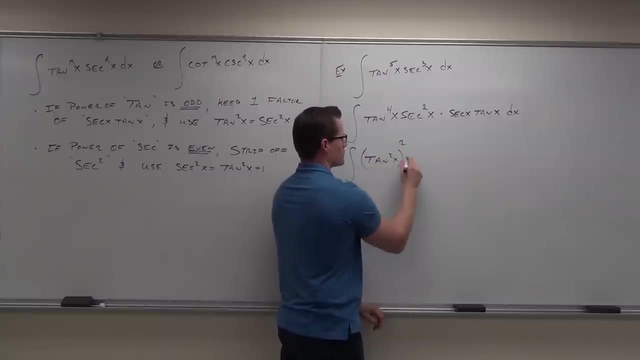 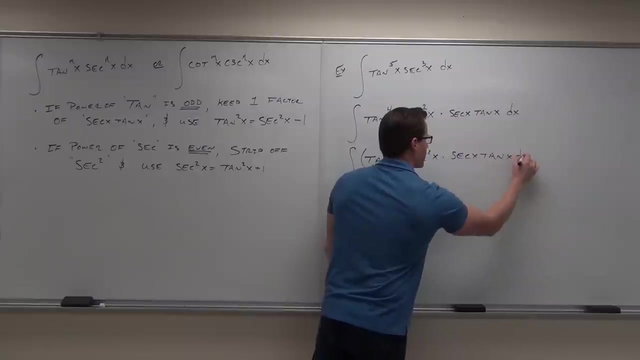 Maybe we manipulate the tangent a little bit. I don't want tan to the fourth. I want to make it look like my identity here, So I'm going to do a tan squared x squared. So the whole idea is identify what identity you're going to be using. 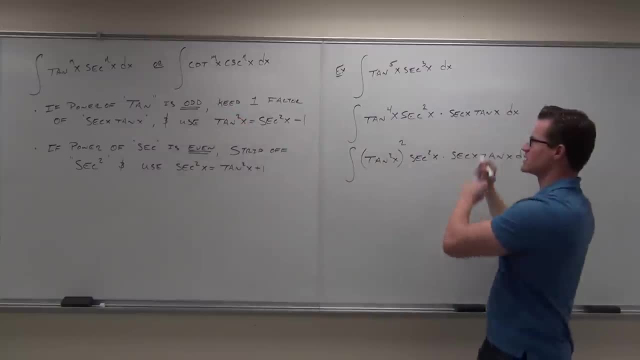 Then use it. If we have an odd power of tangent- strip off a tangent and a secant- Then make your tangent into a secant. In order to do that, we've got to have our identity, just right. So secant to the fourth. 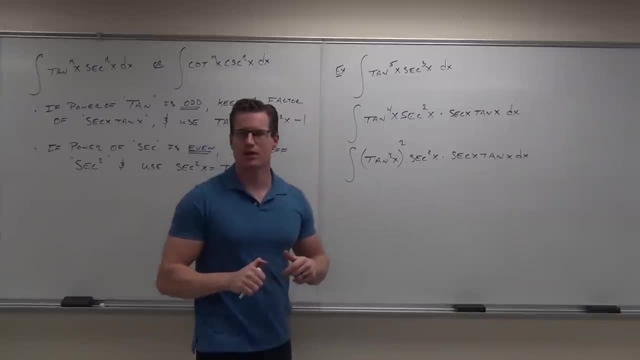 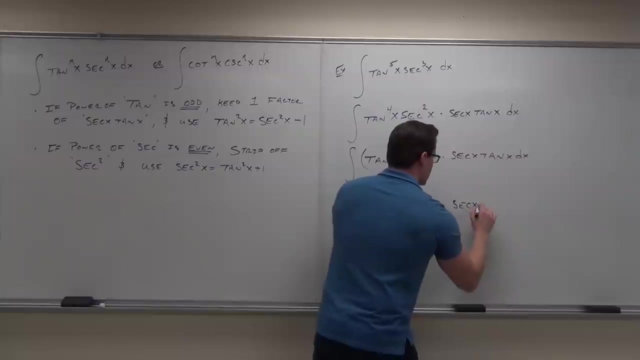 Now I'm going to do tan squared squared. How much is tan squared x? What is that? Secant squared minus one? So we're going to have secant squared x minus one all squared. Then a secant squared x times a secant x, tangent x, dx. 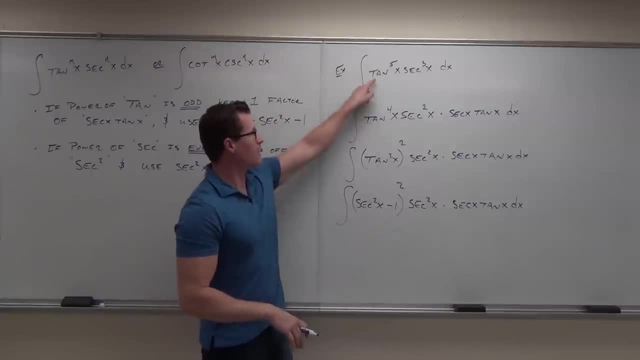 So ten second recap before we actually go on and do this thing. Are you guys okay with the idea that if tangent is odd, we're stripping off a secant, A secant tangent? Yeah, This is because we're going to work towards making a substitution. 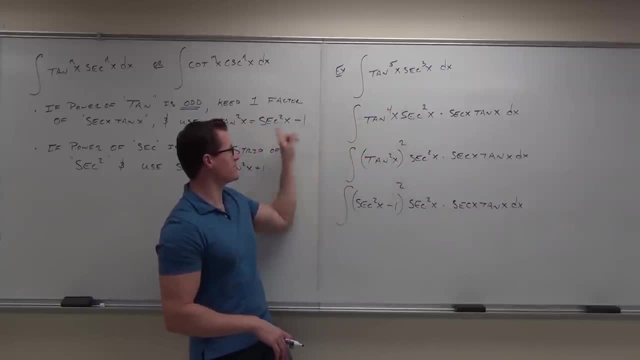 We do that by making it look like it fits the identity, doing the identity and then doing a very simple substitution. If we do our simple substitution, u equals what Secant squared x. Don't distribute now. Please don't do that. 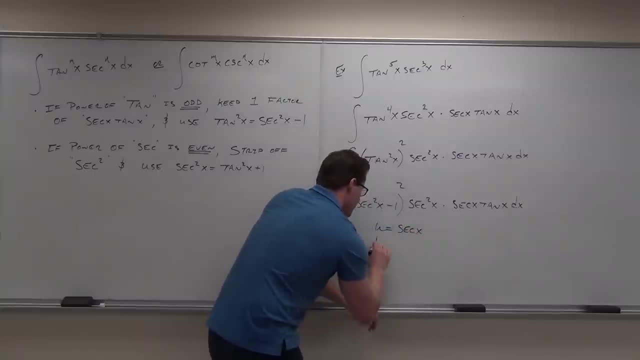 You'll have to do it later. U equals secant x. Do you equal what's? do you equal Secant x, Secant x? This, ladies and gentlemen, is why this works. When you strip off the secant x, tangent x, you're actually stripping it off, so that 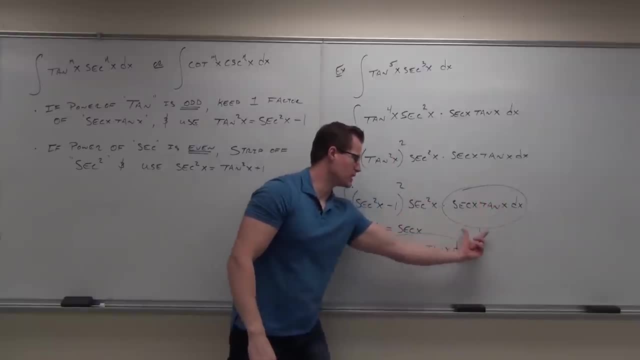 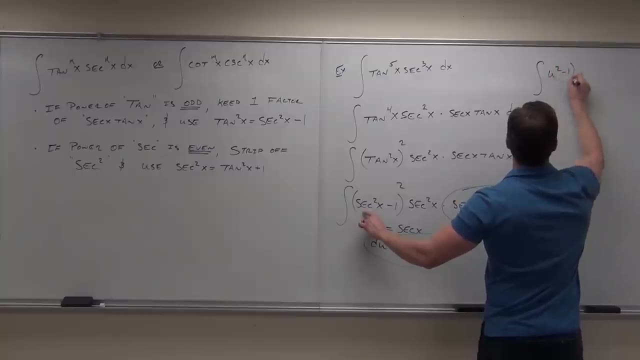 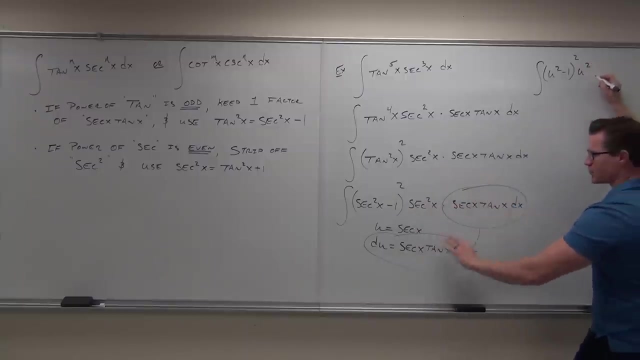 you can do this so that secant x, tangent x, dx will equal your du. You'll change this to a u. u squared minus one squared. You'll change this to a u. But this whole piece- why we stripped it off- was to allow this to happen. 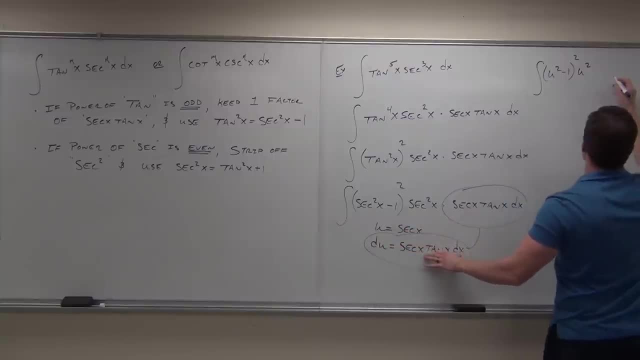 The derivative of the secant x Is this: Therefore, du equals secant x, tangent x, dx. I want to show it. if that makes sense to you, you can follow that What I want. it's very simple after this. 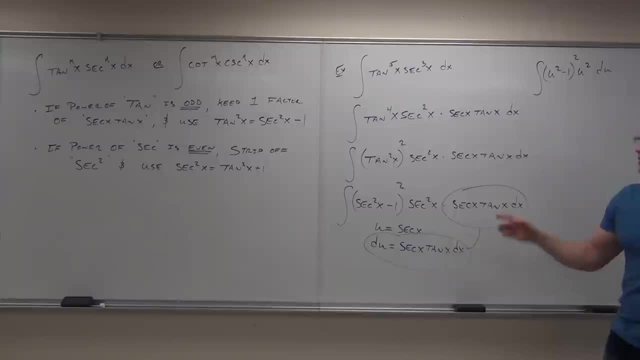 What would you do? Foil And then distribute everything. That's right. So distribute all this crap, Distribute everything And then do your integral. Go ahead and do that at home. It'll take us maybe a minute next time we come in. 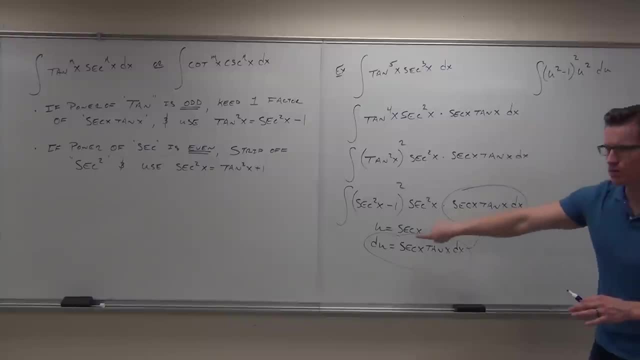 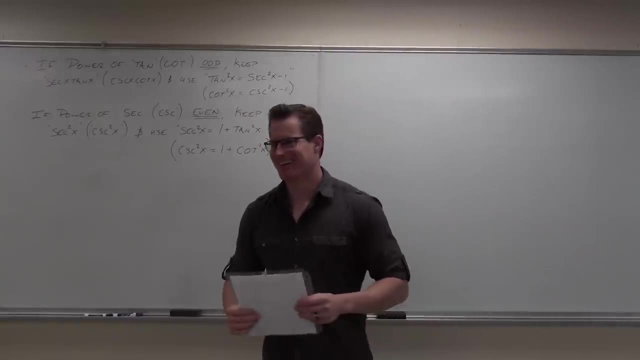 Just make sure, at the very end you're going to have to substitute back in for whatever you use. So more torture, I mean fun, Ha ha ha. More calculus. So what we've learned is that if we have some integrals which follow some trigonometric patterns, 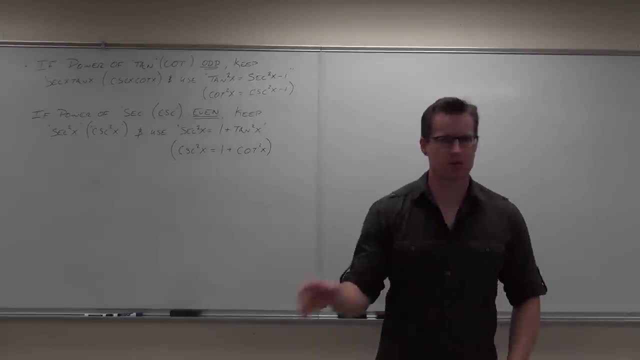 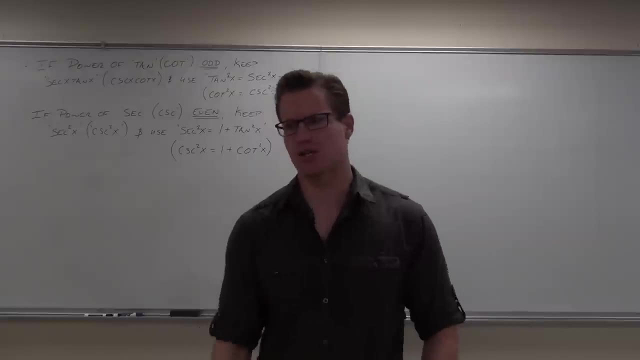 Such as we have sine and cosine, where sine is odd or cosine is odd, Or they're both odd or they're both even. We can do stuff with that. We can work with them with following the patterns that I've given you earlier in this section. 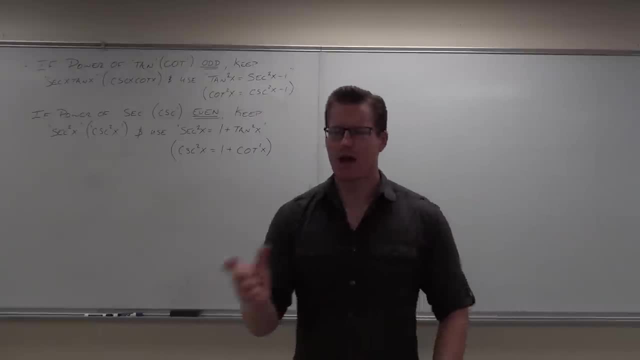 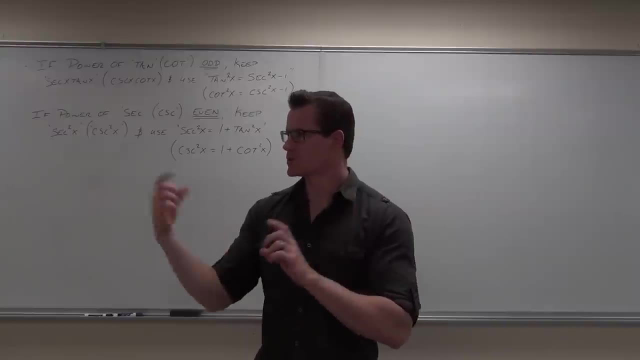 We're also moving on to what happens when we have tangents and secants. Of course, we use sine and cosine together, Because the derivative of one gives you the other. That's why they work. We use tangent and secant together because the derivative of one kind of gives you the other. 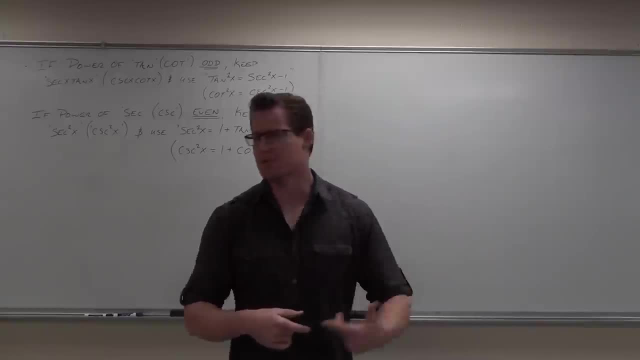 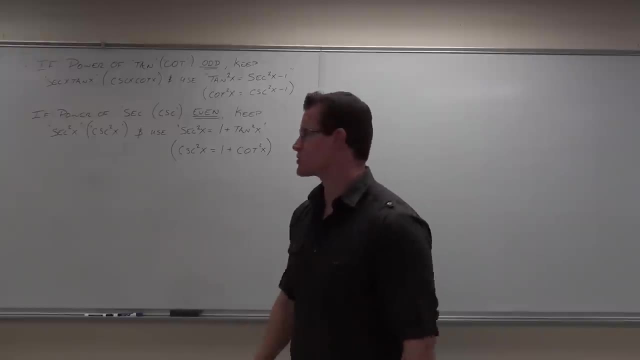 They're related as far as their derivative is. So what that means is we can use substitutions a lot of the time if we do a little manipulation. Same thing works with cotangent and cosecant. So here's the ideas. If you have a power of tangent or cotangent, that is odd. 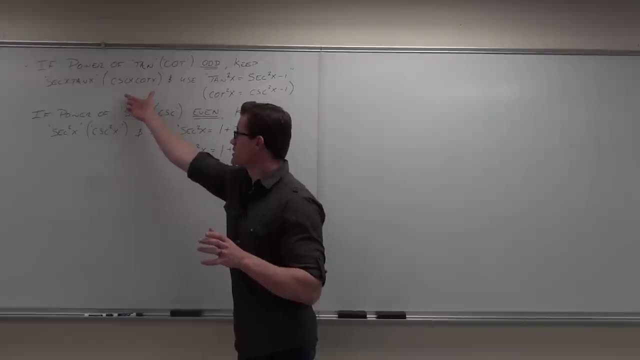 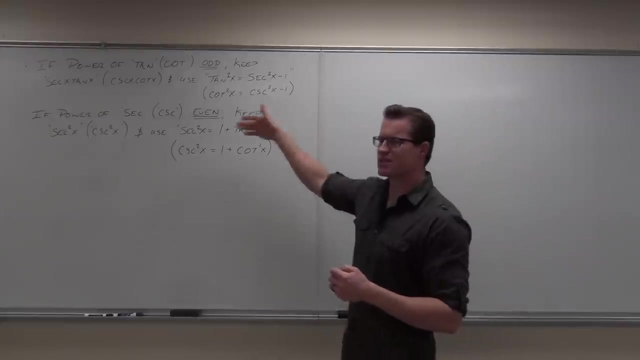 we're going to keep a secant tangent or likewise a cosecant cotangent and use tangent squared equals secant squared minus one or cotangent squared equals cosecant squared minus one. Do you guys see the similarity between the cos and the other functions? 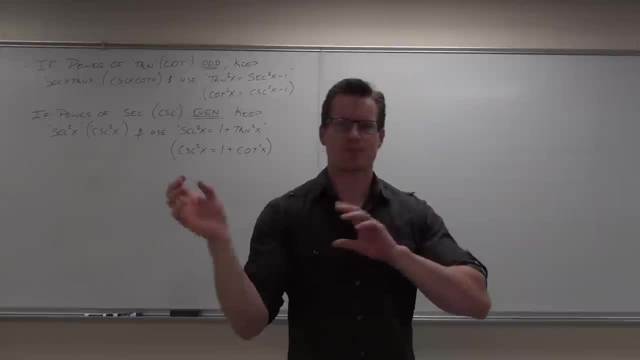 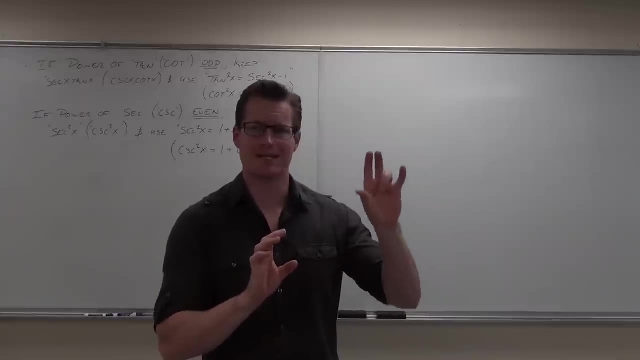 It's very similar. Again, the idea is this: You're stripping off a piece because you're going to be doing a substitution, So basically we're stripping off the derivative of what we're trying to get in our integral. So if we strip off- look at this- if we strip off a secant tangent, 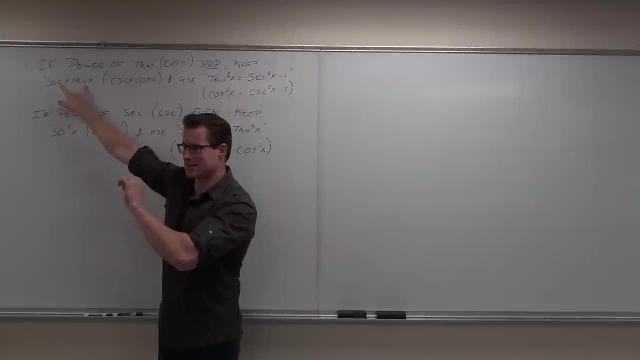 we better be substituting and making everything else in the integral a secant. Does that make sense? I'll say that again: Does that make sense? I'm sorry if you guys weren't really listening here. If we're stripping off a secant tangent, everything else in our integral better change to a secant. 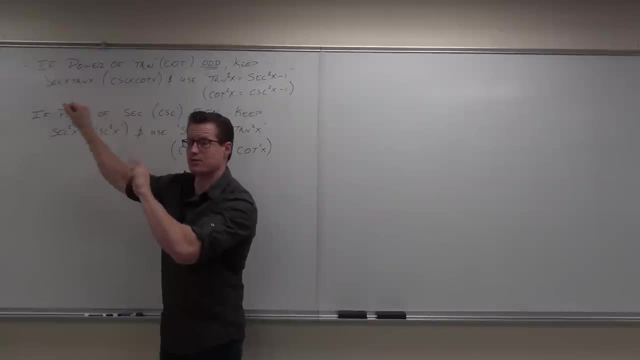 because the derivative of a secant is secant tangent. This is what we're doing: We're stripping off the derivative. If we strip off a secant squared, if we keep that one, then everything else in our integral better be changing. to what? 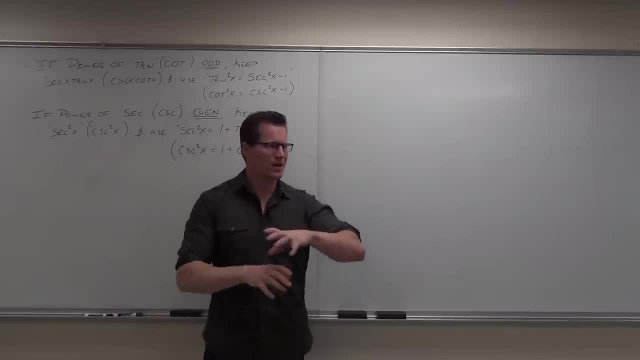 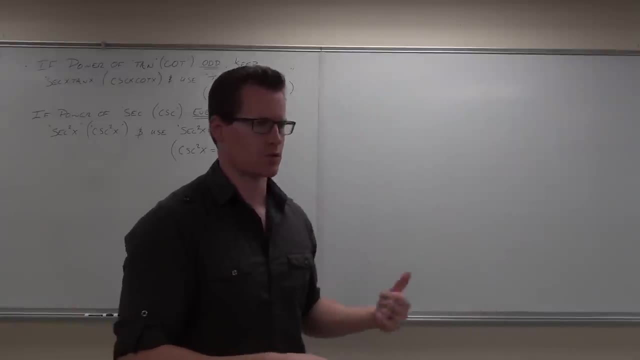 Tangent. Tangent because the derivative of tangent is secant squared. So we're kind of taking a piece of this away of our integral, just stripping it off a little bit. That way we can make a substitution that allows us to do our integral just a basic use substitution. 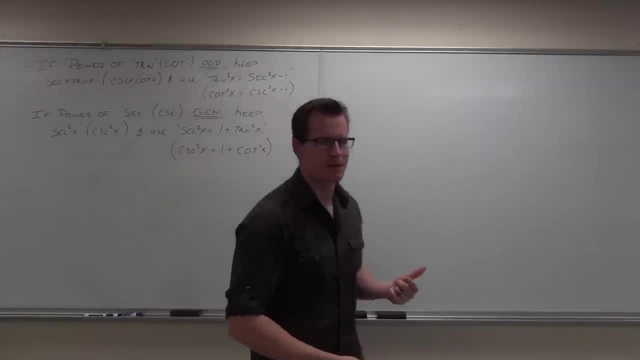 I want to try one more with tangent and secant. show you what that idea is like. I think last time we did one where tangent was odd. I haven't shown you one where secant is. even so, we're going to do that. 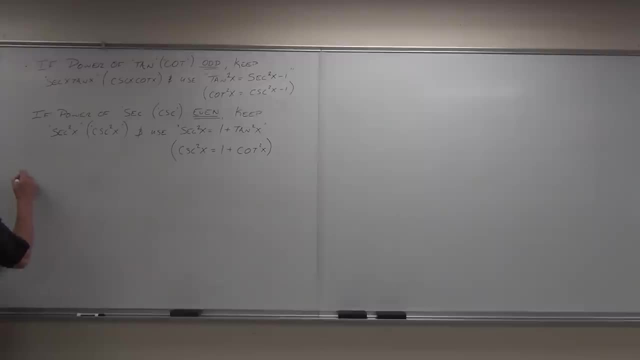 So here we go. Let's suppose we have an integral from zero to five or four. Let's suppose we have an integral from zero to five or four of the square root of tan x times secant to the 6th power of x. 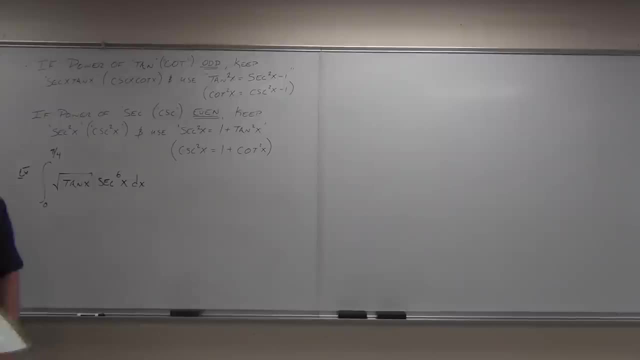 Secant x to the 6th power. Let's see if this follows one of our patterns. see if it fits. So what would this fit as? Would this fit as sine and cosine? Of course not. we don't have those. 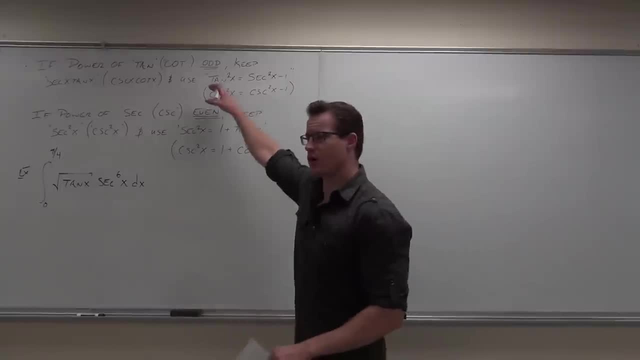 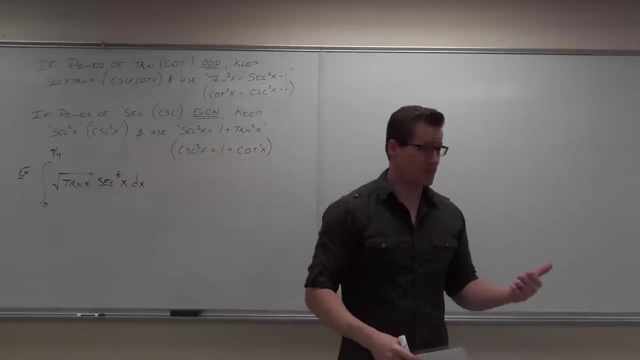 As far as tangent and secant goes, what does this fit? Is tangent, odd or secant? even Which one, I don't care if they're both. even we have one or the other. Either tangent's got to be odd for us or secant's got to be even. 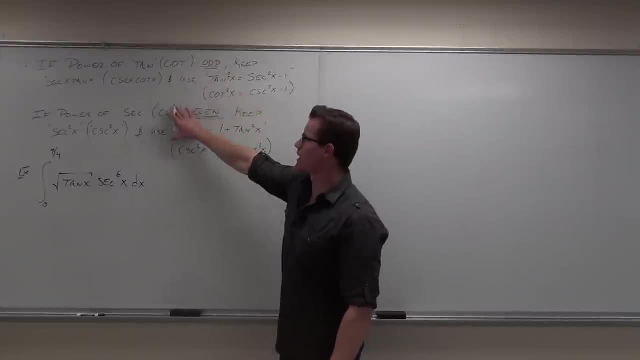 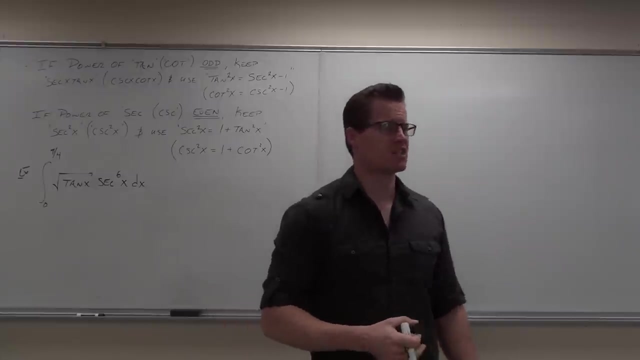 Which one do we have? Okay, so we don't fall up here, we're falling right here. The power of secant is even No problem. Well then, we can do this. What are we supposed to do if the power of secant is even? 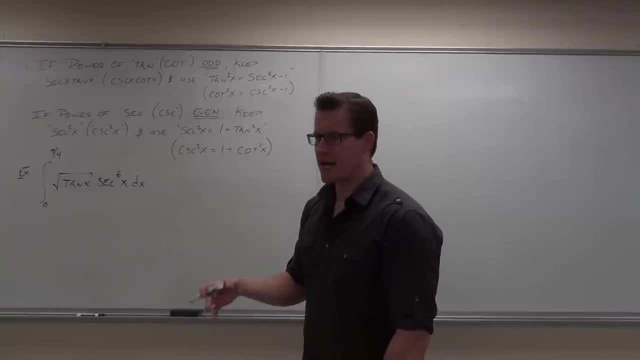 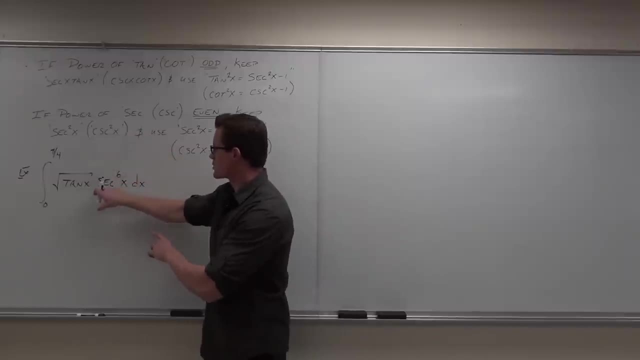 We're going to strip off a secant squared. So basically, here's what has to happen with this: If you fit this pattern, we're going to strip off a secant squared. So this is going to become secant to the 4th. 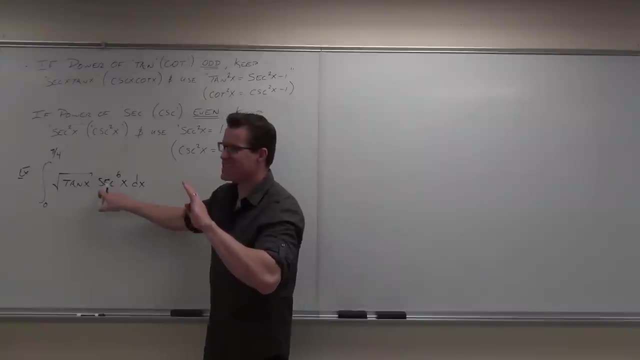 So this is going to become secant to the 4th power. are you with me? The reason why this works so nicely is because, if this is even, I can strip off that secant squared and have something that can be raised such that I have secant to the 2nd power in there. 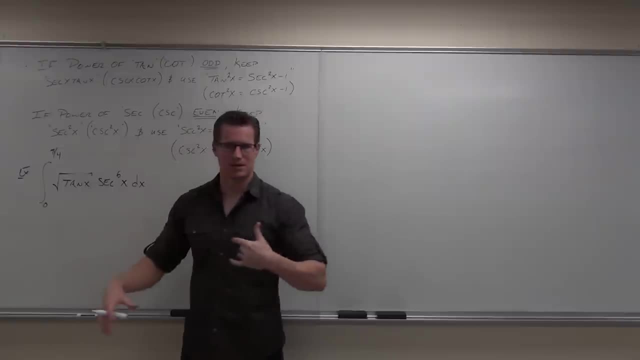 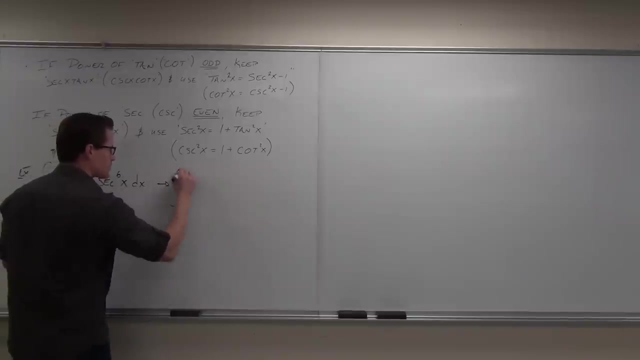 Then I can use my identity, change everything into tangents and make my substitution. So check this out. We're going to follow my ideas here. We'll have 0 to the power of 4, not really any calculus happening. We're fitting this to our pattern. 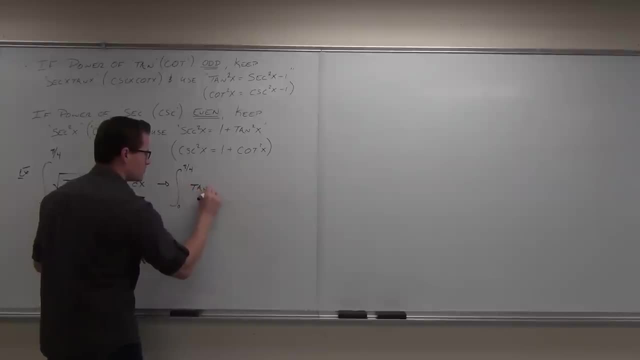 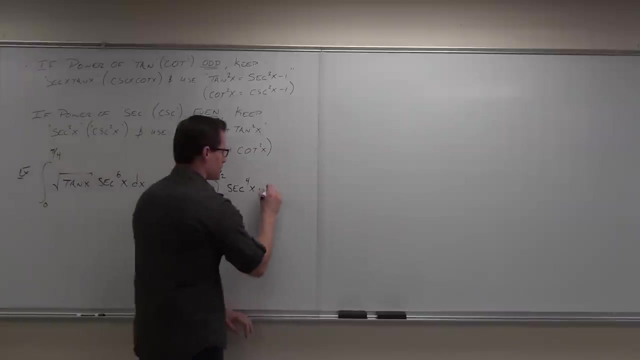 We'll have tangent to the 1 half power. We'll have secant. tell me what I should have. secant to the 4th? very good times. what Secant to the 4th? This is what I mean by stripping off a secant squared. 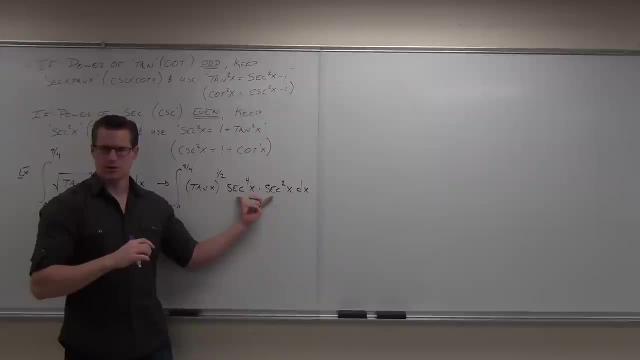 We're taking this well, is that still secant to the 6th? Of course it is. I'm stripping this off. Here's why This is the first time I know it's kind of out there when I'm just talking it through. 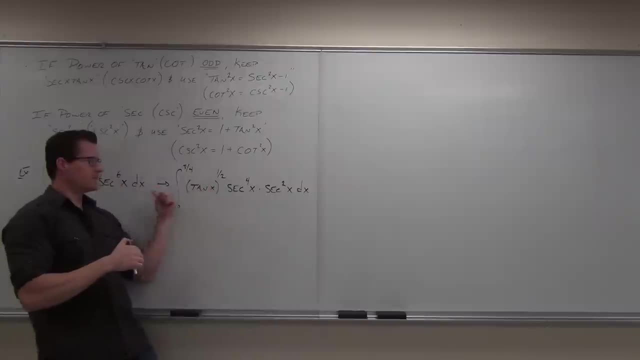 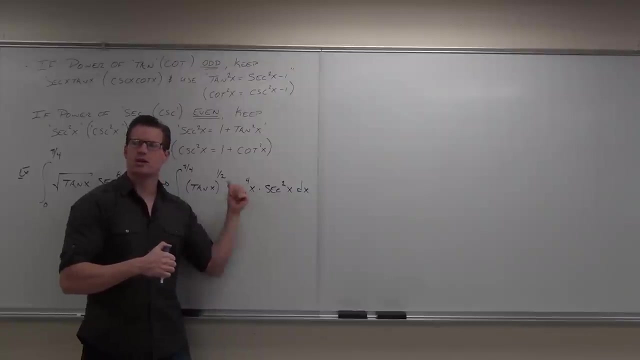 but in the example- hopefully you see this, Because this was even when I strip off that secant squared, it's still even. Does that make sense? That means I can write this as secant squared to some power. If I can write this as secant squared to some power. 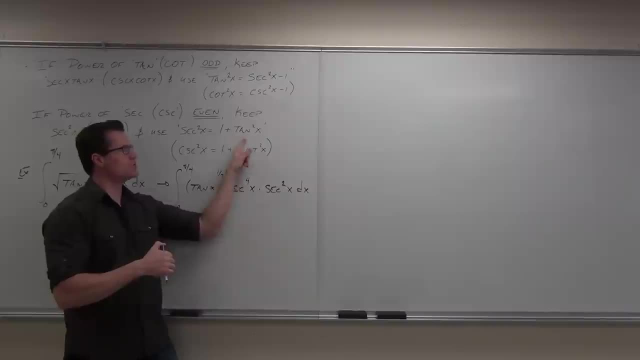 I can use this identity to change everything into tangents. This is the idea. If I have this tangent, I'm good. If I can change this to tangent, I'm good, because then the substitution: hey, what's the derivative of tangent? 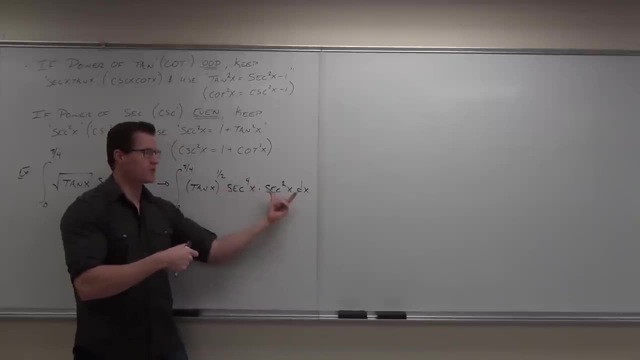 Secant squared. That's why we strip that off. So the idea is: strip off a piece, use the rest of it to change it into whatever. this one is the other trigonometric function. So if I have tangent and secant and I have a secant squared, 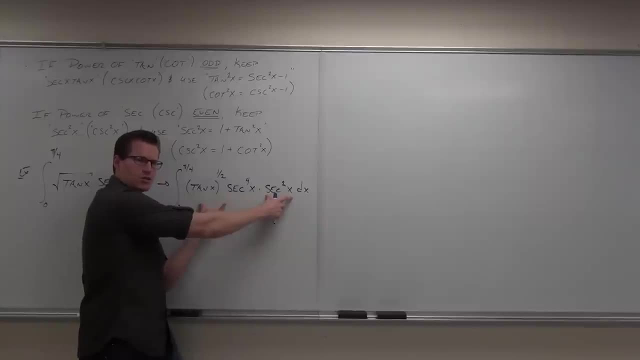 I need to change this into tangent so that my substitution will actually work. Does that make sense? You wouldn't strip this off and then do something with tangent. That'd be silly, because the derivative of secant is not secant squared. The derivative of tangent is secant squared. 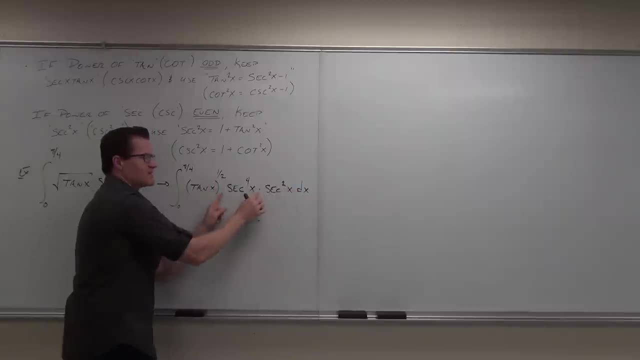 So, even good deal, We'll strip off the secant squared. It's still even. That's the point here. If it's still even, then what we can do is keep the tangent to the one-half power. That's great. 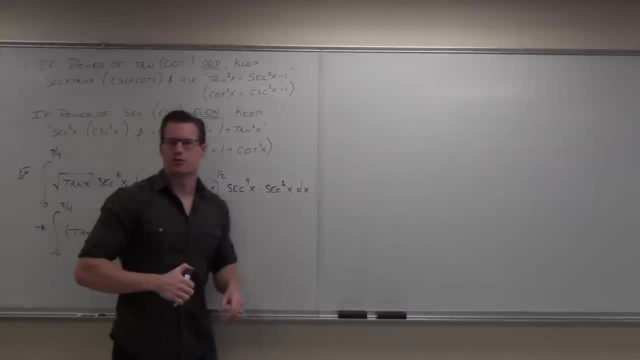 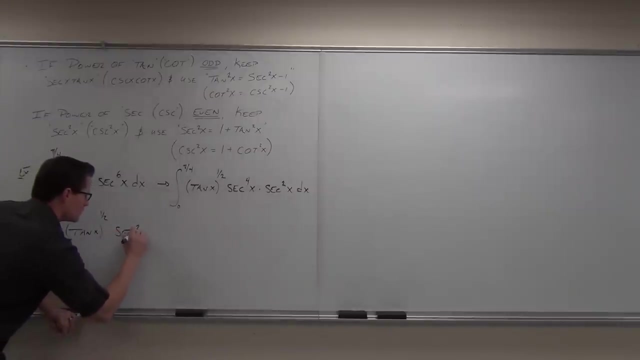 Secant to the fourth. No, no, no. How are we going to write secant to the fourth power? What do you think? Secant to the fourth power? Perfect, And we'll keep this exactly the way it is. I want to know how many people understand why I'm writing this as secant squared to the second. 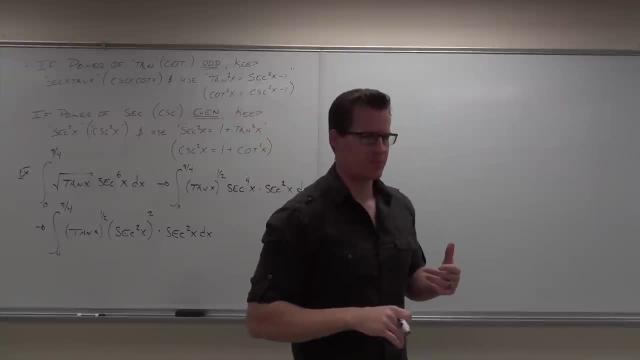 How many people understand that? Why, What's that going to allow me to do? Yeah, that's right, We're going to use our identity. So this one do I want to change that? No, This one do I want to change that. 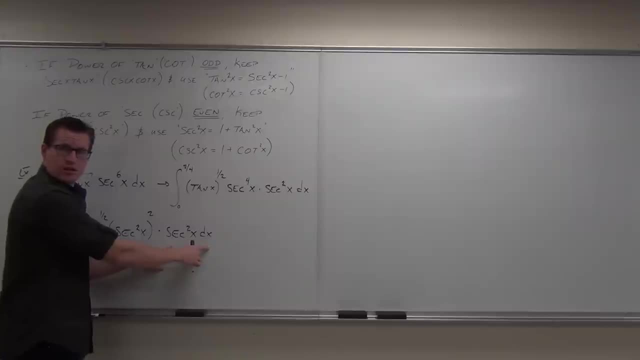 No, This one, No, No. this is going to allow me to make that substitution. Do I want to change this one? Oh yeah, Zero to pi over four. We're going to have tan x to the one-half In here. well, this is why we did this. 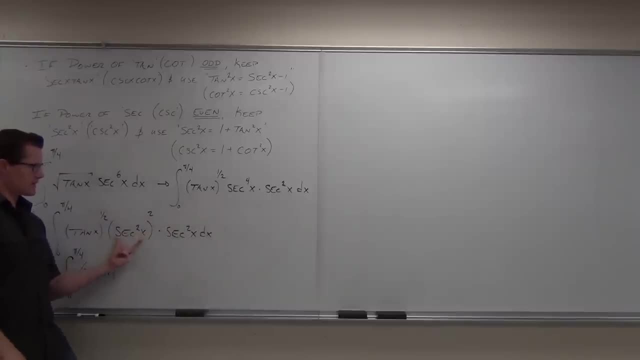 Because this was still even. I can write this as secant squared, squared. It's our secant squared, which we want, because we're going to do that change here. We're going to use this identity and it still raises some power. 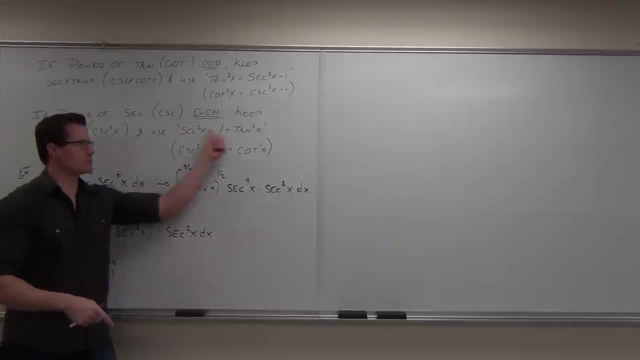 That's fine, We can deal with that, But I had to have a secant squared to be able to do this, to change everything into tangent, So this becomes one plus tangent x. Like that, All of it squared, All of it squared. 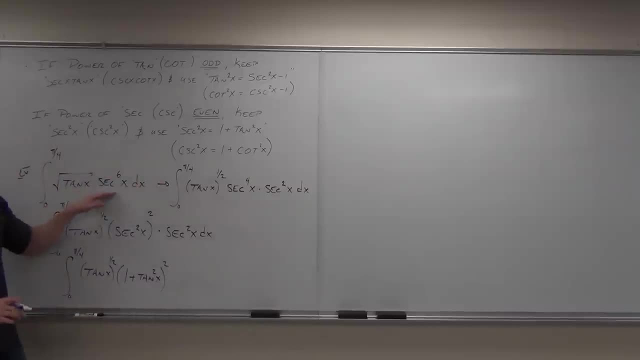 Let's see if that makes sense to you. Even Cool, strip one off, It's still even. that's why we did this. If it's still, even I can write this as secant squared to some power. If that was to the sixth power, that wouldn't be a problem. 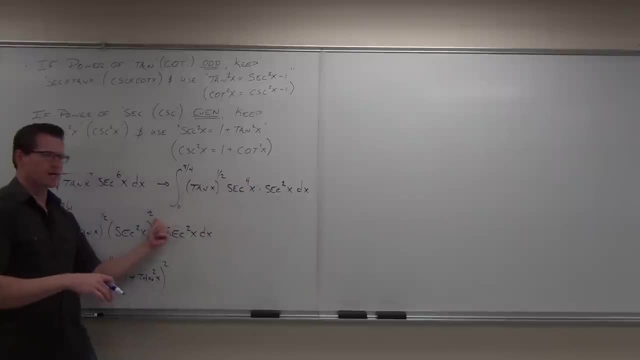 That would just be a three. If that was an eighth power, no problem, That would be just a four. The idea is, if this is even, I can strip it off. I still have something that's even, which allows me to do. 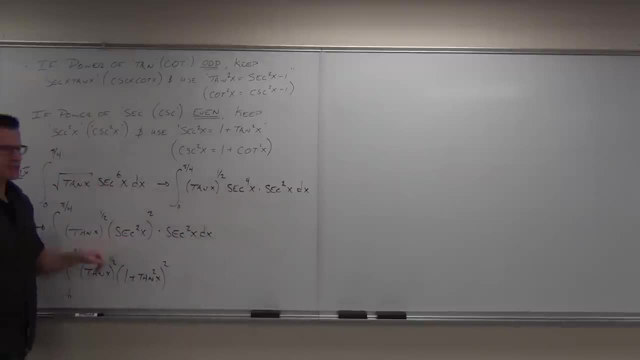 this idea. Once I have this, this secant squared now, I get to use my identity and change everything into tangent, except for this guy, because I want to use this thing for my substitution. You have to have the derivative of whatever you're going to substitute. 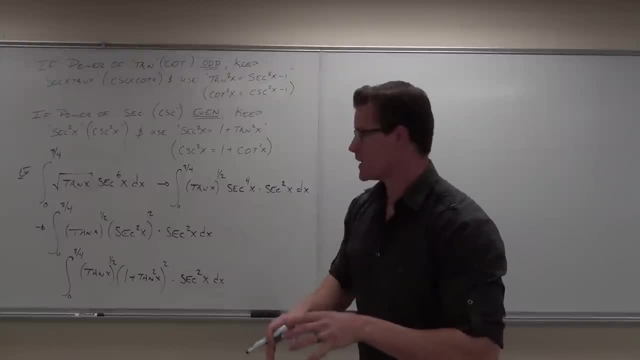 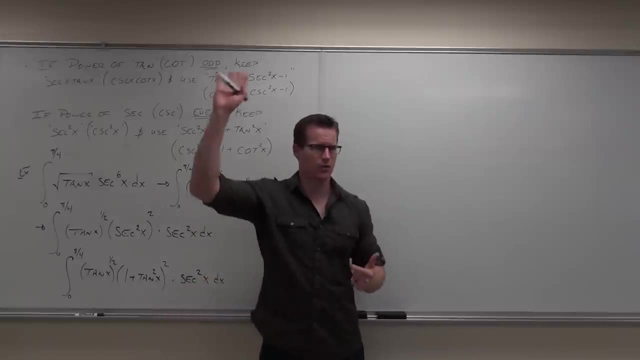 That's the basics of u-substitution- is the derivative has to be there. So if we're trying to change everything into tangent, we've got to have a secant squared, otherwise our substitution will not work. Show of hands if you feel okay with what we've done so far. 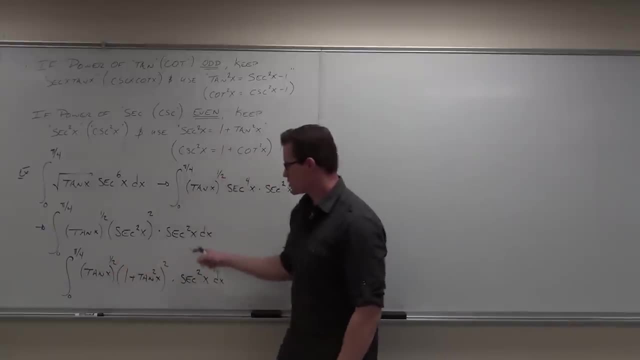 Cool Now. should I distribute right now, or should I do our substitution right now? I would, You can distribute, but there's lots of other stuff, right? So if we change everything to u now, it would be a little bit easier. 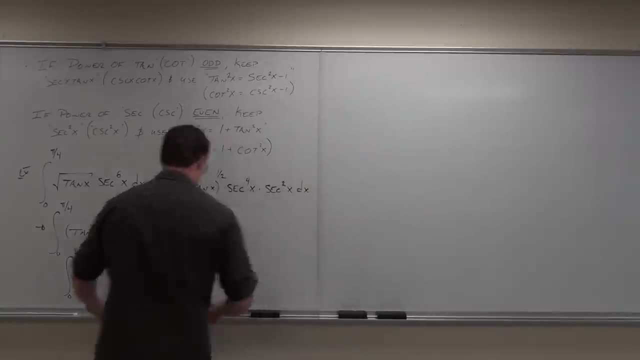 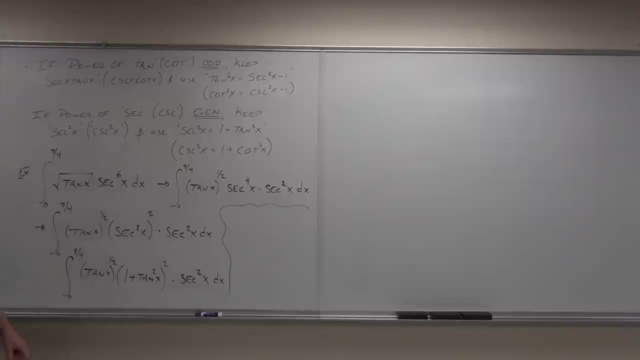 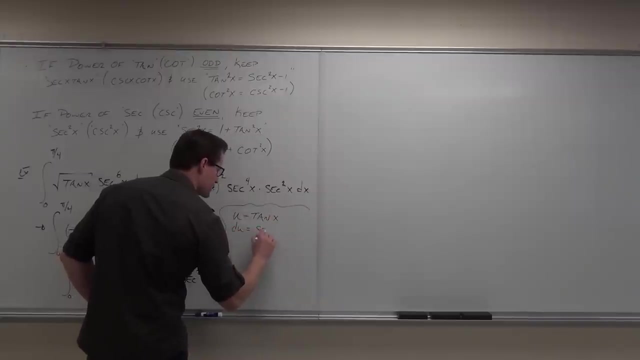 So right now we're going to do our substitution. Can you please tell me- and I'll make a little area here for this- what is our substitution going to be Then? du equals secant squared x dx. This is why we had to have this. 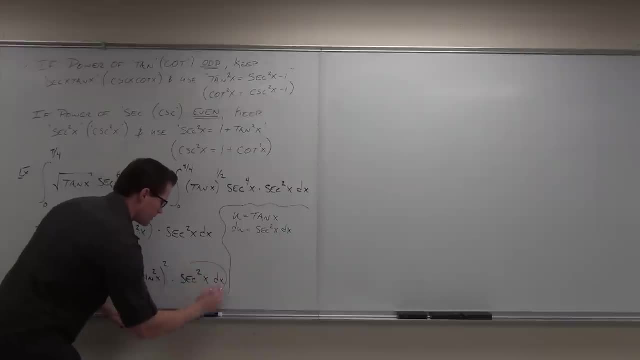 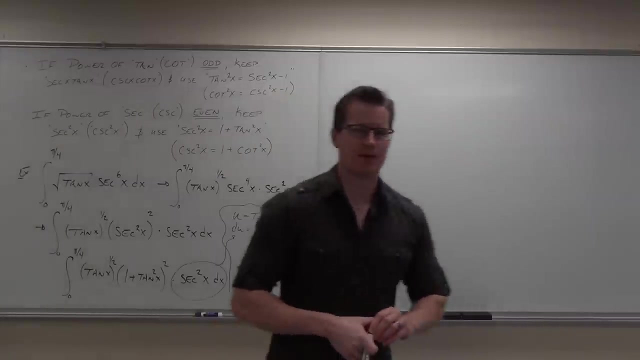 That's why this whole thing works. So now this part is equal to du. That's brilliant. One more thing I'd recommend to you right now is, if you have definite integrals- which we do here- sometimes it's really nice to change your bounds. 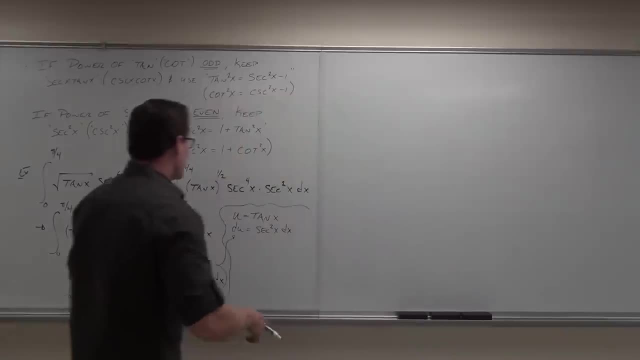 So I would do that if this was my problem, I'd be changing bounds right now, which I'm going to do. So changing bounds, I'm going to look over here- When x- And this is how I show it- I say when x is pi over 4, then u is whatever. 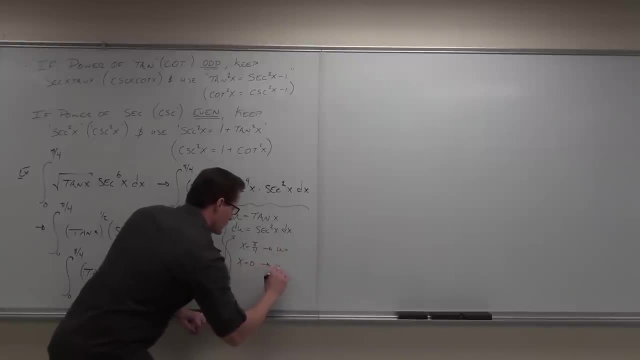 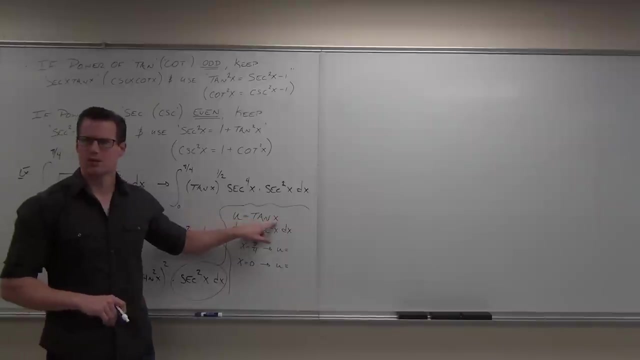 And when x is 0, then u is whatever we get. So when we do it next to our substitution, it makes a lot of sense to do that. If x is pi over 4, can you tell me what's tangent of pi over 4?? 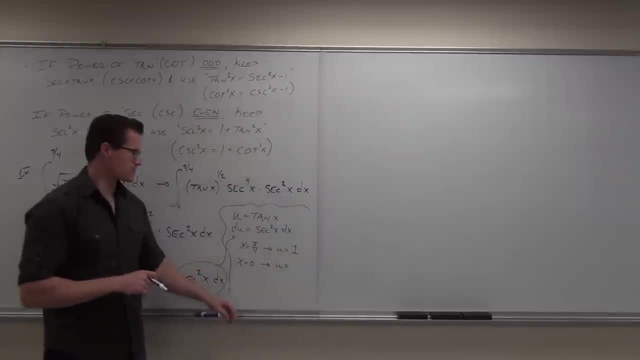 1. Then u is 1.. Right there, that's already a little bit nicer. When x is 0, how much is tangent of 0? 0.. Now what happens? this is Calculus 1 stuff, but I'm going to make it simple. 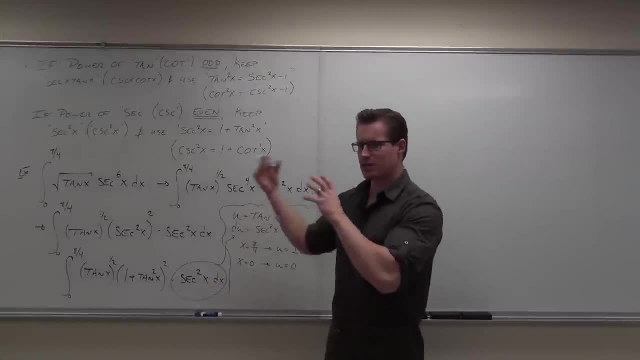 I'm going to make sure you get it. Now that we've changed bounds, when we get down to the integral, will we be resubstituting tan x for u? No, But you've changed bounds, You don't need to do that. 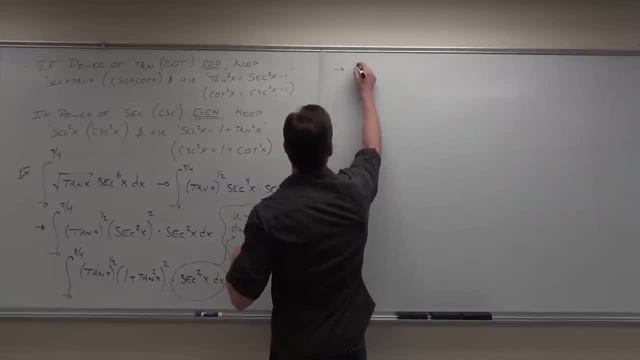 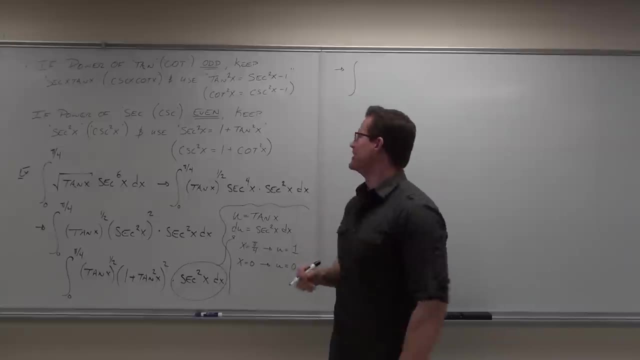 That's why I do it now. So let's see what happens. Why don't you tell me Bless you, Don't tell me bless you. I said bless you to him, But you tell me I love to be blessed. Bless you too. 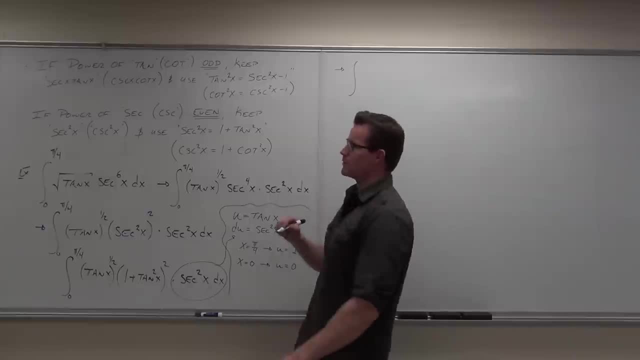 You tell me what I'm going to write. What's my integral now? 1 to 0 to 1.. Which one? 1 to 0 or 0 to 1? 1 on top, 0 to 1.. 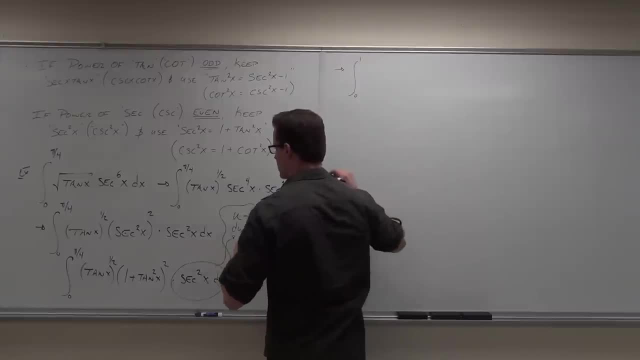 So 0 to 1.. 0 to 1.. Okay, what's inside? u squared. u to the what 1 half? Perfect, yeah, u to the 1 half. And then what 1 plus u squared. 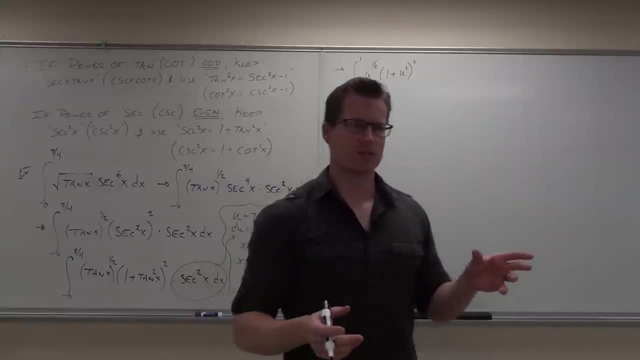 We really want to make sure we don't miss any of those powers, because that would really blow this thing out of the water. So we have u to the 1 half. We got it, Tangent is u. So u to the 1 half. 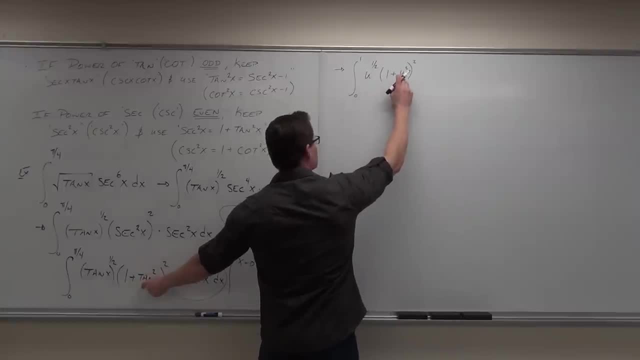 We've got a 1.. We've got a 1.. We've got a plus. We've got a plus. We've got a tangent squared. So u squared, Whole thing being squared. What happens to my secant squared x dx. 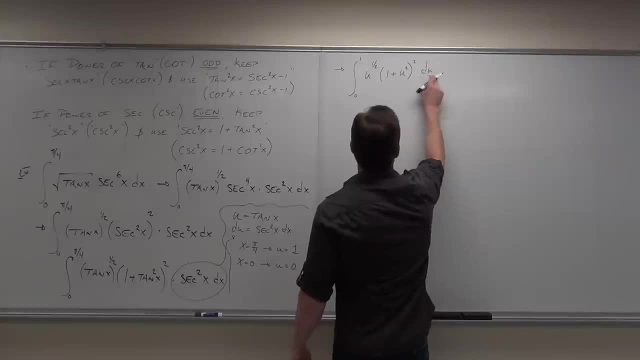 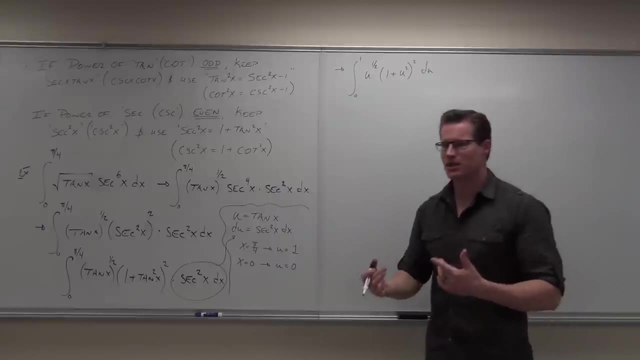 What does that do? This has to match your variable. It does. We're good to go. Can you guys do the rest of it from here? Yeah, Go for it. Do your simple integral. You're going to be distributing a lot of course. 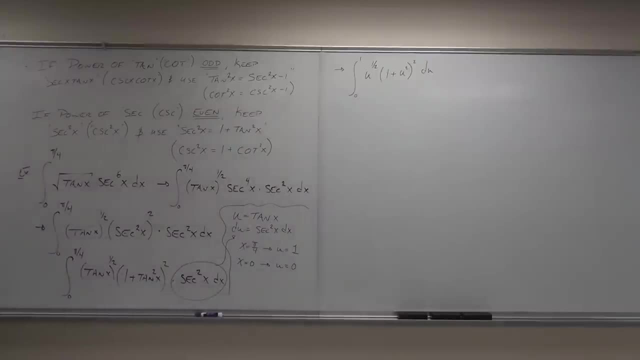 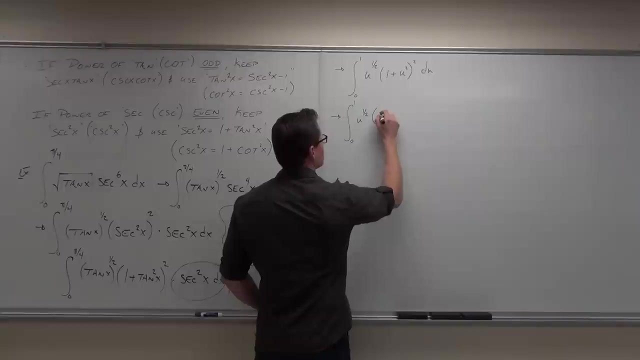 And then evaluate it. Let's see if you guys get to work on it on your own. Let's see if you guys get the same thing I get. So u to the 1 half. Let's see if 2 plus 1 half. 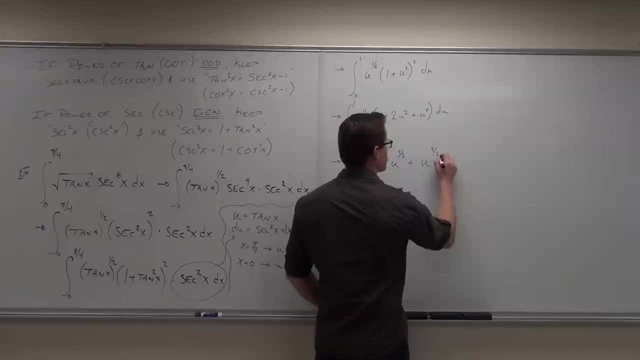 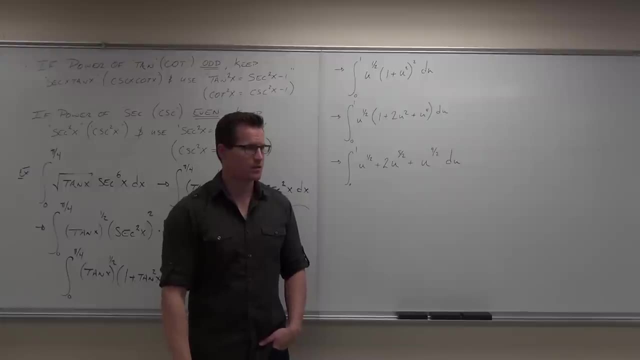 Let's see if it's going to be 8. 9 halves. Let me get a work check from you. Did you distribute the same that I did? Did you get the same thing I did? Yes, Good Fractions, Use your calculator if you have to. 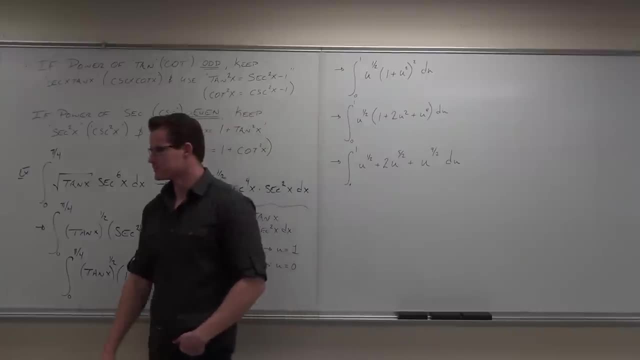 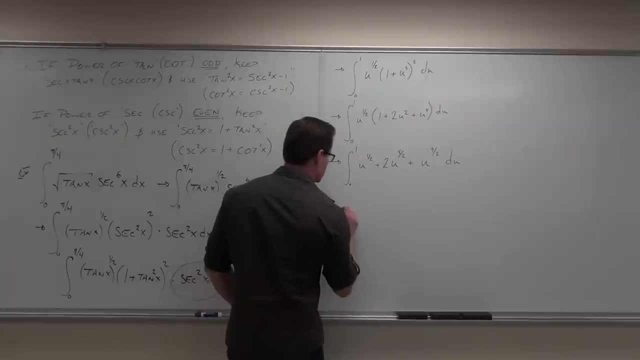 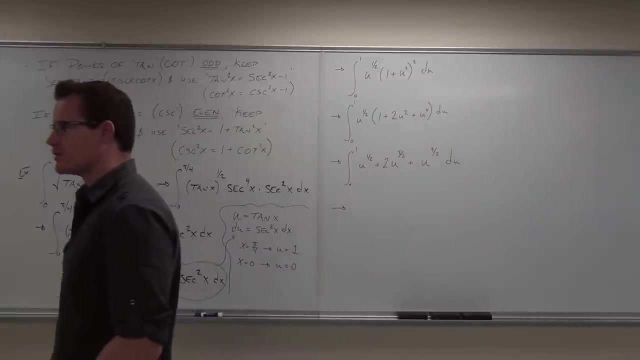 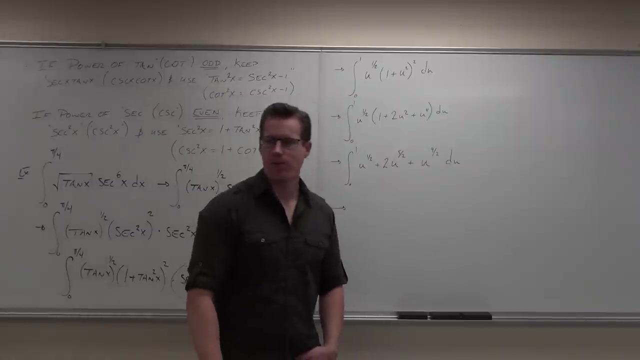 I hope that you don't, But make sure your fractions are correct. Keep on working. Are your fractions right? You got 1 half, 5 halves, 9 halves, I hope All right. All right, Who has the same thing you just got to work on? 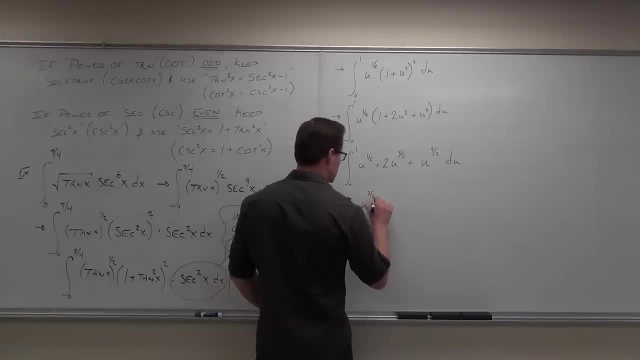 Let's see if you guys get it. Yeah, Go for it. Good, All right, We're going to do a work. check on the 35.. This is the same. Don't forget the 5 halves. Yeah, Goodbye. 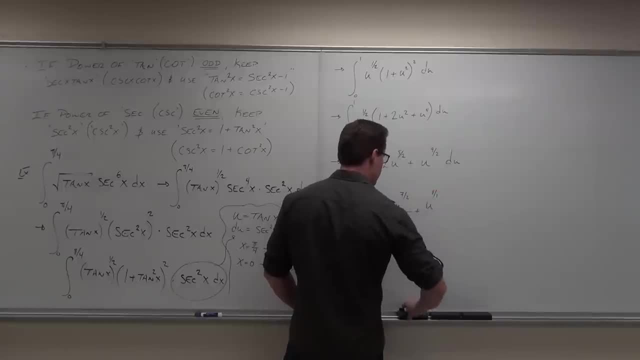 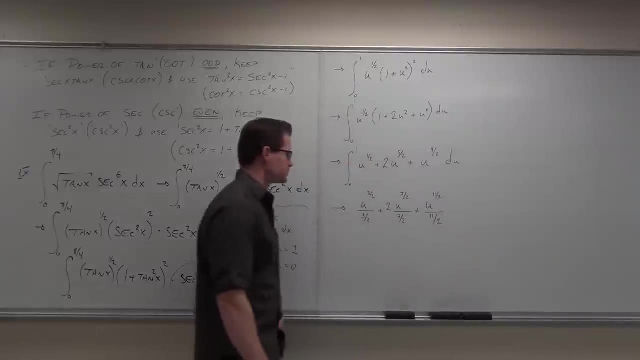 Bye, Bye, Bye-bye, Bye, Bye-bye, Bye-bye, Bye-bye, Bye-bye, Bye-bye. You know what the hard part is? The hard part is really getting down to here, right, It's using this stuff. 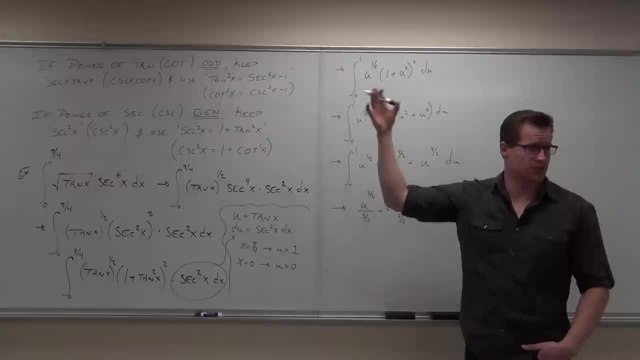 This I'm hoping you guys are okay with. This is old stuff. This is just distribution, making sure you know how to do fractions, adding fractions and then doing some basic basic integrals. U to the 1 half. integral of u to the 1 half is u to the 3 halves over 3 halves. 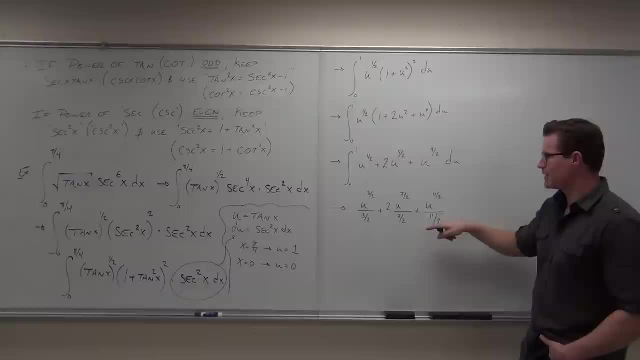 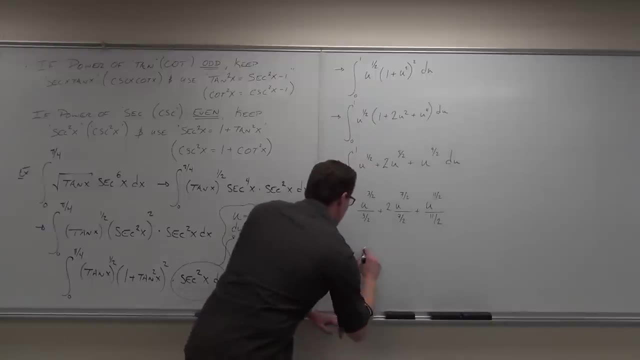 2? u to the 7 halves over 7 halves. u to the 11 halves over 11 halves, And then all of these bottom denominators just move up to the numerator. So in our case we would have 2 thirds? u to the 3 halves plus 4 sevenths? u to the 7 halves. 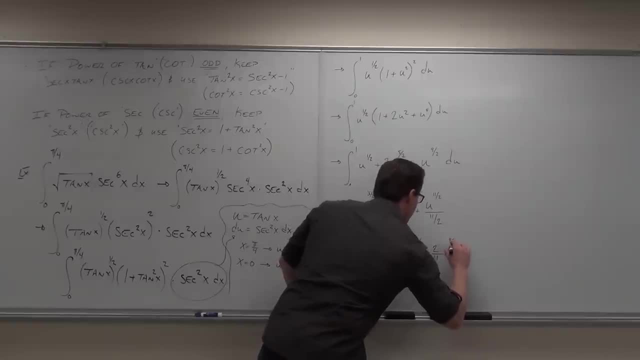 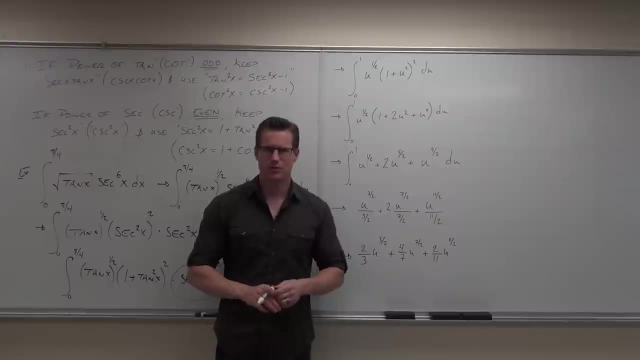 plus 2 elevenths? u to the 11 halves: 2 moves up. 2 moves up gets multiplied by 2, 2 moves up. No big deal. Quick hit note, if you're okay with that one so far. 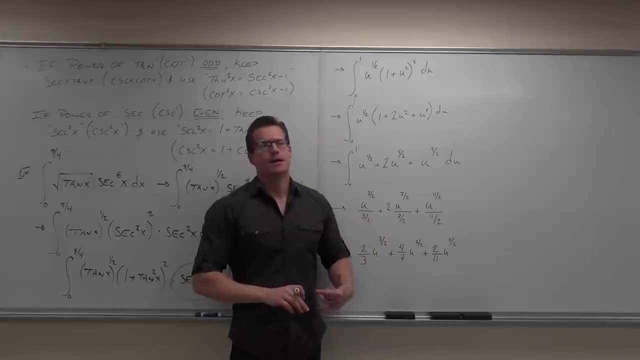 Okay now, this is what I was talking about earlier. I want to make sure that you get it. Do you, at this point, have to substitute back in your tan? If you didn't change bounds, would you have to plug in your tangent here? 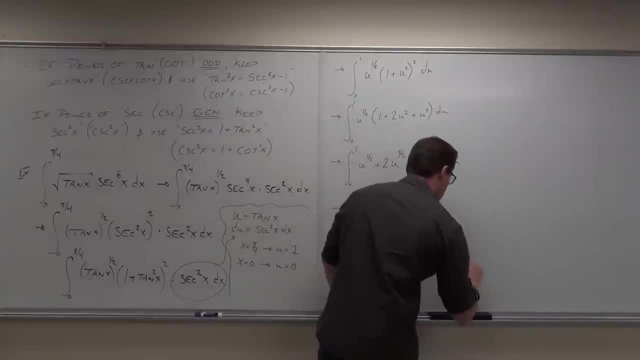 Okay, so what are our bounds of integration? Where are we going to again? So we're going to plug in 1,, we're going to plug in 0,, we're going to do it right to our u's. That makes it look kind of nice. 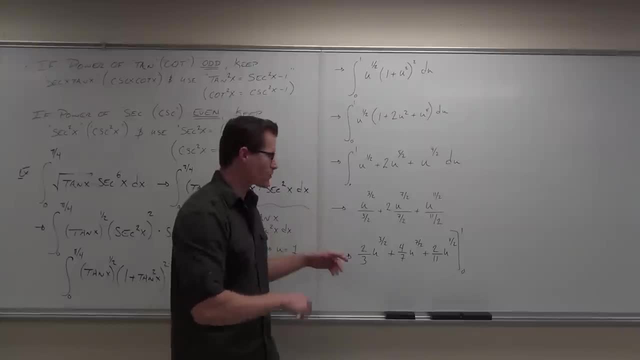 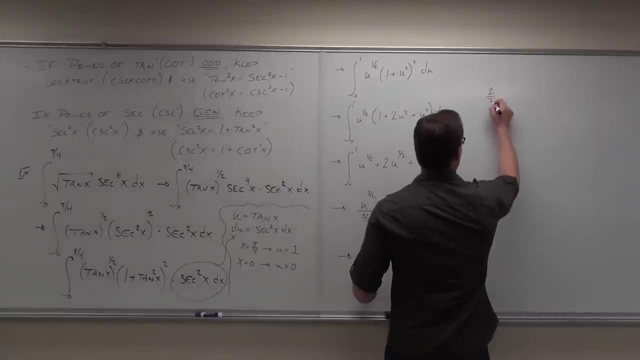 So I'm going to do this in my head because we have some fairly simple numbers. This was nice for us. If I plug in 1,, 1 to any power gives you 1.. So basically we get 2 thirds, 2 thirds plus 4 sevenths. 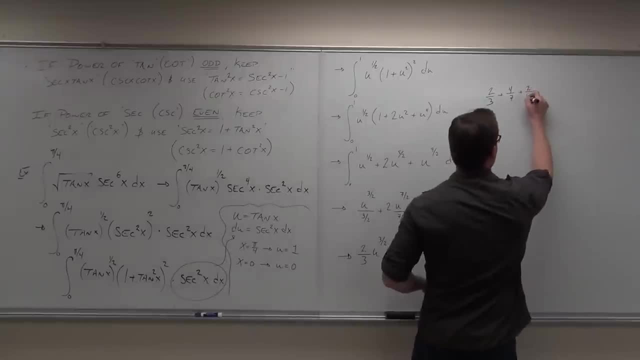 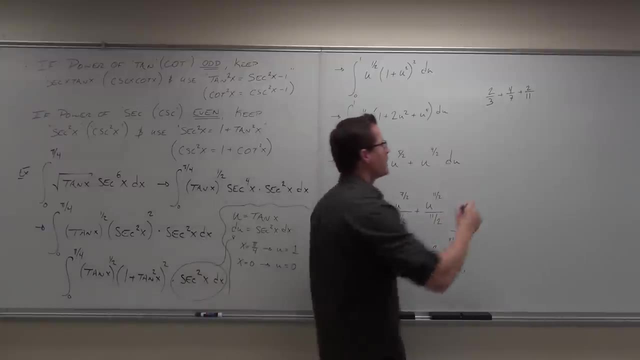 Plus 2. elevenths: If I plug in 0, I'm going to get 0 and 0 and 0, but I really want to check that and make sure you're checking that. So this will be minus 0.. 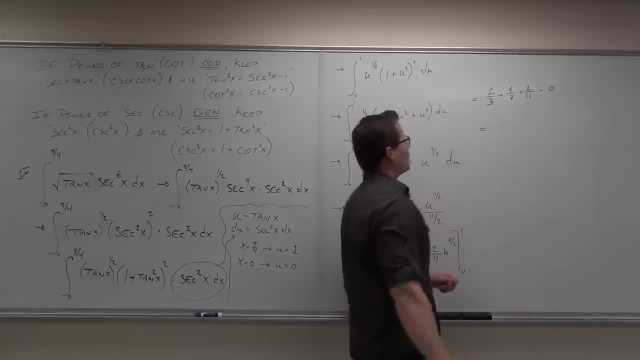 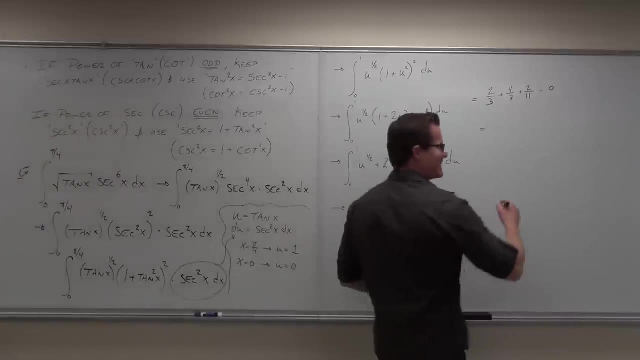 So, essentially, we just got to add up all of these fractions, which of course you can do in your head, and get 328 over 231.. I mean easy? Yeah, I'm joking. Obviously, I did that in my head. 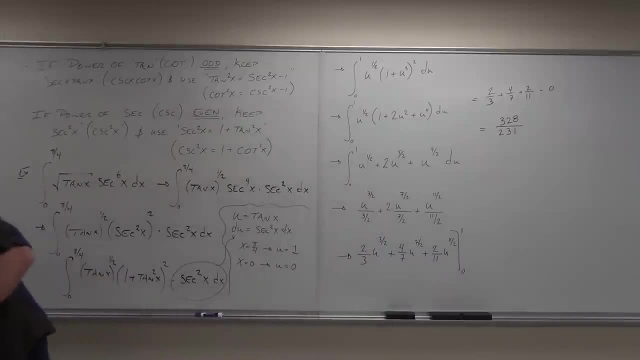 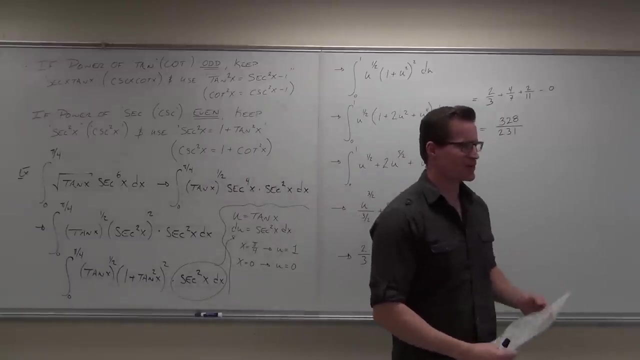 I didn't do that. I didn't do that in my head. I'm not going to waste some time adding fractions right now. I had that done beforehand. So 328 over 231 is what you would get if you added up all those things together. 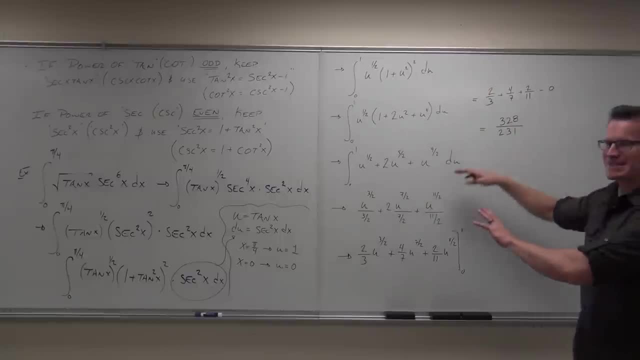 So you'll probably be okay with this one. I'm not going to waste time doing the basic stuff. This is really it, right? This is the stuff you guys should know already. So hopefully we're okay, Are we okay? You want to do one more? 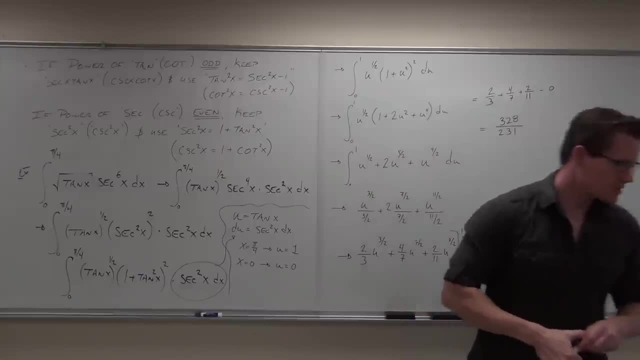 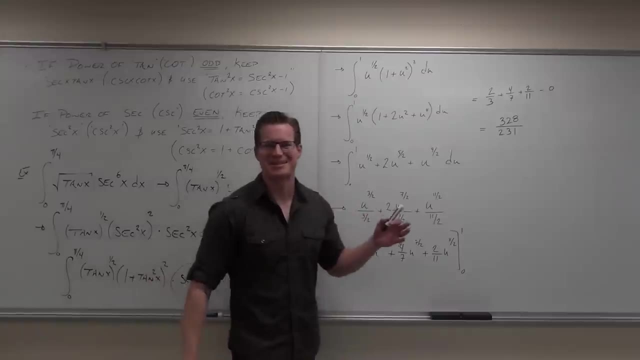 I don't think we've done a cotangent cosecant. Let's take out one of those, See how that works. Are there any questions? Are there any questions on this before I erase it this time at all? So you were saying that if an original problem had been like secant to the 10th? 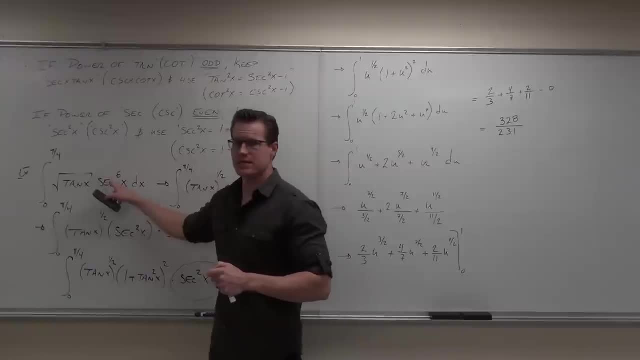 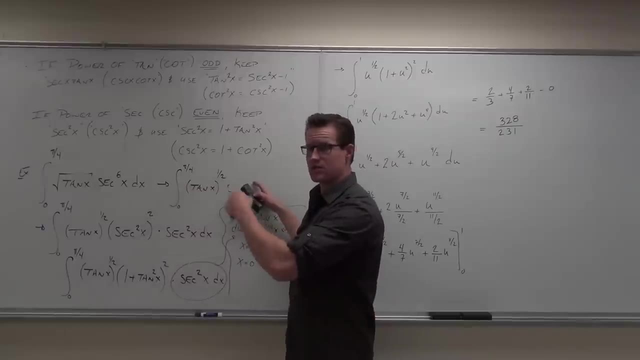 then we would just still. If this was the same thing with secant to the 10th, you would go about it exactly the same way. The only difference is this would be a secant squared correct, And you have secant to the 8th. 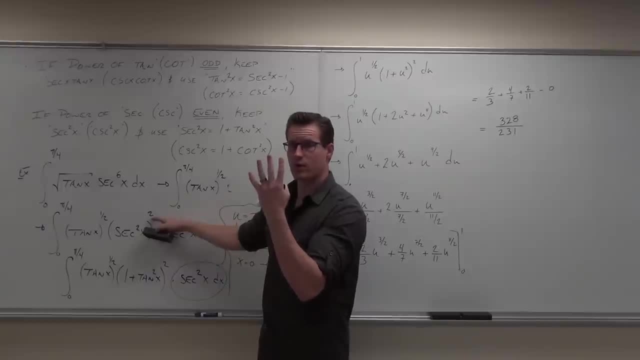 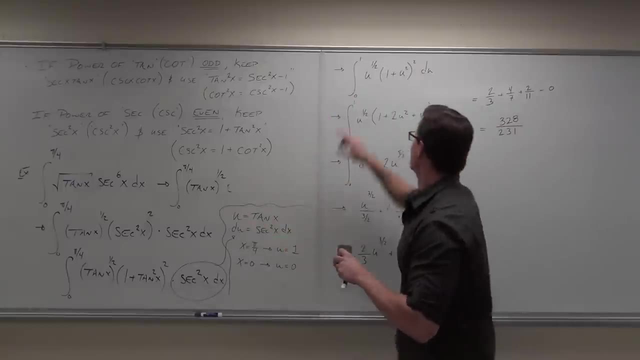 This would be secant squared and this would be a 4.. The only problem with doing this is that when you get down to your u sub, you'd have to distribute a lot, because you'd have one plus u squared to the 4th, so you'd have to distribute all of that stuff. 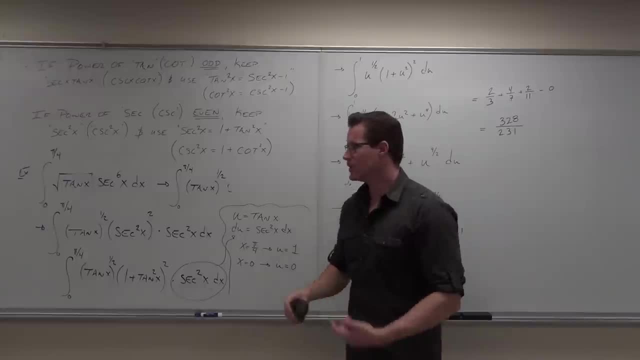 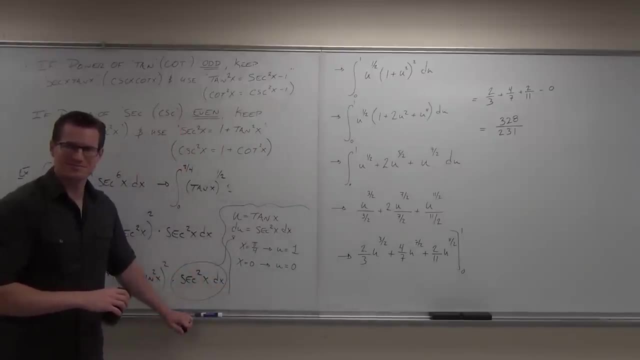 You'd have lots of terms there. Yeah, right, So that's the. it can be done, but it's a lot of distribution. More No, You sure It's doable, It's just a lot of No. I'm just wondering if you could just split it twice and then do two. 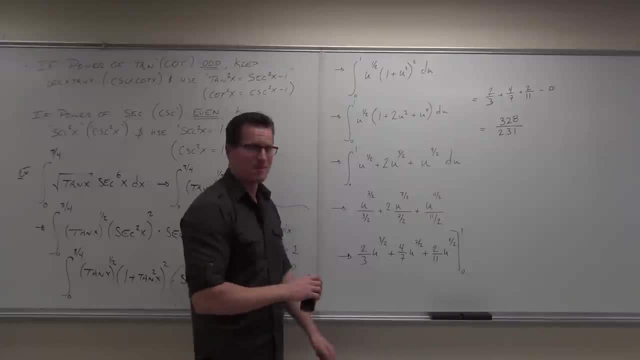 At some point you will be distributing somewhere with this stuff, because if you do secant to the 8th, you're going to get a 4.. And if you do split it right, you'll have multiplication. And when you do, when you do your identity right here, from here to here, you get a plus. 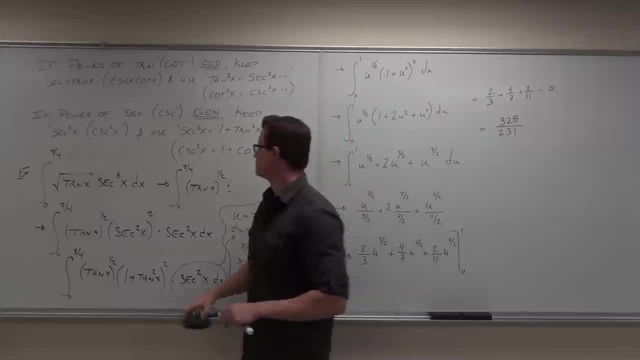 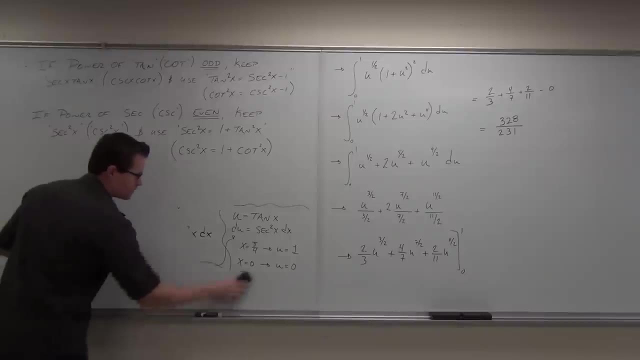 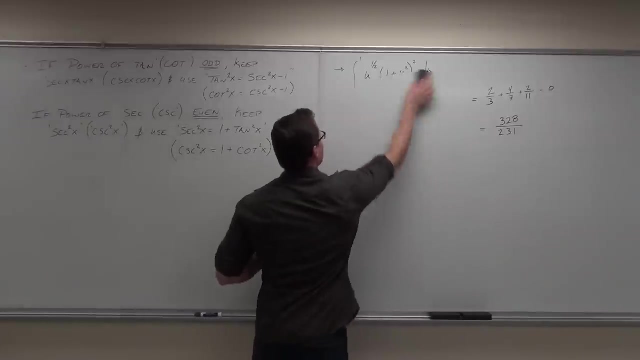 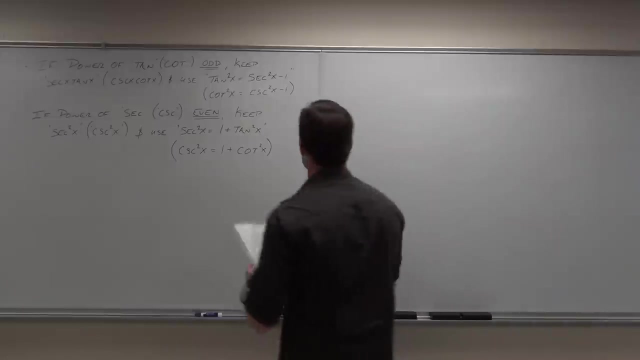 After you get a plus, you will have to distribute all that stuff. That's the idea, Okay. So last one before I give you some other ideas on this section. Let's work over here this time, Okay, So let's check our pattern out. 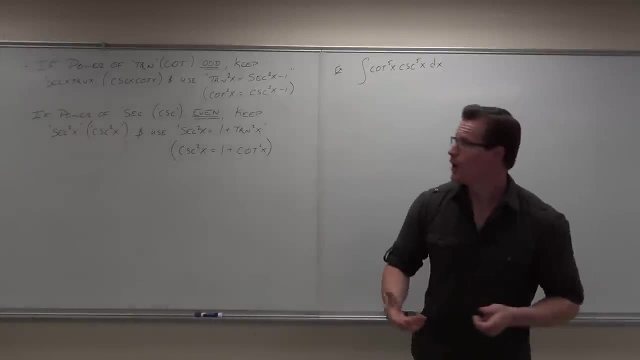 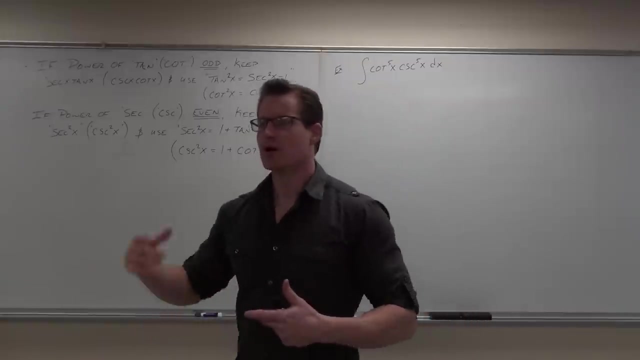 We know 1 for sine and cosine. We know 1 now for secant and tangent. Secant and tangent work, or actually I should say it this way: Cotangent and cosecant work really, really similar to tangent and secant. 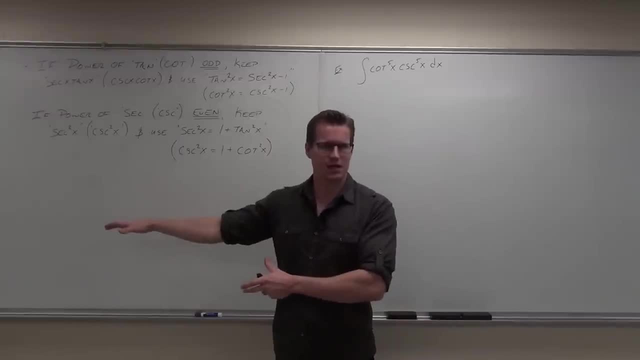 So the same thing that we just did with tangent and secant, we can basically do it with cotangent and cosecant. Of course the derivative is a little bit different, So it's got a negative in there we'll have to be aware of. 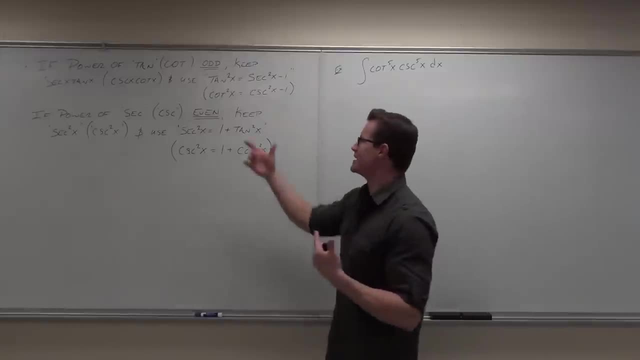 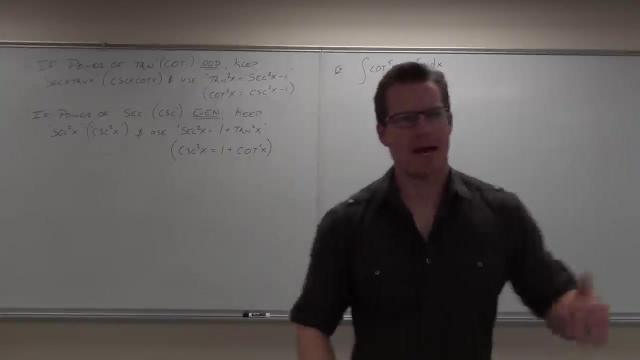 As long as we don't mess up that negative, it works really similar. Even the identity is pretty much the exact same thing, So it's really close. So let's check it out. Which one does this fit? Which pattern Is this? the one where power of tangent or cotangent? 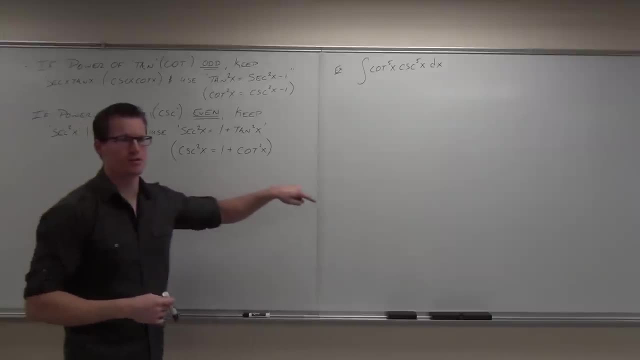 Is odd, Or the one where power of secant or cosecant is even. Which one? Yeah, the cotangent's odd. So that fits this top one. It says the power of tangent or cotangent is odd. We're going to do something. 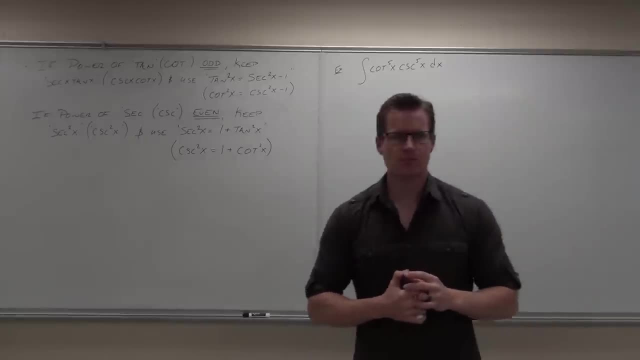 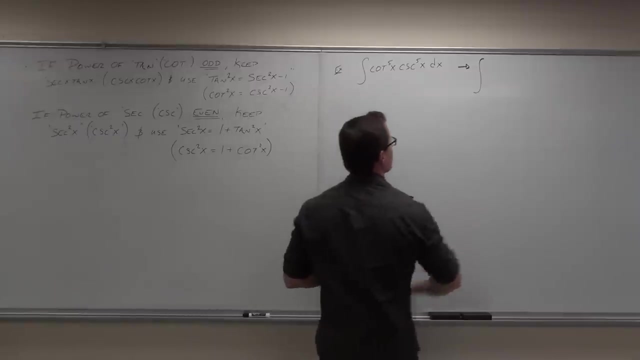 What are we going to do with this? Okay, So that's what I want you to do right now: Do the first step. Don't just wait for me. Do it yourself. You know what I'm going to need: more room than that. 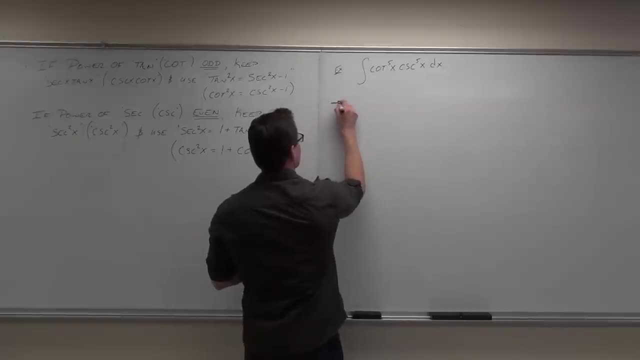 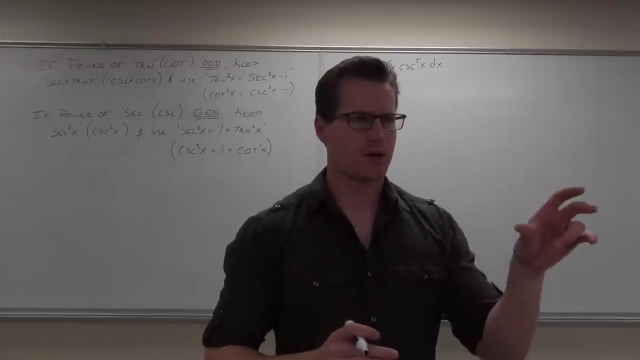 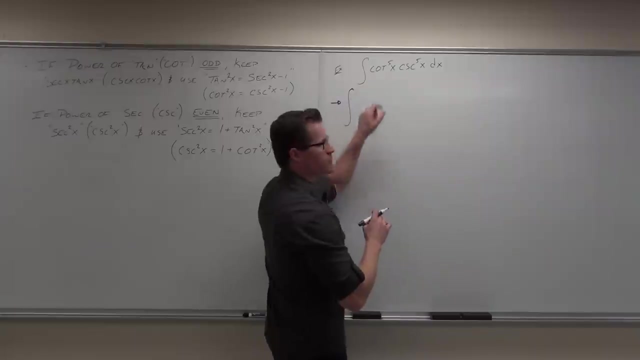 So if cotangent is odd, you strip off cosecant cotangent. That's the idea. Strip one of those things off. Let me see if you wrote, What did you write? What did you write down? What does cotangent become? 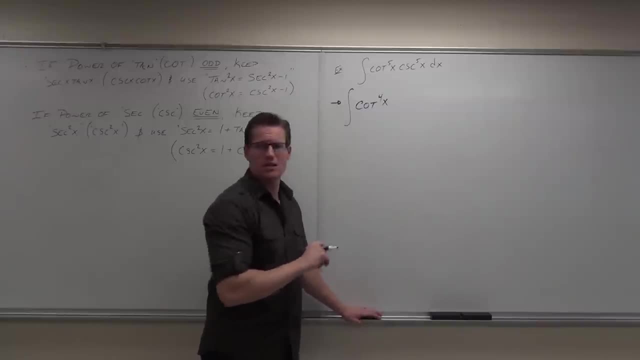 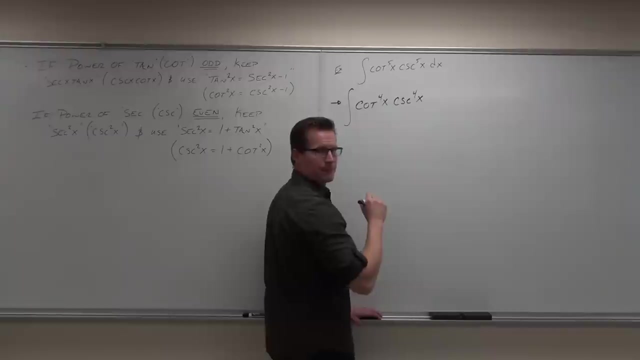 And what else Cosecant to the fifth? or to the fourth, Fourth, Okay, Then what Cosecant to the fifth? Would you flip them? I would, Just because I'm used to seeing cosecant x, cotangent x, dx. 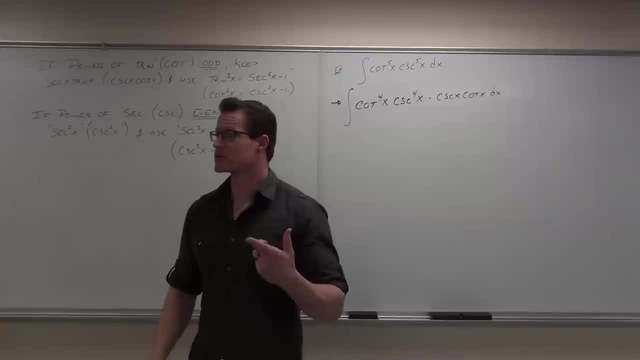 I would do that because that's the way it looks in my head when I do derivatives. That's the way it looks, So if I should be okay with that one so far. Now, I need you to understand that. don't just follow this. 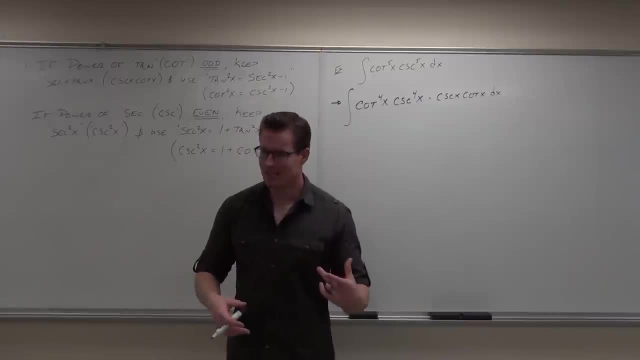 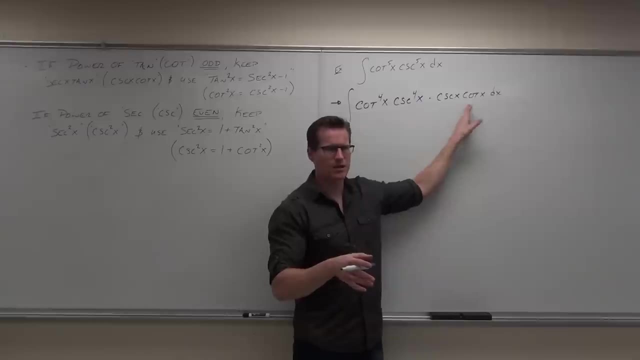 as a pattern. okay, Really understand the process. The idea here is that this is supposed to be a derivative of something. Is this the derivative? Think about this when you're doing these problems. Is this the derivative of cotangent Or is this the derivative of cosecant? 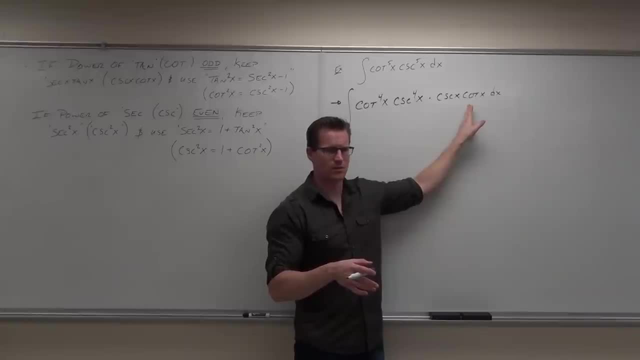 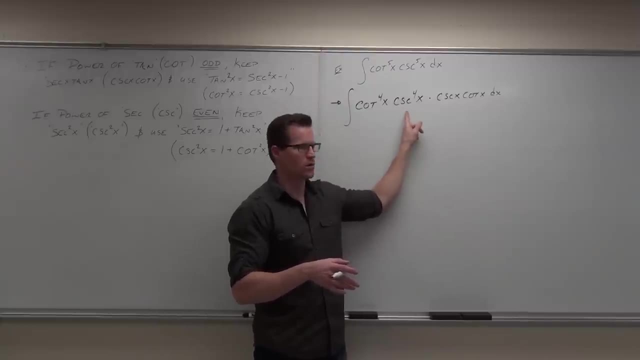 It's the derivative of cosecant. You with me. What that means is that I want all of this to become cosecant. Am I going to change the cosecant? No, Am I going to change the cotangent. That's why it's written this way for you. 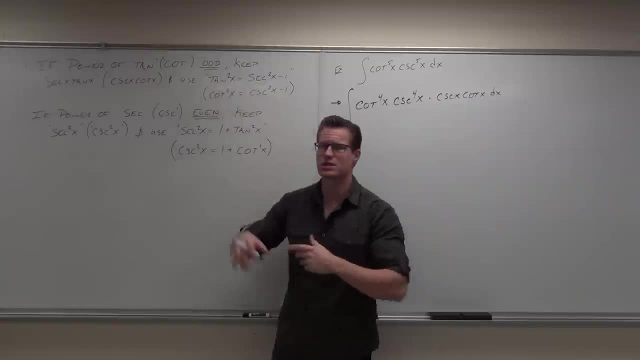 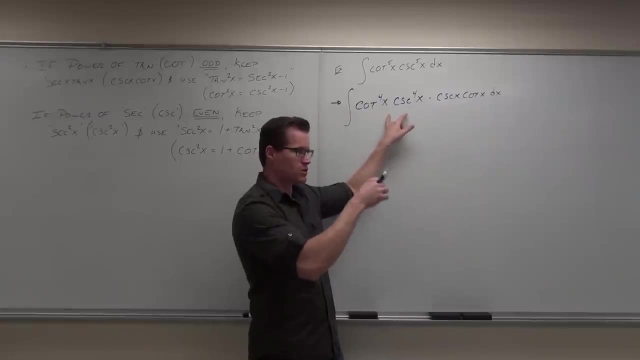 Use cotangent with this identity right here, Make it into cosecant. You're stripping off these pieces as a derivative. So you want to change everything else so that when you do the substitution the derivative exists. If you do this and you start, 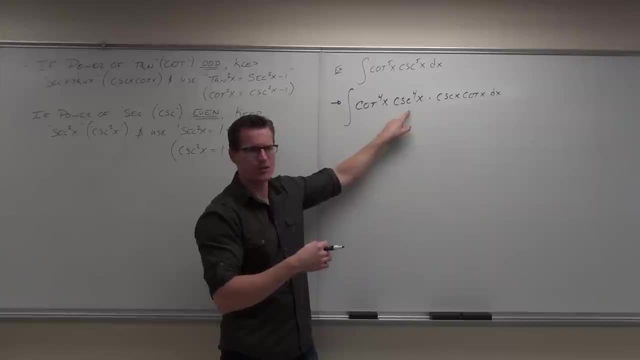 using an identity on cosecant and change it to cotangent. the derivative of cotangent is not cosecant cotangent, It would be using this one. It would be. the derivative of cotangent would be the cosecant squared. so we couldn't do it that way. 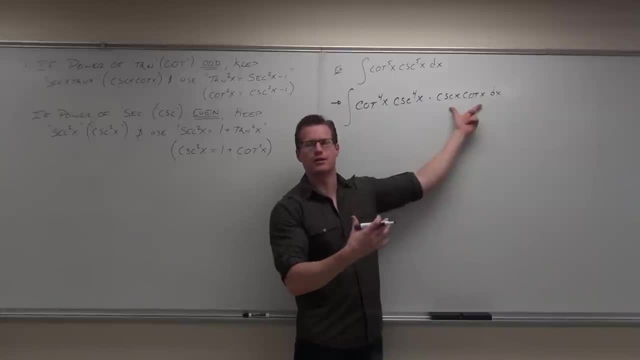 So again, the idea is, when we're stripping it off, we're actually getting a derivative here. Change everything else to the trigonometric function that gives you this derivative. Is that clear? So change cosecant. No, The derivative of cosecant is. 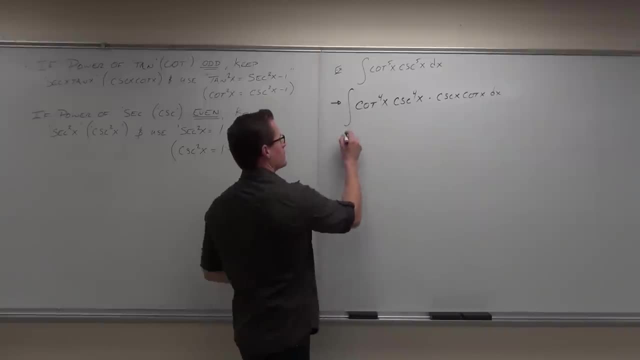 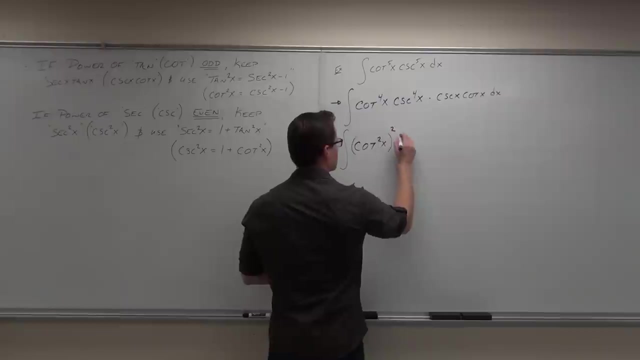 Is this Change cotangent? Yes, Yes, So in our case? well, probably got to write it a little bit different. Cotangent to the fourth is not our identity. How can I rewrite that, please? Yeah? 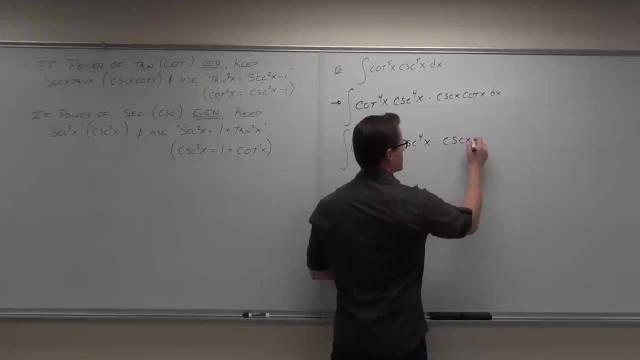 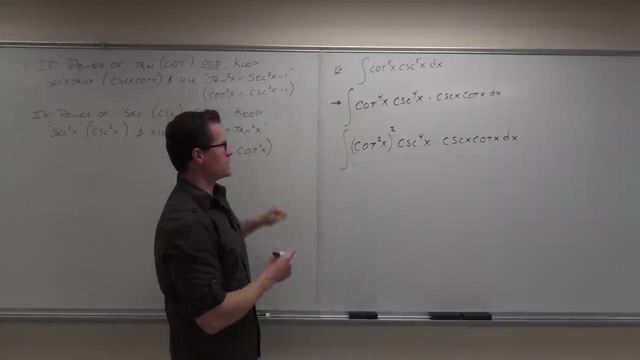 I don't want to change cosecant. Those are great for us. That's going to give us our substitution in just a second. So we write it so that we can actually use it, So that we can actually use our identity. Our identity says: if we had cotangent squared. 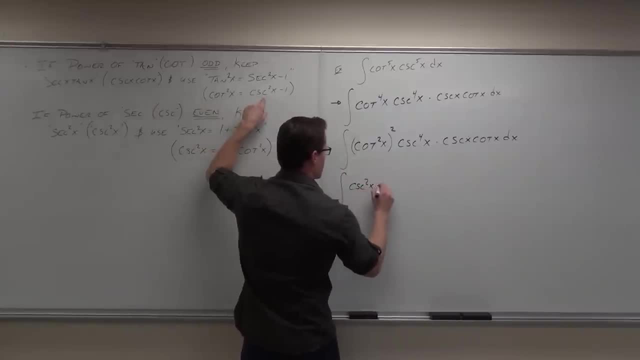 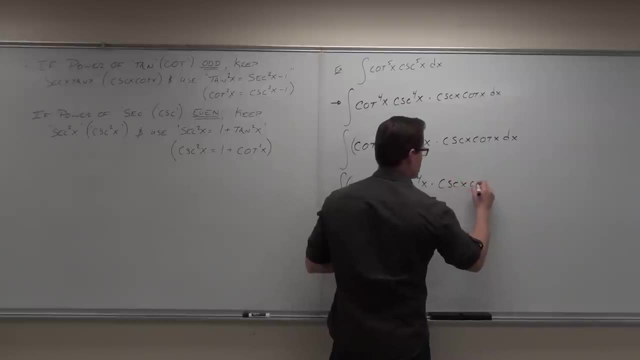 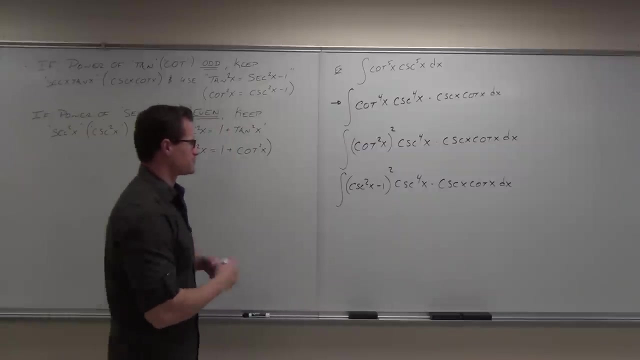 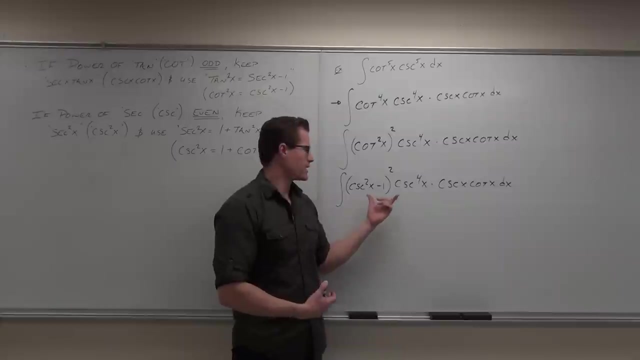 that's the same thing as cosecant squared minus 1 squared. Believe it or not, we're almost done. Ladies and gentlemen, are you OK so far? I want to know if you understand the reasoning behind what we're doing here. 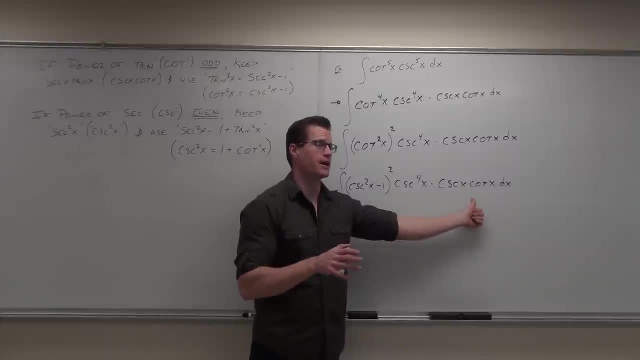 be cosecant, because this is the derivative of cosecant. So once you have that, as soon as you have this down, where they're all the same and the derivative is right here, what should you be doing? That's like the definition of when to use a u-substitution. 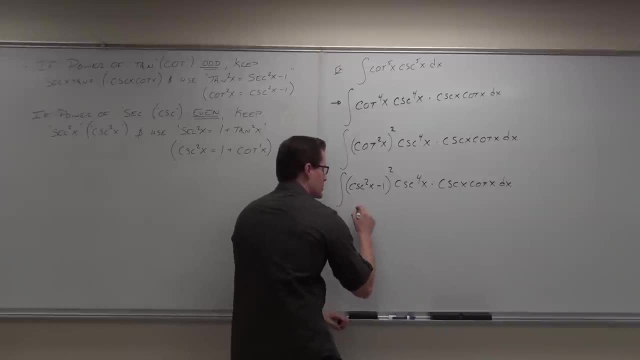 is when you have one piece that if you take it out with a substitution and you take a derivative and the derivative's in there, it'll work. Now here's the deal. You do gotta be pretty good about your derivatives of these things. 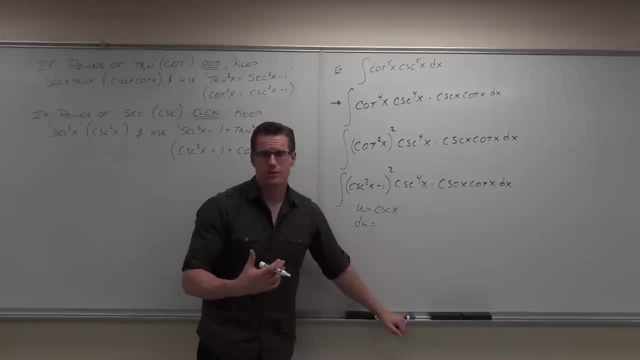 We don't use derivative of cosecant a lot, but you still gotta know it. Derivative of secant is positive, secant tangent. Derivative of cosecant is negative. cosecant cotangent- Let's switch over that negative. So negative. du equals cosecant x, cotangent x dx. 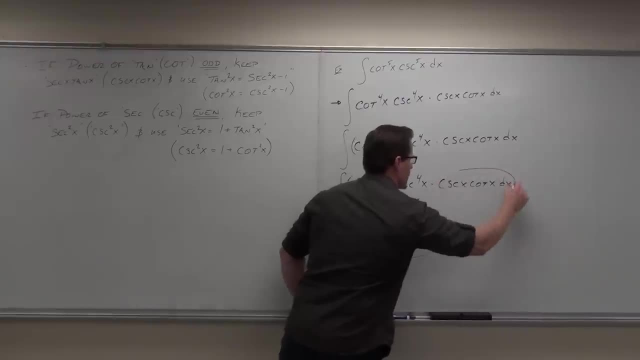 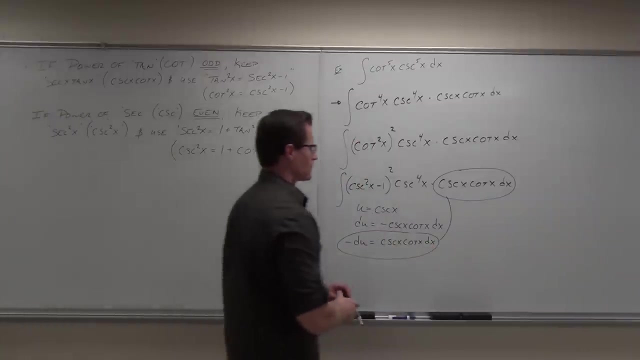 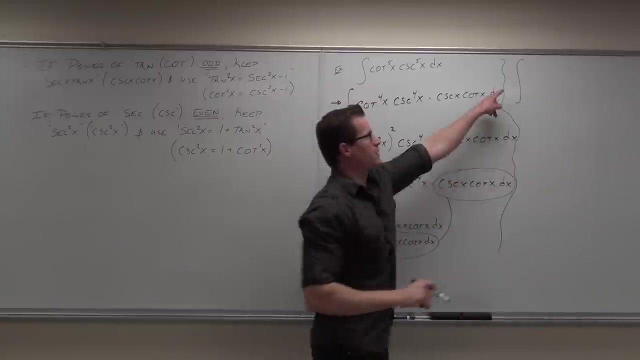 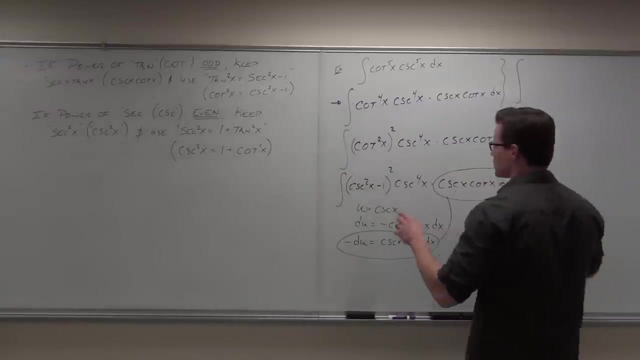 And now this is exactly what we have here And that'll let us do our substitution. I'm gonna move up here. Can you please tell me what this integral will look like after I do all of this substitution? Integral of what's this become? 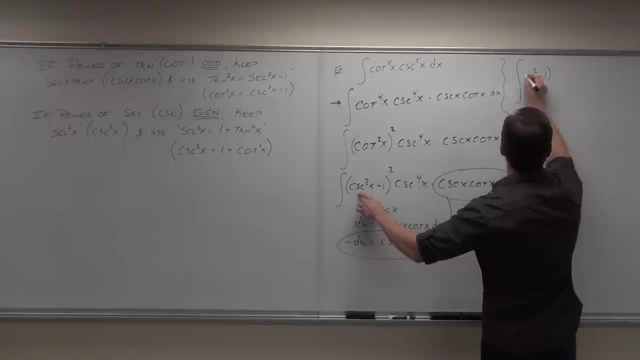 E squared Minus one, Minus one. E squared Minus one, Minus one. U to the fourth, Oh good, u to the fourth, And Negative du Good, Perfect. So this is u: u squared minus one, squared cool. 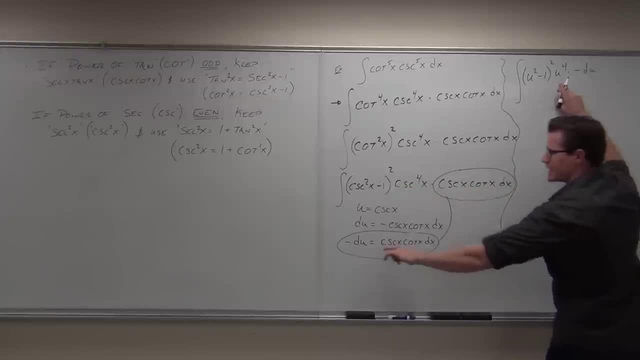 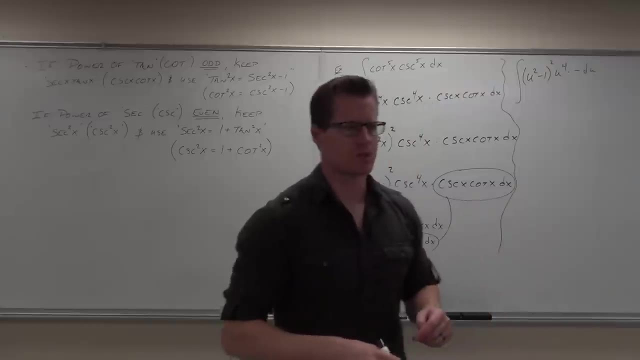 We got u to the fourth power, no problem. This whole thing is equal to negative du. Do not forget about that. negative, that's a big deal. So negative du. and now we'll just do a simple integral. Tell me some things that you're gonna do here. 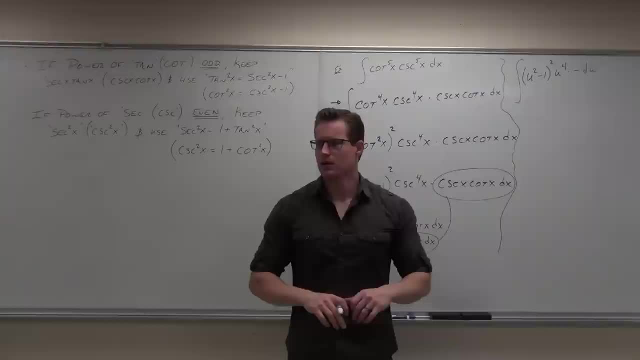 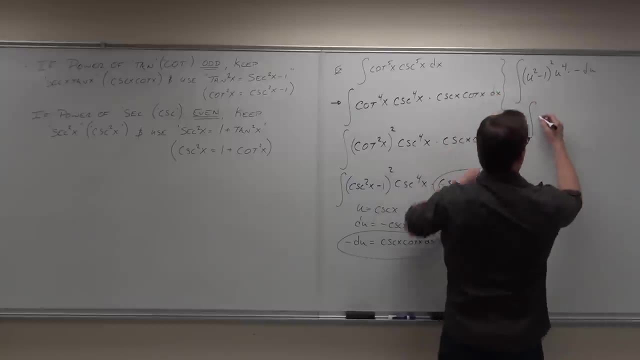 Negative out front. Negative out front. very good, What else Distribute? You're gonna have to distribute Oil. So negative comes out front. Negative comes out front If we distribute. we got u to the fourth minus two. u squared plus one. 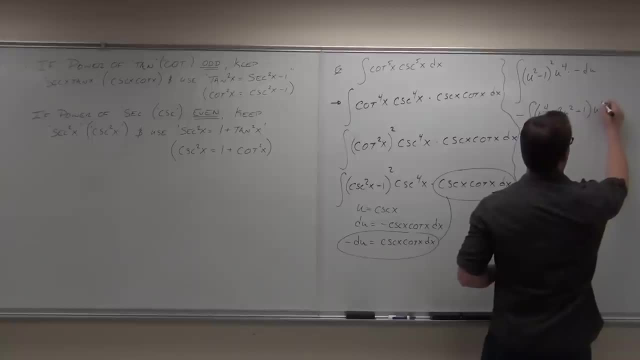 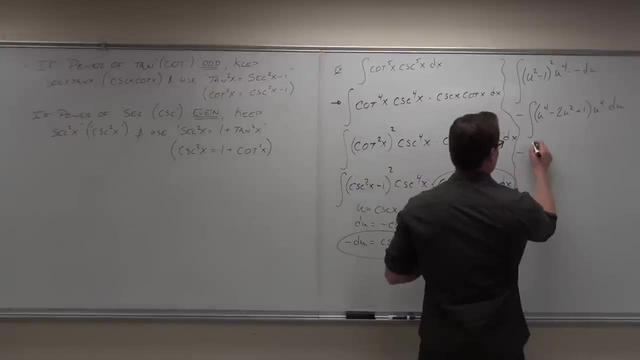 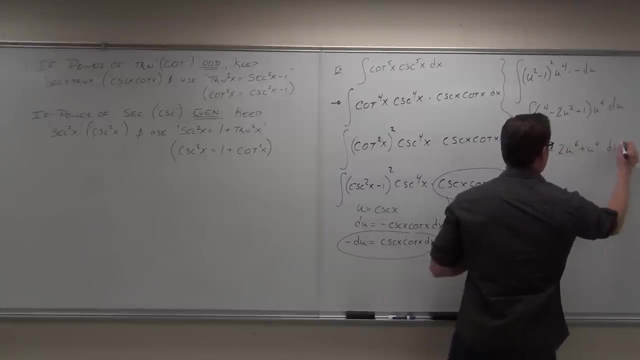 If I did it right, Did I do it right? Yeah, Okay Times. u to the fourth. Now what Distribute? Do it again? Negative integral: u to the eighth minus two. u to the sixth plus u to the fourth du. 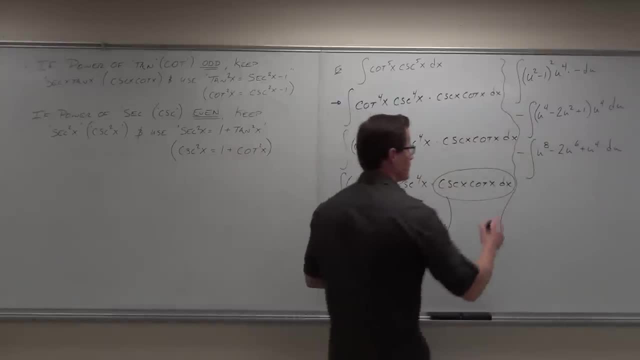 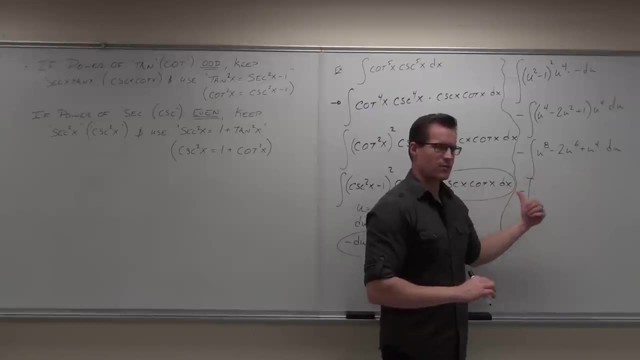 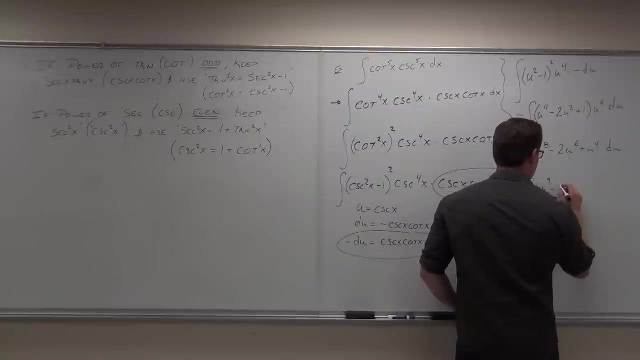 Can you guys do that integral, Yeah, Negative. just don't forget that you either need to distribute the negative now while you're doing this, or have it out front, because it will distribute eventually One-ninth u to the ninth minus one-third. 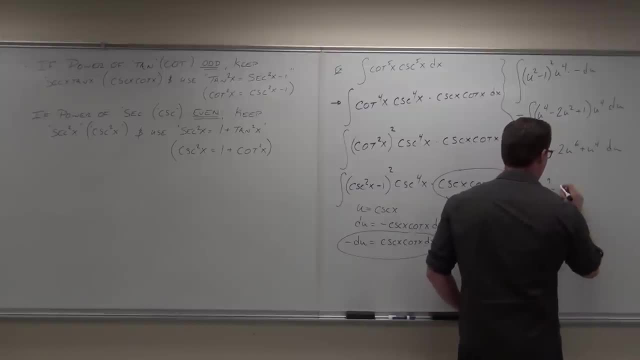 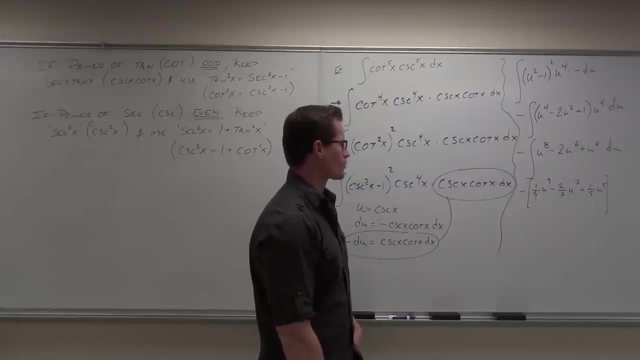 oh, no, sorry. two-sevenths, u to the seventh, One-fifth, u to the fifth, And lastly, tell me some other things that we're gonna do here. please Substitute. We do have to substitute. So we don't want, I don't want u's. 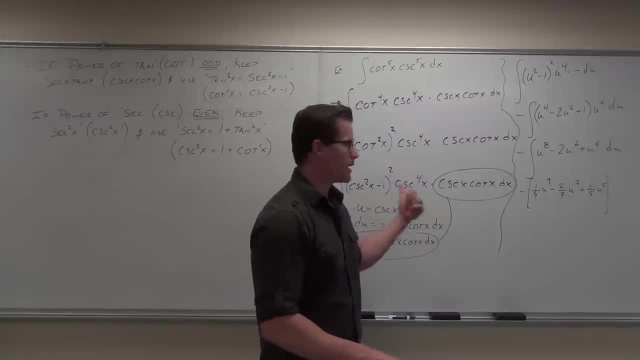 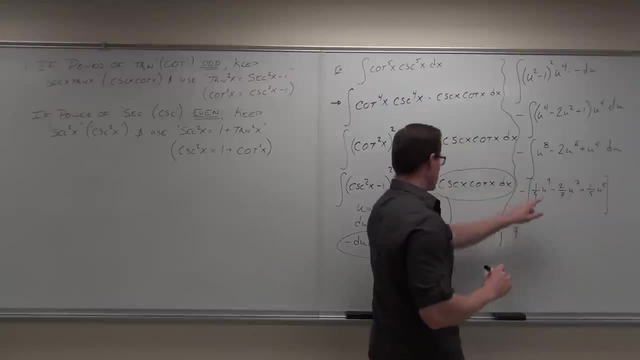 We start with x's. You better give me some x's And then distribute the negative, And then distribute the negative. So I'm gonna do all those steps at once. We're gonna have negative one-ninth. u becomes cosecant to the ninth power of x. 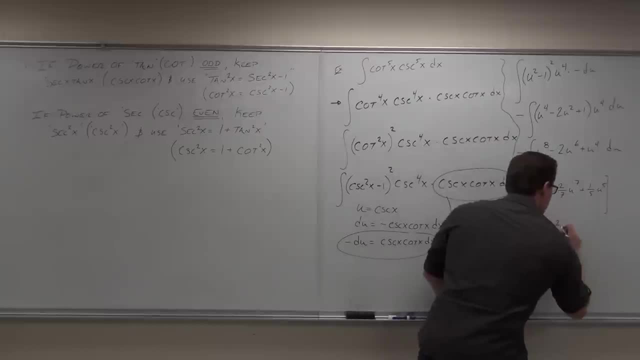 We're gonna have plus Because we're distributing the negative Two-sevenths cosecant to the seventh power of x, plus one-fifth cosecant to the fifth power of x And finally plus c. That means we're done. I like that. 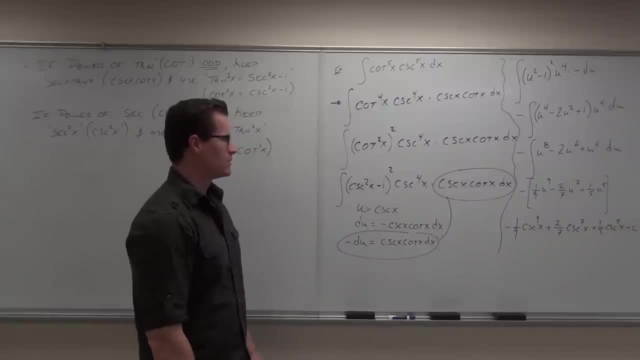 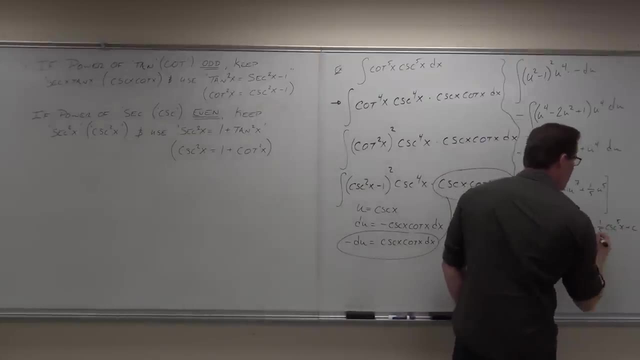 Plus c, But you don't want to factor out the secant five x and one over nine. One-fifth should be negative. Oh yeah, you're right, I'm sorry I missed that. Yeah, good catch, That should be negative. 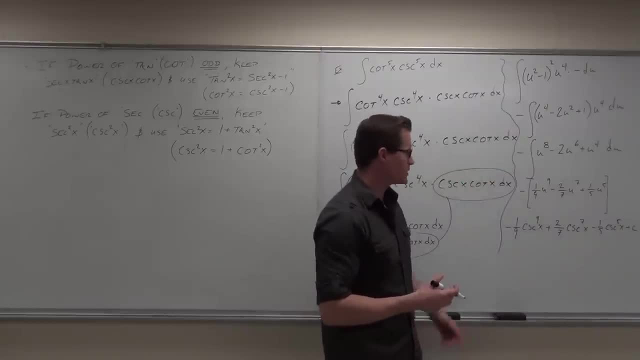 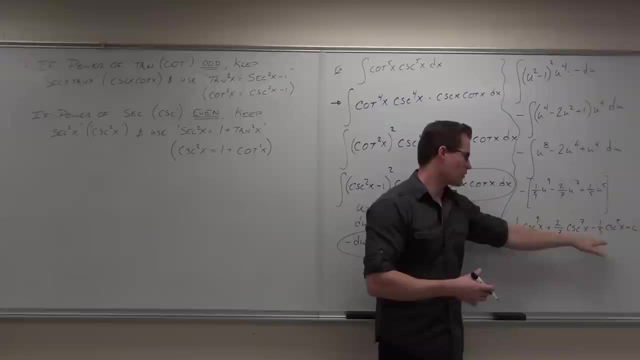 You can factor this if you want to. That's fine, I'm trying to get you to. you get the basic idea of getting down to here. Once you get to here, really, we should know how to do that, right. So if you get down to here, 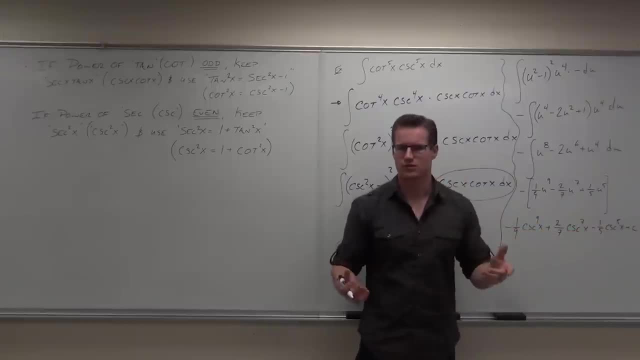 you're like: I want to factor that, Go ahead and factor it. You want to factor out some fractions? factor out some fractions. I don't really care. I want to make sure that you are good. This is really what I'm trying to teach you. 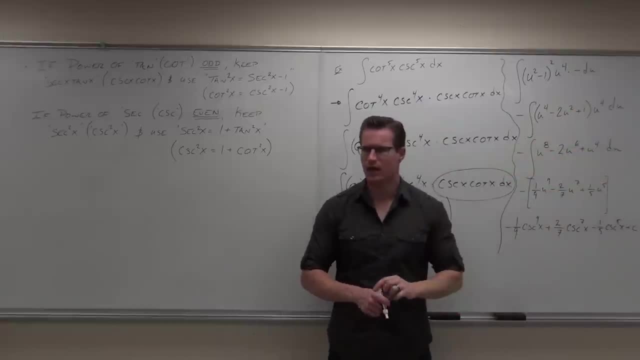 is up to this point. This stuff should be your basics. after that, Let me show the fans if you feel okay with this one. Okay, those are the basic three. If we have sines and cosines, you have patterns for that. 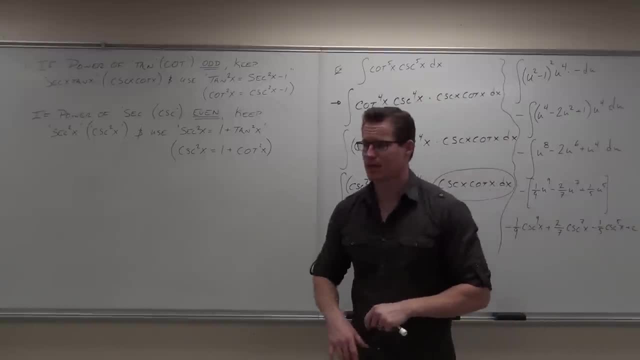 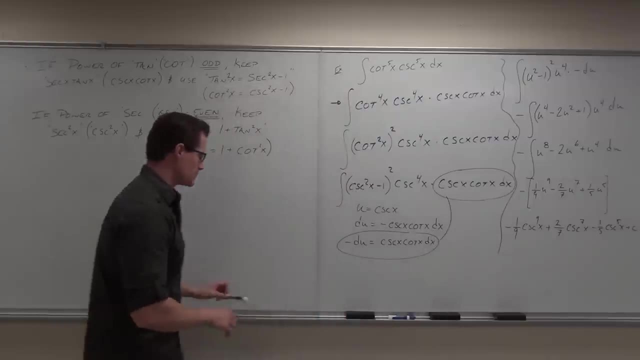 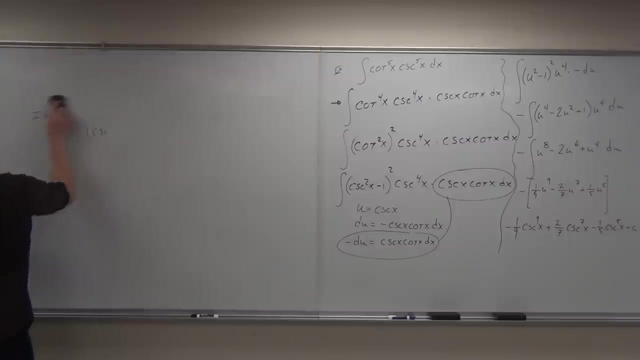 You have secants and tangents. now you have patterns for that. You have cosecants and cotangents, no problem. What happens if they don't fit those patterns? We're going to talk about that right now, Like if you have one more cotangent. 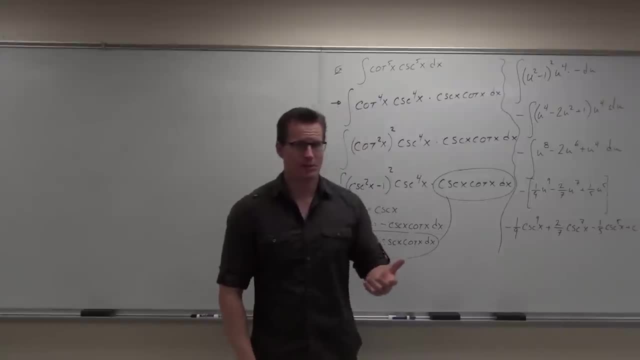 in that last problem. Yeah, some of them can't be done. I mean some of them. there's no real good way to do them. Some of them, like, I'm going to show you the only way around doing this, like this one. 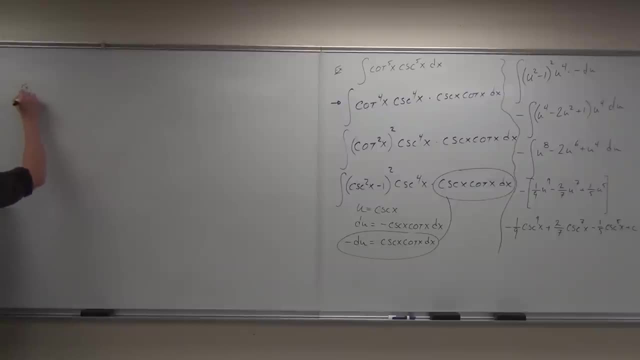 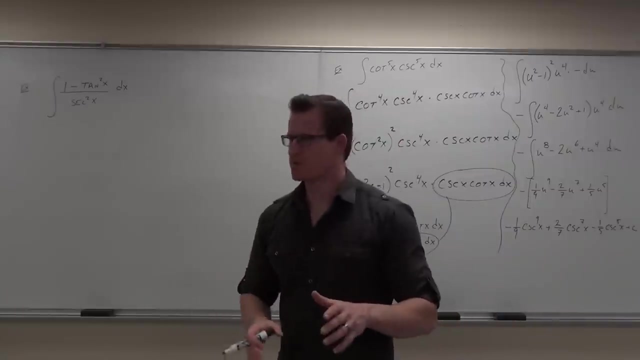 Like if I were to give you that, If it fits the patterns I've given you, for goodness sakes, use the patterns and do them. okay, If it doesn't fit exactly, sometimes we can change it so that it fits a good pattern. 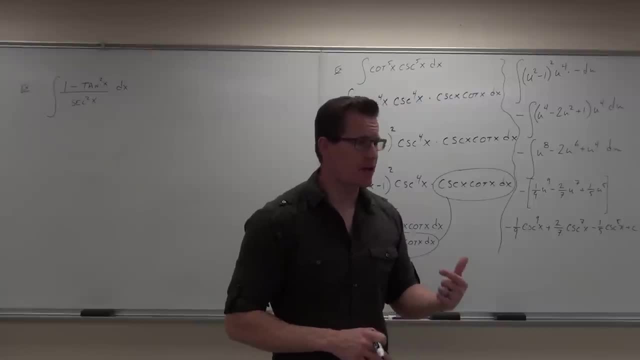 Okay, Okay, Okay. If it doesn't fit a good pattern, sometimes we can't. If it doesn't fit any pattern at all like this one, does that fit anything? It's got secants and tangents right, But they're not multiplied together. one's being divided. 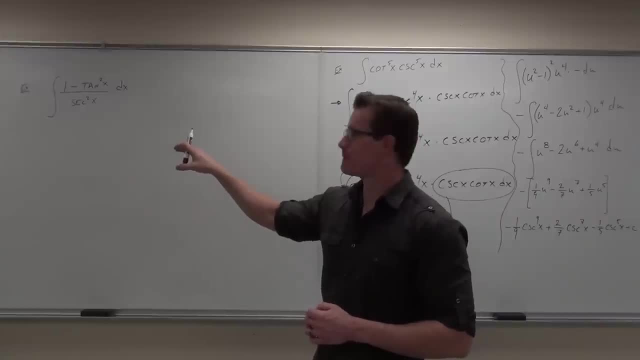 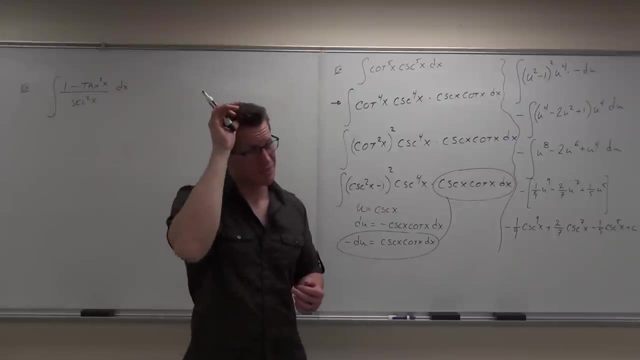 This doesn't count. This is more like tangent and that's actually a cosine. if you move that to the numerator, That's tangent and cosine. So that's really not exactly what we're looking at. So one big hint for you is: if it doesn't fit the pattern. 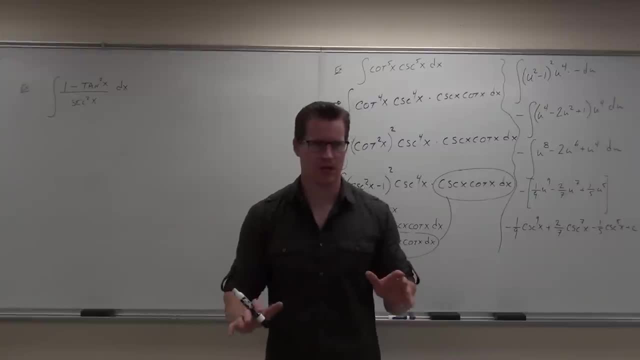 if it doesn't fit. so first thing, don't do this first. okay, Check the pattern first. If there's sines and cosines, you can work with it. You can work with any sines and cosines that I've given you. 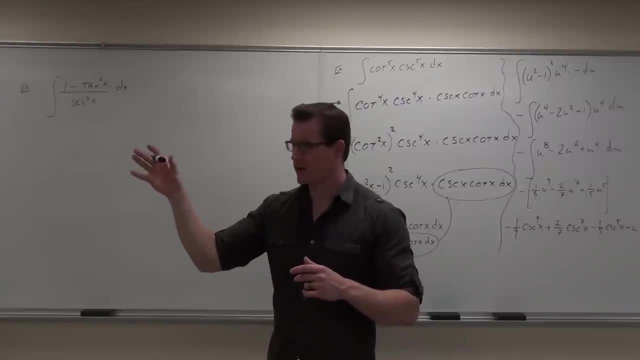 If there's secant and tangent and it fits so that either tangent's odd or secant's, even you can do it. If you have cotangent and cosecant, where cotangent's odd or cosecant is, even you can do it. 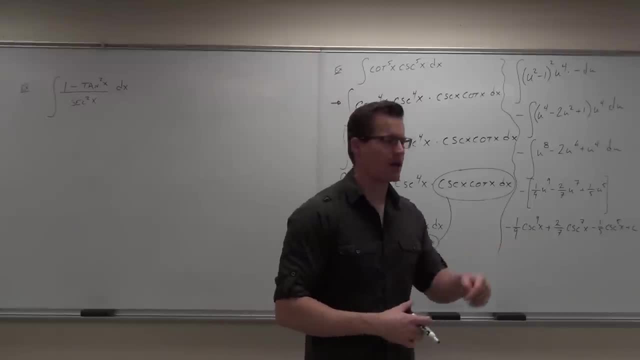 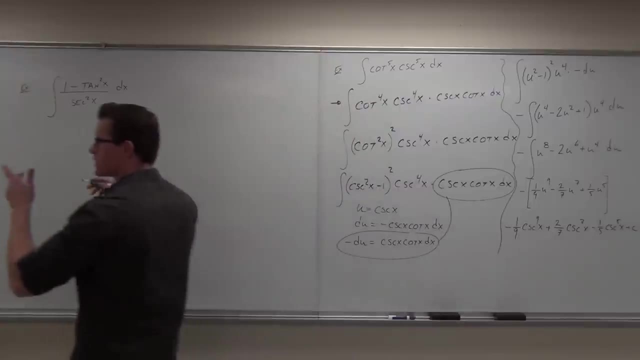 If it doesn't fit those things. the one thing you try after you check that see if you can change it to sines and cosines using those identities and then see if it will work. So let's try to change it. So the note that you probably should write down: 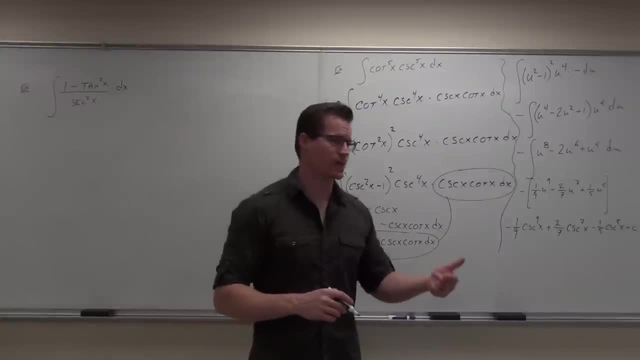 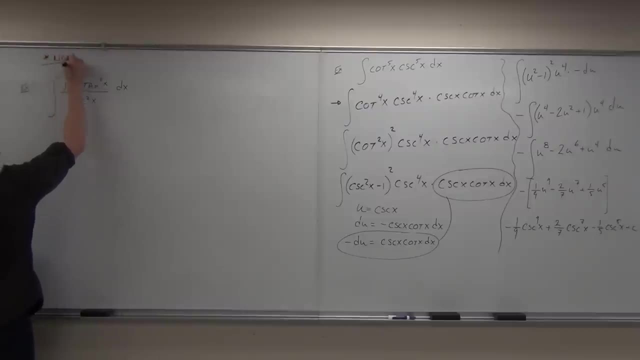 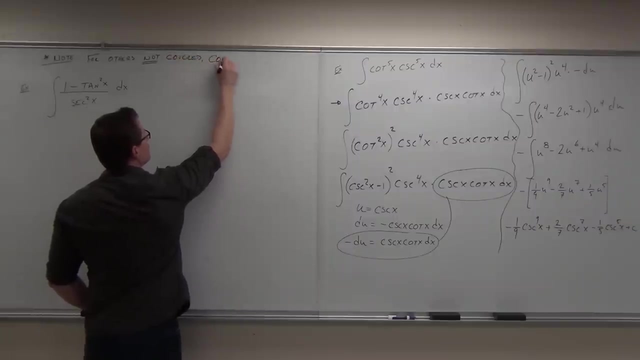 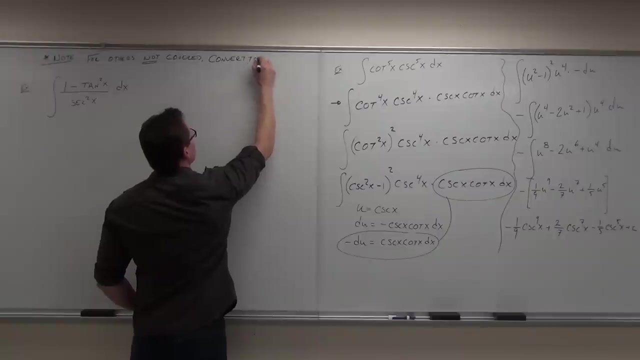 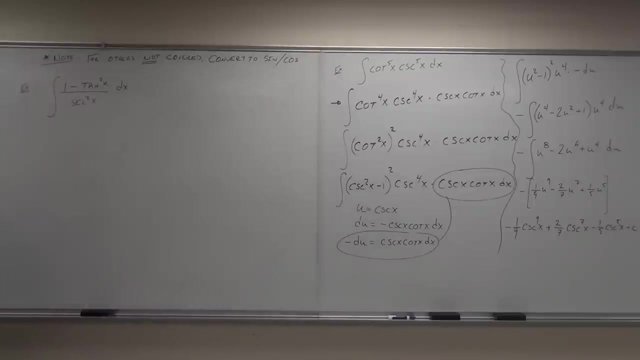 is, if it doesn't fit the pattern, try changing it to sines and cosines, That's if, though. So for others not covered, try converting to sine and cosine. So let me show you some ideas that I would do if I was looking at this problem. 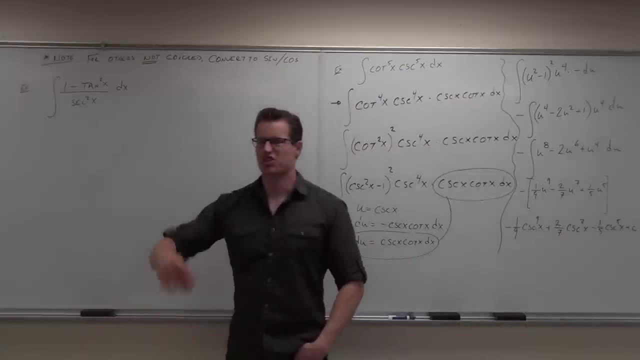 The first thing I would do is I'd look for an identity so that I could just nail right off the bat: Now this one's pretty close, but that's not an identity. One plus tangent squared, That would be an identity. That would be easy, because one plus tangent squared. 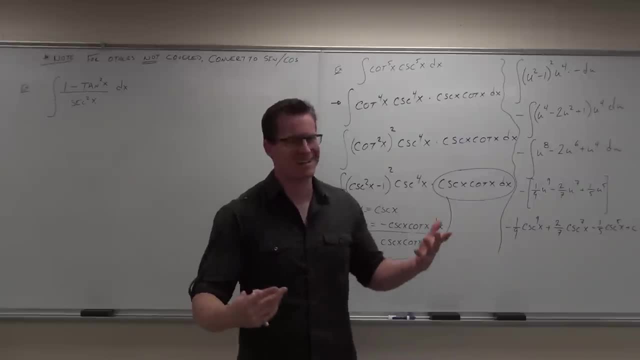 would be secant squared. Secant squared over secant squared would be one. You'd get x. Hey, that'd be nice. We're not that lucky, okay. So that's not an identity. Don't create your own identity. 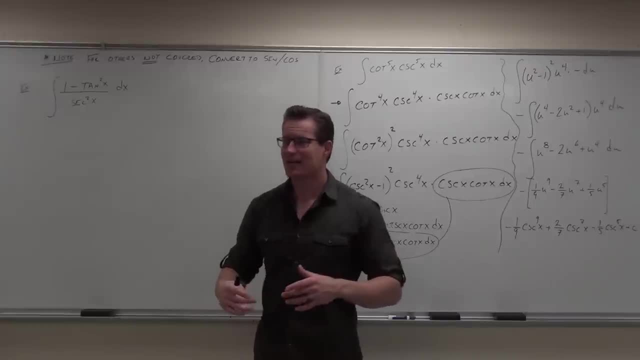 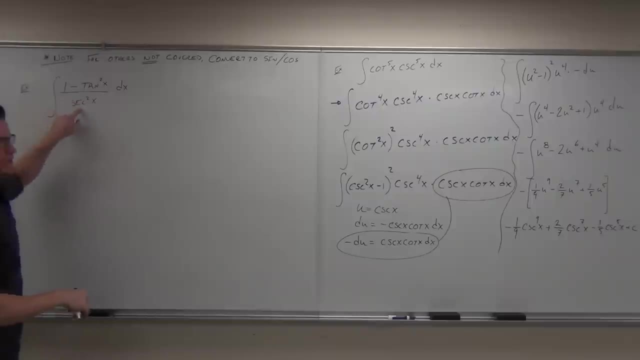 Some of us like to do that in this class. Instead, work with this thing with identities that you do know, or if you don't try to break pieces apart. So first thing I'd say is I don't really like secant squared. 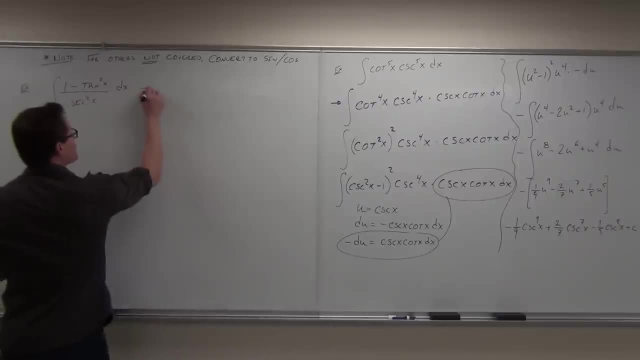 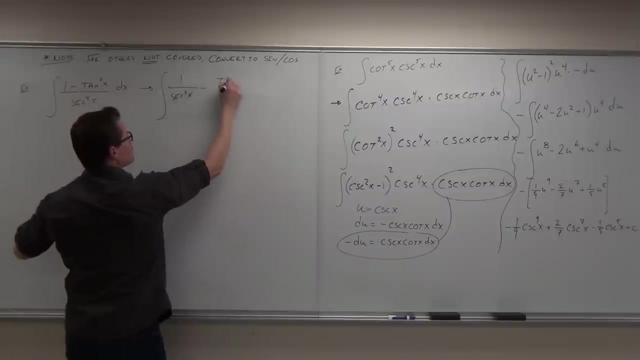 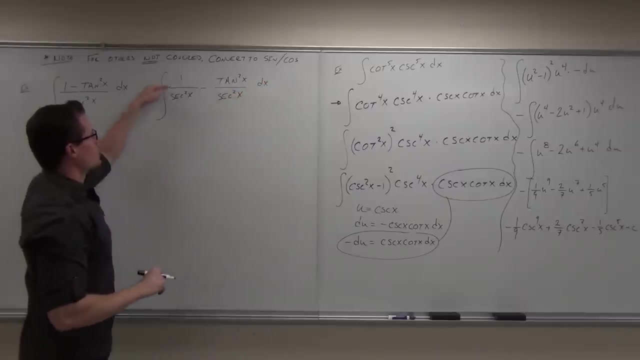 Secant squared isn't cosine, So one thing I would try is I would split up this integral into one over secant squared. Secant squared x minus tangent squared x. over secant squared x. The reason I'm doing that is because I know that one over secant squared x is actually. 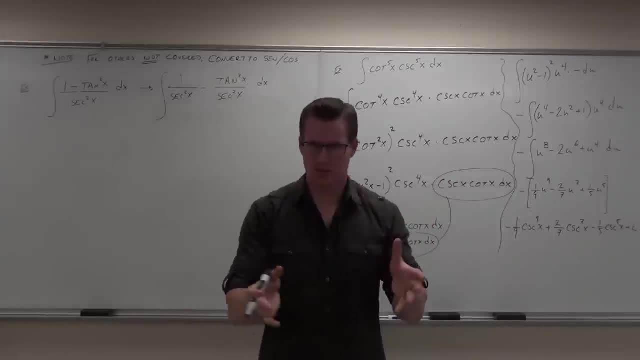 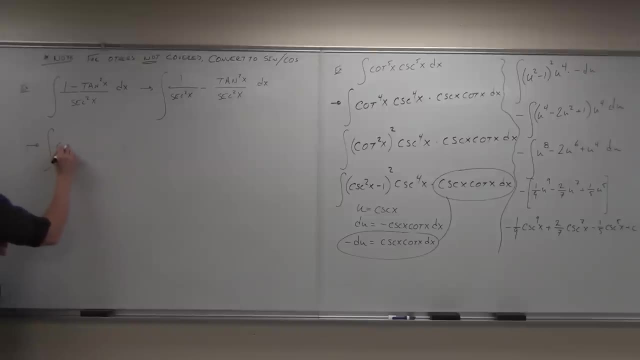 the same as what Cosine squared? Cosine squared, Remember, convert to sines and cosines. That's one way we can do it. So then this becomes cosine squared x, And let's take a look at what this actually is. 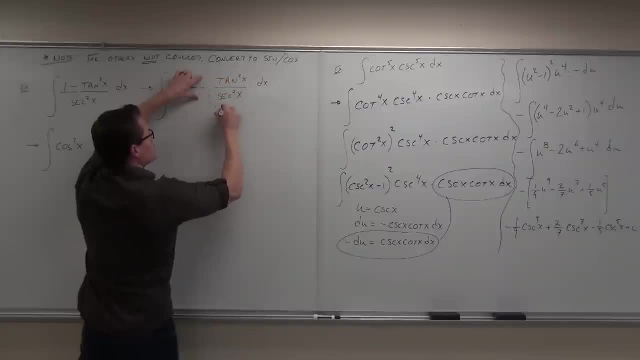 What this actually would become. this is tan squared x times cosine squared x. Believe it. This is cosine squared x. That's what that is. So one over secant squared is cosine squared, Understood? Well, what's tangent? So tangent squared is sine squared. x over cosine squared. 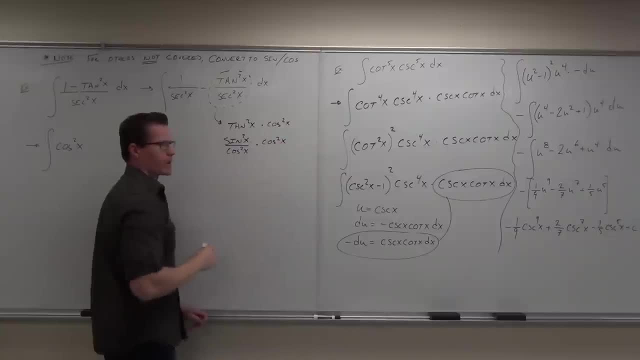 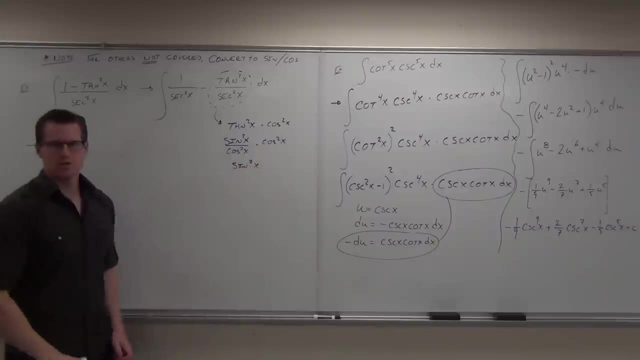 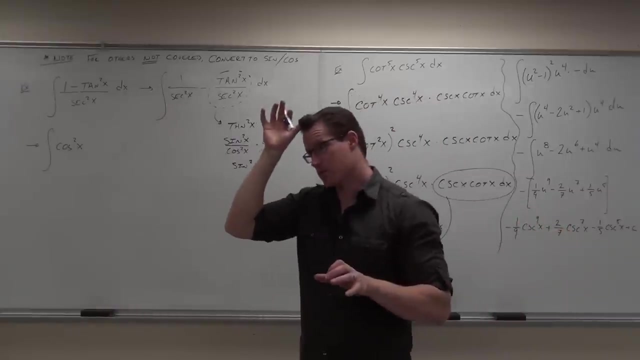 Cosine squared x times cosine squared x. What happens here, by the way, That's fantastic. So just by doing a little bit of a change here, by pulling those fractions apart and by using our identities for what one over secant squared is, for what tangent is, 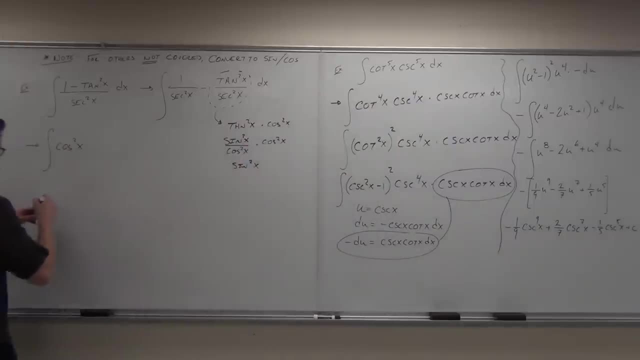 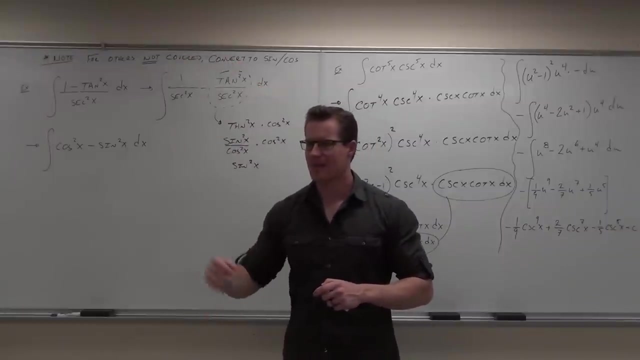 what one over secant squared is. we can simplify this fraction from this nasty thing to this really nice thing. I need a show of hands if you're okay with that one. Hey, have we done any calculus right now? Not yet. This is trigonometry. 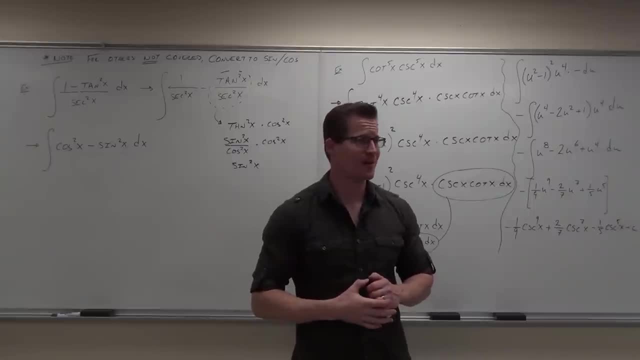 Purely trigonometry. In fact, the next step is going to be trigonometry, because this is kind of awesome. There's an identity and if you want to look it up right now, you can look it up. This is actually an identity. 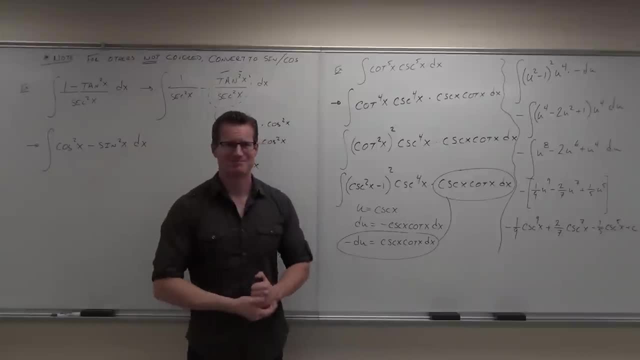 Do you know what it is? Negative 1.. Please don't say 1 or negative 1.. Sine 2x: This would be 1.. That would be 1.. This is not negative 1.. That's not the way that this stuff works. 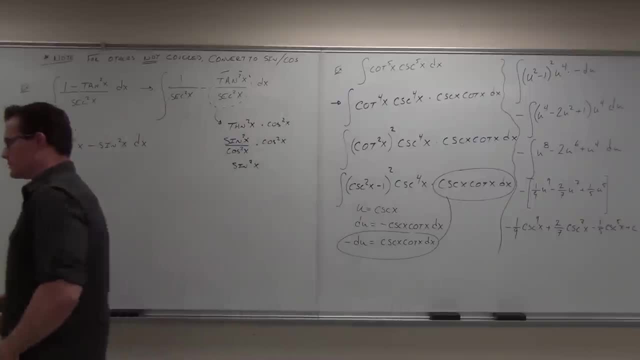 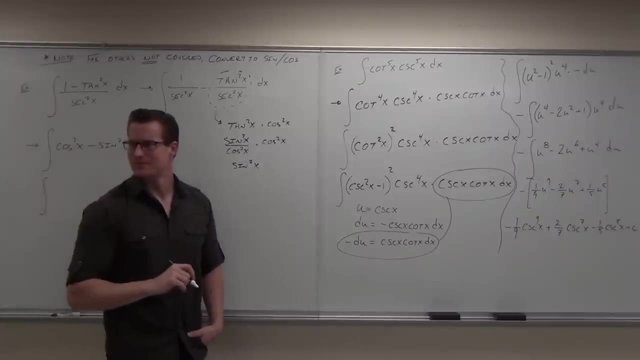 No, no, it's not, It's not. But if you want to look it up, go ahead and look it up. Ooh, I think I know what it is. OK, Rob, It's going to be 0 sine 2x. 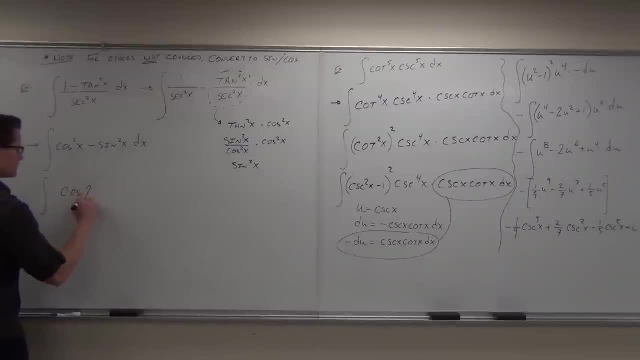 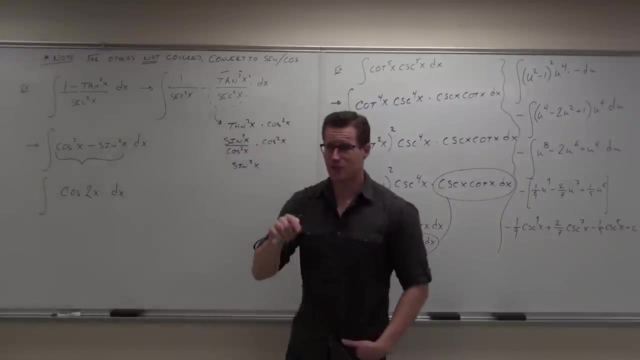 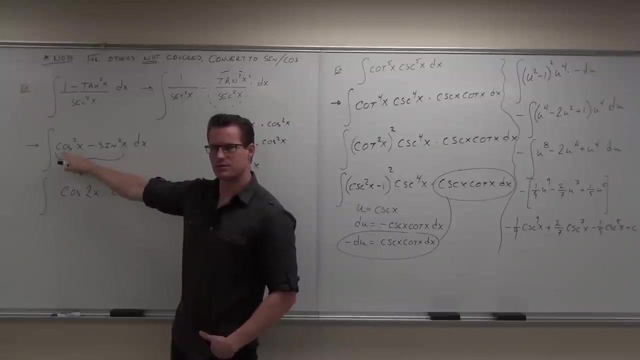 Perfect. Does it help to know Your trig identities? Because if you didn't, if you didn't know that, look at this: You know how to do cosine to evens, don't you? You know how to do that, You'd have to do this one. 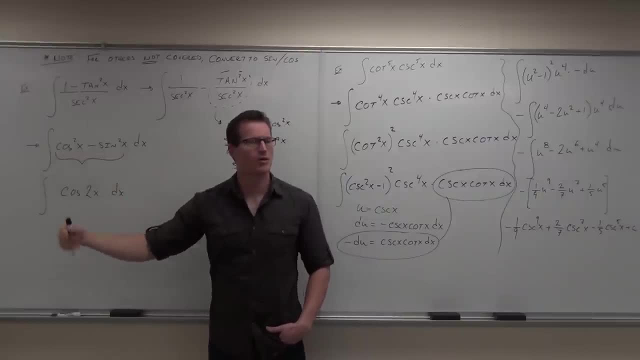 You'd have to do this one independently And then you'd have to put them all together. But if we know our identity, we go: oh hey, look at it, That's cosine. Can you do this? That's now a piece of cake. 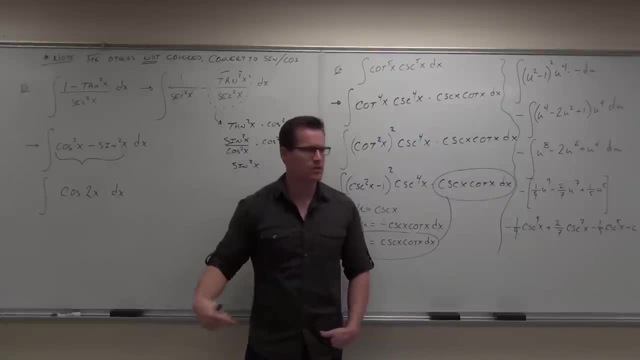 This would be like I would do the u sub in my head. I don't write out the u subs for a lot of these trig ones because they're so easy And they take And we do so many, So many of them, especially, like you found out. 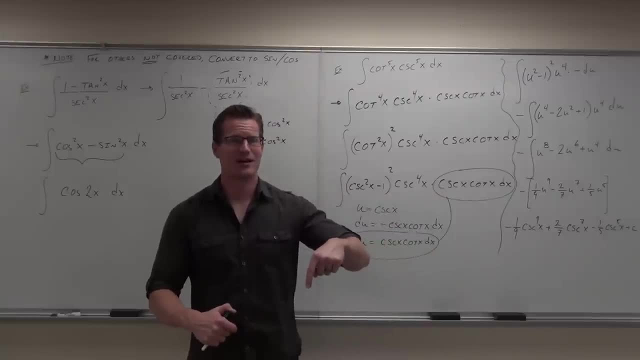 in your last homework or this homework, I'm sorry. When you have like cosine squared of 2x, well then you're going to be getting 1 half 1 plus cosine of 4x. That angle's going to change. 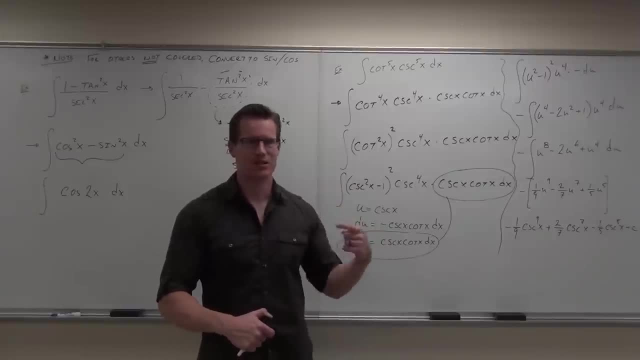 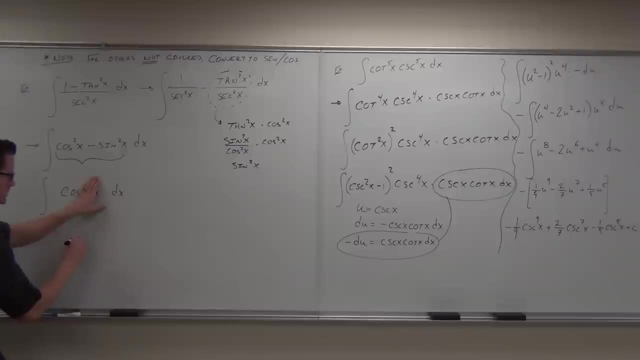 If you do a u sub right off the bat with that you're going to have like 8 u subs per problem. That is going to suck. So I just do in my head I go: OK, what's the integral of cosine? 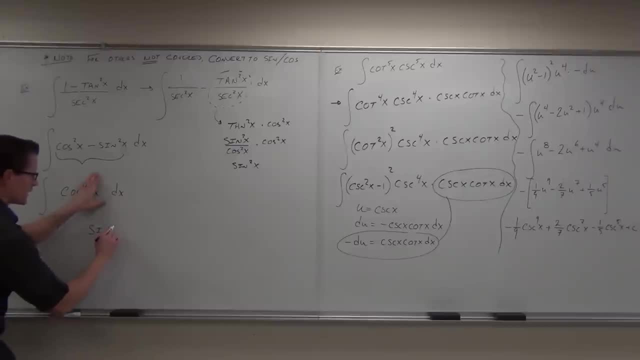 It's positive sine. Whatever's on my hand, I don't change, But I divide. I divide by the derivative of whatever's on my hand. It's like the opposite of a chain rule: Instead of multiplying by derivative, you just divide by derivative. 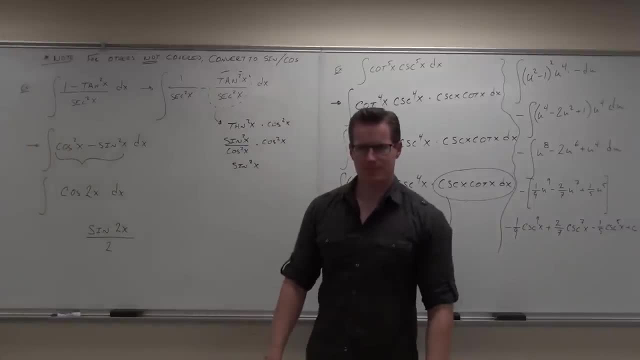 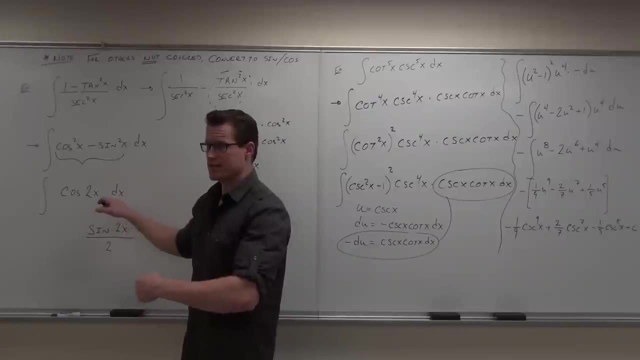 And that works. Does that make sense to you? That's doing u substitution in your head. That's a u sub in my head. I'm doing: u equals 2x. right Derivative is 2.. dx equals du over 2.. 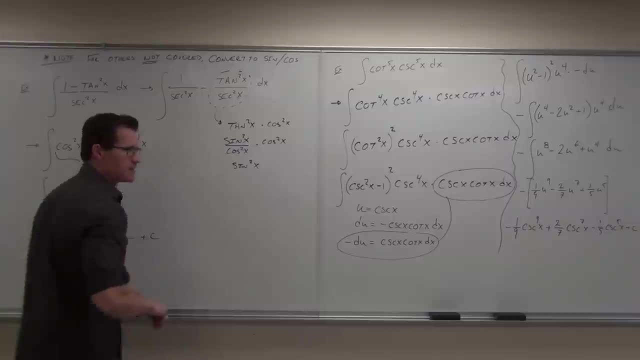 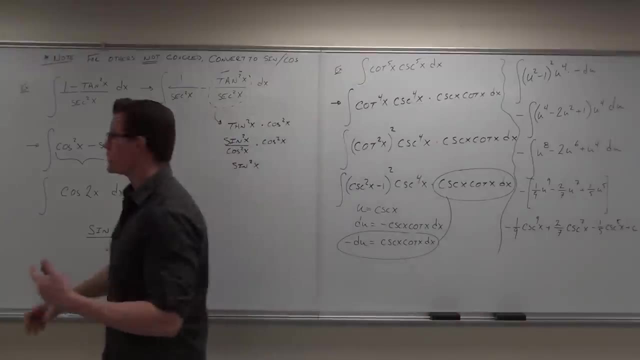 That's where the over 2 is coming from, Plus c. lets me know I'm done And I'm done. So if hands feel OK with that one, look at those and try to use them. Identities are nice. Try to use those. 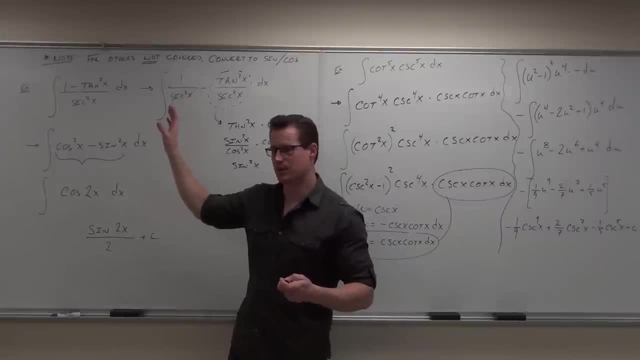 And the ones that don't follow the pattern. you are going to have to change the sine and cosine for most of them. Once you do that, please, for your sake, look at some identities and try to work with them. Just follow the correct identities down. 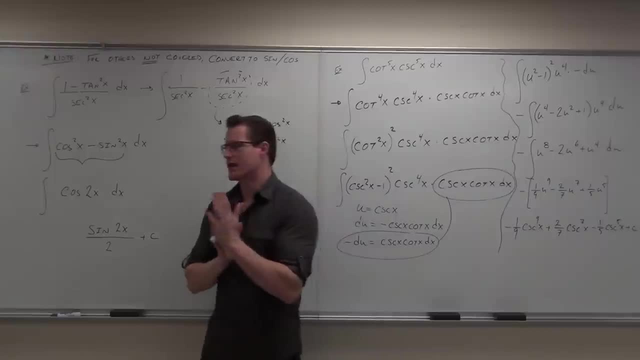 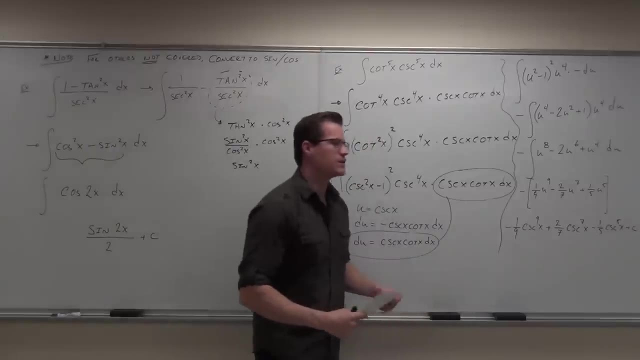 and you'll be good to go. Can we move on Now? there's one more thing that we haven't talked about that I want to give you one example with- And we'll call it a day. Have you noticed, in all of these patterns, that these angles? 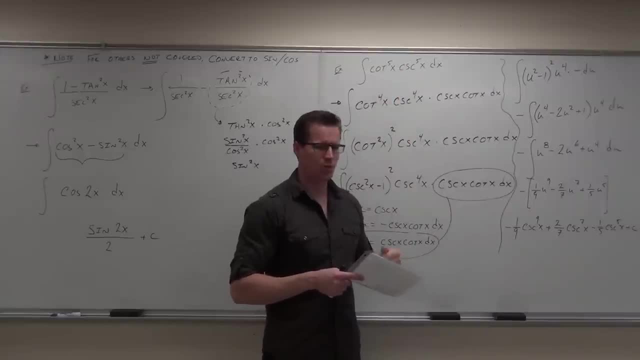 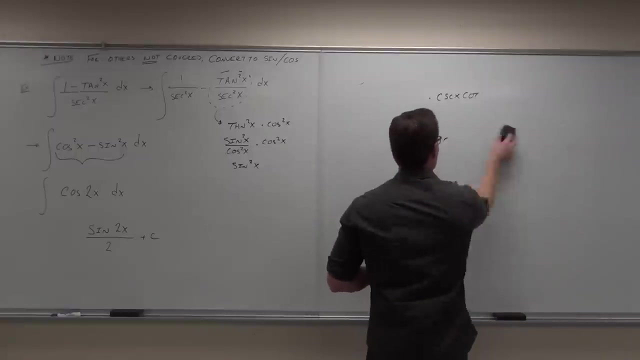 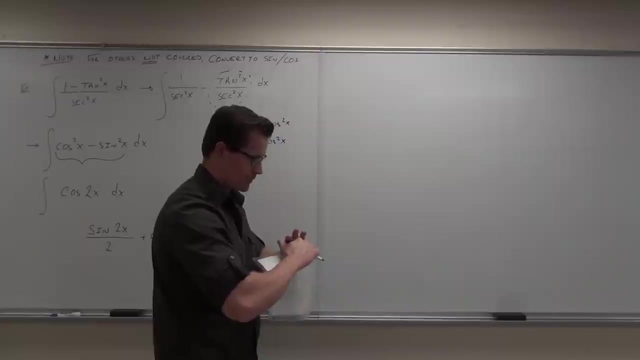 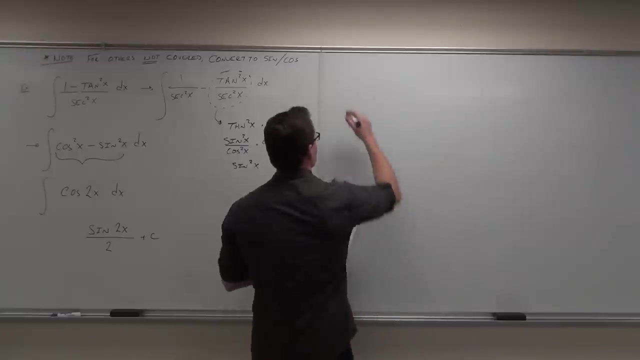 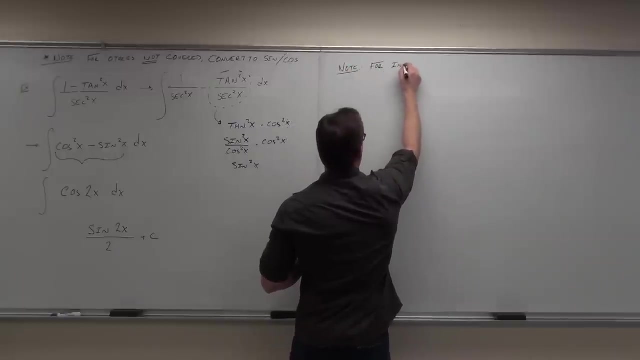 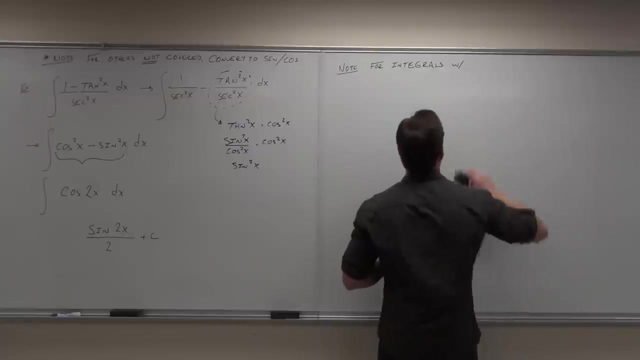 These angles are always the same. Have you ever wondered what if the angles aren't the same? Have you wondered that We're going to do one like that right now? So what happens where the angles of sine and cosine are different? So for integrals, where sine and cosine 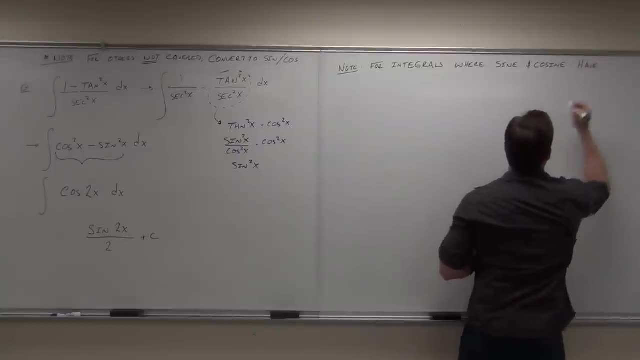 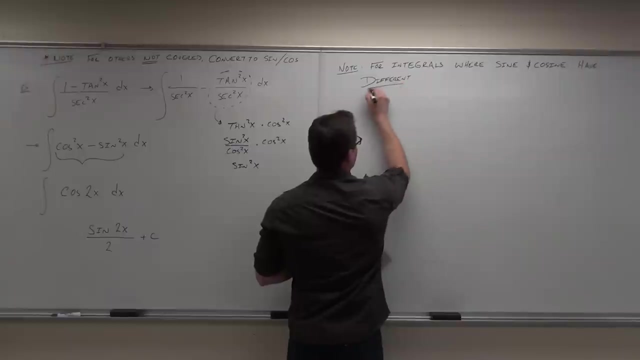 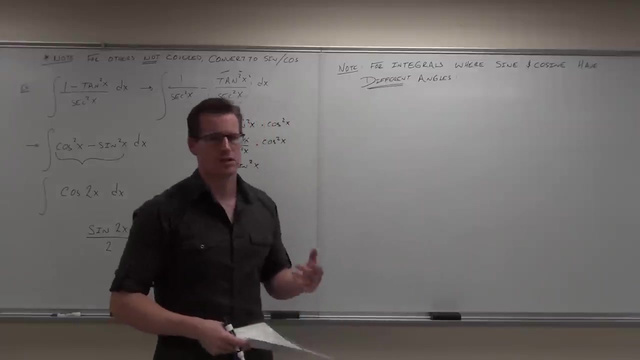 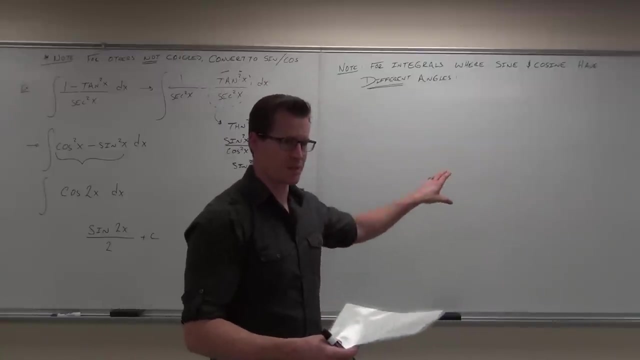 have different angles. try using these three identities Again. of course, with trigonometry we almost always go back to identities at some point. Even with our basic patterns we're using identities. Same thing happens here If you've got integrals with two different angles. 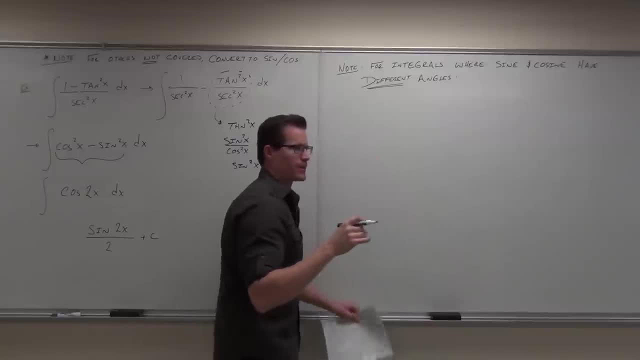 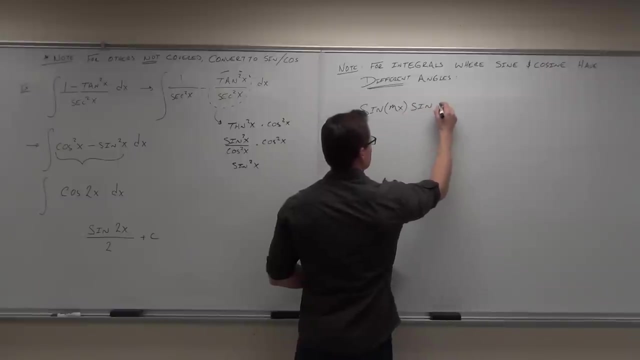 this is what you do. There's three cases. There's where you have two sines, where you have a sine and a cosine, or where they have two cosines. There's only three cases. So let's suppose I have sine, times sine. 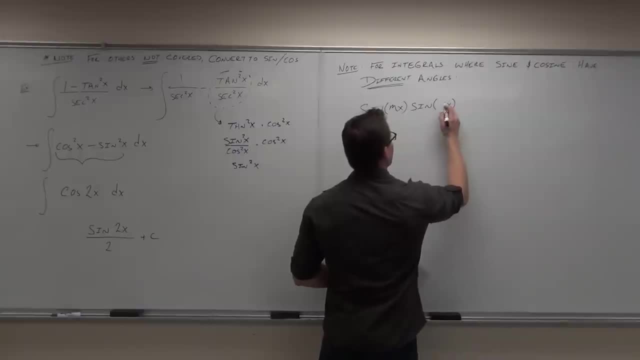 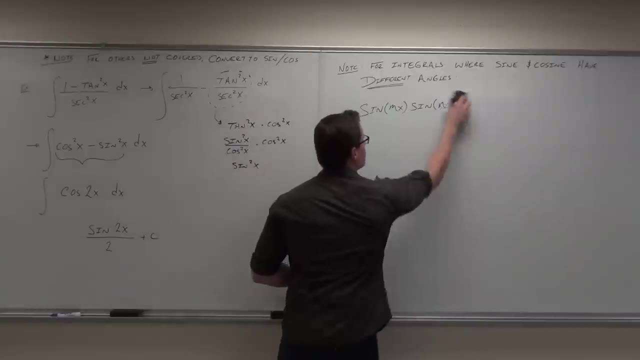 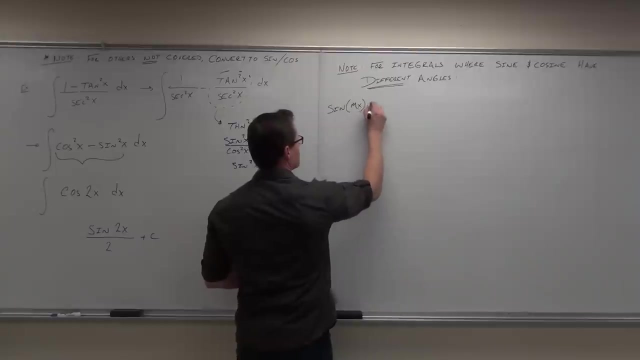 where the angles are different. Where the angles are different, You know what? I'm going to need: more room. Let's write that down. I'm going to write it just over here a little bit. Or where we have a sine and a cosine. 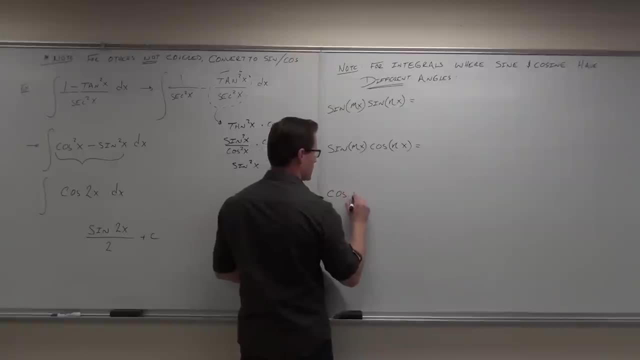 where the angles are different Or, lastly, where we have a cosine and a cosine where the angles are different. Here's some identities. I don't know if you've ever seen these before. You may have, I'm not sure. 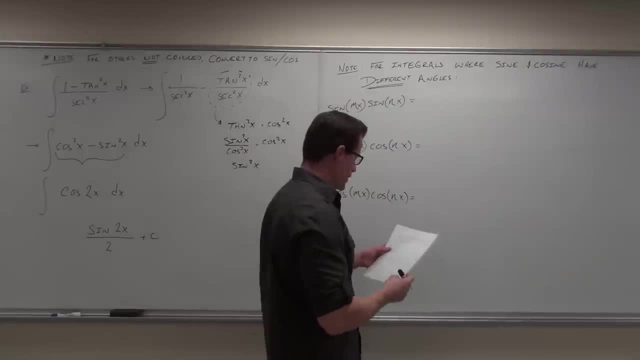 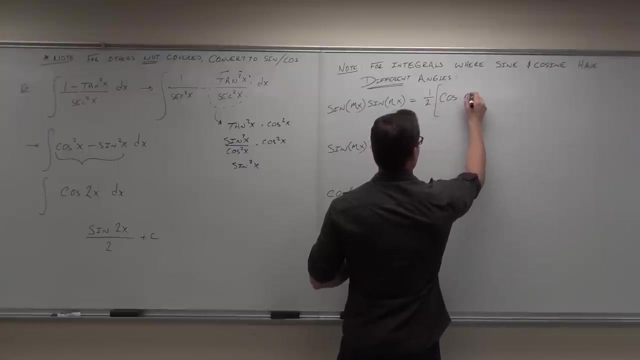 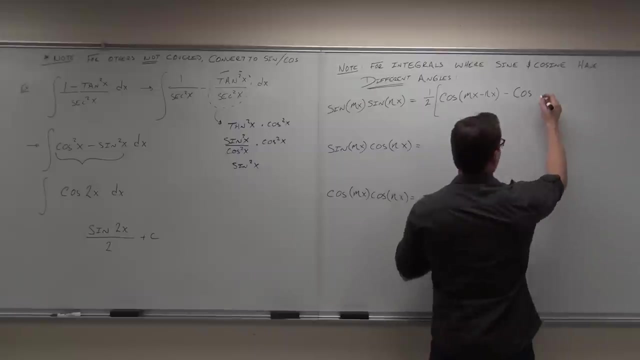 You probably have somewhere, But we don't use them very often. Here they are, So if you have sine of something times sine of something where your somethings are different, here's how to do it, Probably something you're going to want to write down. 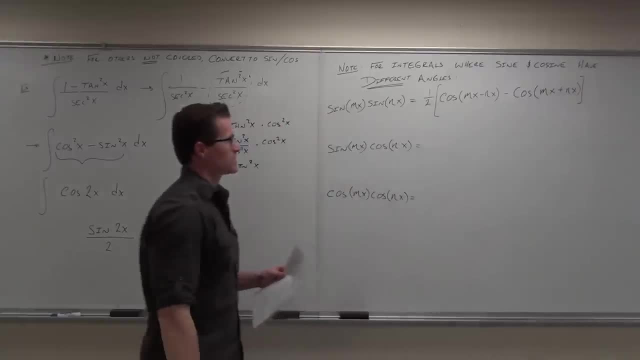 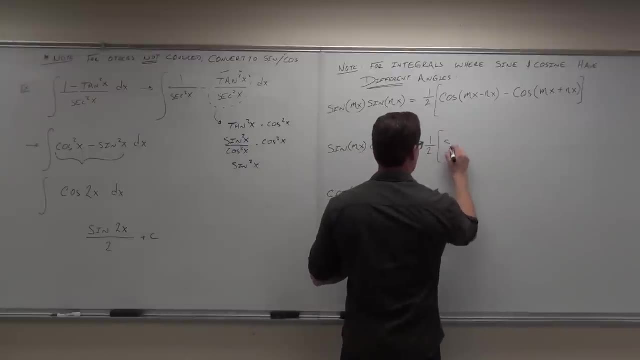 and have next to you when you're doing your homework. At least I would, Problem 40.. Did y'all solve that? Yeah, Problem 40.. Let's do it, trying to equate ourанизms. You're not allergic to this, are you? 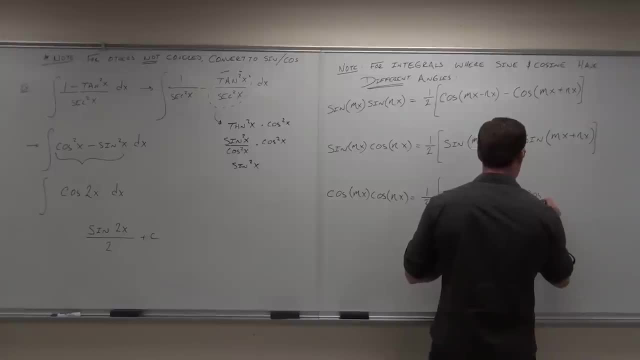 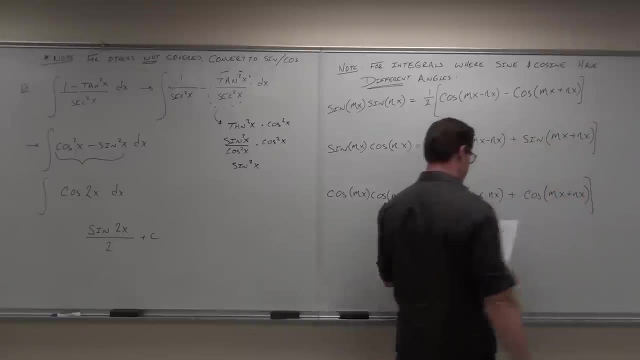 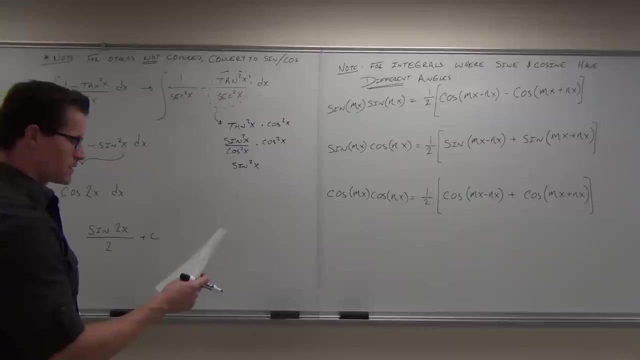 Okay, goodness, I've got to make sure I'm right too. so let's look at that. One half cosine, yes, minus cosine, okay, good, and that one, cool, and that one, okay, write them all down. 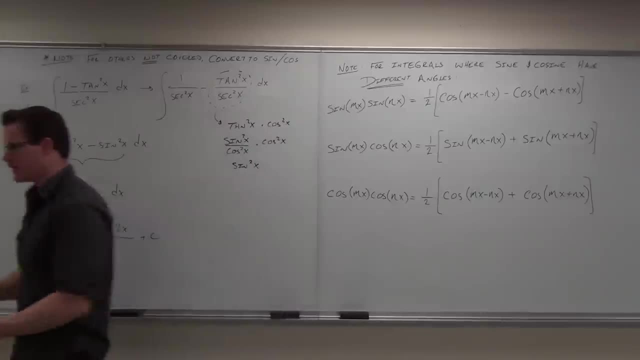 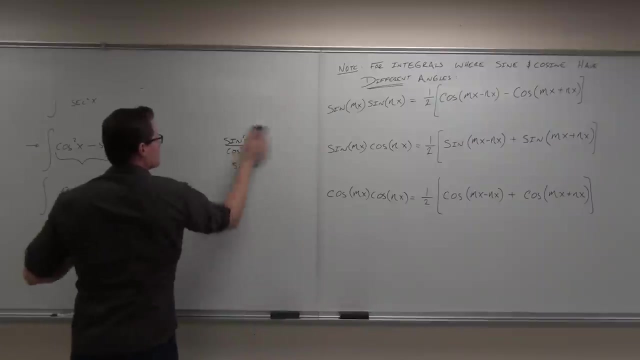 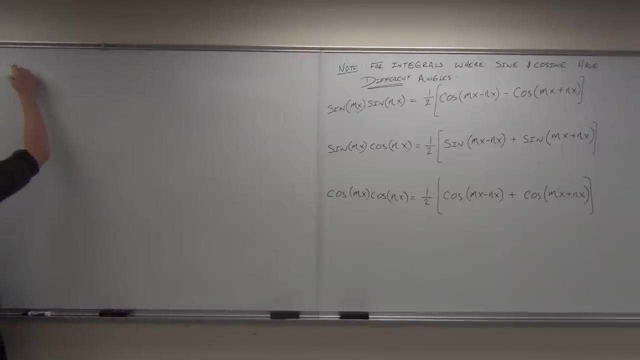 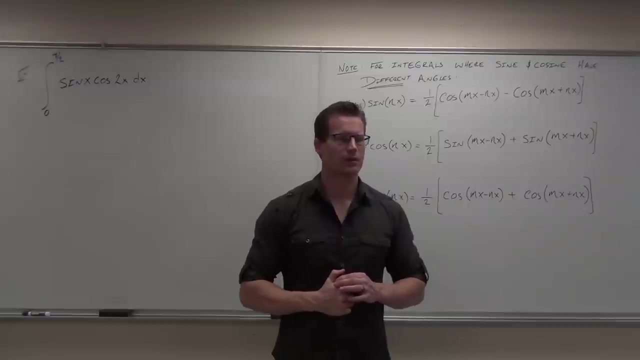 Look up here when you're done. That way I can talk at you. We're going to do an example here, So continue writing and let me know when you're done, And then we'll do an example. So here we go. All right, have you written all down? 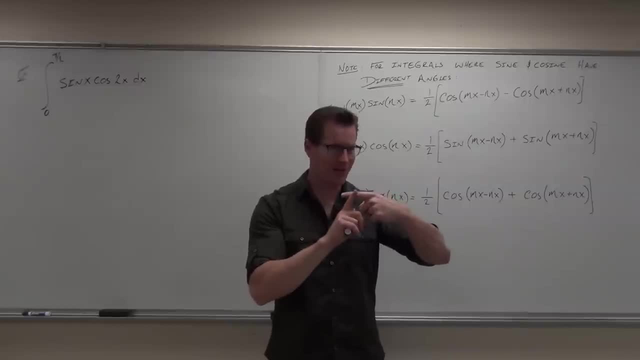 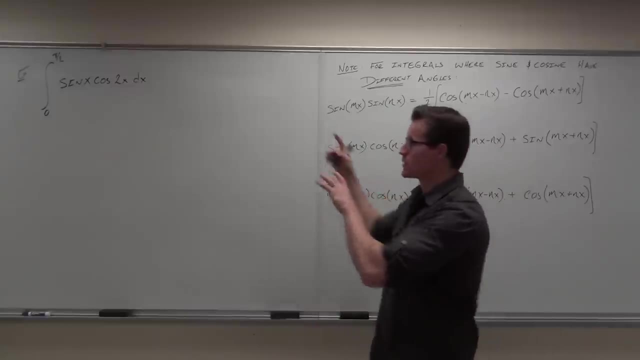 You got this perfectly right: Sign for sign, pluses and minuses, sign for sign as well. okay, good, So let's check this out. If I hadn't told you this, could you do that problem? Well, you might. 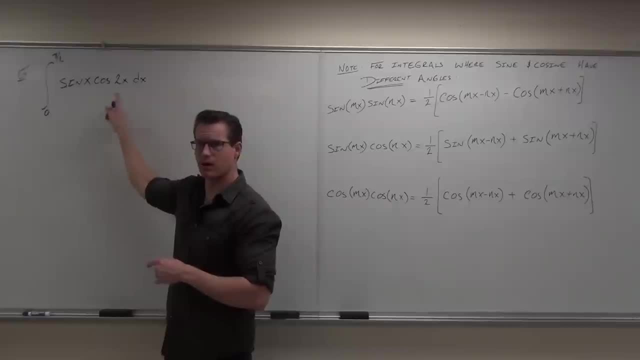 You might be able to change this, because it's a problem. cosine two x- I'm sure there's an identity for that one, But we have an identity that will change this directly and make it a lot quicker, a lot easier for us. 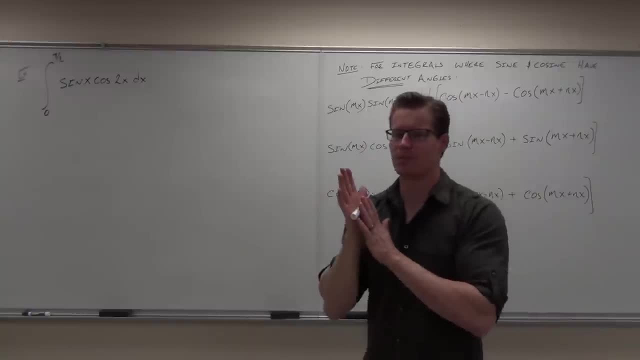 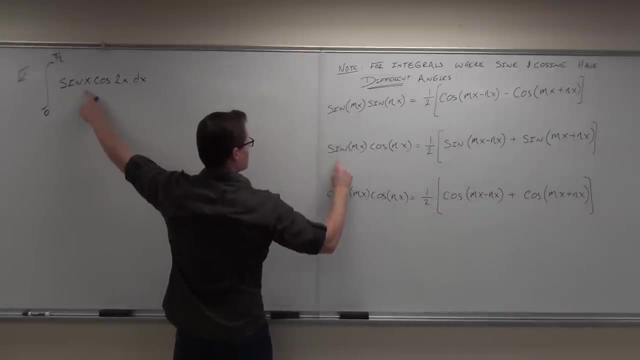 So let's check it out. We got sine x, cosine two x. Do you see what I mean about different angles? So what this says is: this would be our mx. it's just one x. This would. oh wait, which one are we at? 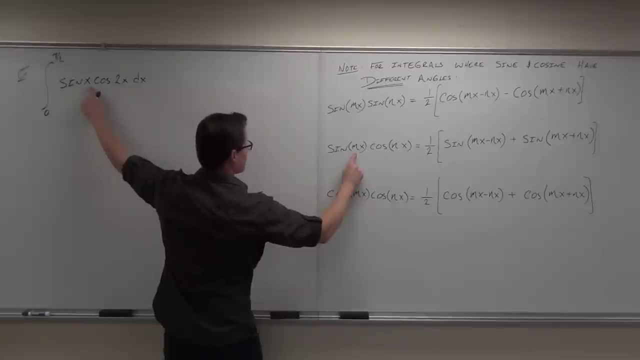 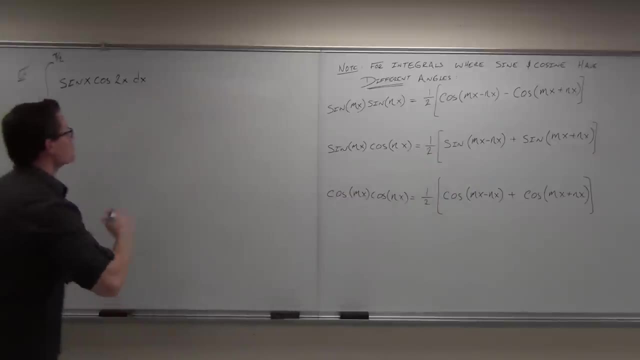 Top one, middle one, bottom one. So this is our one x, this is our two x. It's just basically says: look at this angle, look at this angle, do this with it. So when we're doing this with it, 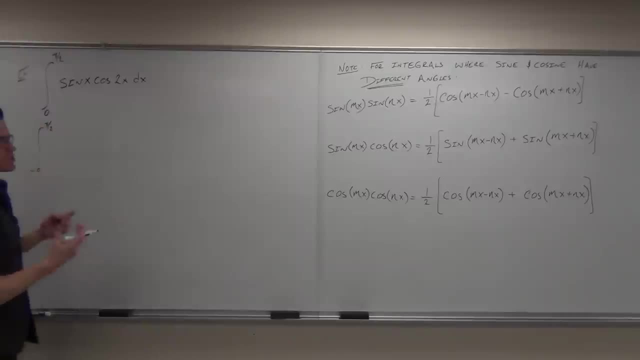 we still maintain our bounds of integration. We're just gonna do our identity here. So what's the first thing that we're gonna do? One half, One half's gotta be there. What are we ultimately gonna do with that one half? 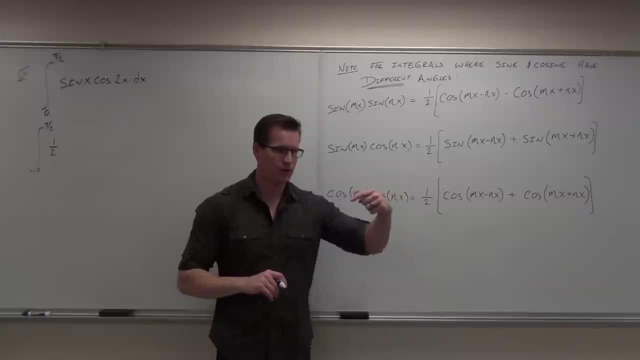 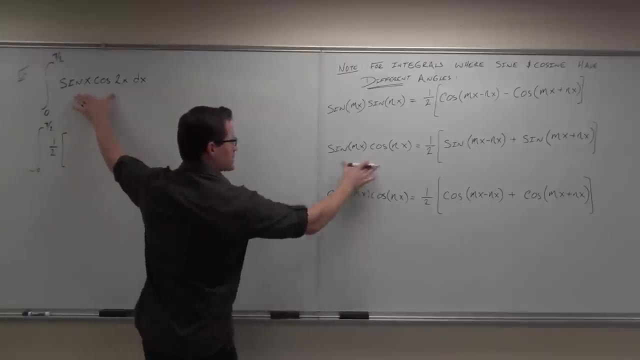 Contribute it. No, we're not gonna contribute it. Oh, We're gonna pull it out. Okay, so I'm gonna draw my bracket here. Let's change this using this identity. Tell me the first thing I'm gonna write. 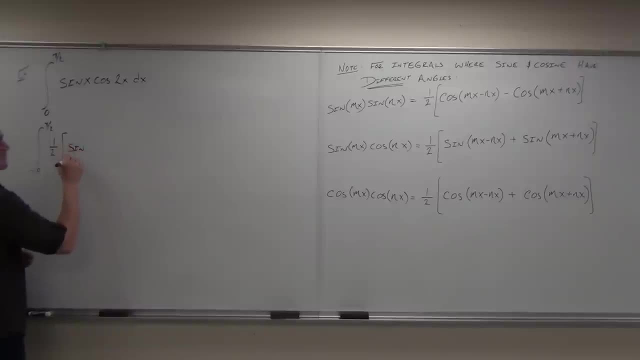 inside of my bracket, Sine, Sine of what Sine of x. Good, that just says this angle minus this angle X. Oh, x minus two X minus, not two x minus that X minus two x. 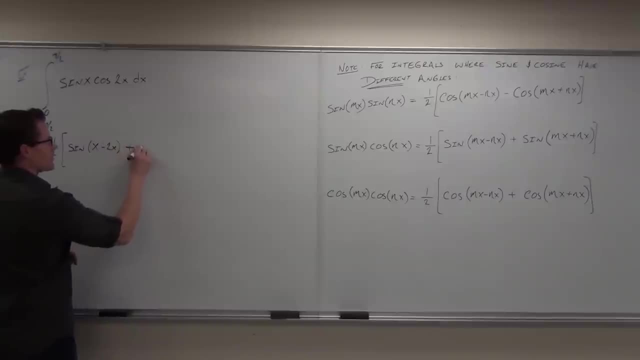 Okay, what else Plus? There's a plus holding those together, And then another sine, and then what? X plus two? x plus two, Perfect. So you get your d x's. Let's simplify it a little bit. What do we got here? 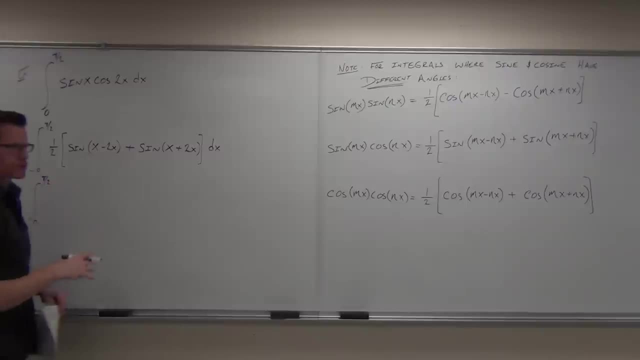 Pi over five minus x, Still zero to pi over two. We're not gonna change those. yet We haven't done any substitutions, So we still have that. What now? One half. One half is out front. Okay, what now? 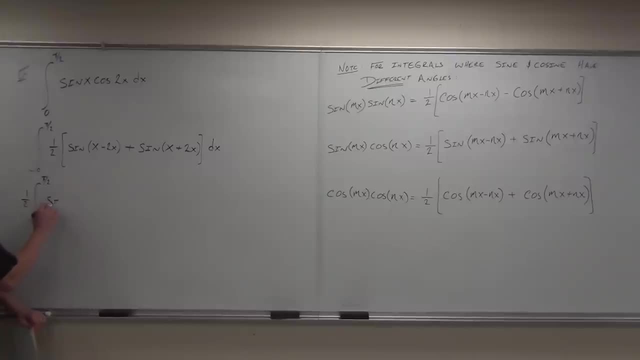 Sine of x. Wait, sine of what? Negative x, Positive x, Sine of Negative x. Combine them: Negative x, Negative x. You okay with sine of negative x. Does it equal negative sine of x? Are you first I wanna make. 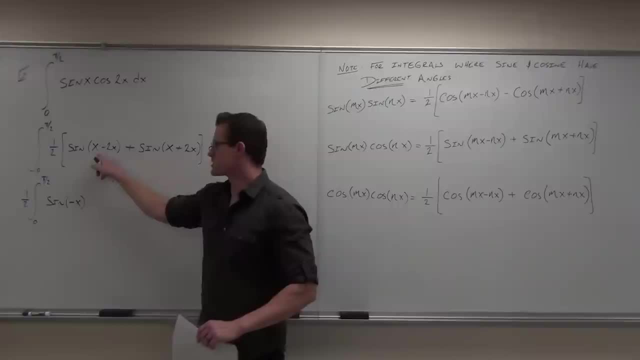 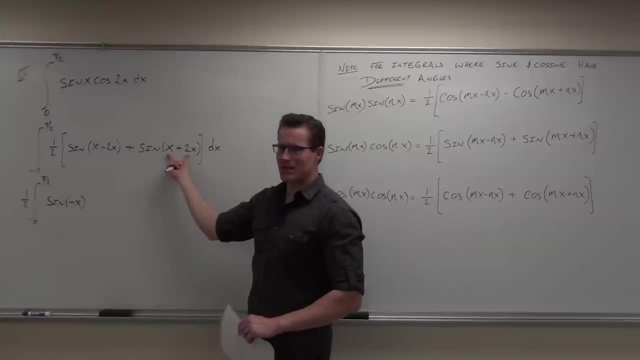 I get some weird looks. I'm not like: what are you doing? What's x minus two x. Negative x? Okay, you can do this stuff. okay, Just combine them. They're inside the parentheses: X plus two x's. 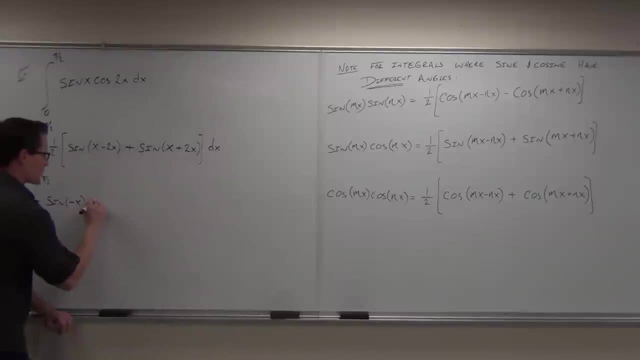 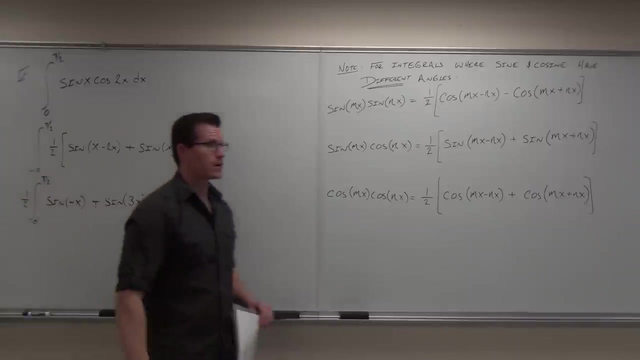 Negative. Some of you are thinking so hard you're missing the easy stuff. That happens a lot in this class. Quick hit note if you're okay with that so far. The reason why this exists is so that you can actually combine the angles. all right. 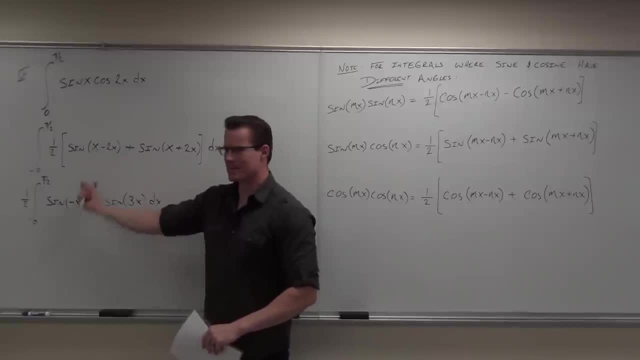 You wouldn't? this looks crazy. I mean this: yeah, combine the negative x and the. now, this is an issue because we don't wanna end with the sine of a negative x. We want sine of x. We wanna end with that, or whatever we have here. 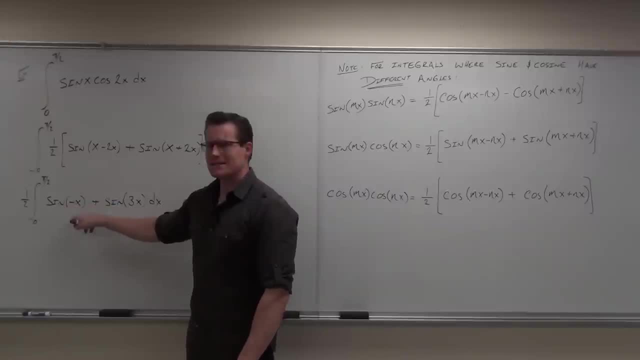 So let me cosign. actually, you need an identity for this one: Sine of negative x. Negative x equals Sine of sine of x. Good, it's an odd function. So when we do this, you're all right. this is not a problem. 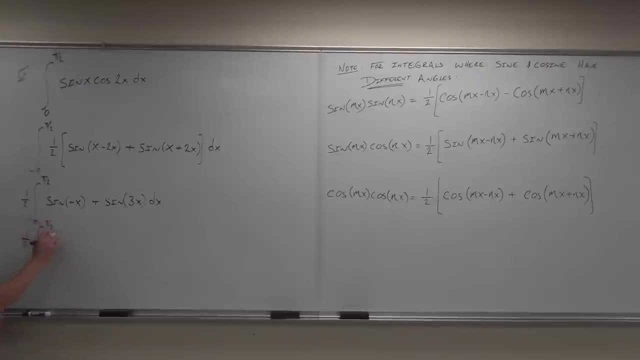 This will be one half zero to pi over two of negative sine of x plus sine of three x dx. Let me ask you something: Can you do this integral? That's a piece of cake. It's not cosine. What's the? Can you do this integral? 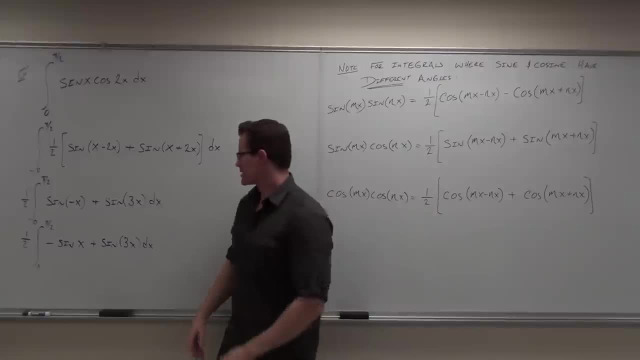 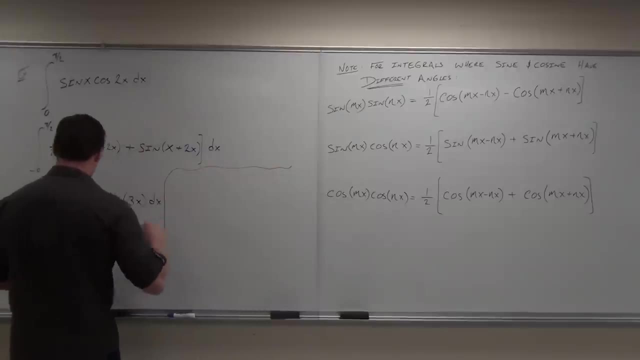 It's a piece of cake too. No problems, Let's do the integrals. What's the integral of? and let me write this out here: One half's gonna be there. no problem, Let's create a bracket here, so we don't lose anything. 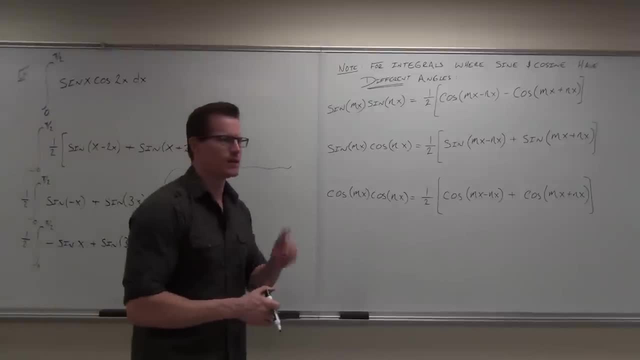 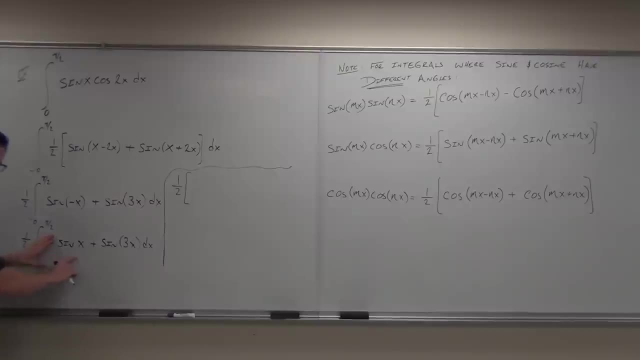 What's the integral of sine x? Can you tell me? Negative cosine, Negative cosine. So watch carefully, I'm gonna do some math in my head here. If this gives you negative cosine, negative cosine, This gives you Cosine x. 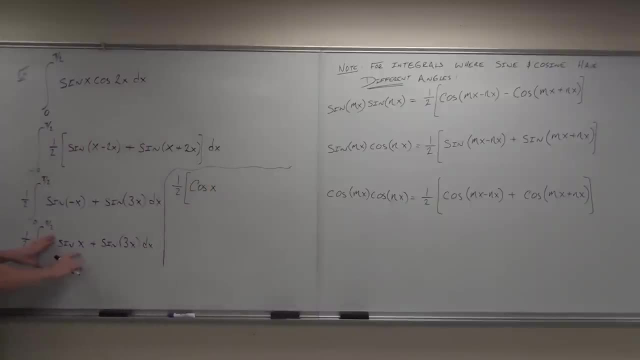 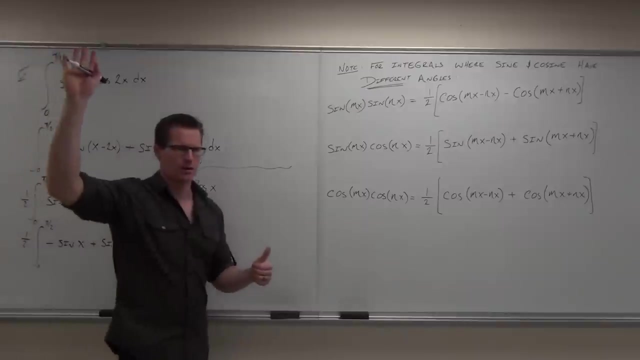 Cosine x. This would give you integral of sine. x is negative cosine, So negative. integral of negative sine x is positive cosine x. Show me if you should be okay with that. one Double negative, Okay, double negative. Two wrongs: make a right here. 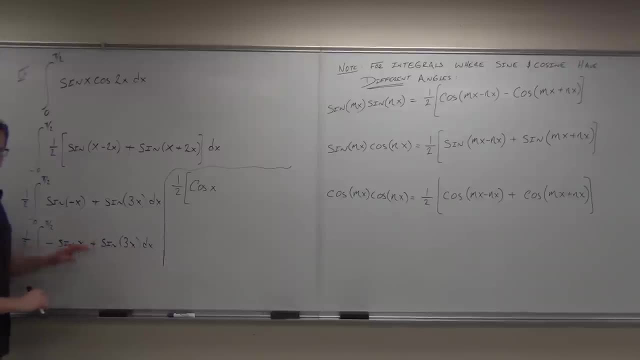 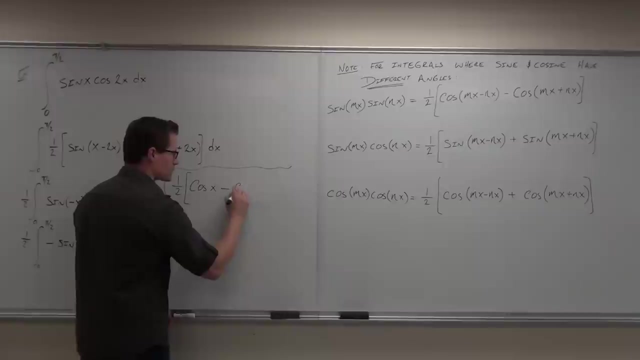 So let's do the next one. What's this gonna give you? Negative cosine three x. Negative cosine three x. Okay, so instead of plus, I'm gonna have minus Minus Cosine three x Divided by three. 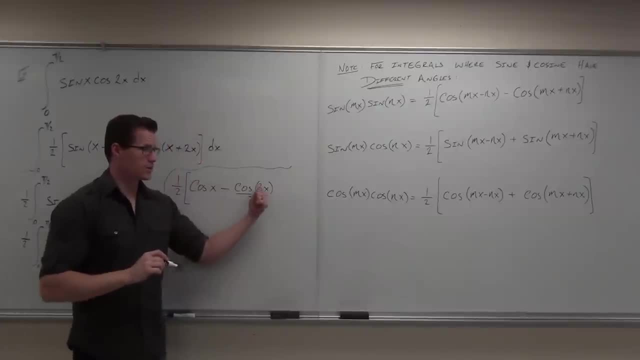 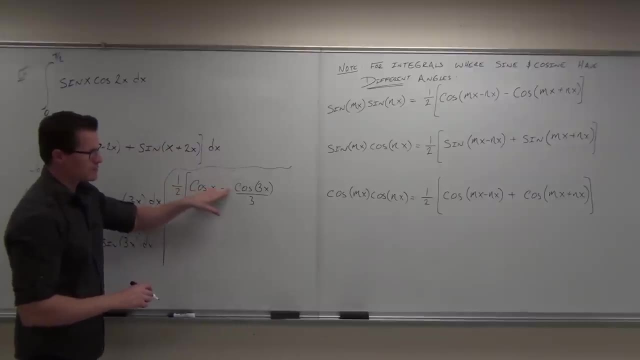 Oh, divided by three Over three- That's a little use-up in your head- the over three. So when you're doing these, do the integral, No problem. Negative, so minus negative, so minus cosine three x over the derivative of three. 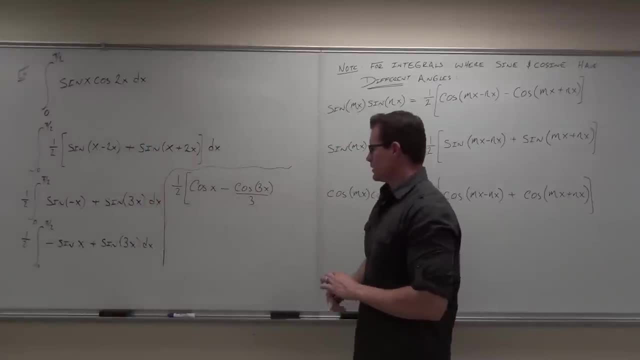 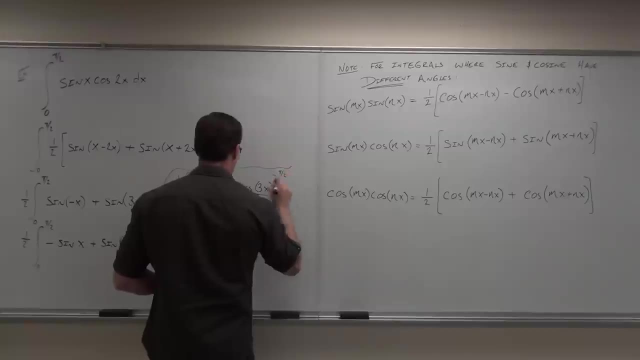 Show me if you should be okay with that. one Good deal. Now what? How do you do a definite integral Cosine two, So you could choose to distribute that if you really wanted to. You don't have to. You can wait til the very end. 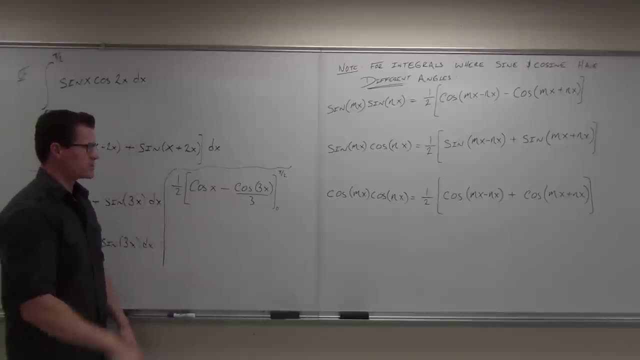 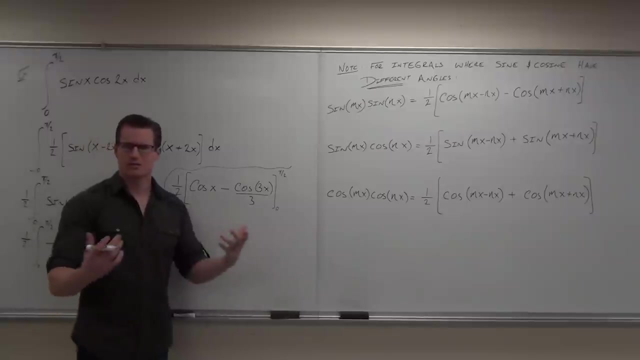 I would I like dealing with this and that separately. You could actually divide out a one-third. if you want, You could do divide out a one-third. this would become three cosine x minus cosine three x. Not a problem, That would get rid of that fraction in there. 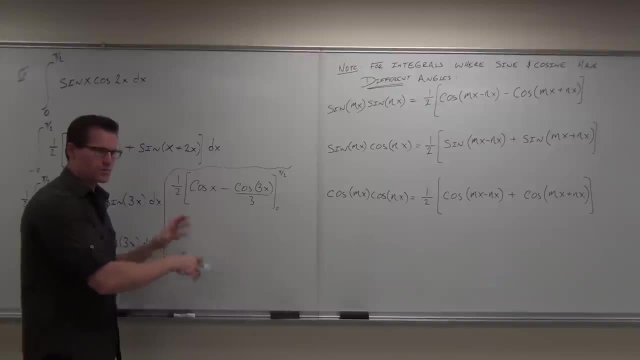 So, whatever you want to do as far as this goes, This is just algebra, Just plugging in some numbers and doing it. So I'll leave the one-half. Just remember that in here when you, when you have done some of this. 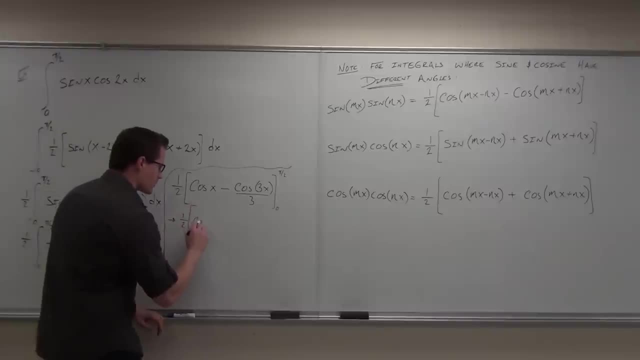 just remember that in here when you, when you have done some of this, just remember that in here. when you, when you have done some of this, when you, when you evaluate, you'll have cosine of pi over two minus cosine of three times pi over two. 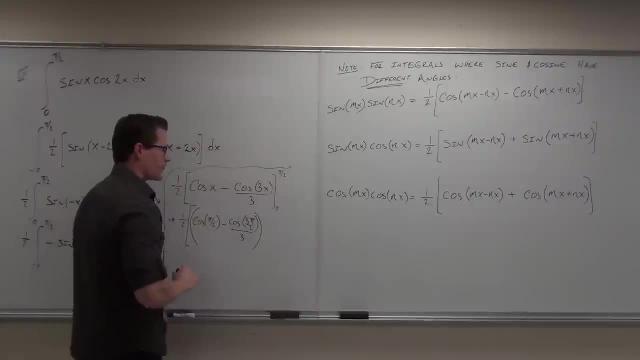 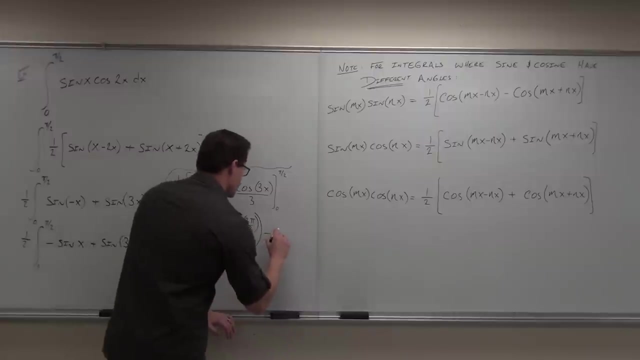 That'll give you nice numbers. Should I bother to plug in zero? Yes, For heaven's sakes. yes, Yeah, Minus cosine of zero, minus cosine of three times zero. What about the one-half Minus cosine of three times pi over two? 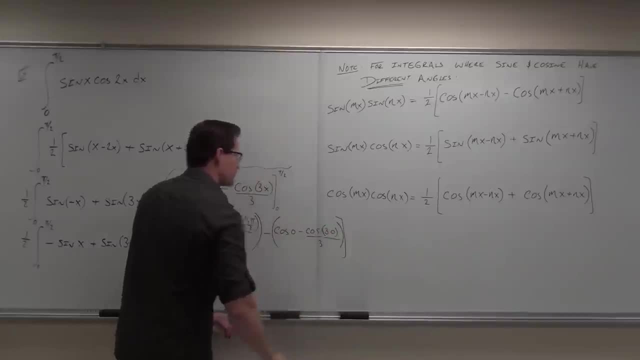 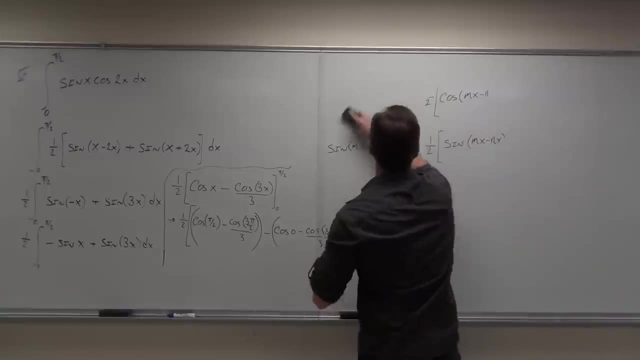 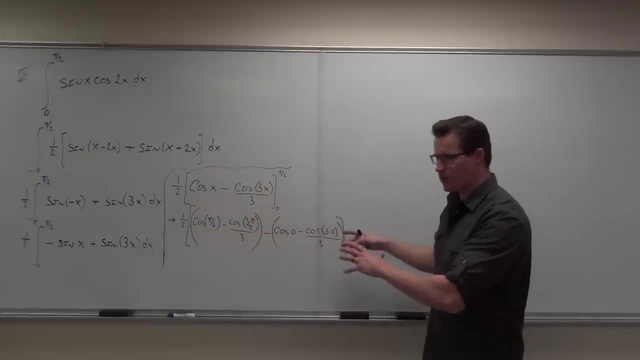 Over three. I don't think I forgot anything, but you let me know if I have. Have I forgot anything? No, Okay, so we got the one-half. we got the one-half. Big old bracket. You need the big old bracket. 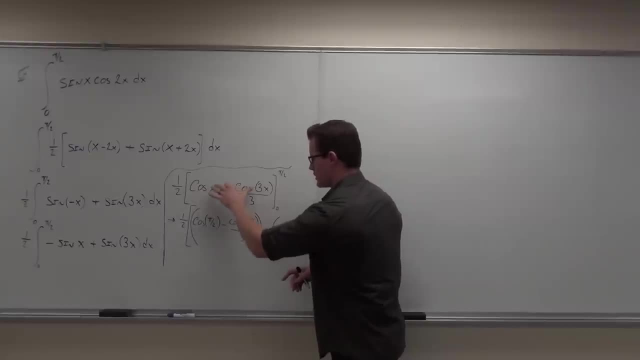 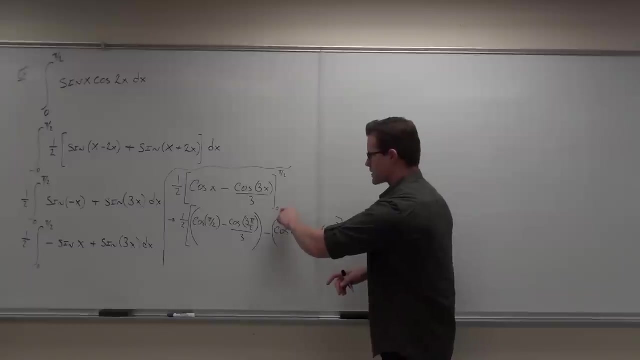 This is the evaluation of pi over two, So cosine pi over two, cosine three times pi over two over three. Are you guys okay with that? one Minus, No problem, Because you subtracted this Cosine of zero minus cosine of three times zero over three. 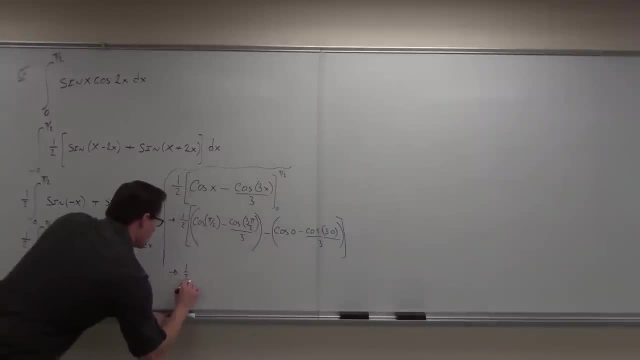 Let's work it out. So this will give us one-half Big bracket. Don't lose things here. What's cosine of pi over two? Zero? How about cosine of negative? I'm sorry, cosine of three, pi over two. 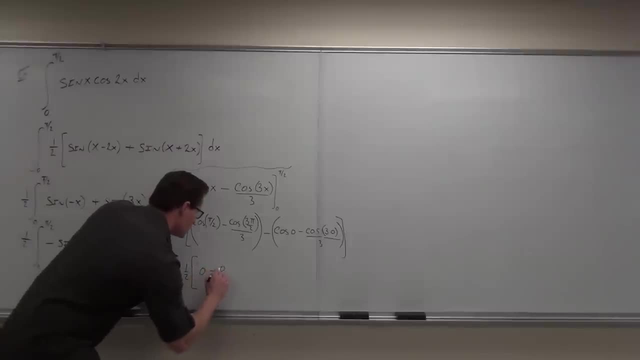 Zero, Zero, Zero, Zero. over three. Big difference: Cosine of one, One. Oh shoot, Cosine of zero. Cosine of zero is one. How about? this is also cosine of zero minus one-third. Don't forget about the three. 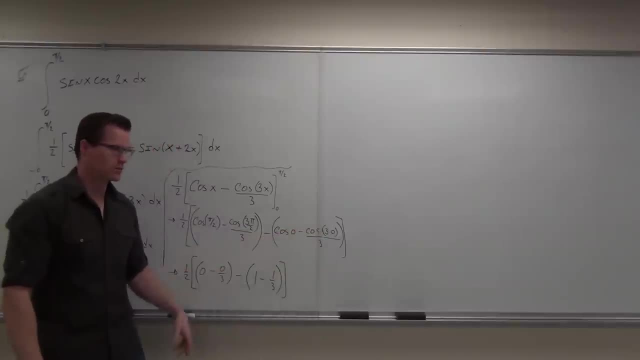 This is one-third, You okay, Forget about the three. This whole thing goes to zero. You go wait a minute. That doesn't make sense. We can give an area that's zero. We can Complex analysis doesn't matter. 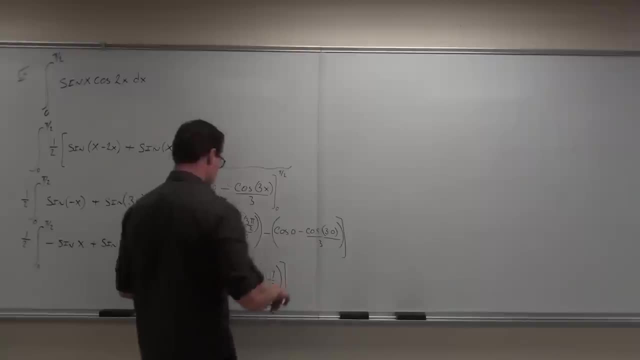 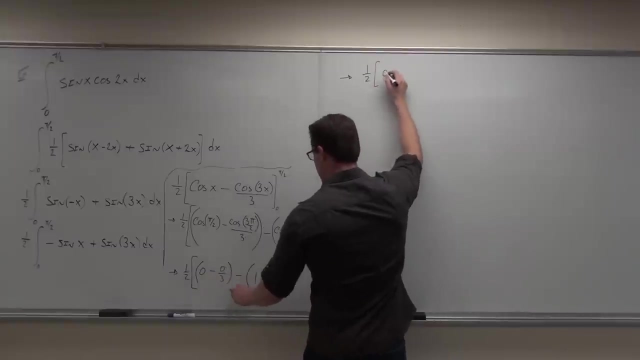 What happens here? Zero, Zero. So this is zero, One-half Zero Minus Two, Minus one-third. I get negative one-third. Did you get negative one-third? Yes, Yeah, We are done. Does that make sense? 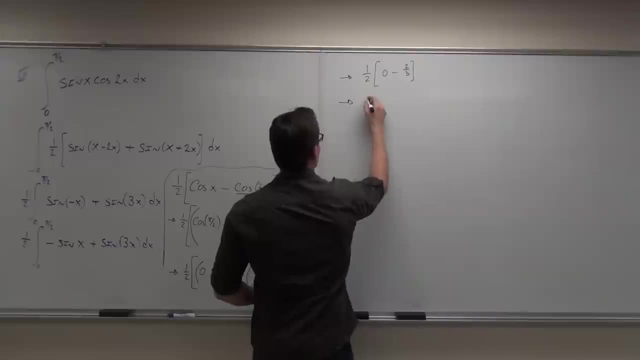 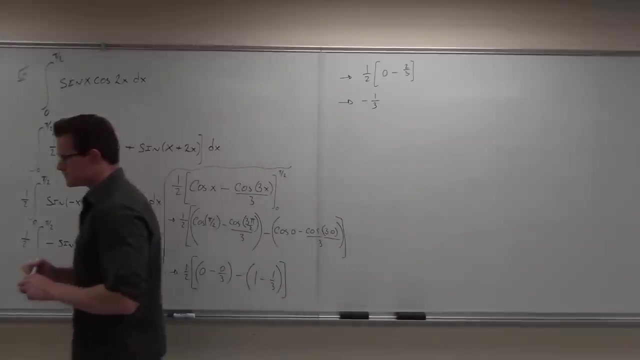 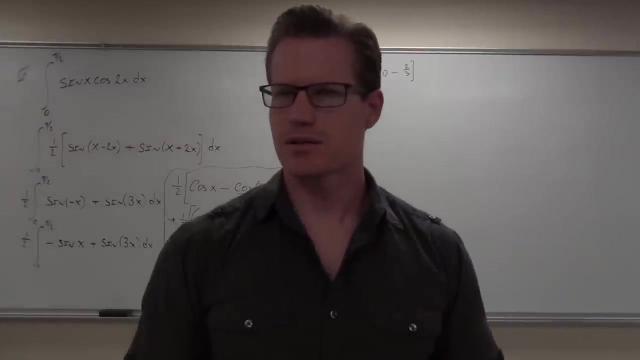 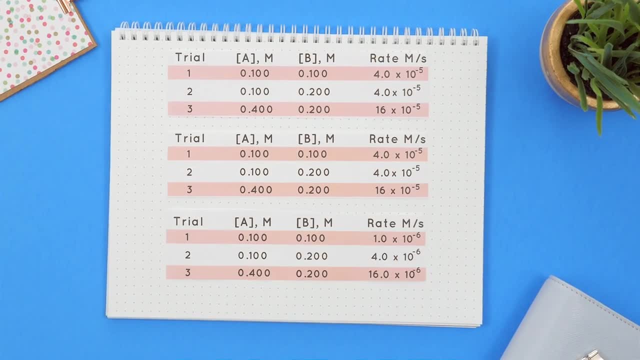 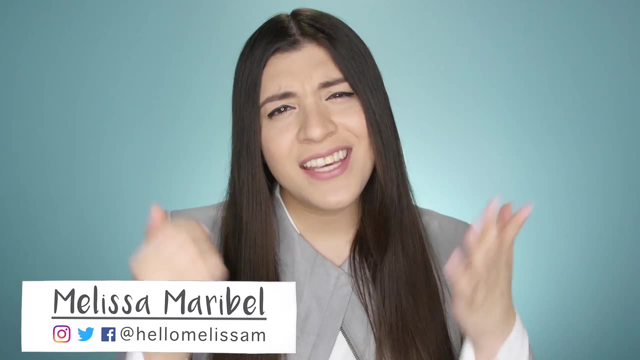 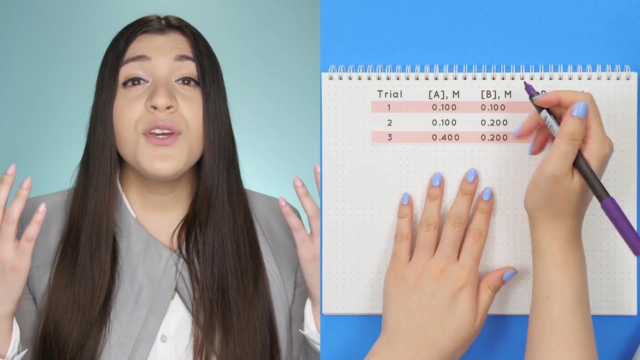 Looking at all these given tables, you'll be able to quickly figure out the reaction order by just knowing a few tricks. Hello everyone, I'm Melissa Maribel, your personal tutor, and here are the tricks. Trick one: zero order If you increase the concentration of the reactant. 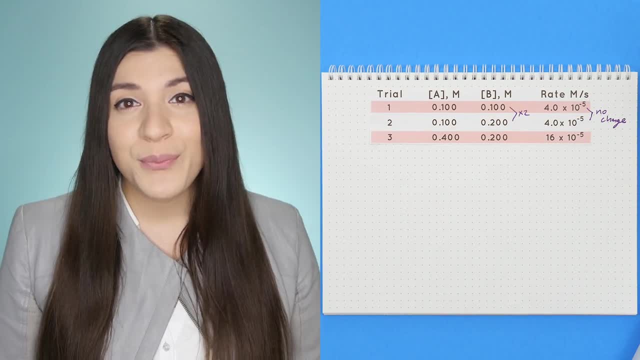 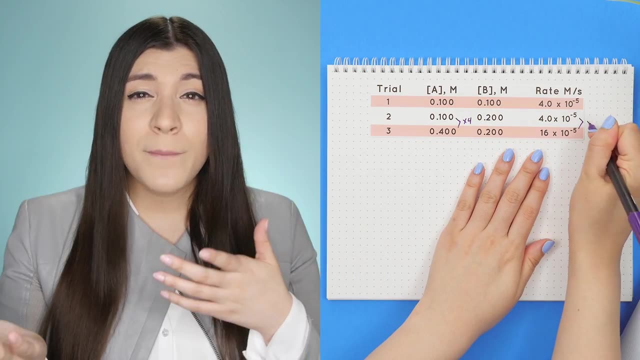 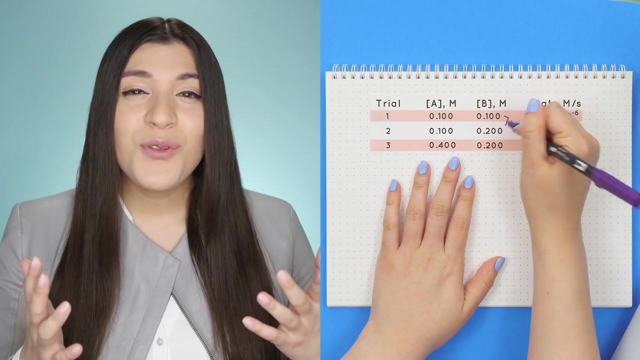 but the rate does not change, then it's zero order. Trick two: first order: If whatever you multiplied by your reactant's concentration is the same number you multiplied by the rate, then it's first order. Trick three: second order: If whatever you multiplied by your reactant's concentration, 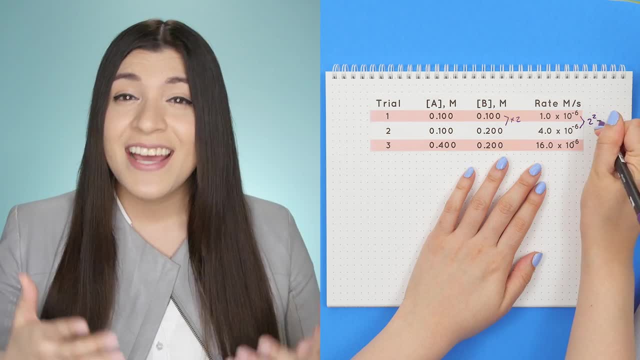 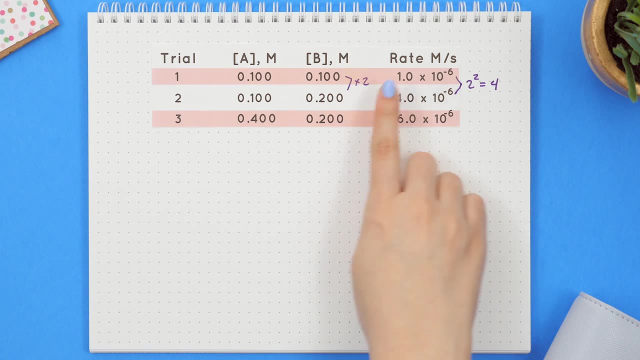 is the same number, but squared to your rate, then it's second order. Here are some examples: We are multiplying by two here, and for the rate we are multiplying by four. Since two is the same number as the rate, then it's second order.